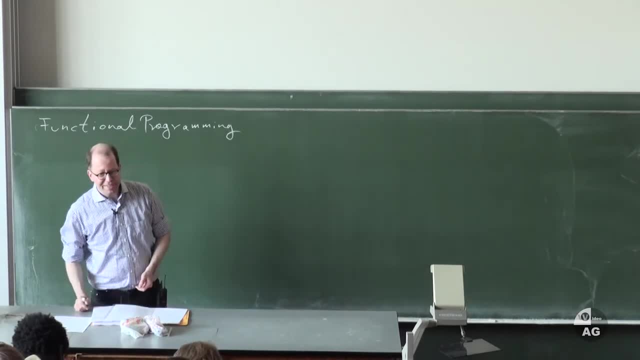 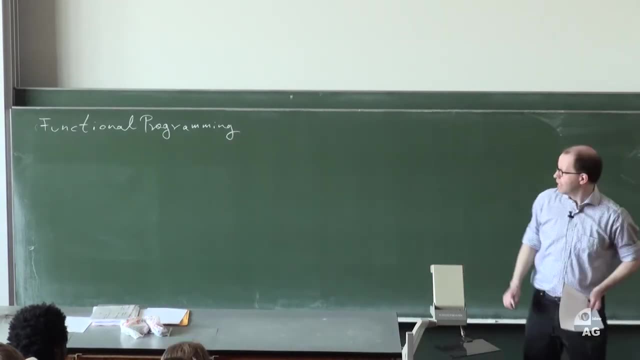 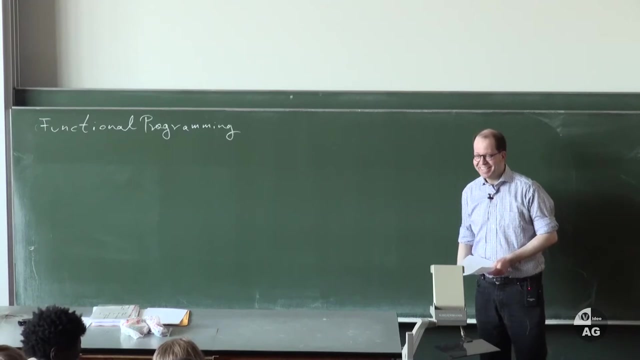 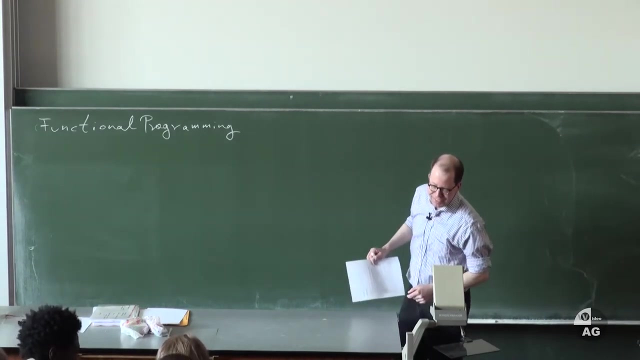 is about, and then I will. Some mobile phone is entertaining, Okay. so then you have an idea what the lecture is about, and afterwards I'll tell you something about the contents. Okay, as soon as the music stops, If you put it deep down into your backpack, Okay so, 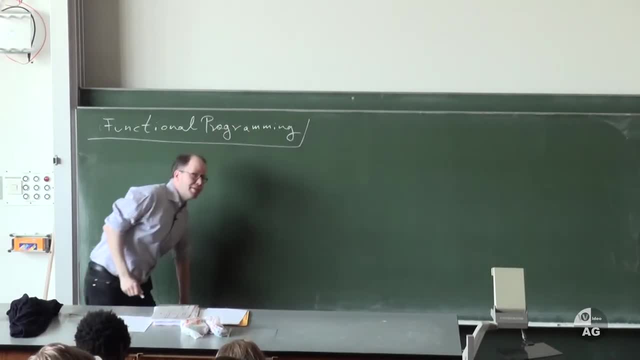 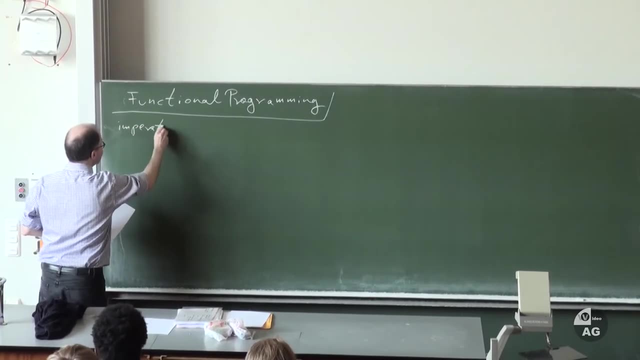 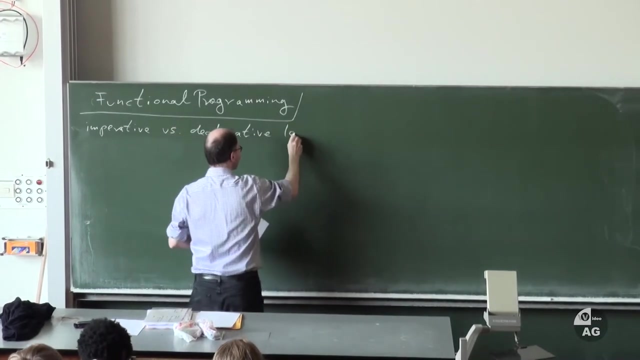 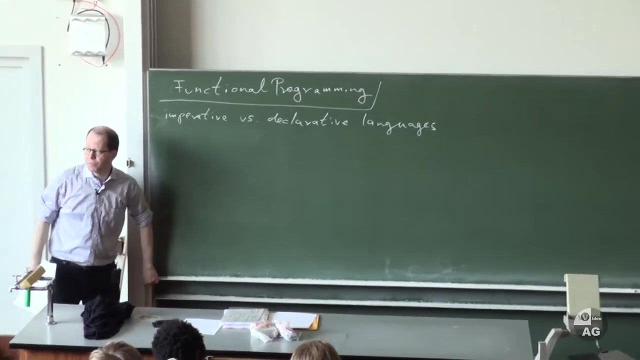 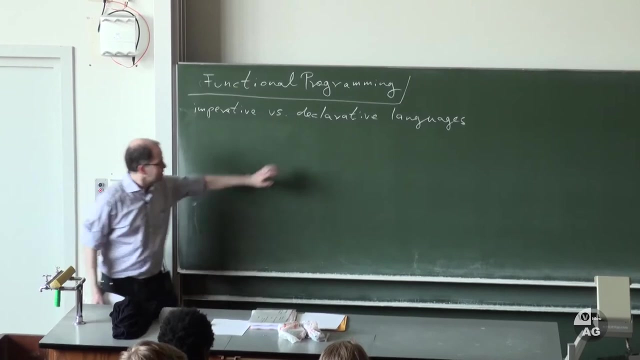 what is the lecture about? So, in principle, there are: There are two big families of programming languages, namely the imperative languages, versus the declarative programming languages. And well, imperative languages, these are the languages that you are probably most used to, and examples are languages like C, Java and whatever- And declarative languages, well, 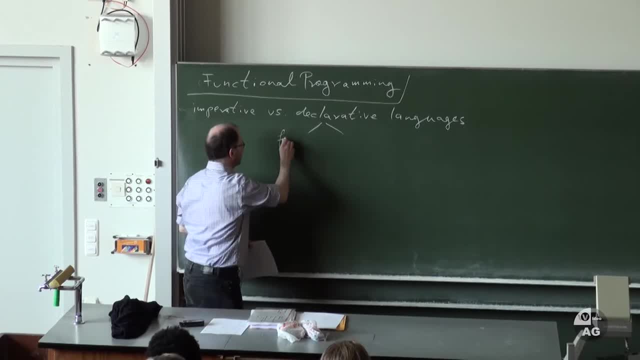 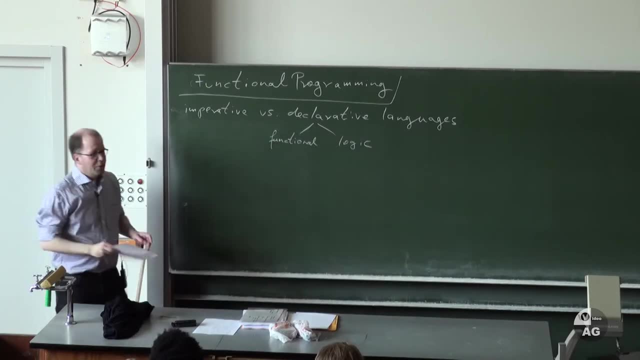 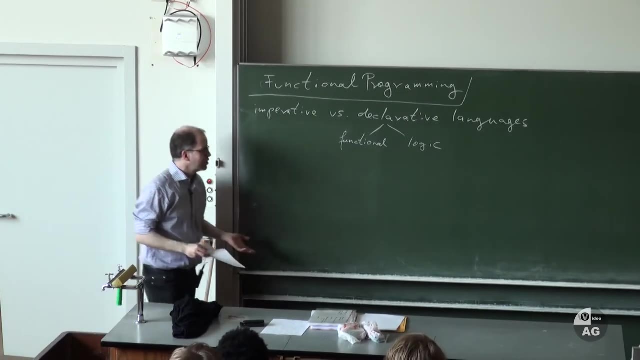 there are two big groups of declarative languages, namely functional and logic programming languages. And well, the essential idea is that these languages should be much nearer to natural language than to machine language. So this should be somewhat near to the way that humans 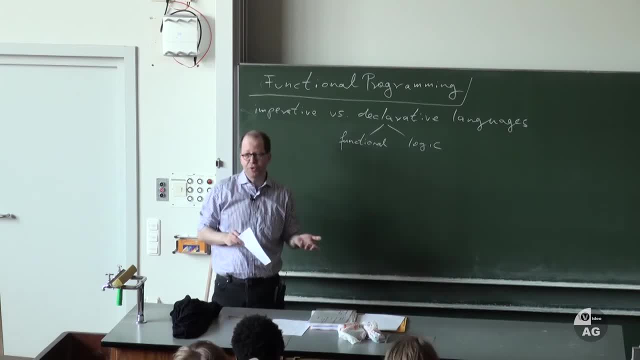 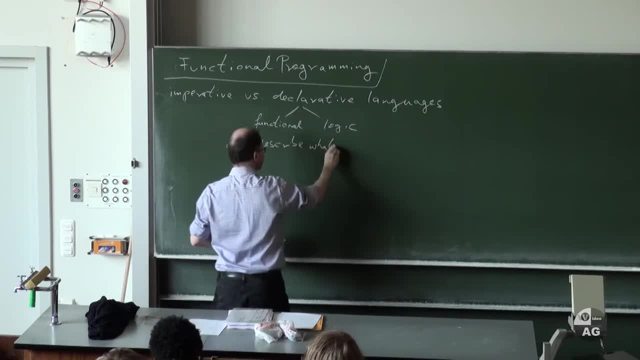 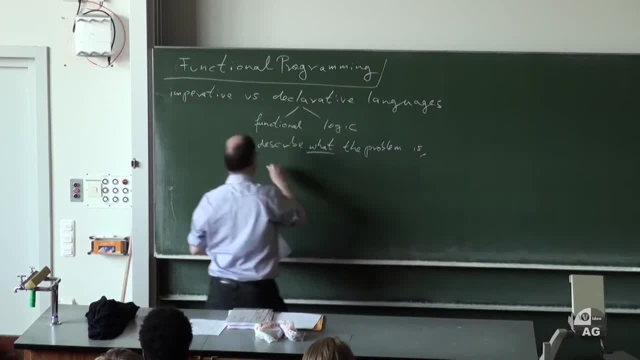 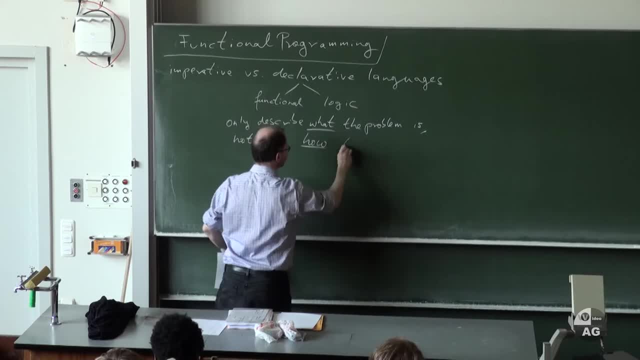 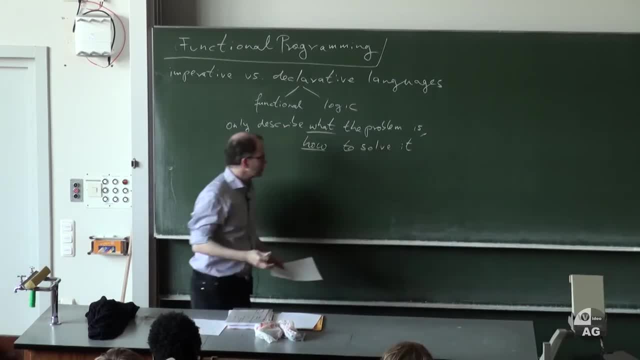 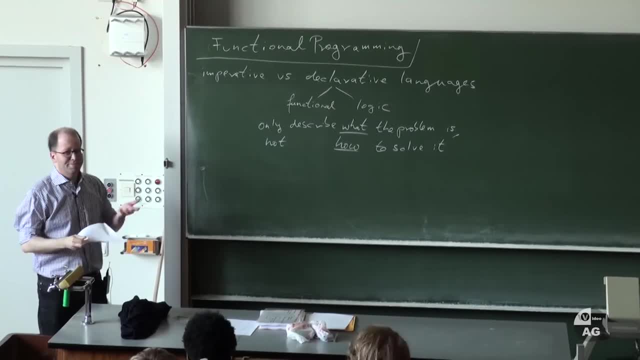 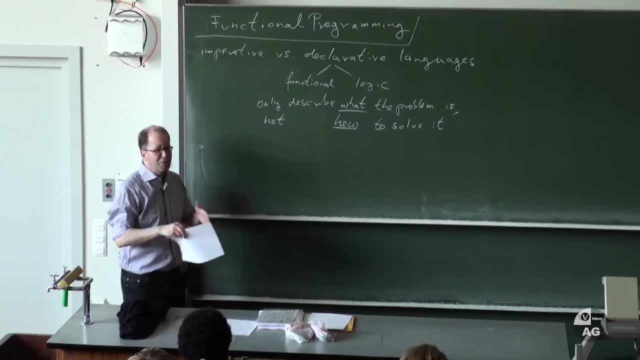 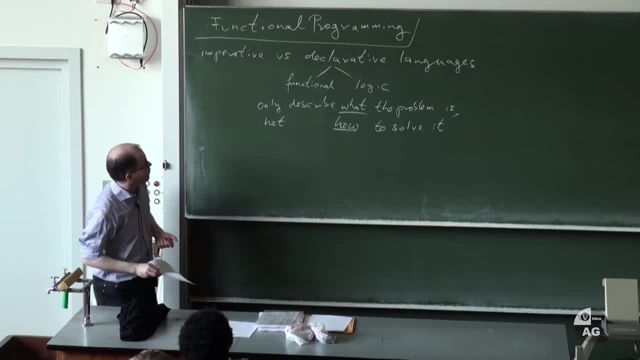 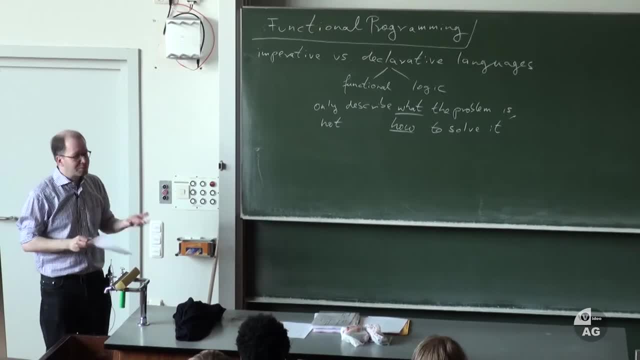 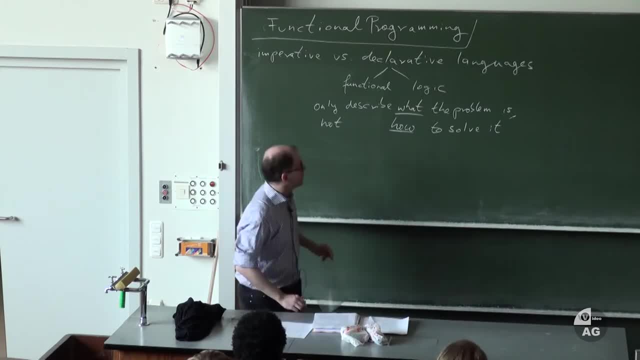 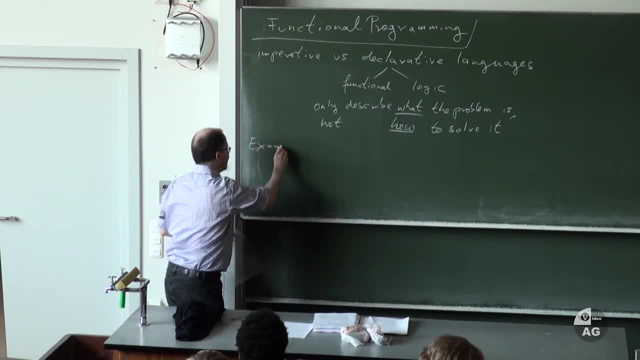 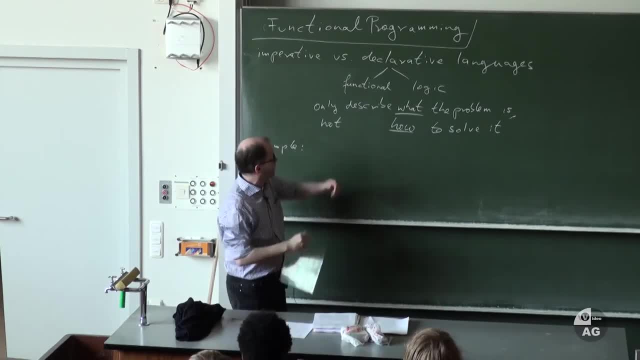 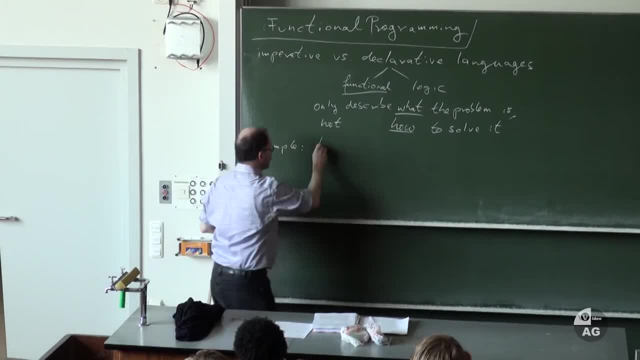 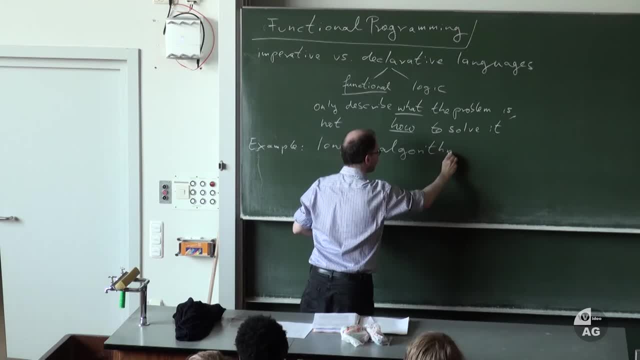 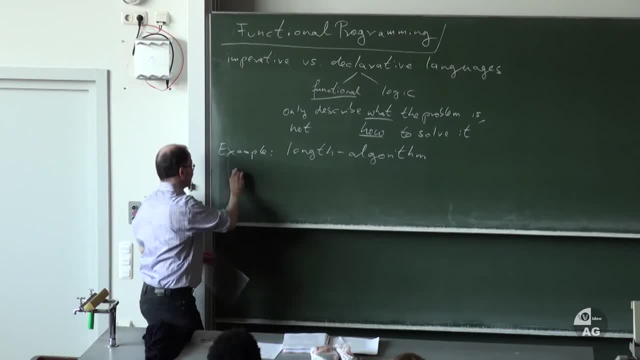 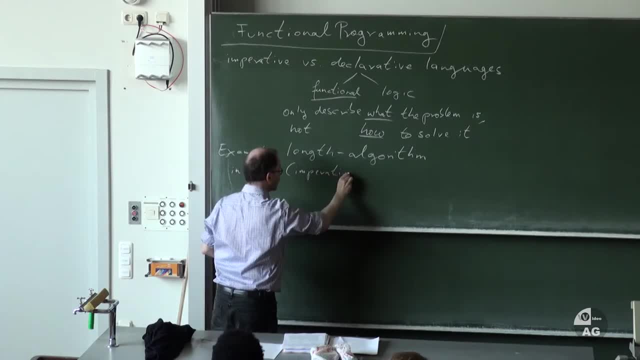 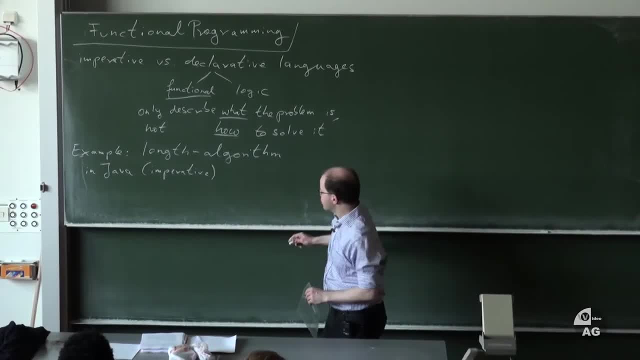 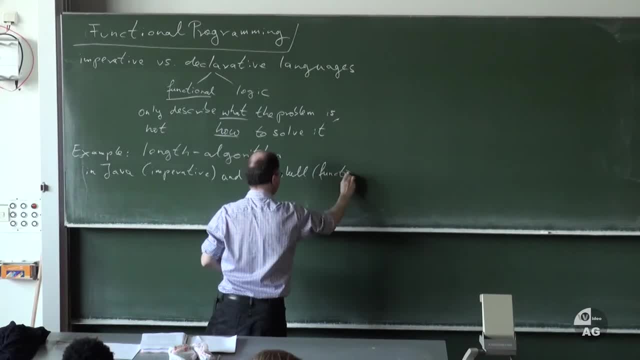 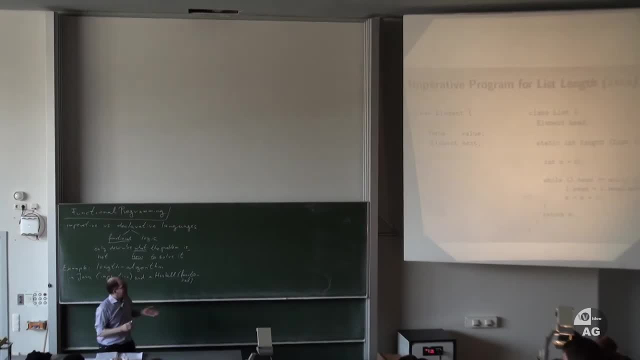 You, just You, just Okay. so to illustrate what function programming is, let's look at the length program in Java and let's look at the length program in Haskell, in a functional language. So how would we solve the problem in Java? 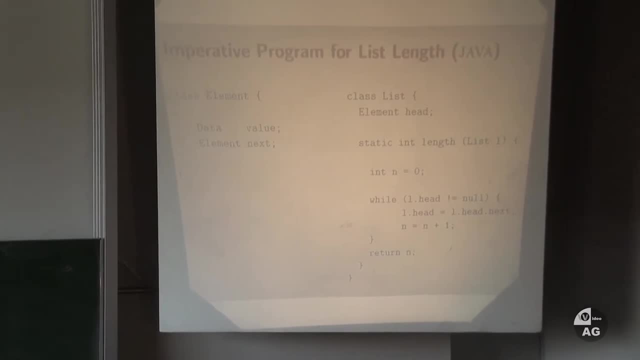 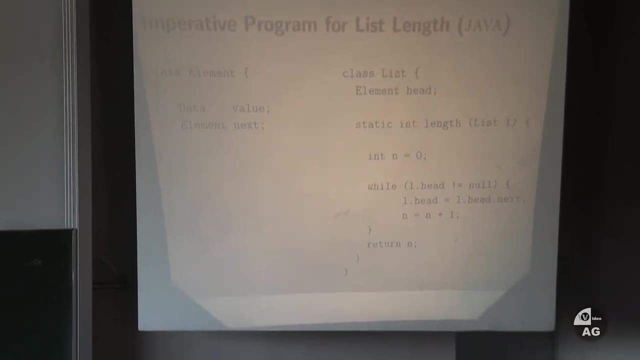 So the idea is we have a list, a linear list, and the goal is to compute its length. And in Java we could do it like this: We could have two classes: a class element and a class list. Now, if you don't know Java, don't worry. 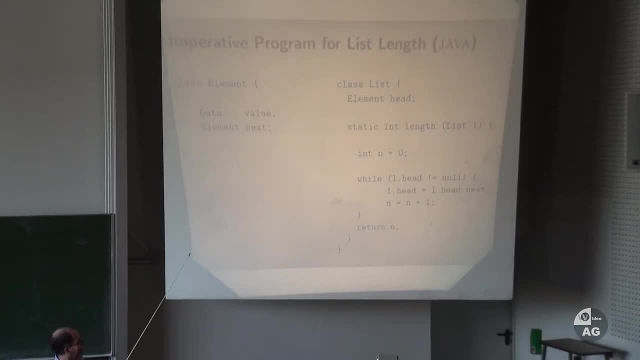 This is the only time that Java occurs in this lecture, so it will not occur again. So if you don't understand this, never mind, But if you understand it it's even better. So we have a class list and list has one field called element. 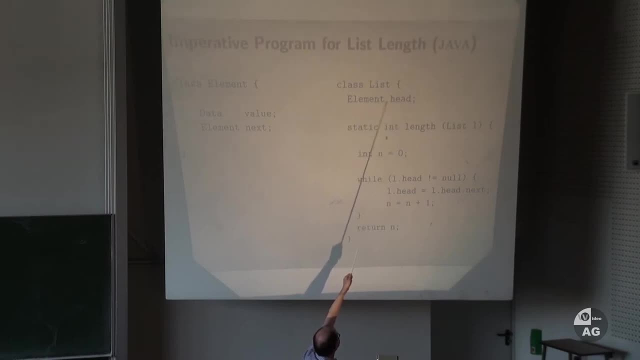 and head is the name. It's one field called head and the type of this field is element And elements. well, elements have a value and a pointer to the next field. So to realize a list, this would look like this: 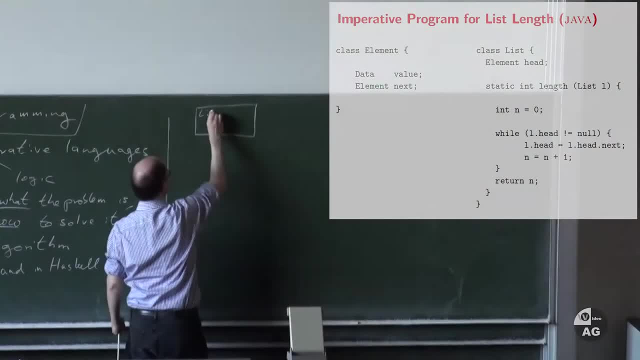 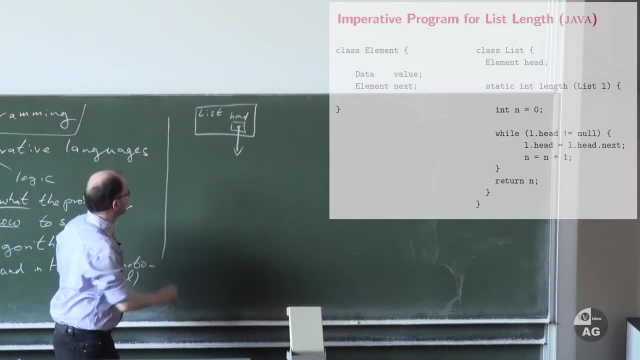 We would have some object of type list and it has a field called head And in this head we have a pointer to the first element of the list. So this would point to an object of type element. And now these elements have two fields: a value field and a next field. 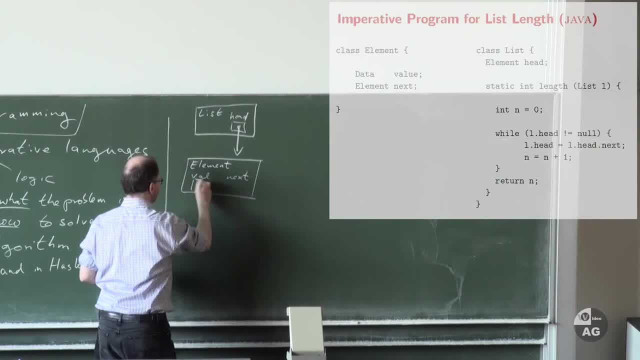 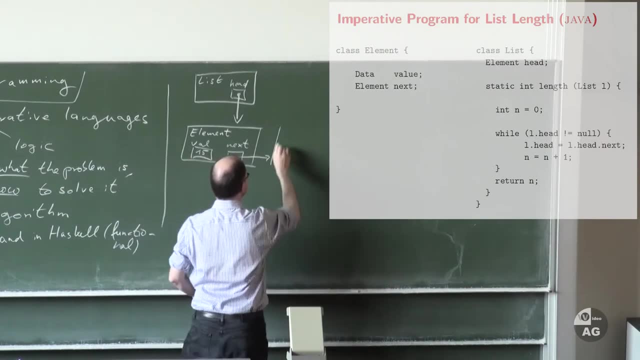 So a value field and a next field, And well, for example, here we could have some number in there: 15.. And next would be a pointer to the next list element. So this would be another list element, And let's say here we have the value 70, and the next pointer. 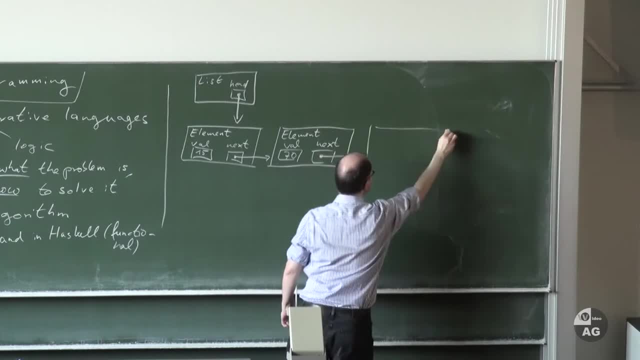 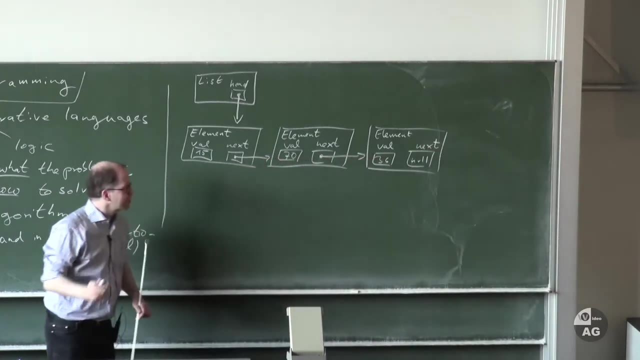 and maybe another last list element, And here the value is whatever 36.. And now it's the end of the list, and so in the next field we have null. So that's the pointer to nothing. So this would be the realization of the list with the numbers 15,. 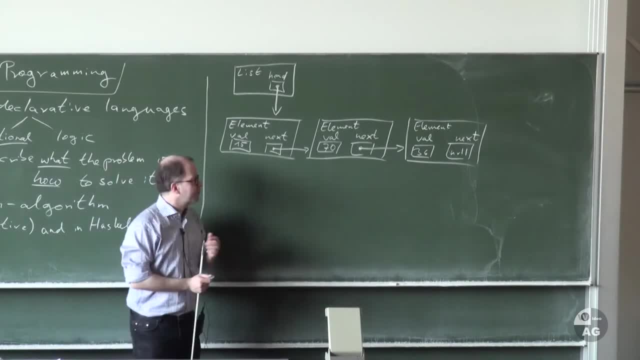 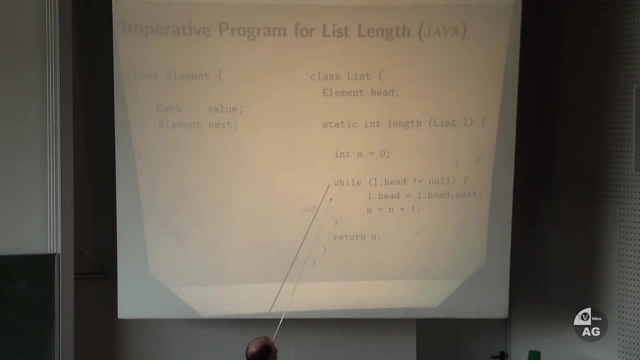 70, and 36.. And now we want to compute the length of this list. And here we have a method length. The method gets the list as input and then it starts iterating. So it initializes a counter, n, and now we have a while loop. 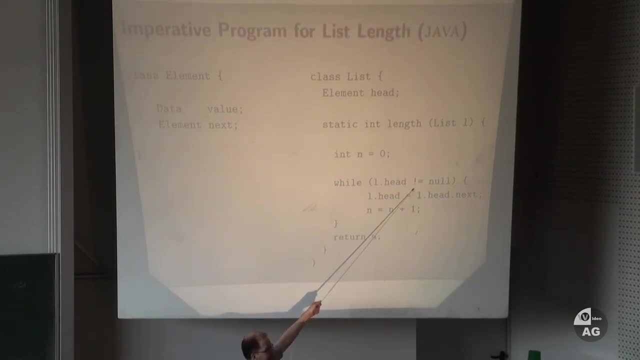 And as long as the head of the list is not null. so as long as we really have a list element, we move lhead to lheadnext, So we move to the next list element And we increase nheadnext, And we do this until we reach the end of the list. 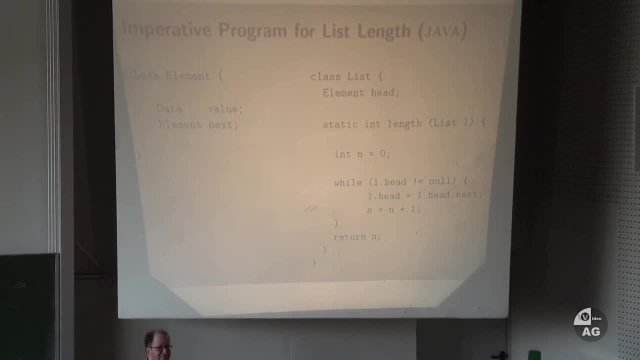 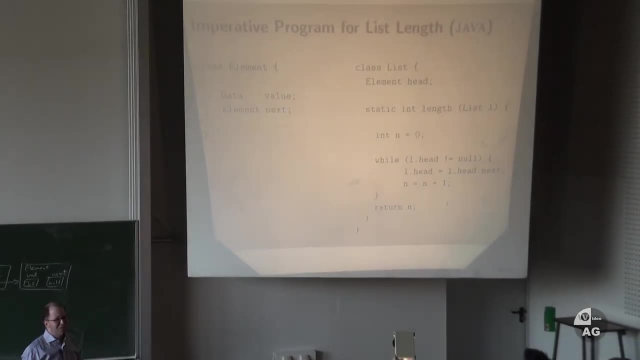 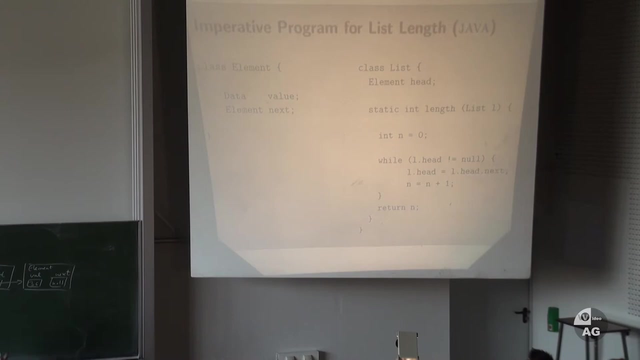 And in the end, we return the value of n. Yes, Yes, on purpose. So, as you notice, this is a bad algorithm and this is meant to illustrate one of the disadvantages of imperative programming. So, of course, you can solve this in a more sophisticated way. 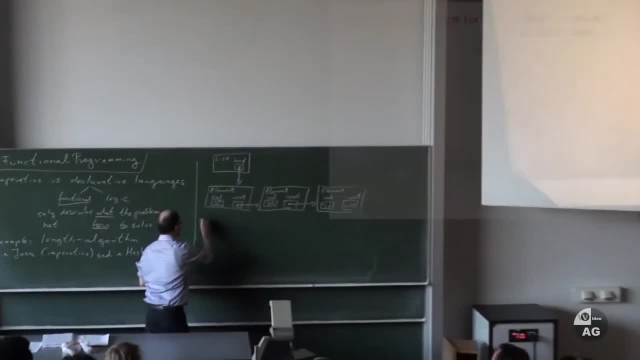 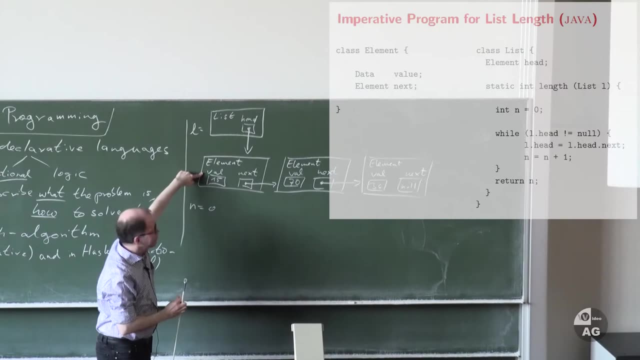 So, yes, this destroys the list, So let's see what happens. So in the beginning, n is 0, l is this, lhead, is this? It's not null. so that's fine. So we run through this while loop. 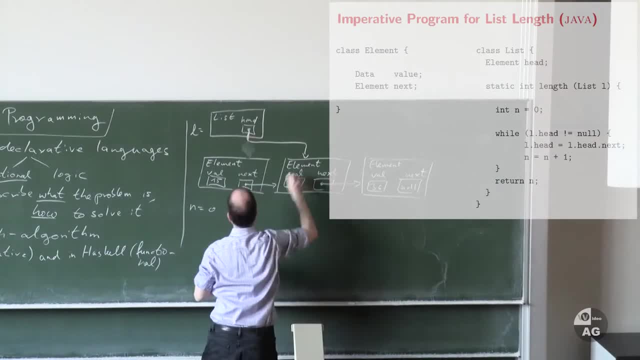 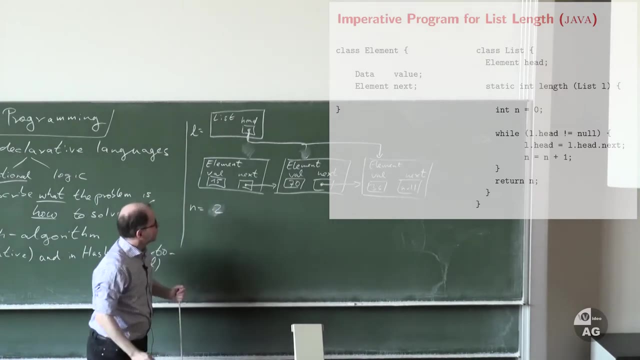 We move the pointer here to there and we increase n by 1.. And now we run again through this. while loop, We see that lhead is still not null, So let's move it here and we increase n by 1.. 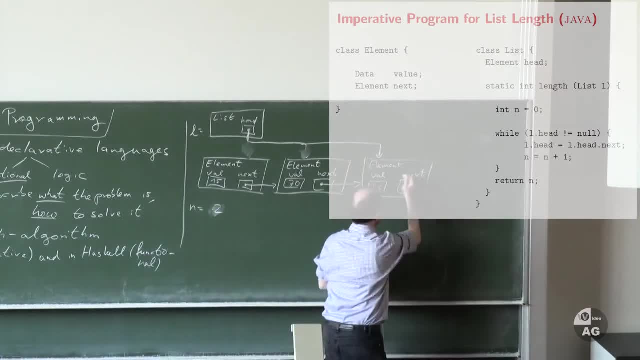 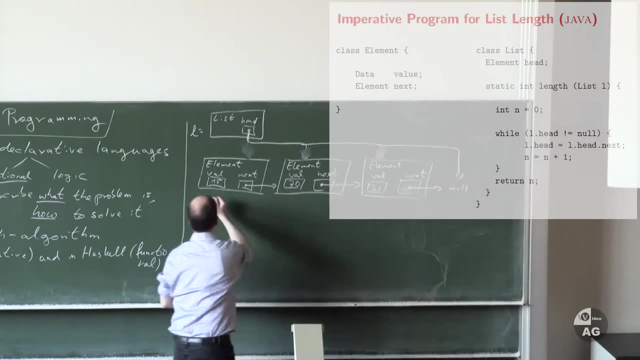 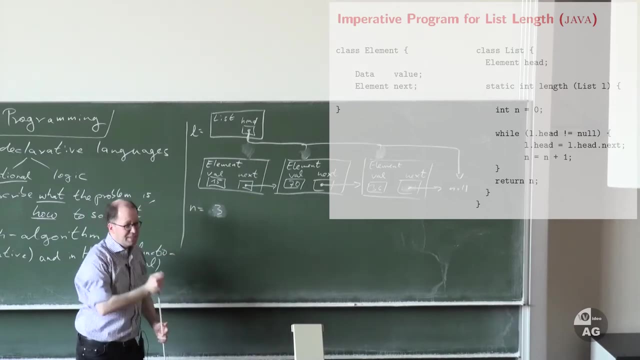 Now lhead is still not null. Maybe we should move. Let's write it like this: So We move the pointer onwards and we increase n by 1. And now lhead is null. so this is the result. Okay, the result is correct. 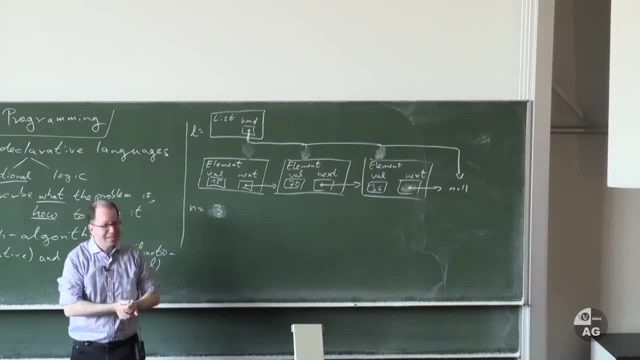 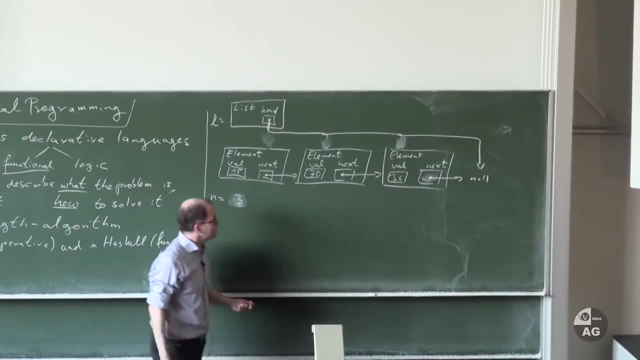 The length of the list was 3.. But, as you pointed out, this has a severe drawback because we computed the length of the list but as a side effect we erased the list, So in the end lhead is null, so the list is lost. 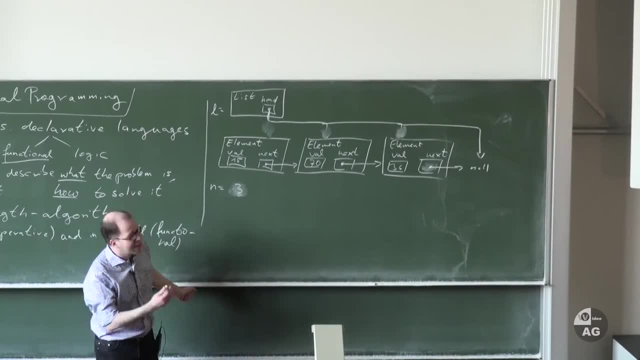 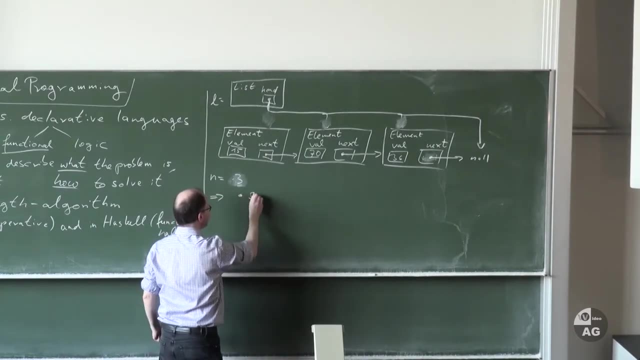 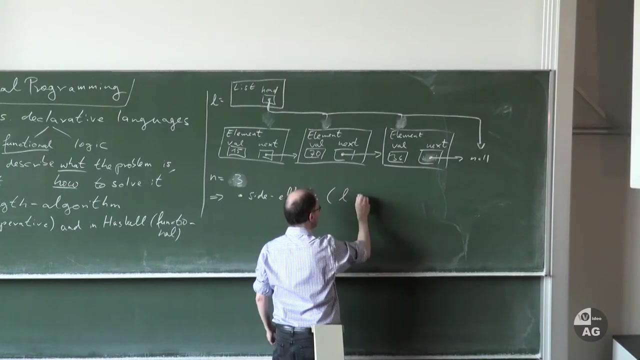 And well, this is most likely a programming bug, So it's it's very unlikely that the programmer intended this. So what we can see is: well, programs can have side effects. So, as a side effect, l is erased. as a side effect. 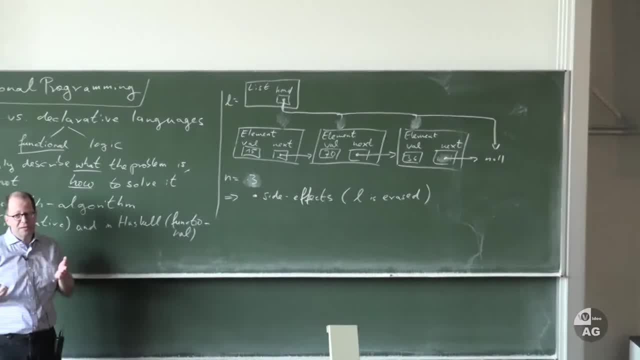 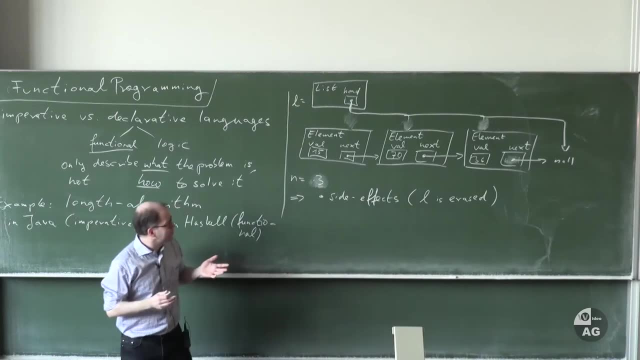 So what? what does this mean? This means that the programmer has to think about what happens in the memory. So the programmer really has to think of something like this. He or she has to think of pointers And what happens in the memory. and do side effects happen? 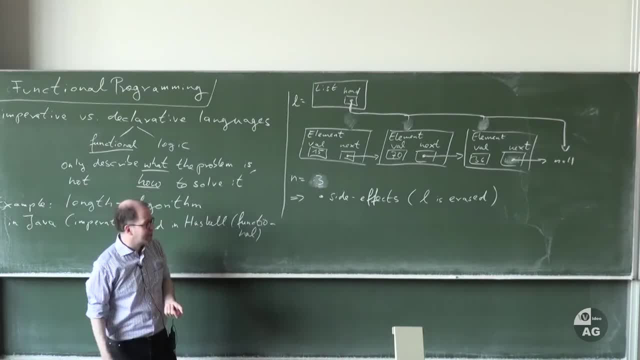 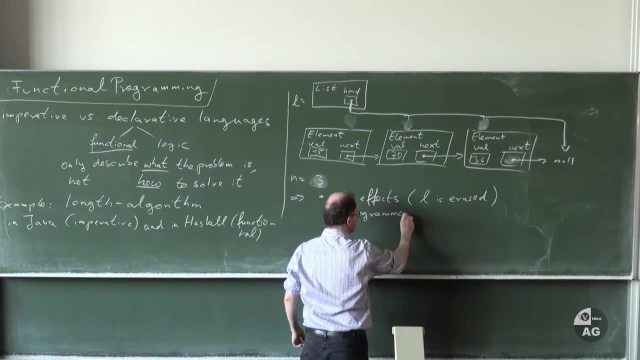 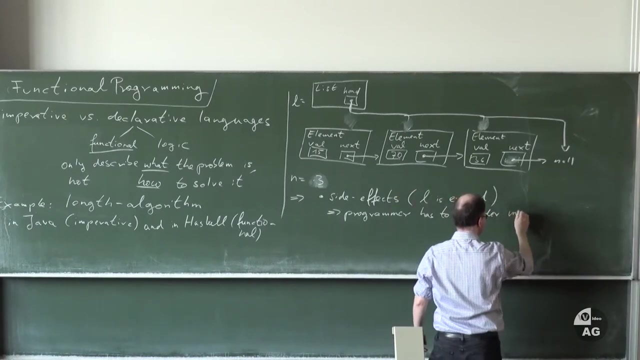 And of course some side effects are desired, some side effects are undesired, So that's something that the programmer has to keep in mind. So the programmer really has to think about the machine, Has to consider what happens In the memory of the of the computer. 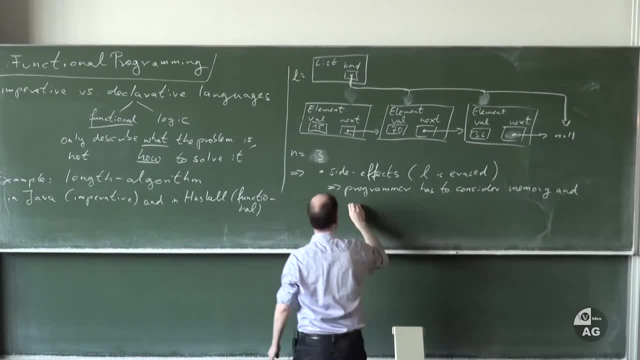 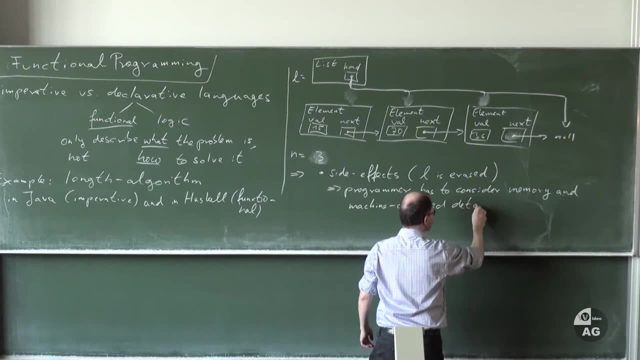 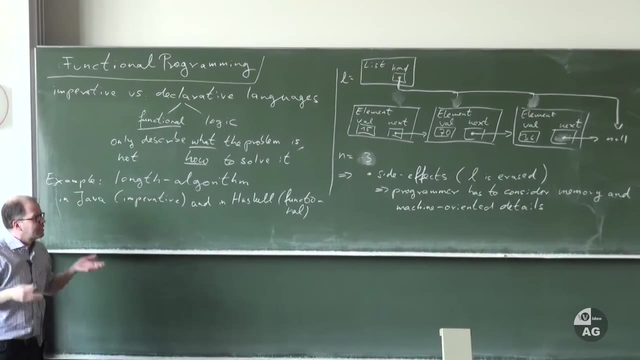 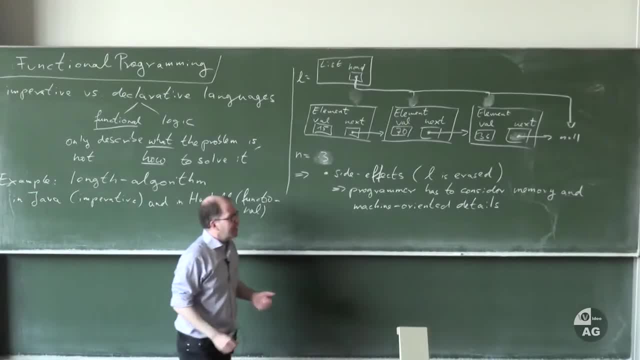 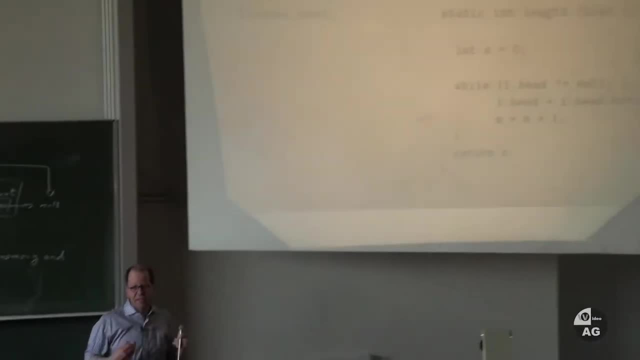 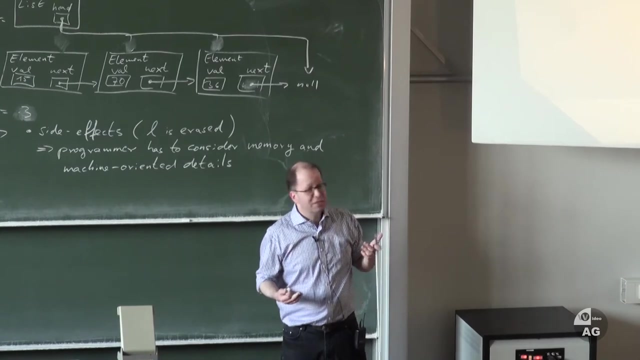 instructions and they are executed from top to bottom. and we have some control structures like this while loop, and there are other control structures like if, then else, and these control structures they can influence the control flow of the program. so they can, they can influence in such a way that execution does not only work from top to bottom, but sometimes statements are. 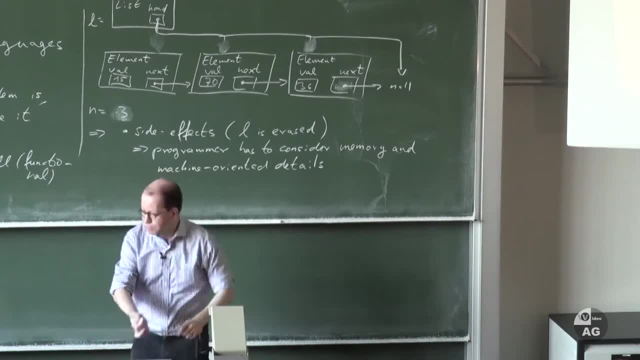 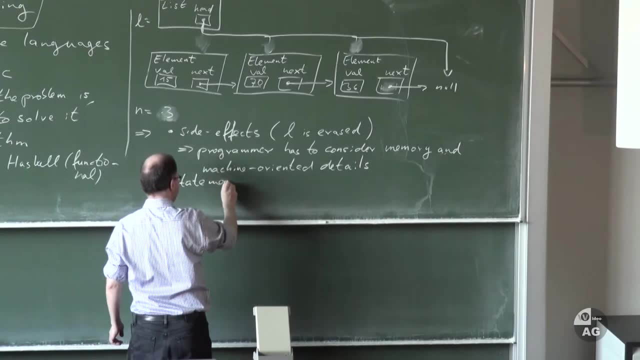 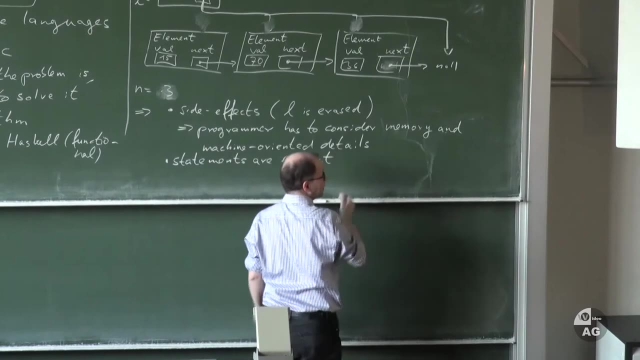 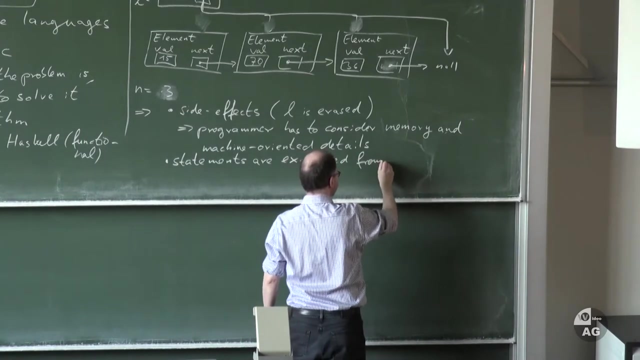 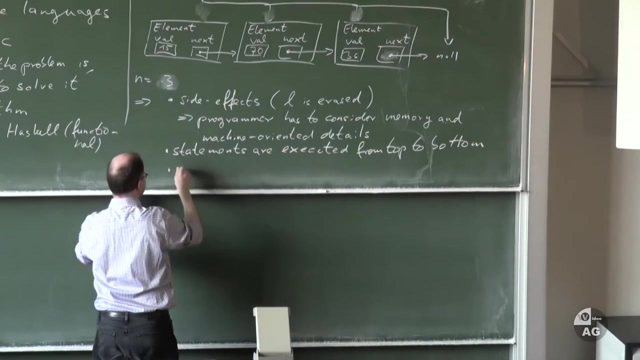 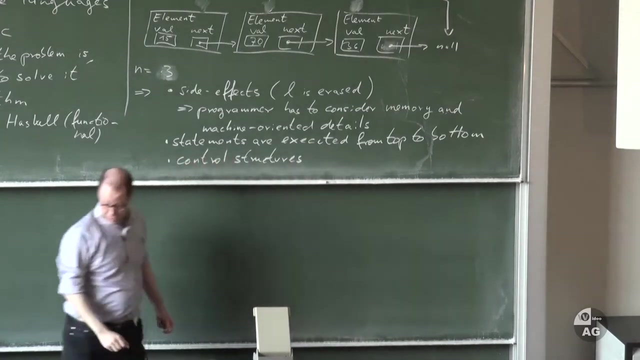 executed repeatedly or you can have branching, so that's typical for imperative programming. so statements are executed from top to bottom and we have certain control structures like while loops and branching operations or go to operations, of which things like this are executed from top to bottom and we have control structures like while loops and so on. okay, so this is probably what we. 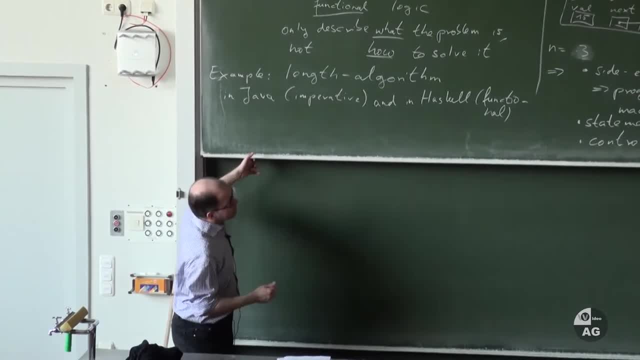 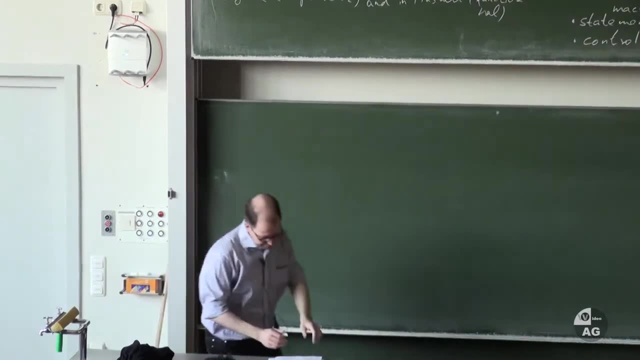 should say about imperative programming. this is a typical imperative program. now let's solve the same problem in a functional way. so let's program this, this algorithm again, but this time we program it in Haskell. and well, as I mentioned, the idea is to do it in a declarative way, so we 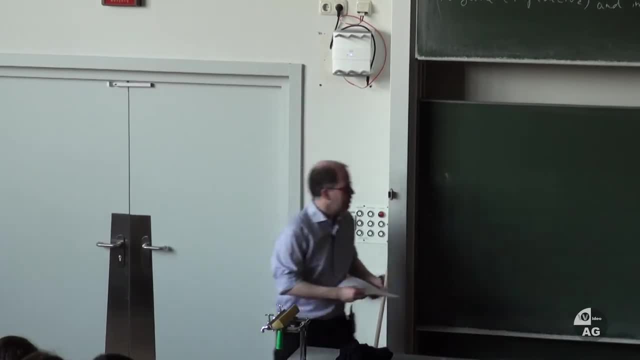 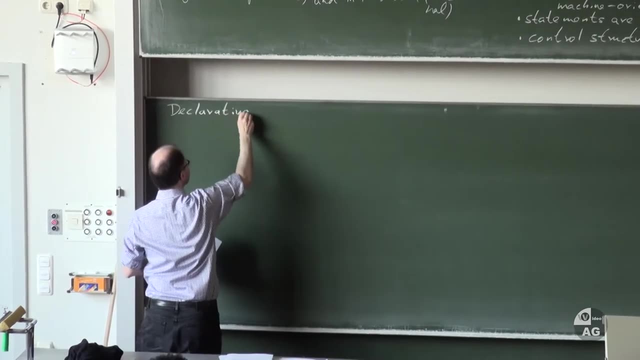 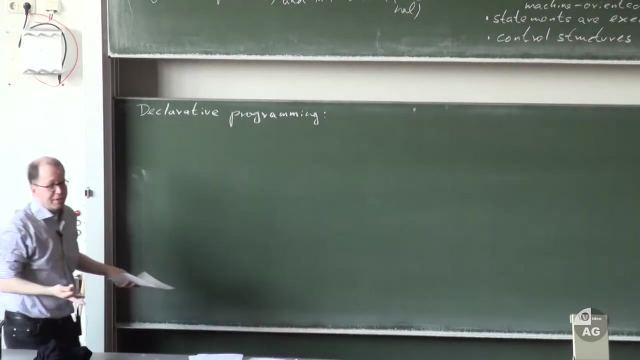 only describe the problem and then the solution has to be found by the computer. so to program this in a declarative way. so this declarative programming. well, the idea is, let's just describe the problem. so what is the problem? the problem is we want to compute list length. so what we have to do is we 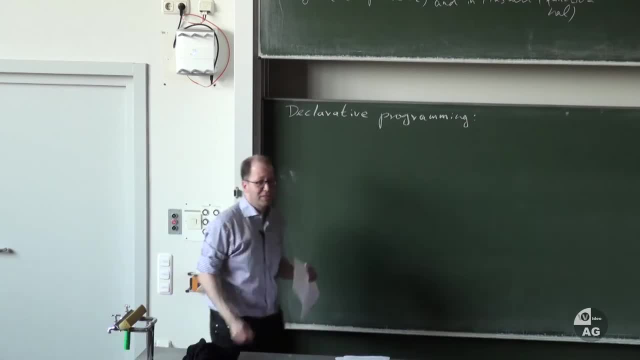 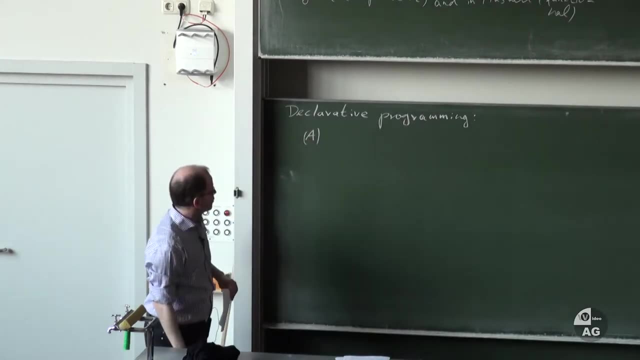 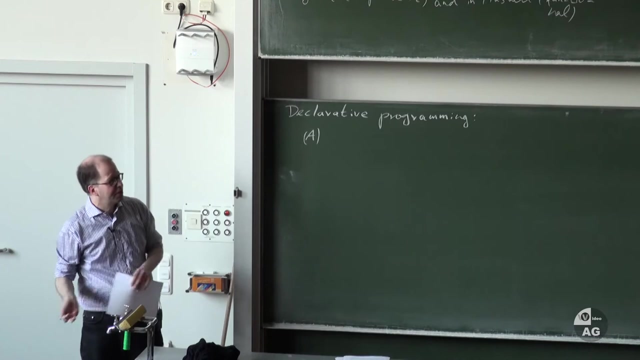 have to define what list length means. so what? what's, what's this concept? what does it mean? list length of a list. well, let's do this in natural language first. so we have to define what list length means. okay, so there are two cases: either the list is empty, or the list is not empty. 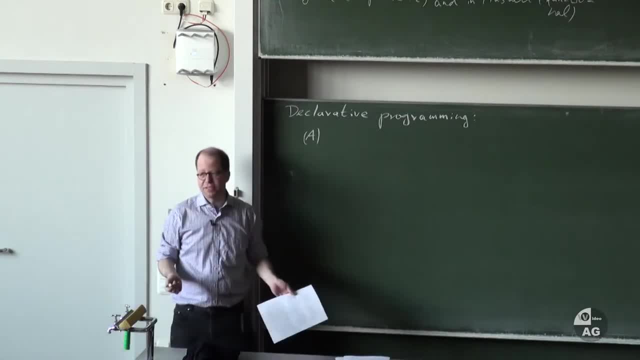 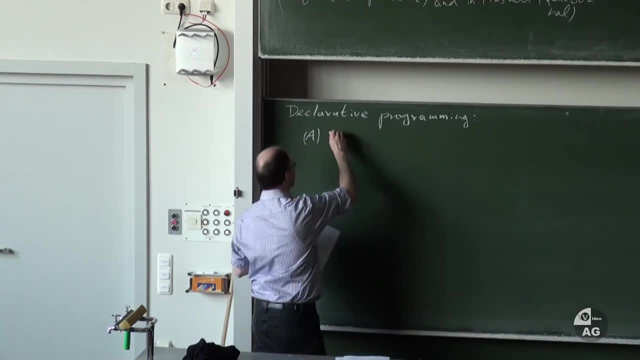 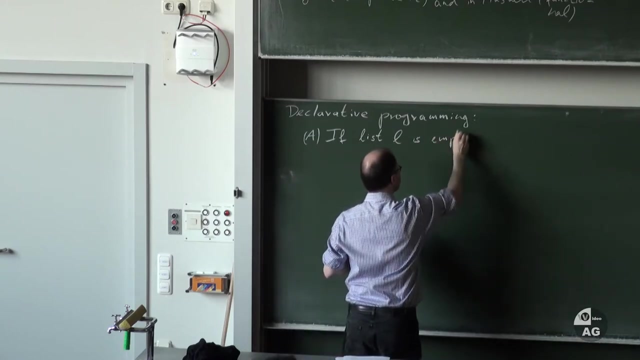 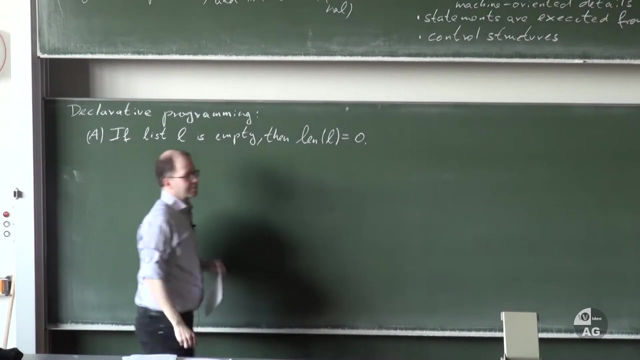 and if the list is empty, then the length is zero. I mean, that's the definition of list length, so that's one of the things that we have to tell to the computer. so let me write this down: if the list l is empty, then the length of the list is zero. so that's one part of the definition of. 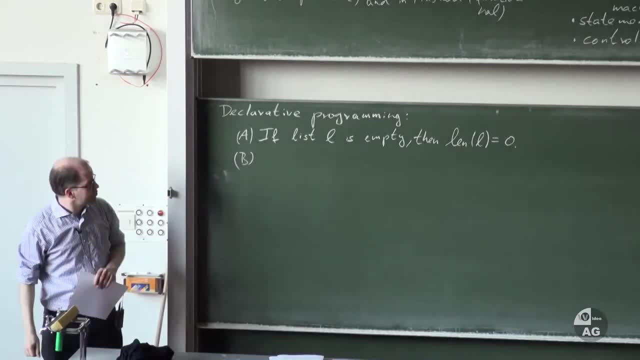 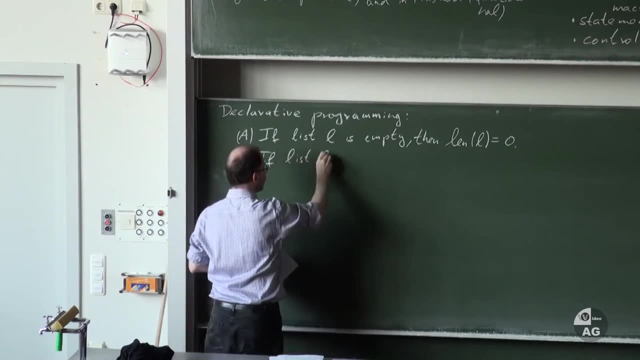 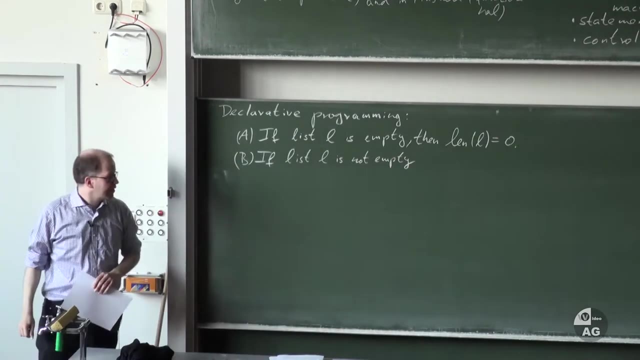 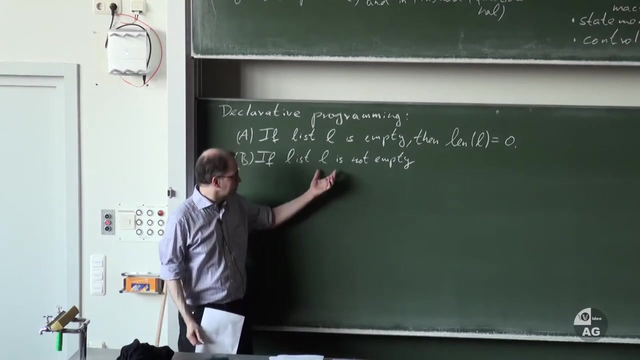 list length. and the second part concerns the case where the list is not empty. so what happens if L is not empty? okay, how could one define list length in this case? well, we could do it in a recursive way. you could say: let's reduce this problem computing the. 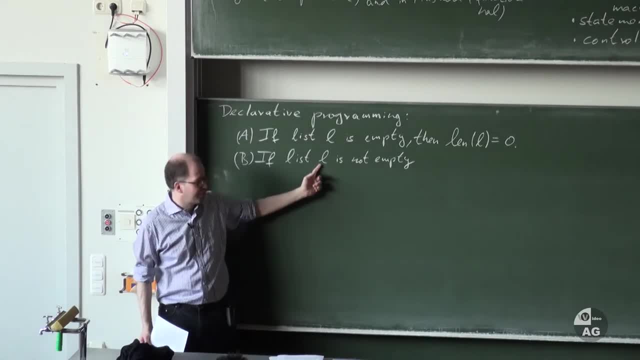 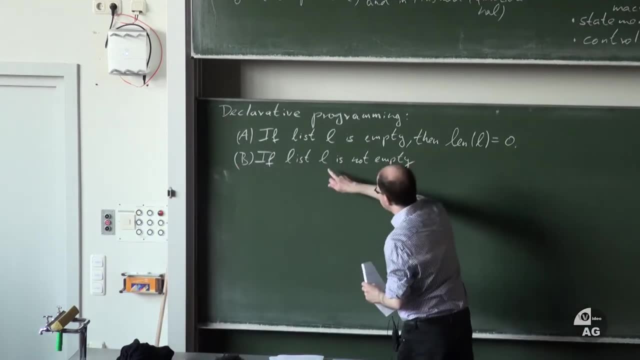 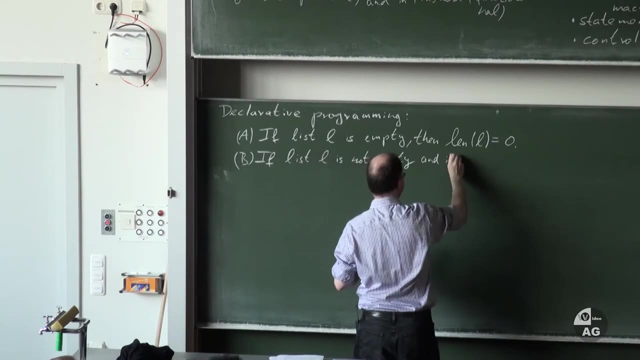 length of L to a simpler problem, namely computing the length of the list that we get by removing the first element. so let's say the, the rest of the list where we remove the first element, let's call this XS. so if L is not empty and if XS, 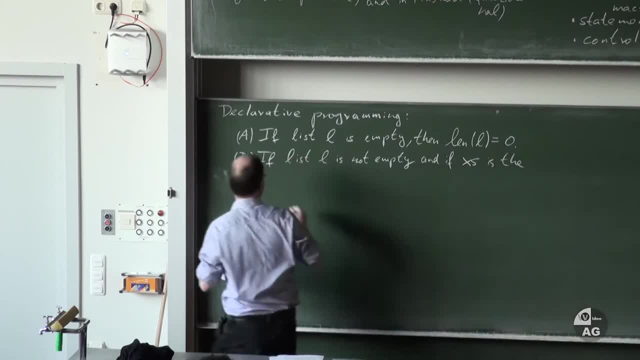 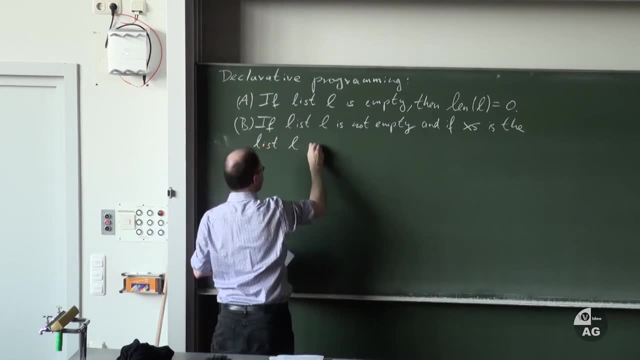 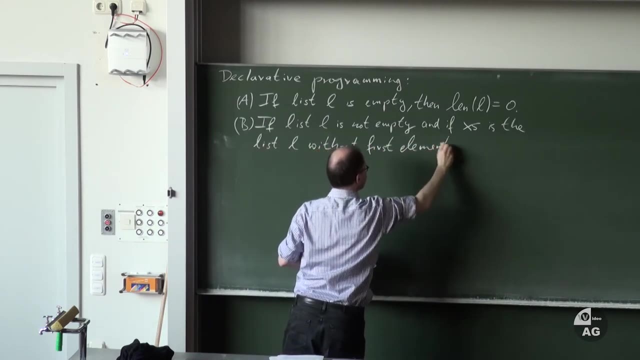 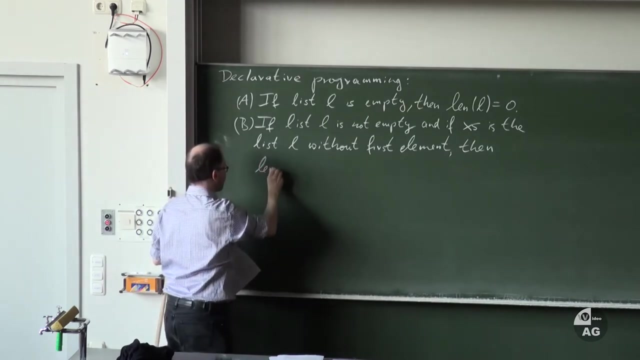 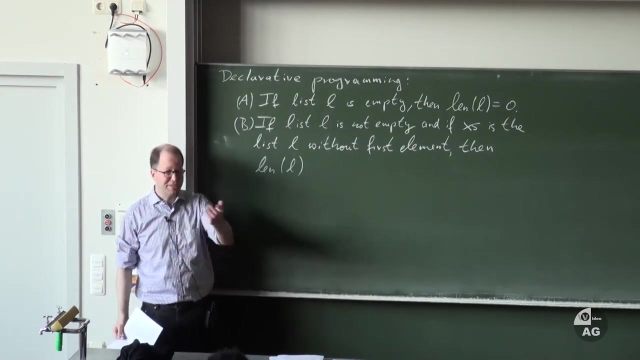 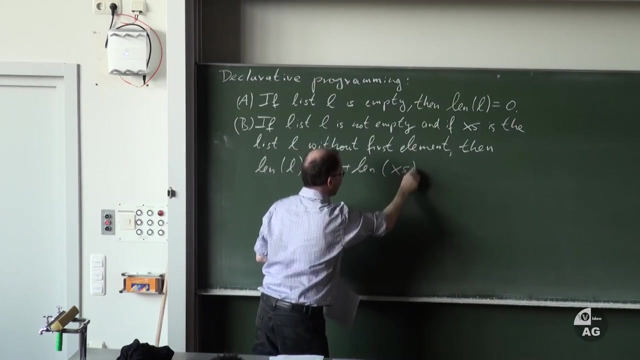 is is the list L without its first element. it's the list L without the first element. then, what is the length of L? well, what's the length of L? how would you do this in a recursive way? yes, right, so it's one plus length of XS. what if we knew already the 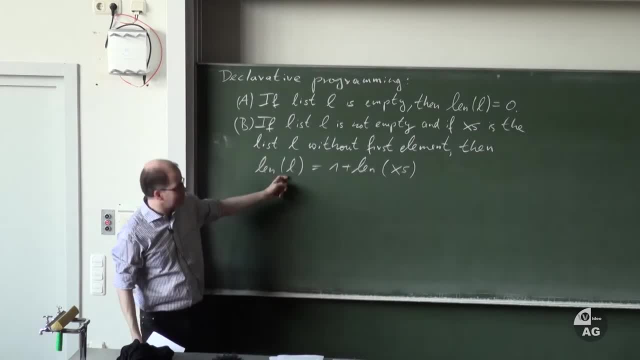 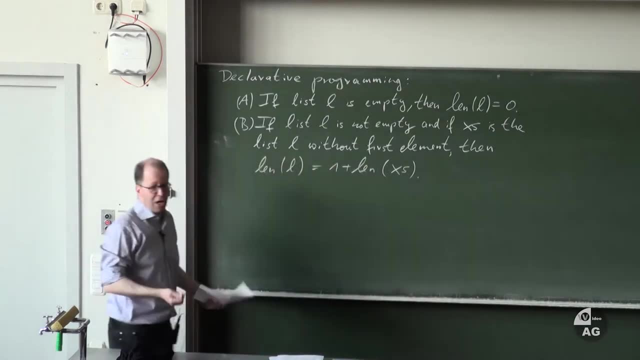 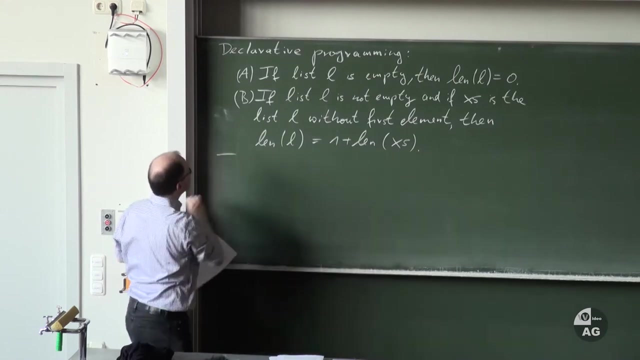 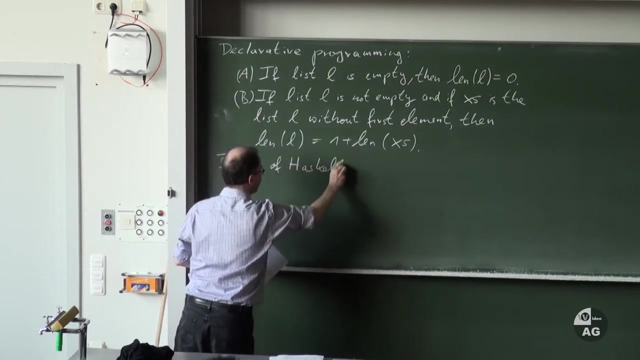 length of this rest list, then we can compute the length of the full list by simply increasing it by one. okay, so that's the definition of list length, and you- yeah, for instance, you can use this, though you can do like a, you know, get it down alive. so now we can translate this natural language. 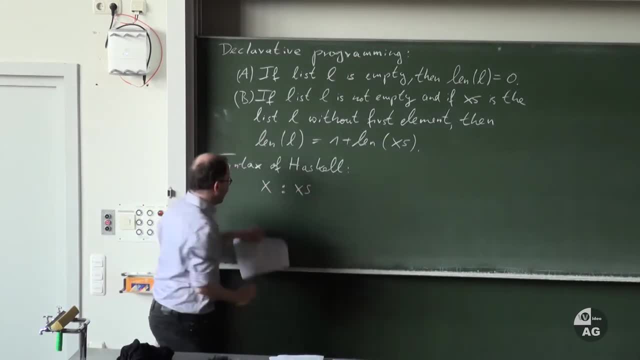 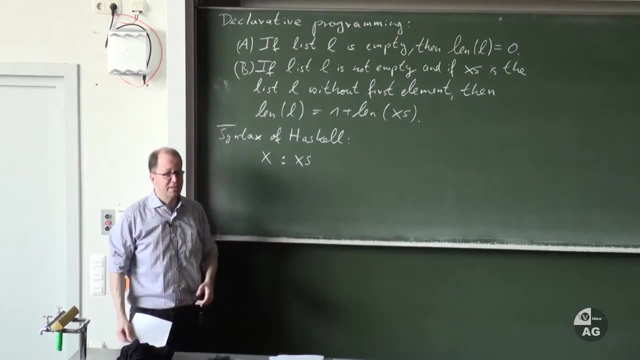 definition into a functional program, and the only thing that you have to know is a little bit about the syntax of the functional programming language, and of course, the syntax is different in every language. so what do we have to know For the list that starts with this element x and where x is the remainder of the list? 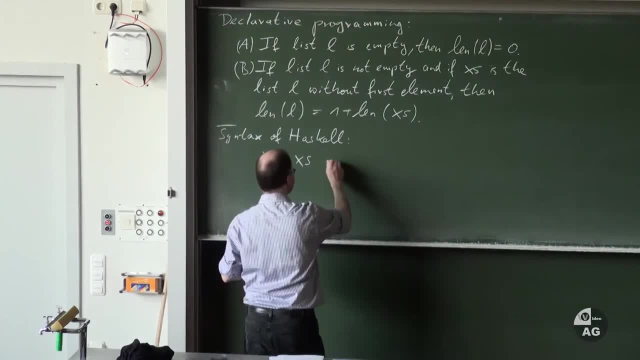 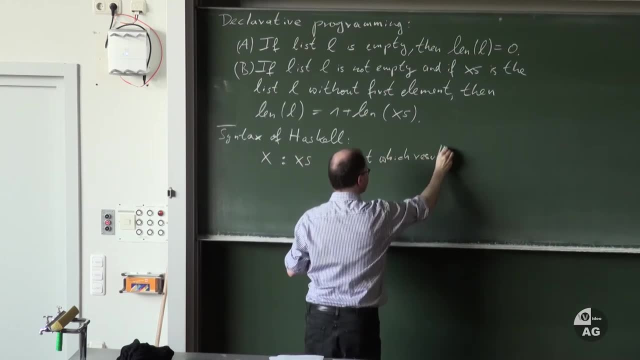 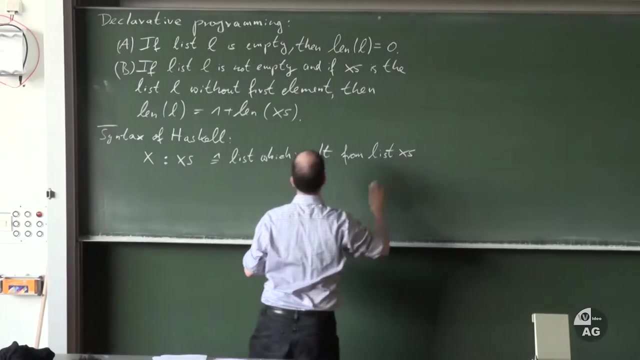 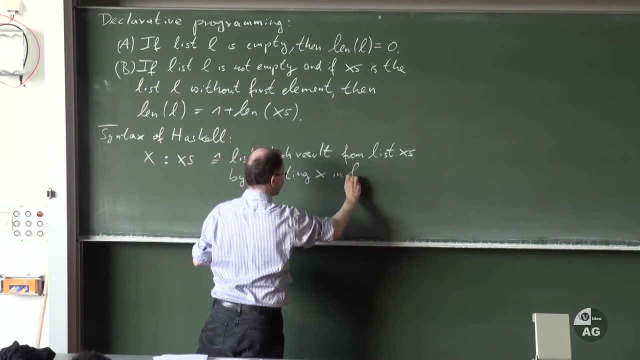 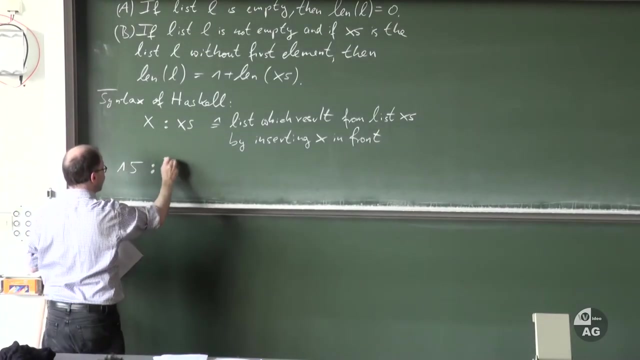 So it's the rest of the list without its first element. So this means the list which results from the list x's by inserting x in front, From the list x's by inserting x in front. So for example, we can write down this list 15, colon 70, 36.. 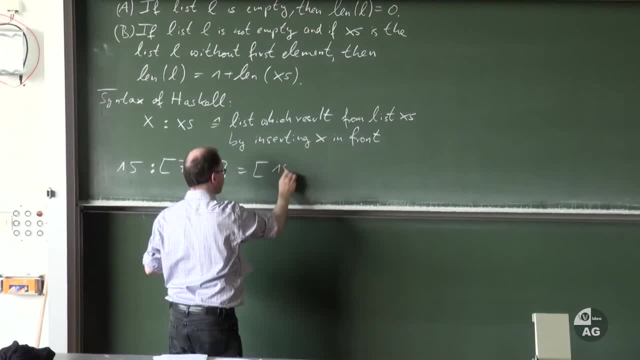 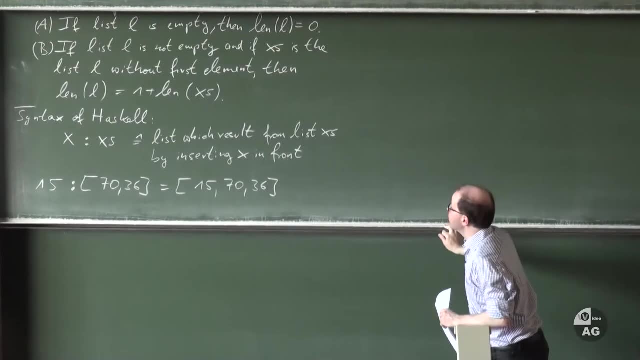 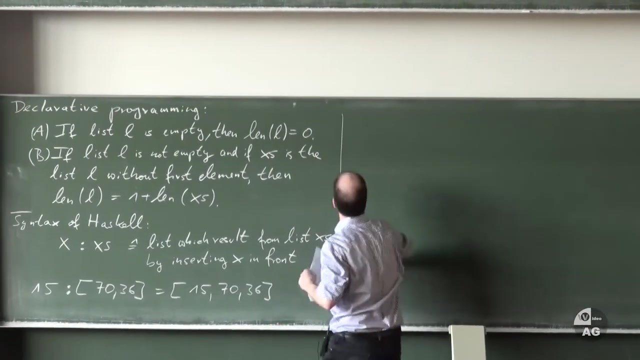 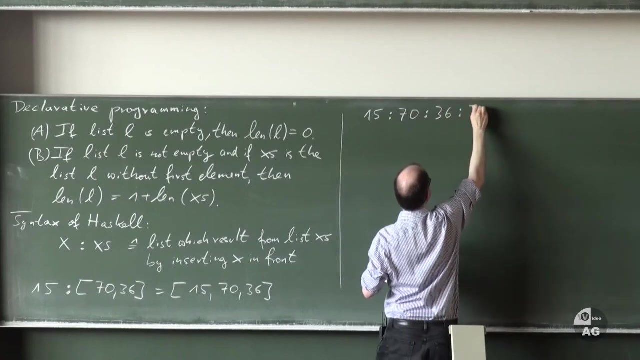 And this is the same as the list with the three elements 15,, 70 and 36.. So colon means list insertion and list insertion in front, And you can also write down things like this: So you can write 15 colon, 70 colon, 36 colon, empty list. 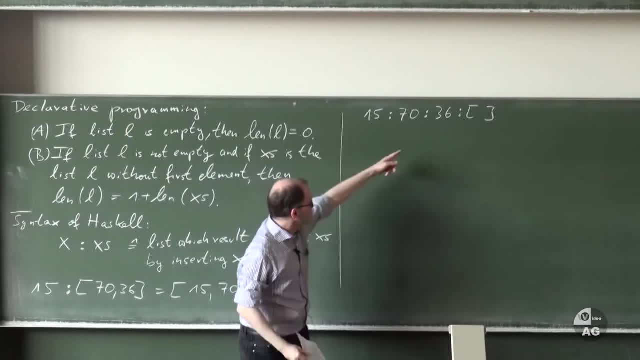 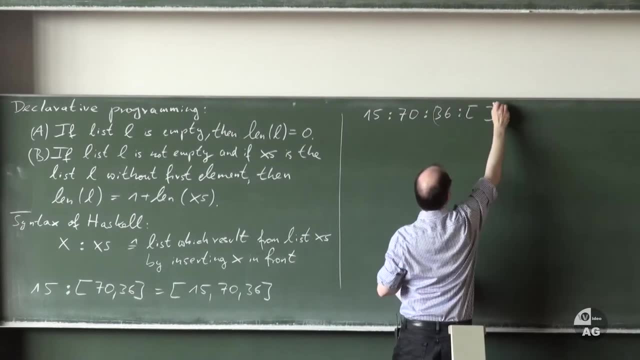 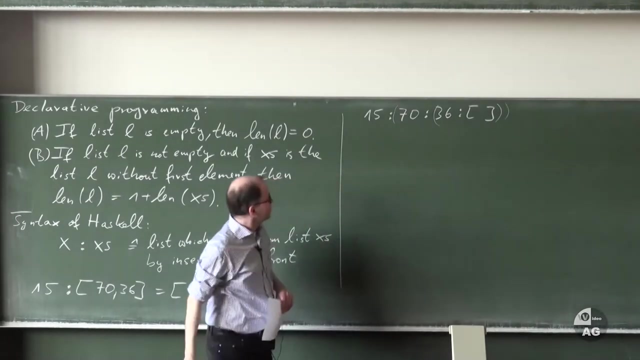 So this means the empty list And these colons are operated, are executed from right to left. So this stands for the expression where you first insert 36 into the empty list, Then you insert 70 into this list And in the end you insert 15.. 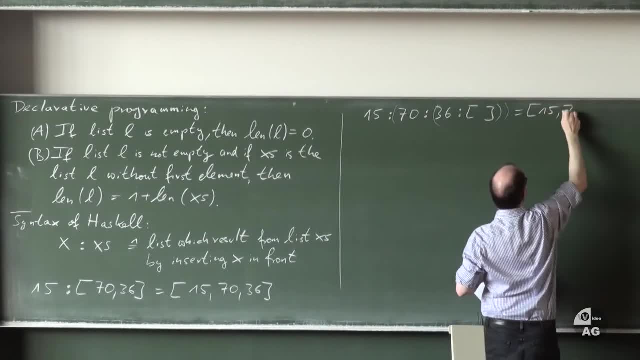 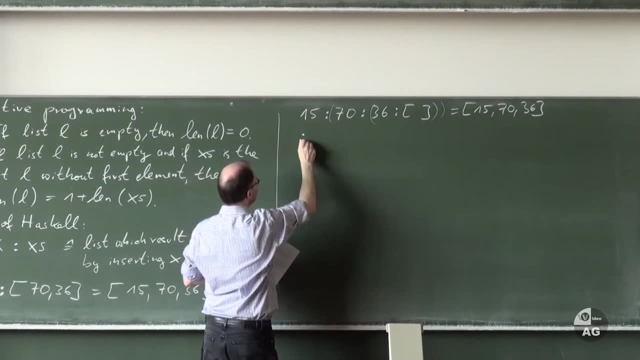 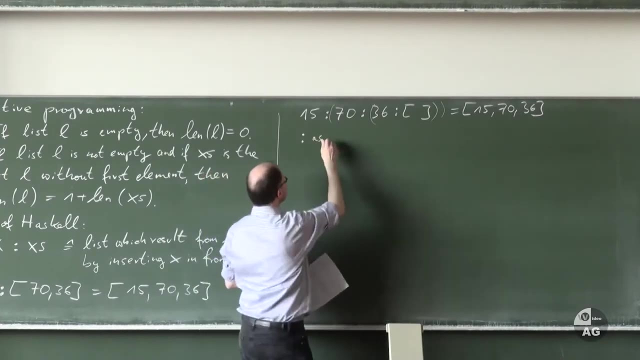 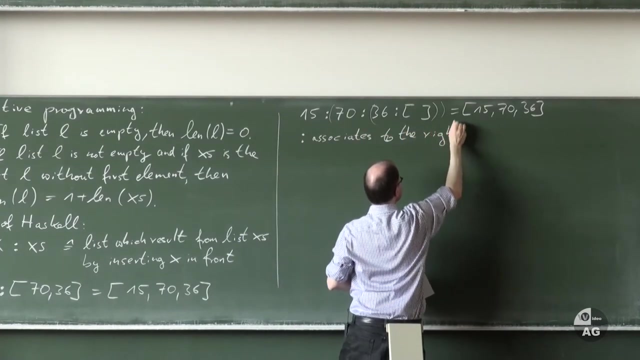 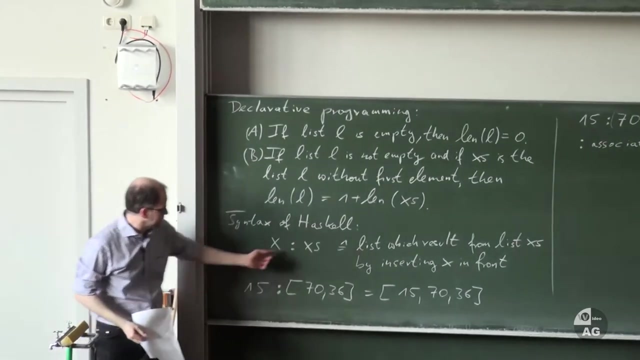 So this is the same as the list 15,, 70, 36.. So colon associates to the right. So if you omit these brackets, then Haskell inserts these brackets automatically. So this associates to the right. Okay, so this means that every non-empty list can be written in this form. 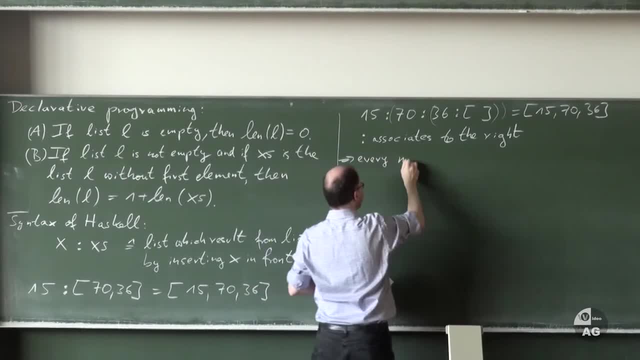 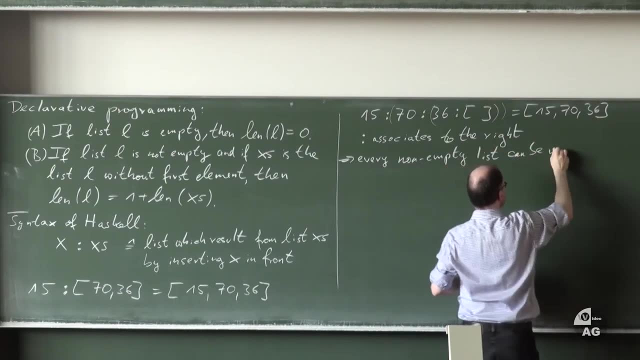 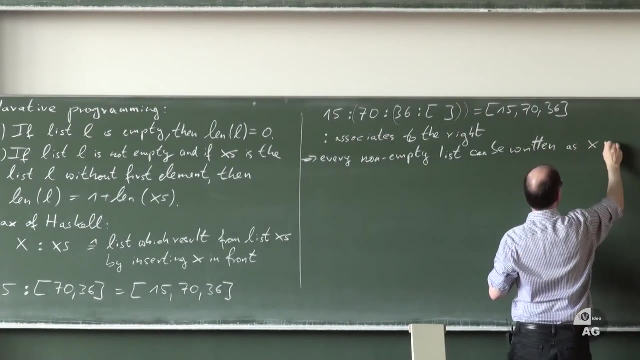 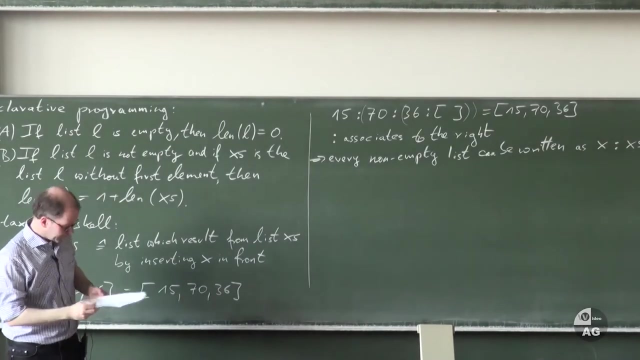 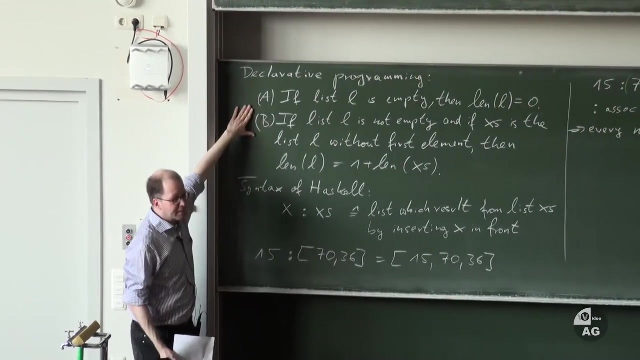 So every non-empty list in Haskell can be written in the form as: x, colon x's, Where x means the first element And x's means the rest of these elements. Okay, and now we can translate these two sentences here, These two sentences in natural language: 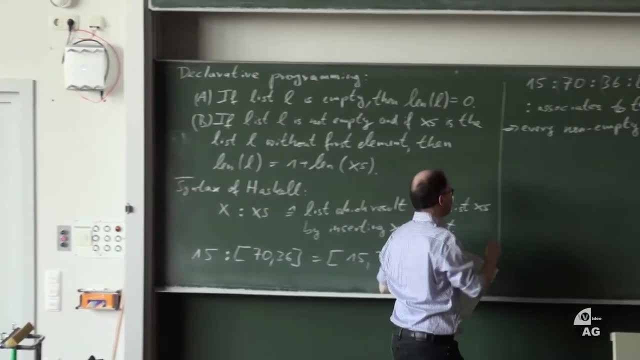 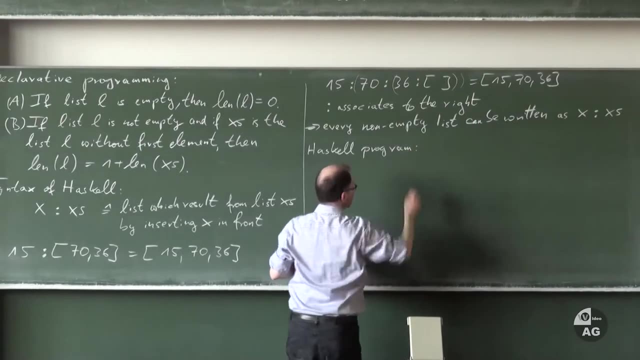 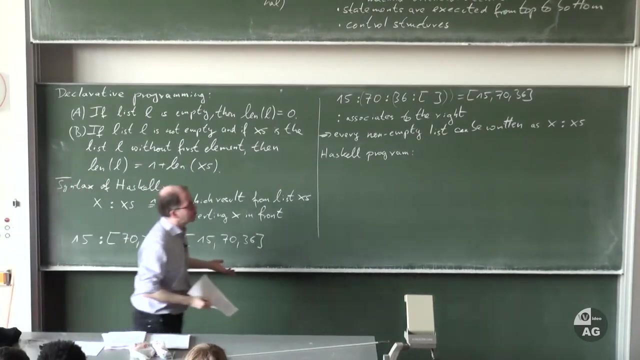 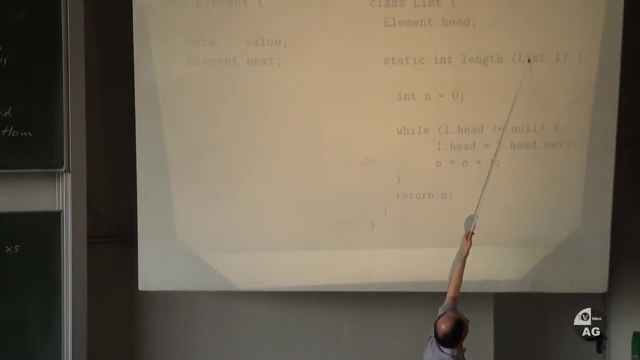 We can translate them to Haskell. So how would the Haskell program look like? So in the Haskell program we would also write a function length or len, And Like in Java, this is a function that maps lists, So that maps an element l of type list to an integer. 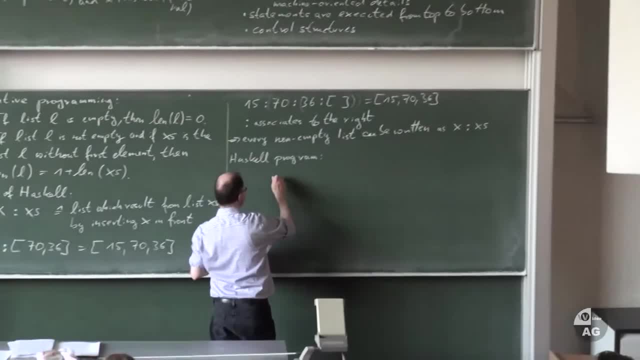 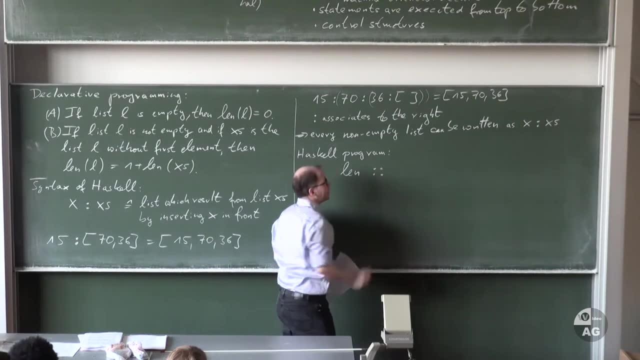 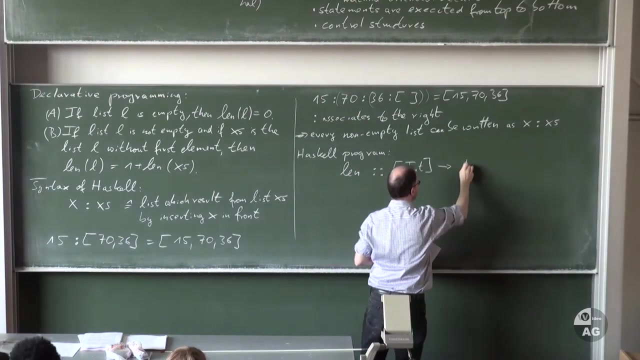 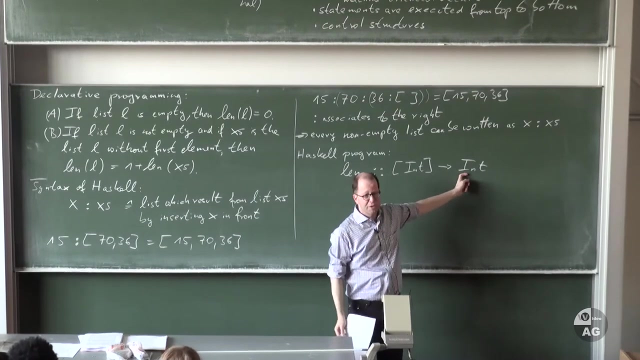 So this is the same in Haskell. So len is a function And the syntax is as follows. We say: well, the type of len is a function And this function maps lists. So, for example, lists of integers to integers. So Well, for integers. the only difference is that in Haskell, int is written with a capital: i. 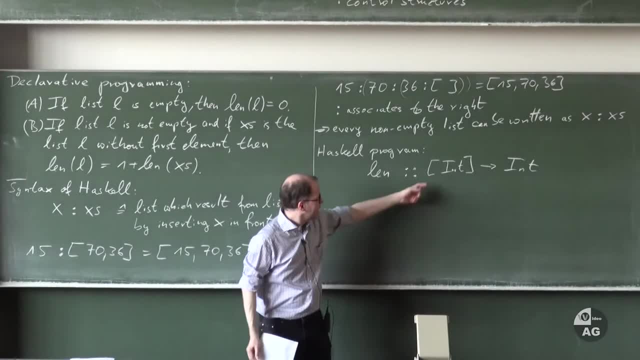 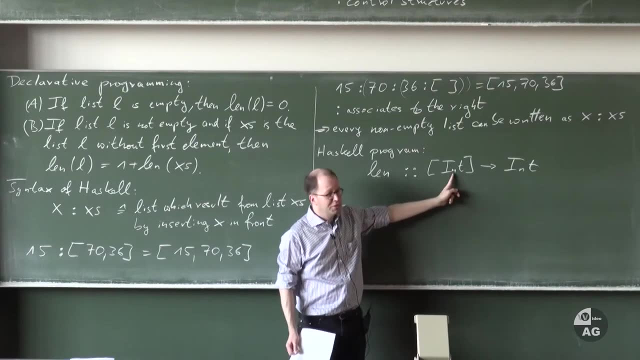 And in Java it's written with a small i, But apart from that it's the same And this is the data type for lists of integers. So typically you write it like this: You write square brackets, And between these square brackets we write the type of the elements. 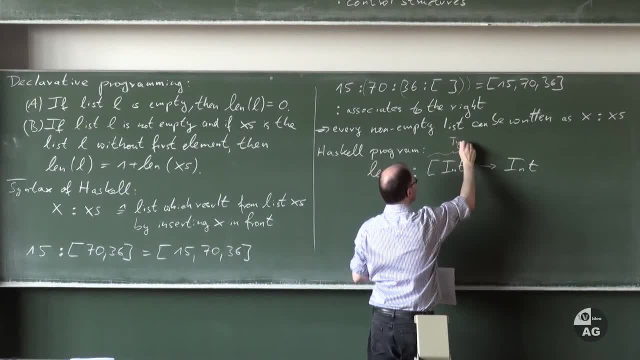 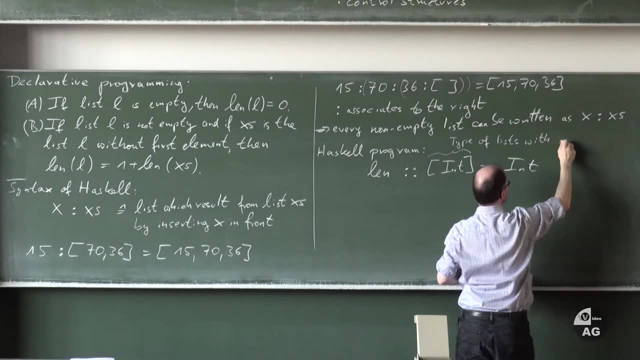 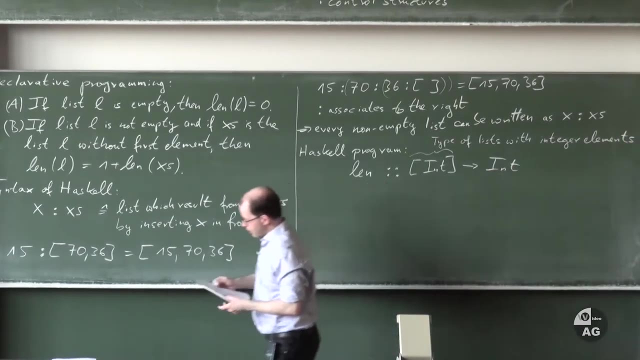 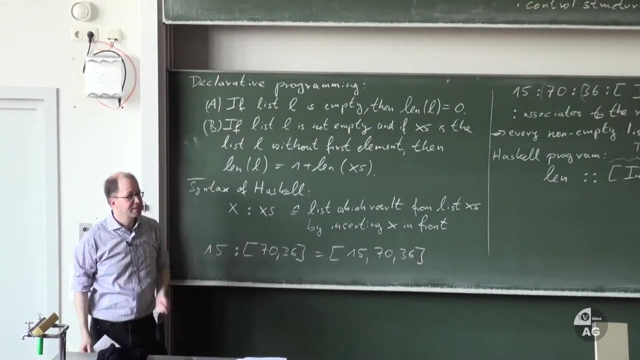 So this is the type of lists with integer elements. So this is the type of the function len. And now, how does len work? Well, let's simply translate these two parts of the definition. Yes, Because I want to start with the simple case. 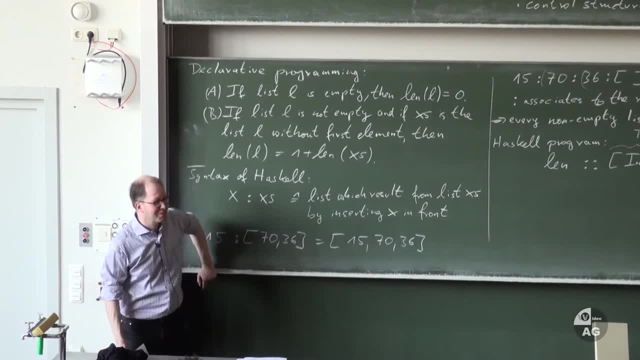 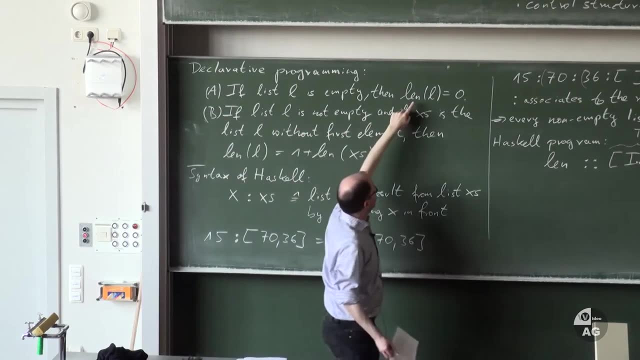 And I will replace this by a type variable in a minute. Okay, I will do this in a minute. Okay, Here we have the following statement: The length of the empty list Is zero. So in Haskell this would read like this: 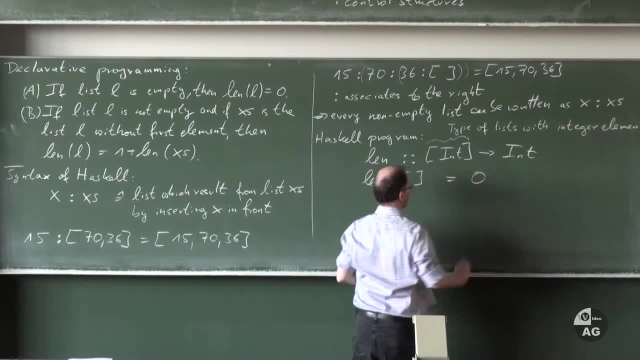 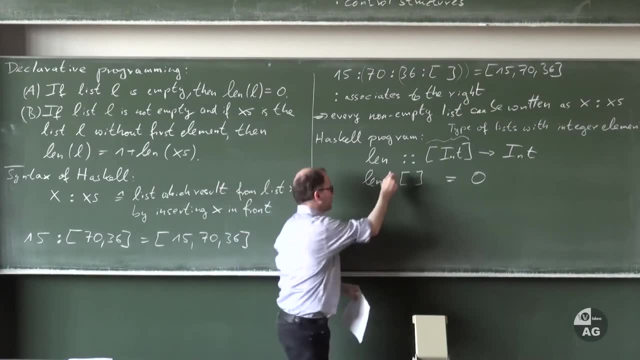 The length of the empty list is zero, So this looks just like in mathematics. The only difference is that I didn't write round brackets around the argument, So I didn't write this. But in Haskell you can write this. But well, Haskell programmers are lazy. 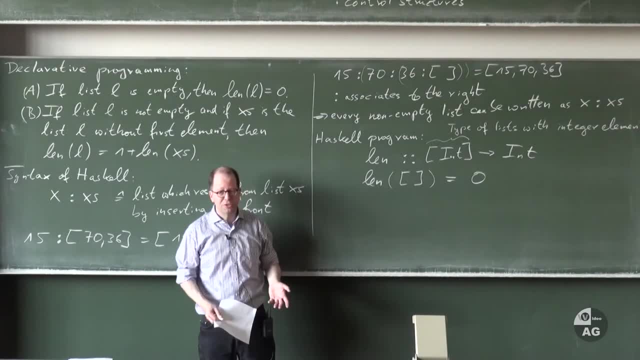 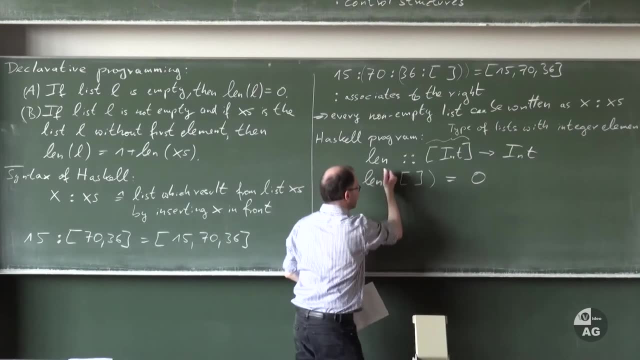 They want to write as little as possible, And so whenever it's possible to omit brackets, we omit brackets, And there's no need to write brackets around the argument. So the normal Haskell programmer would write this, But if this confuses you, you can also write brackets. 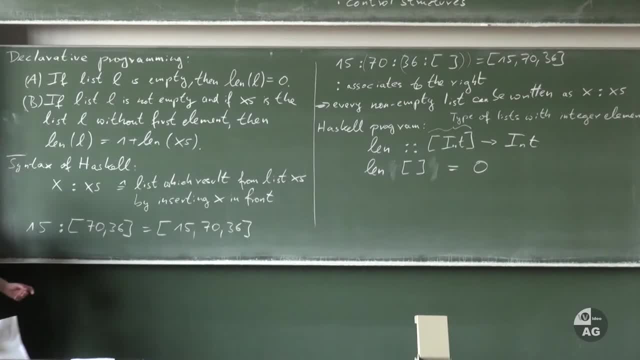 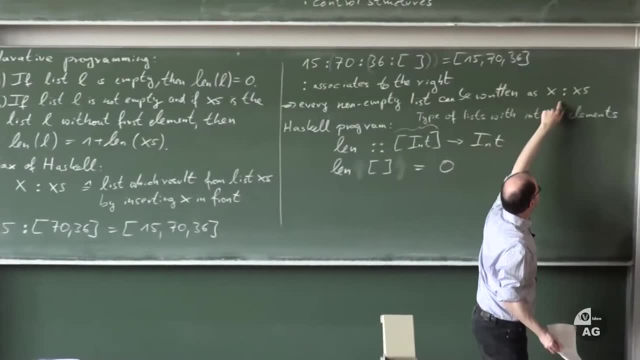 So the length of the empty list is zero. And what happens if the list is not empty? Well, if L is a list that is not empty, then we can write it in the form x, colon x's. So what's the length of a list of this form? x, colon x's. 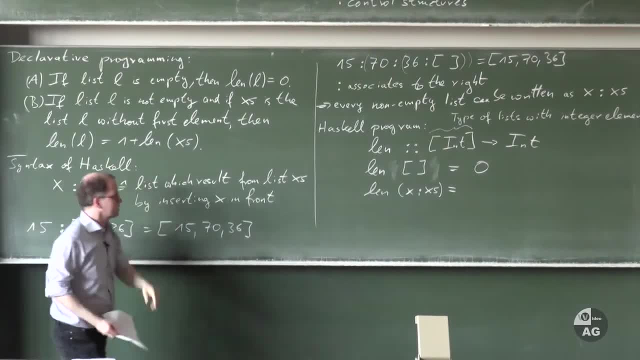 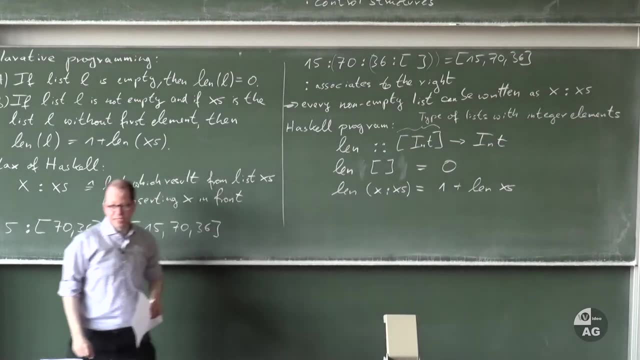 Well, here we have it. It's one plus length of x, So it's one plus length of x's, And that's it. That's the Haskell program. So the step from this natural language definition to the Haskell program is rather straightforward. 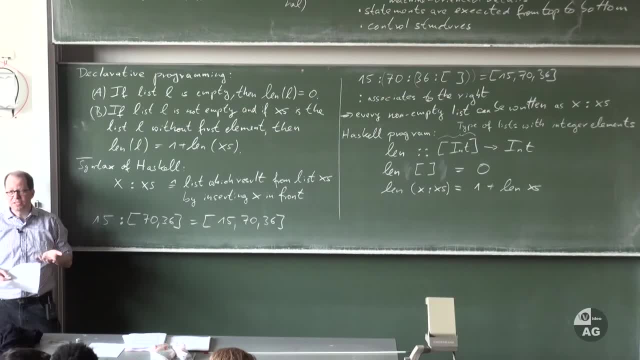 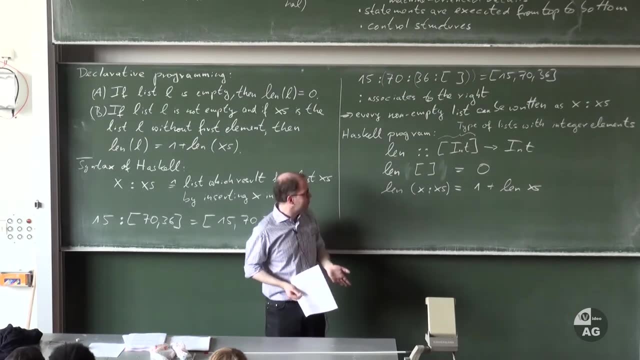 And well, this is what I meant by declarative programming. So this is very near to the declaration of the function or to the natural language description, And therefore this is rather easy to read and rather easy to understand, And you don't have to think about what happens. 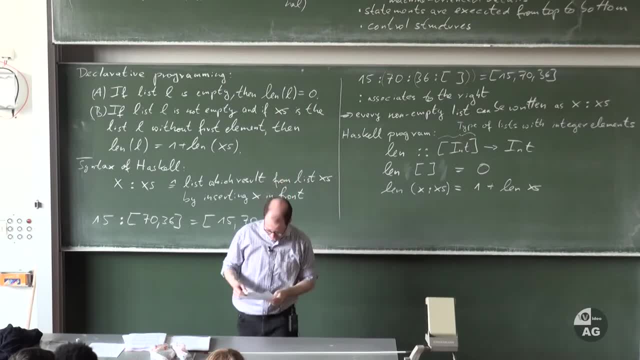 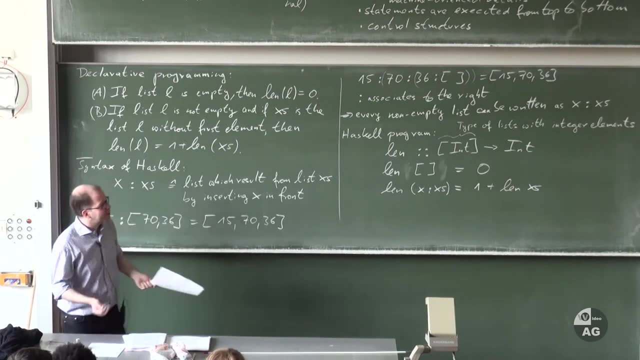 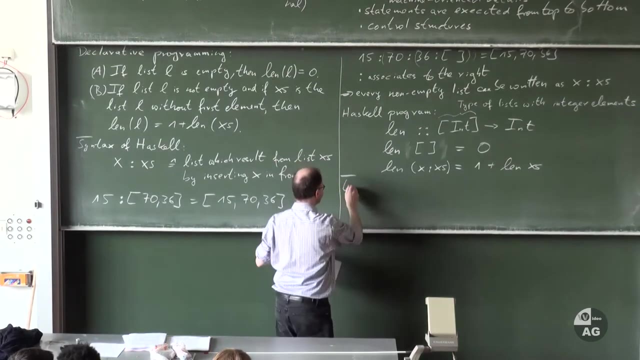 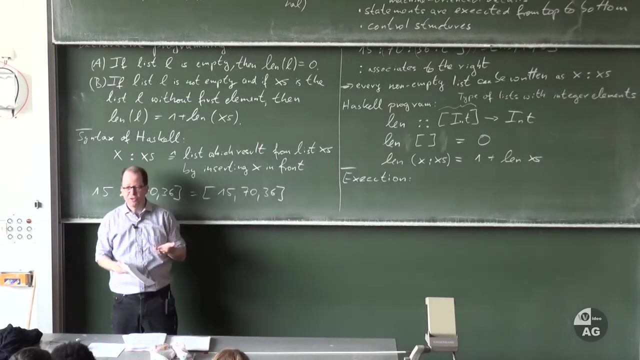 This is just the definition of the length function, and that's it. So how do you now execute such a program? I mean in Java, you compile the stuff and then you call the main function. And how does this work in Haskell? Well, in Haskell it's like in a pocket calculator. 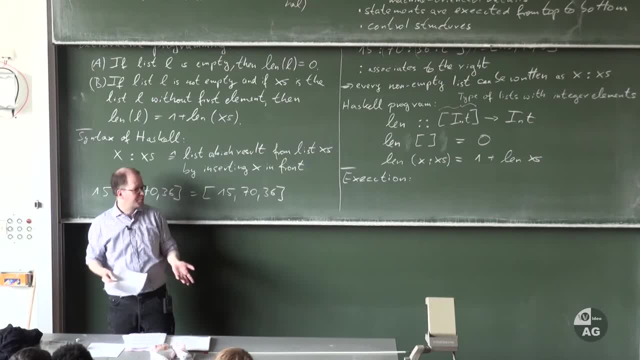 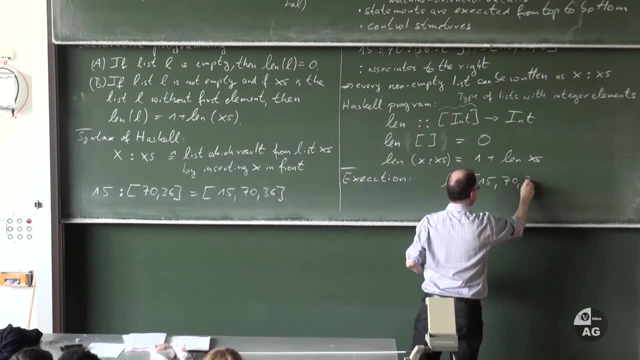 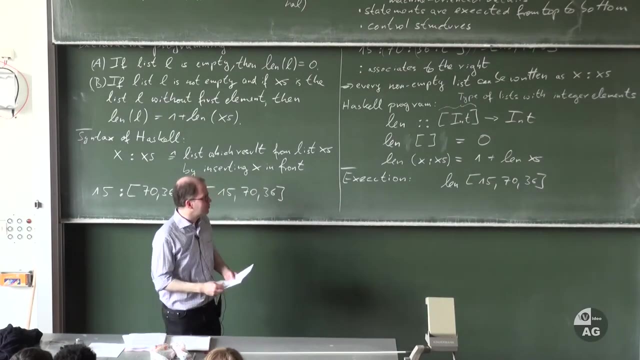 You type in some expression and then Haskell tries to evaluate this expression. So, For example, I can type in this expression, len of 15,, 70,, 36, and then I press return, and now Haskell should give me the result of this. It should try to simplify this expression. and well, to simplify this expression, Haskell uses it's knowledge, and it's knowledge is this: 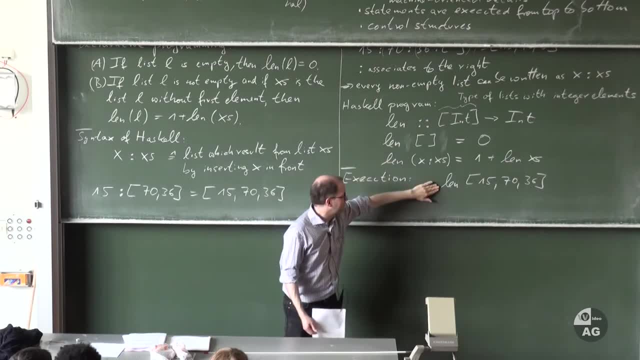 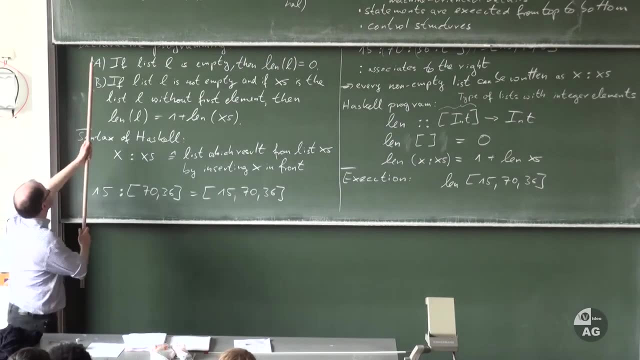 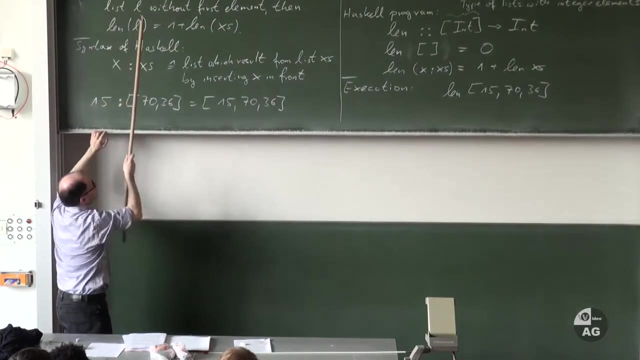 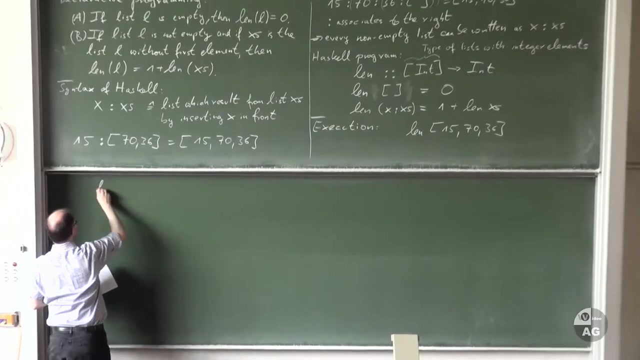 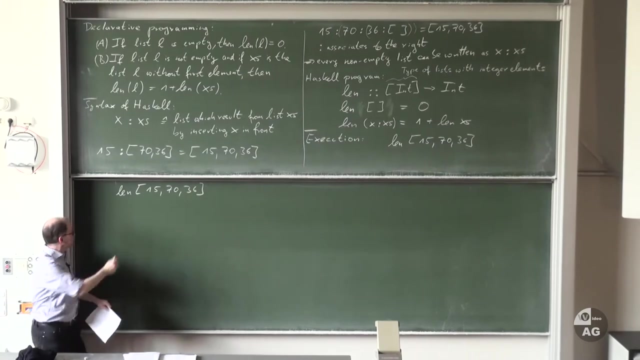 So Haskell knows this definition of length, and now it tries to simplify my expression by applying these equations. So let's do it, Okay. so how can this be simplified If I write len 15,, 70, 36? well then, Haskell knows that this is just an equivalent notation for the following expression: 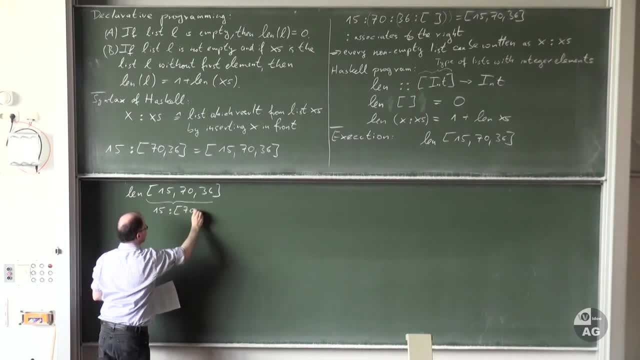 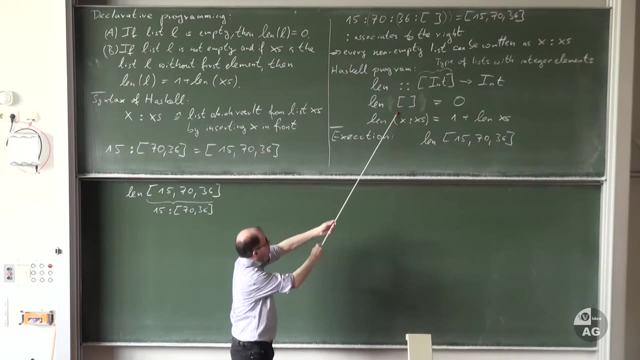 It's 15, inserted into the list 70, 36.. So every list can be written in this form. So, in other words, Haskell now checks from top to bottom. which equation can I use to simplify this expression? Well, in this first equation it's not helpful, because this only says something about the length of empty lists. 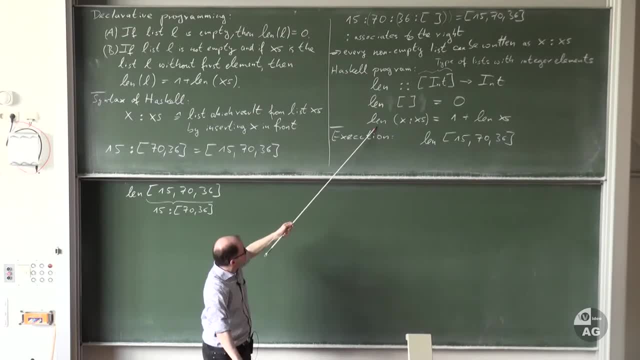 But this list is not empty. So Haskell tries the next equation, and here we see: okay, if x were 15.. So if this were x And if x's were this list, So if this would be x's, then this left hand side here would match. 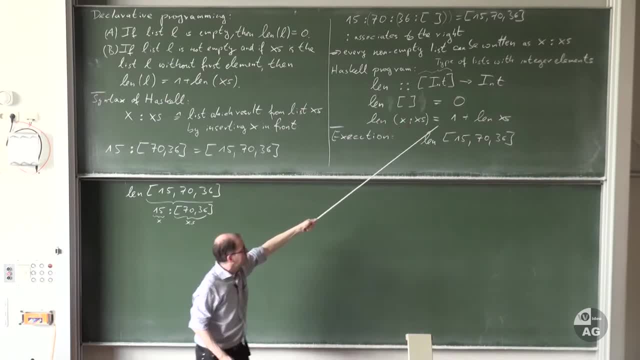 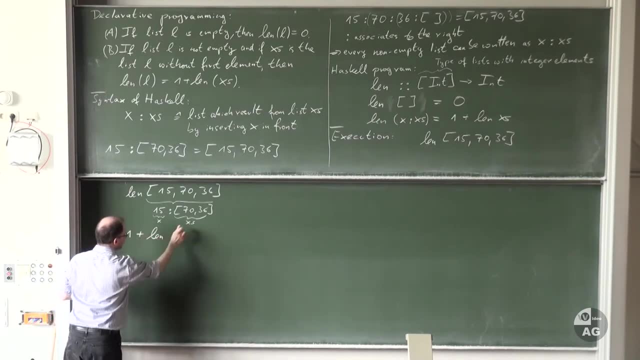 So then we could apply the second equation and replace the left hand side of the equation by the corresponding right hand side. So if I replace this, then I get 1 plus len x's, and x's in our example is 70, 36.. 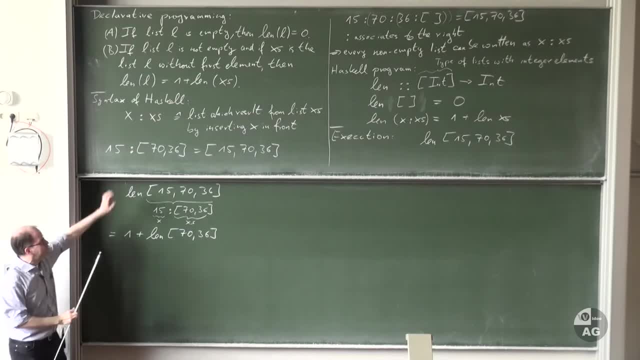 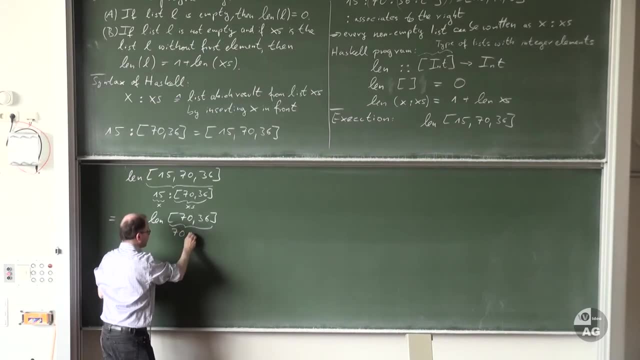 And now, of course, Haskell tries to simplify this repeatedly Until it cannot go on anymore- And 70, 36.. Well, that can be written in the following way: This is 70 inserted into the list 36.. So again, the second equation can be used here. 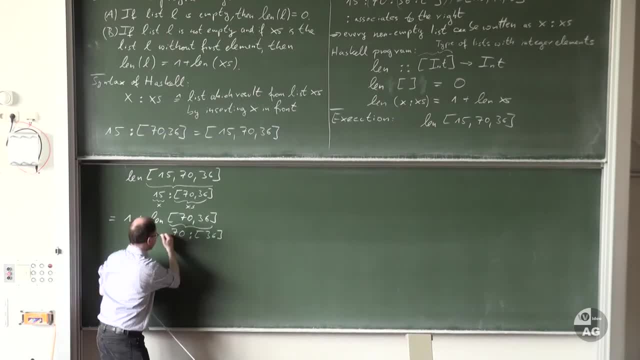 This time x is 70. And x's is the list with 36.. So this sub expression can be replaced by 1 plus len x's, Where x's is this list over here. So we get 1 plus 1 plus len list with 36.. 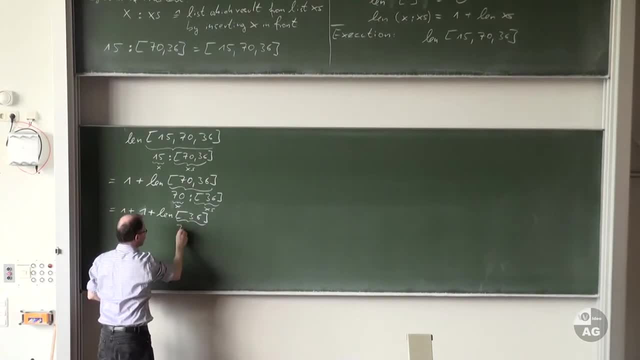 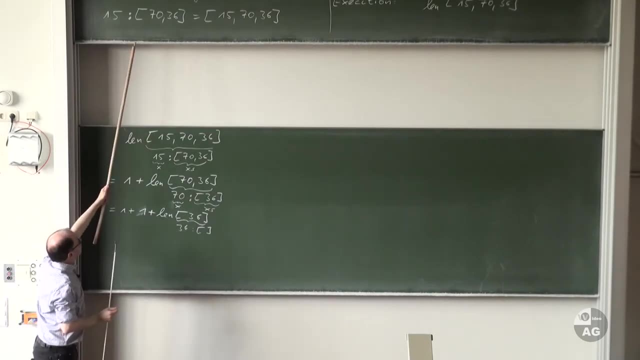 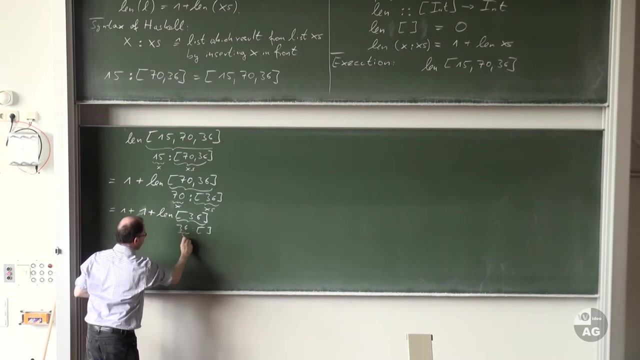 And now the thing can be repeated again. So this is the list 36, inserted into the empty list. Now we cannot see the definition anymore. Here it is. So again, this corresponds to x, This corresponds to x's, And we get. 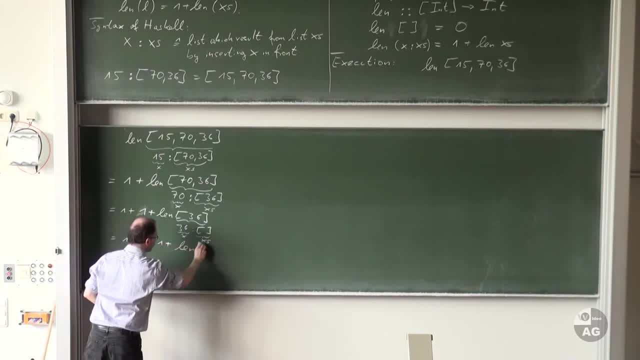 1 plus 1 plus 1 plus Length of the empty list. And now, finally, the first equation can be used And the length of the empty list is 0. So we get 1 plus 1 plus. 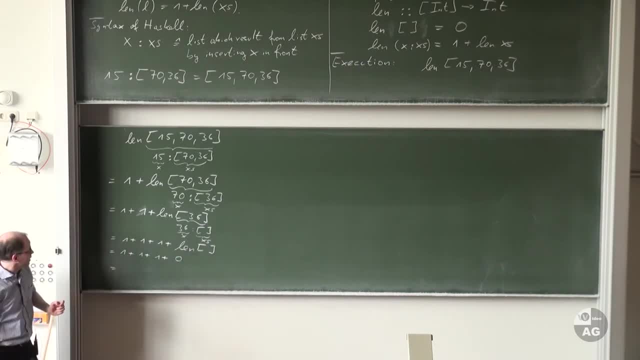 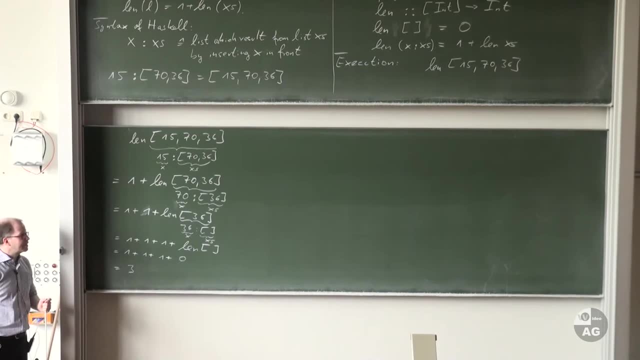 1 plus 0. And plus is predefined in Haskell like in any other programming language. So Haskell can add up all these numbers and we get 3. Which is what we would have expected. So what are the characteristics compared to the imperative program up there? 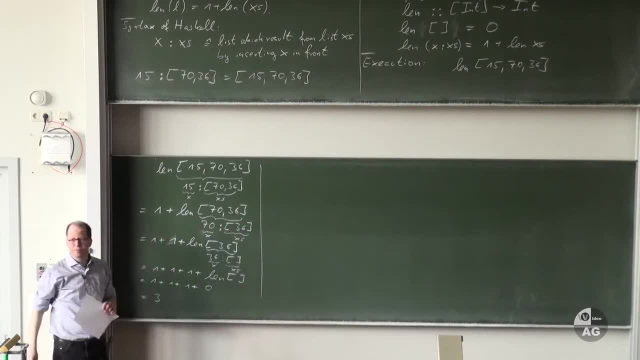 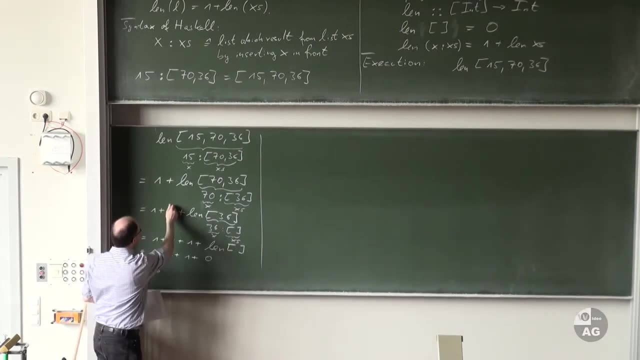 Excuse me, Yes, Wouldn't 1 plus 1 be executed first? Well, it depends. So let me write down brackets, Because in reality we have this, So we had 1 plus length of this, And plus can only be executed in Haskell if both arguments are numbers. 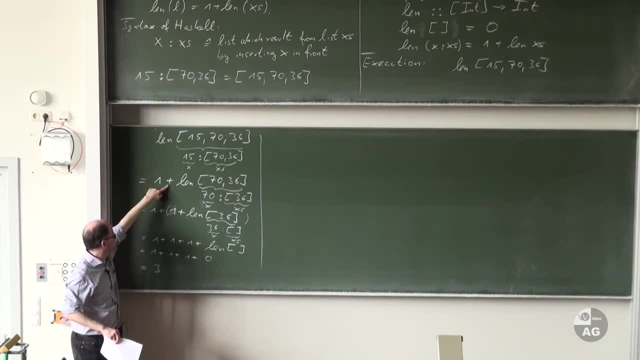 And well, this is not yet a number, So this plus I cannot execute. So I first have to evaluate this len. And now Haskell does not know that plus is associative, So that you can move these brackets over here. Well, we know this. 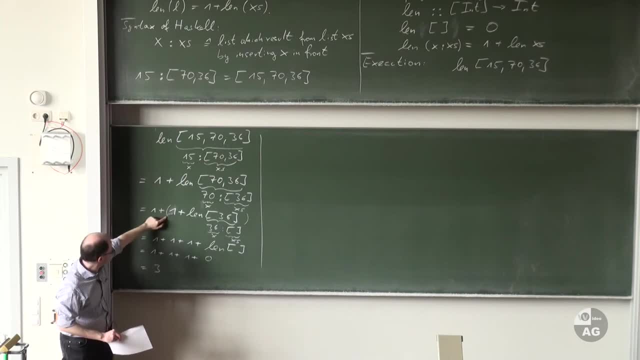 But Haskell doesn't know this, At least I assume that Haskell doesn't know this. So brackets are like this: So we have to evaluate this, And then we have to evaluate this, And then in the end it looks like this: So the first plus that can be executed- because both arguments are numbers- is this: 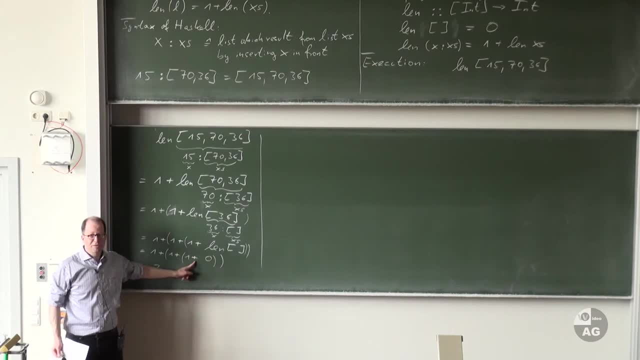 So only at the very end I can execute these pluses. Of course there could be other algorithms where you could Evaluate plus earlier, But in this example you can only evaluate at the very end. Of course you could think of a clever compiler. 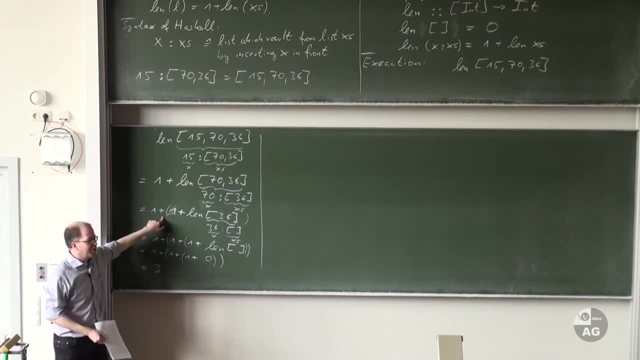 That knows that plus is associative, And then you can move the brackets over here. But I don't know how the This probably depends on the Haskell compiler Whether it knows that plus is associative or not. But if you would do this with minus, 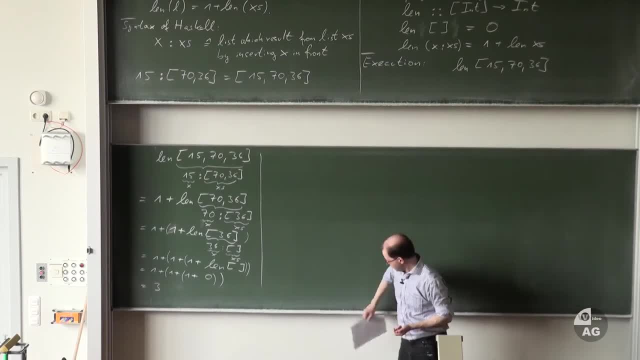 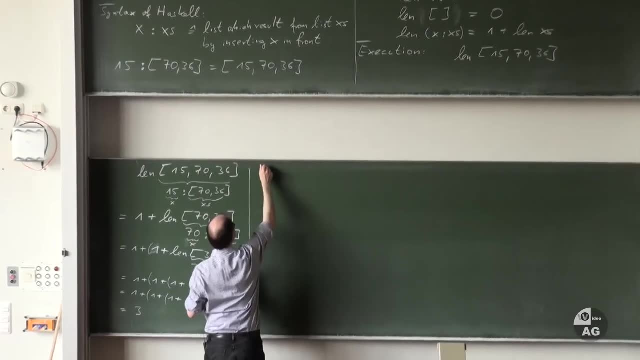 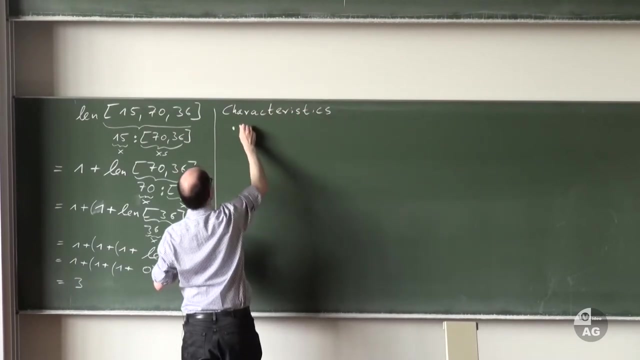 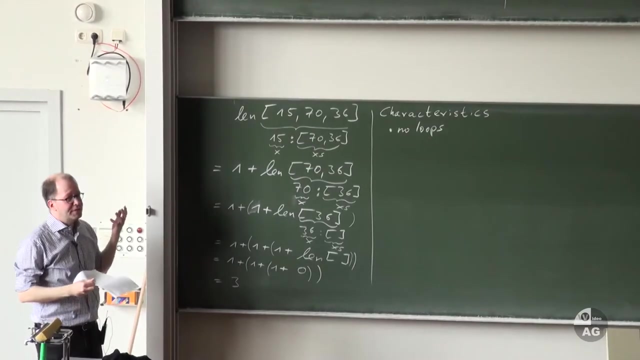 Then definitely minus is not associative. Okay, so what are the characteristics? Well, if we compare the Haskell program with the Java program, What do we see? There are no loops. So the concept of while loops does not exist. So if we want to do something repeatedly, then we have to use recursion. 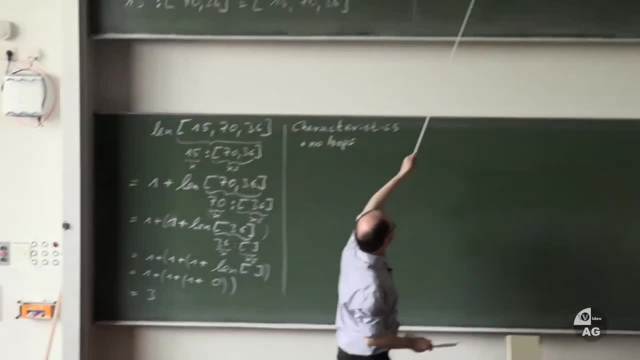 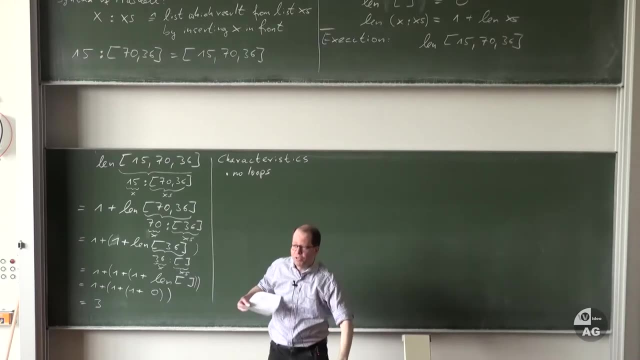 And that's indeed what we did up here. So length is defined recursively. in order to compute length- The length of this list- We have to compute the length of the smaller list, And so the only way to have something repeatedly is recursion. So no loops. 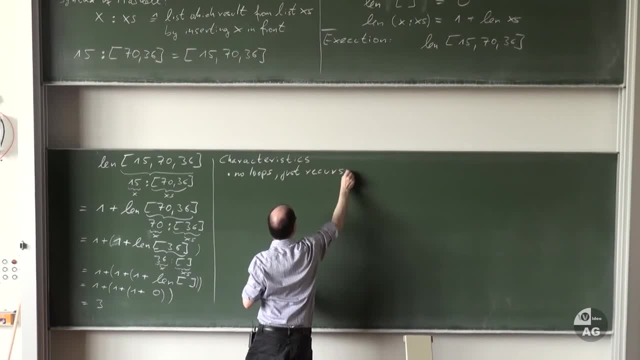 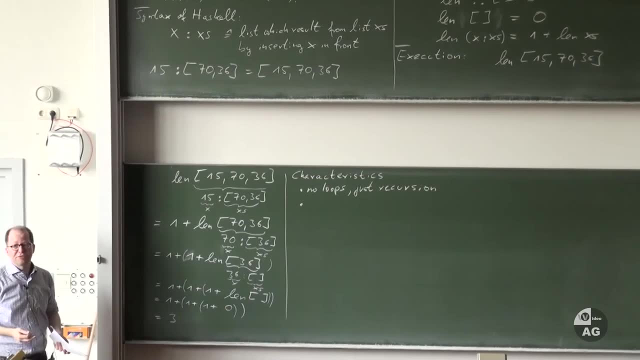 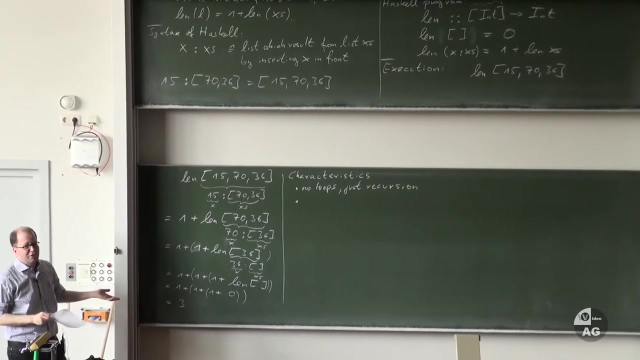 Just recursion. Then something very important is: we have no side effects. So this problem that we had in this Java program, Where we accidentally erased the whole list, That cannot happen here. This is really a function. So it's a function like in mathematics. 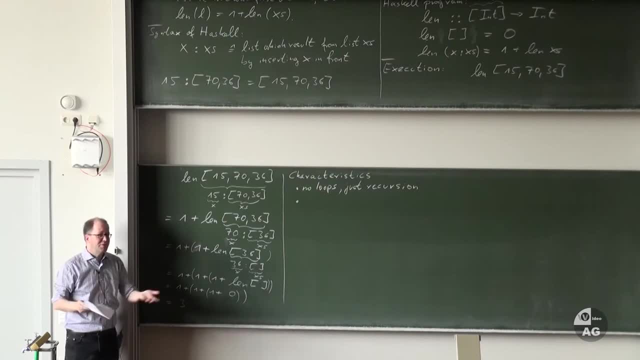 The function is applied to certain arguments and you get a result. And it doesn't matter how the memory looks before And also the memory is not changed afterwards. But if you apply length to this list, you always get the result. 3. Always, 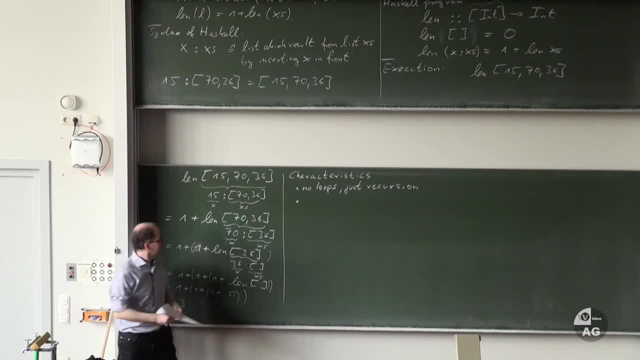 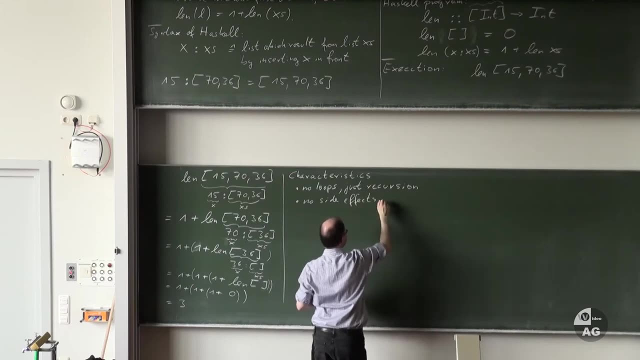 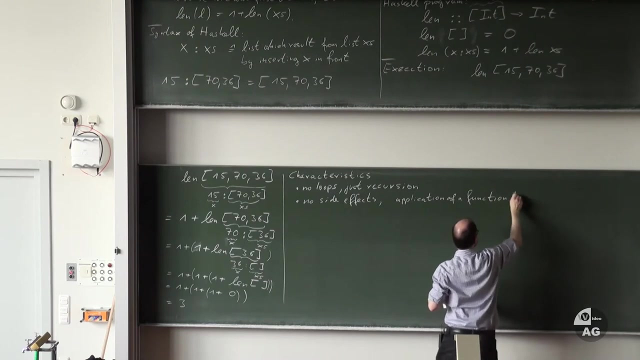 No matter how the memory looks like before. So we have no side effects. No side effects, And if a function is applied to the same arguments, you always get the same result. So application of a function to the same arguments always yields the same results. 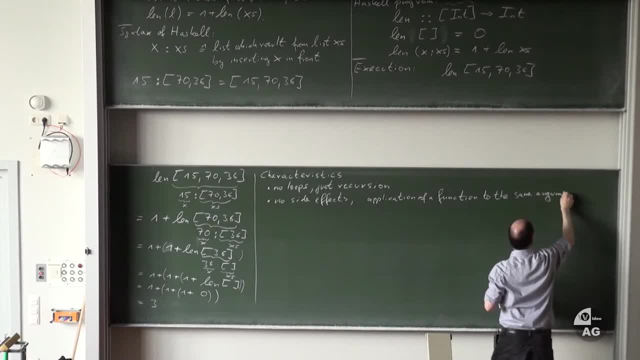 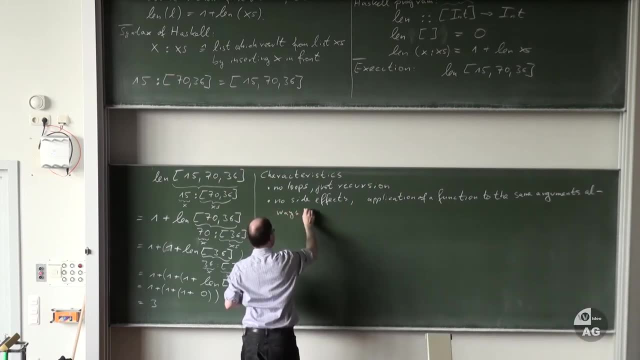 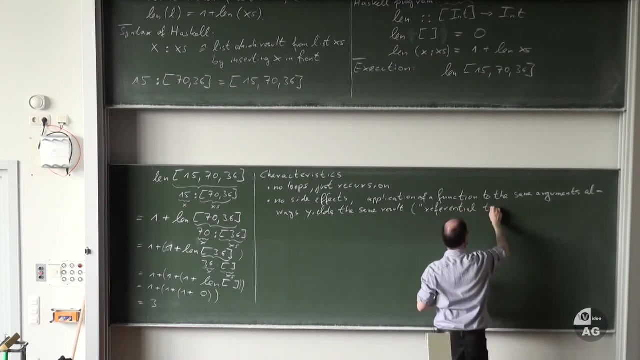 To the same arguments always yields the same result, And this is called referential transparency. Referential transparency. Another important thing is the type system Because, as you already pointed out before, Why do we only use this length algorithm for lists of integers? 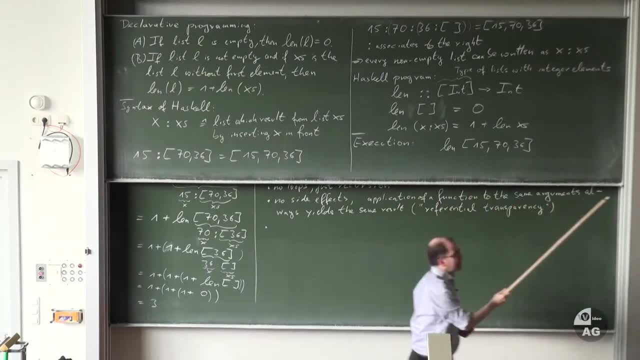 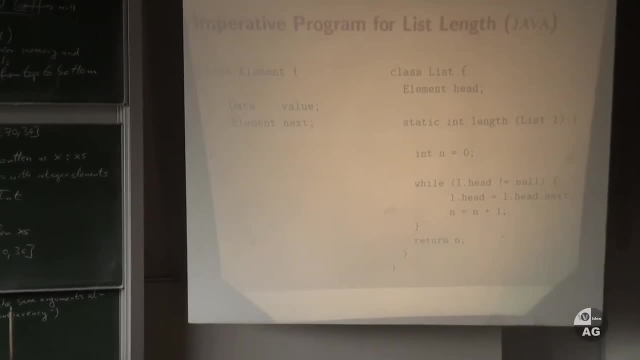 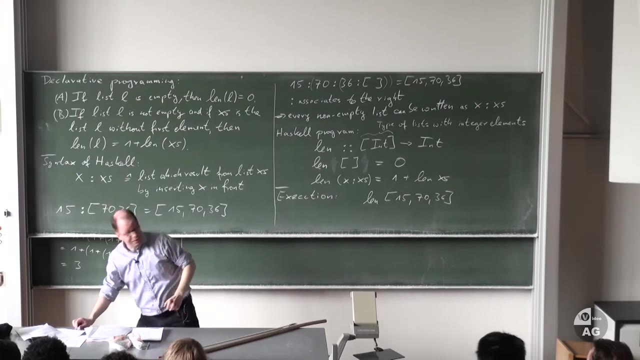 I mean here in this Java program. I said that the values in this list are of some type data, So there is some class data. We don't know what that is. In Java we can do something like this. In Haskell we can do something similar. 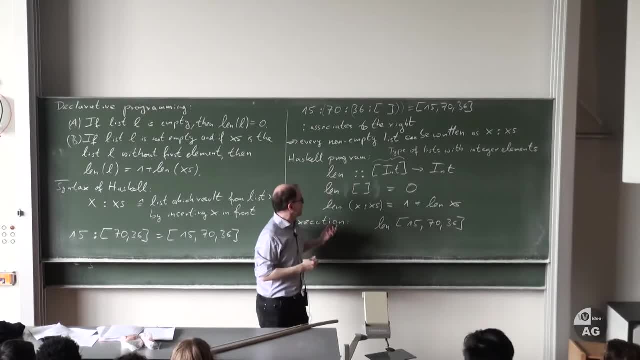 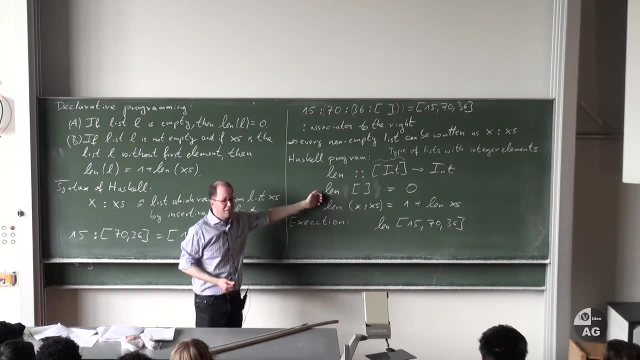 We can say: well, it doesn't have to be lists of integers, But lists of Booleans are fine as well, Because if the list consists of Boolean values, Length would be computed in exactly the same way And lists of strings would also be exactly in the same way. 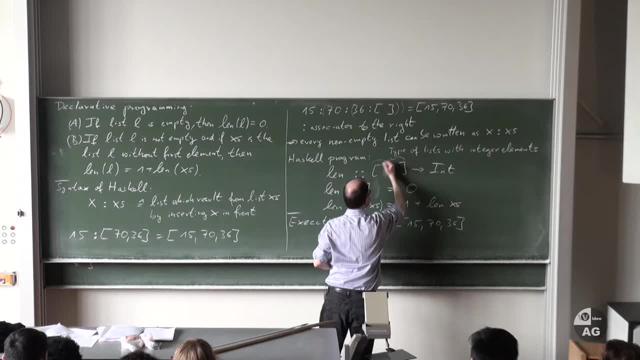 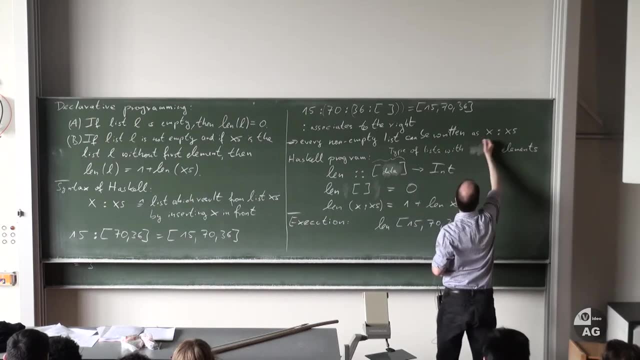 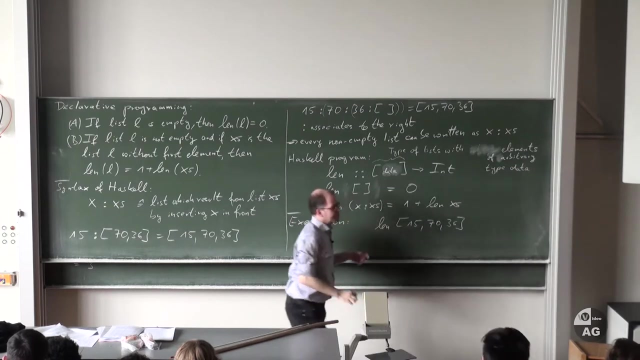 So lists of anything are allowed, And so let's replace this int by, for example, data, And this is the type of list with elements of some type of an arbitrary type data. So now this data takes the role of a type variable, And you can apply this to lists of integers. 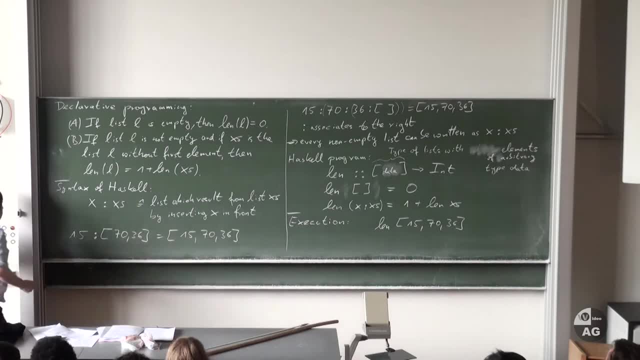 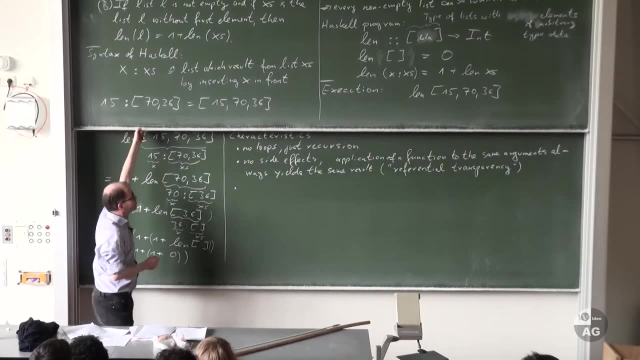 But also to lists of Booleans or lists of strings or lists of anything. So this is the idea of the polymorphic type system. We will do this in more detail later on. I mean, this is just the introduction, to give you an impression what Haskell can do. 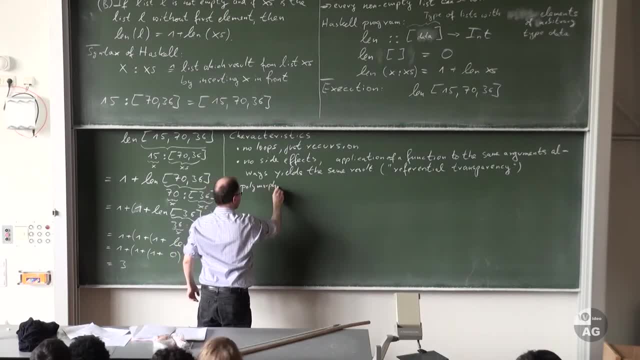 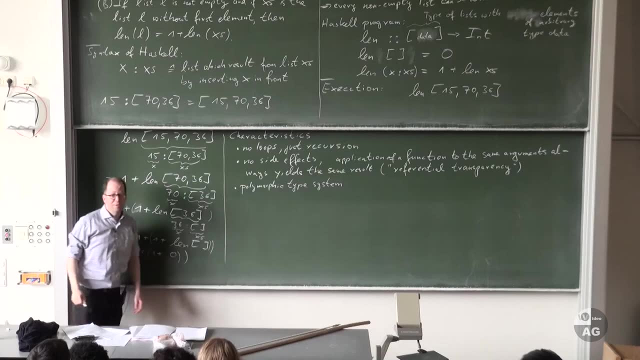 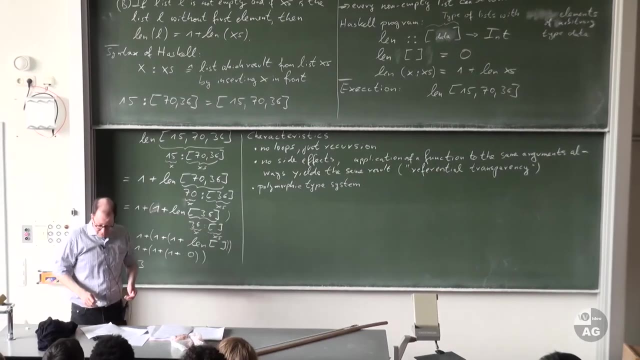 So we have a polymorphic type system And Well, Well, for those of you who know generic types from imperative programming languages, That's the same concept And that was developed in functional programming And later on Imported to the imperative programming world. 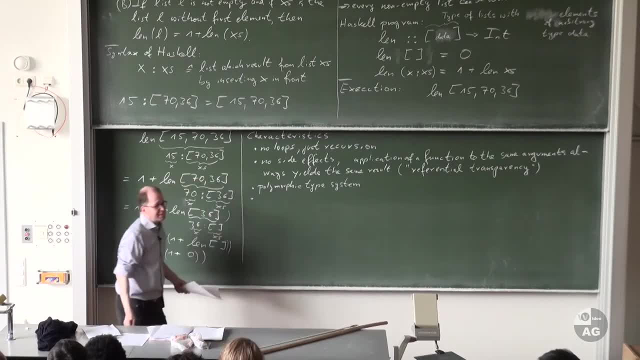 So what else do we have? Well, Memory management is done automatically. So, Yes, I want to refer to the second point. Yes, The side effect I mean in Java you had, It's a memory, There's written something on it. 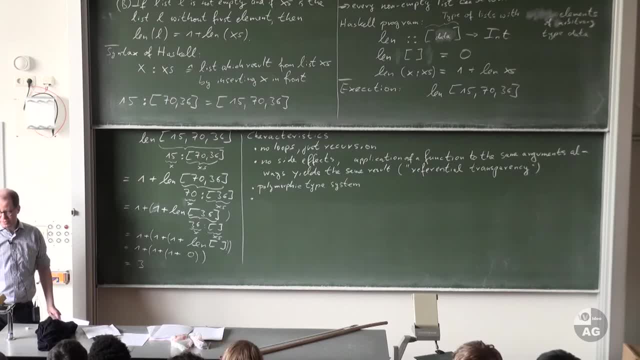 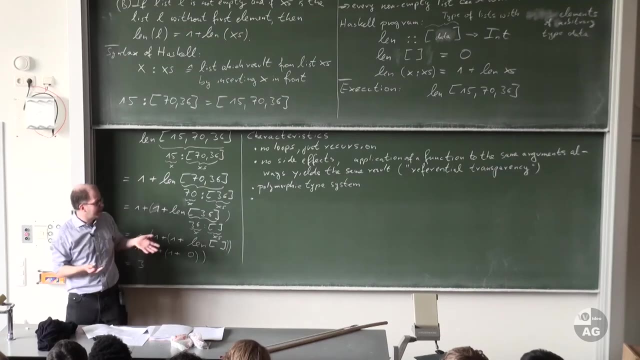 Then you can get wrong results. Yes, Why can't it happen here? It can't happen here because It doesn't matter what the state of the memory is before the execution. You never access anything in the memory except the arguments. So in Java, 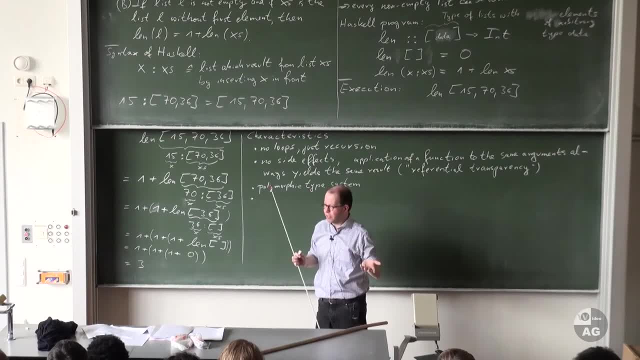 For example, in Java you could have global variables, Or in imperative programming you could have global variables, And when you execute your function You access the value of these global variables. You look into your memory and see what are the values here, And your result depends on the values of these global variables in your memory. 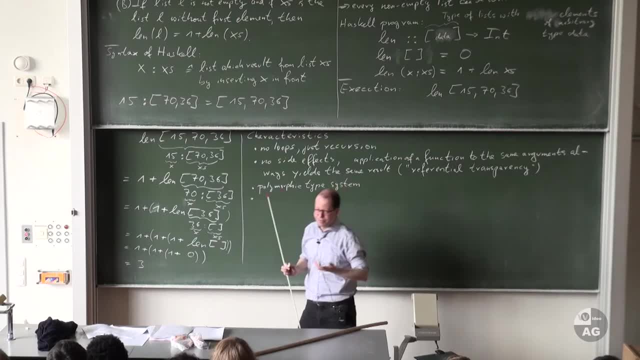 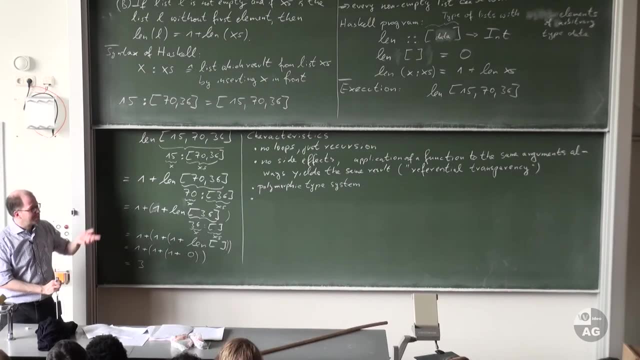 That cannot happen here. So in that sense The result does not depend on the state of the memory And also the memory is not changed. I mean, here we have this problem that the list is erased While computing the length, And something like this can never happen here. 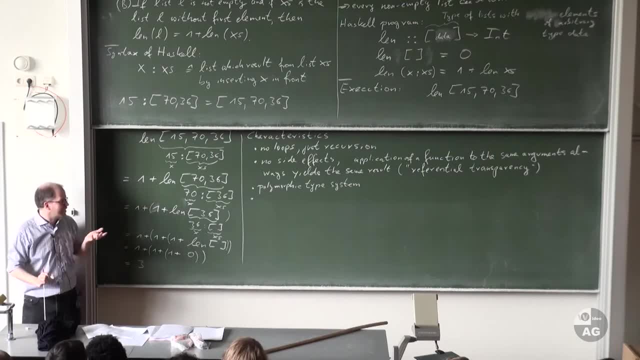 So you don't have to think about- Well, ideally you don't have to think about- what happens in the computer. It's just this function And this function is computed And how this works. You don't have to think about it If you're not interested in efficiency. 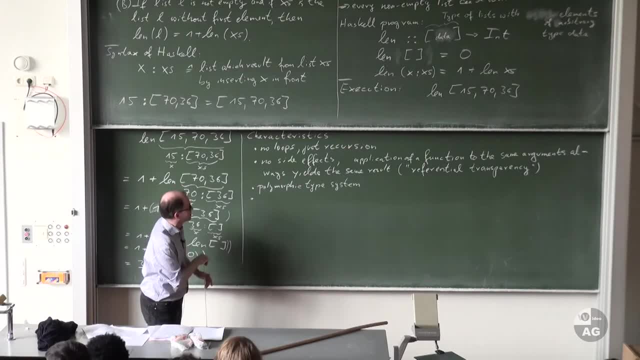 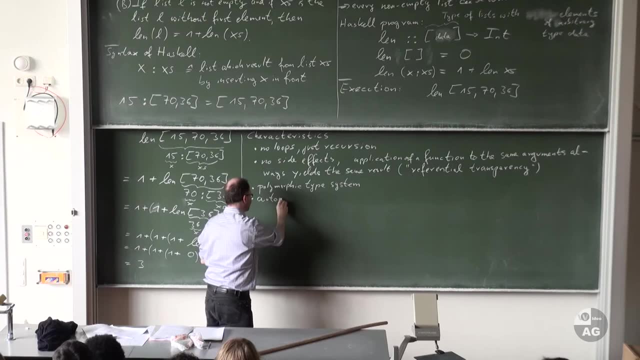 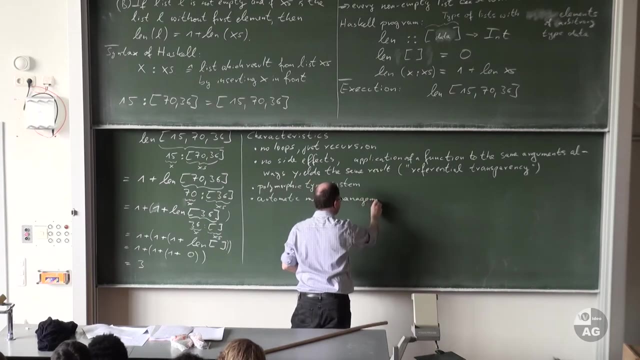 So sometimes you should think about it, But you have to think about it much less than in imperative programming. So we have automatic memory management. So in particular, there's no need to allocate memory Or to free memory again. There's a garbage collector. Of course this is also the case in some imperative languages. So in Java you also don't allocate memory, You also don't free it again And there's a garbage collector. But in languages like C You have to do this yourself. So in functional languages you don't have to do this yourself. 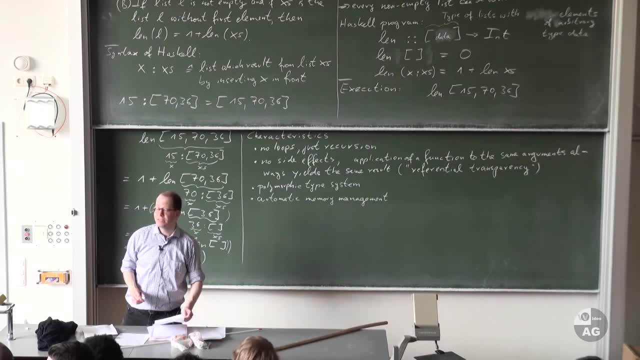 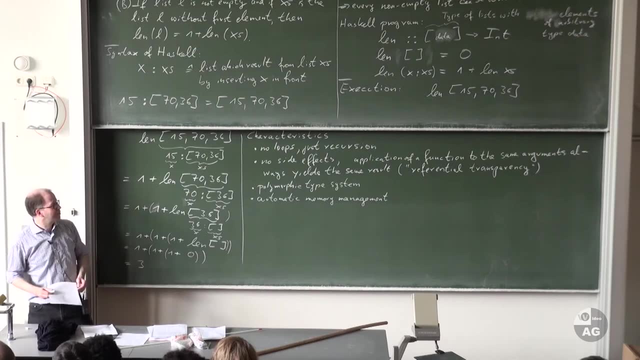 One more question. Yes, You named the type variable data- in the main function. Yes, Doesn't data have a keyword? No, No, you can name it as you like. So very often you just call this a Small a, But I called it data. 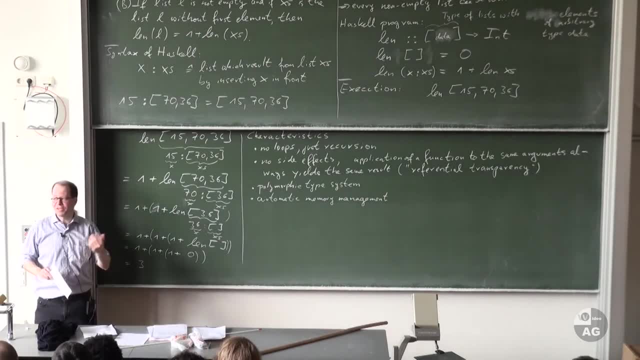 To have the same name as in this Java program, So that was the only purpose. You can call it. I thought it was a Haskell keyword. No, It's not a Haskell keyword. You can call it as you like, So it's just. 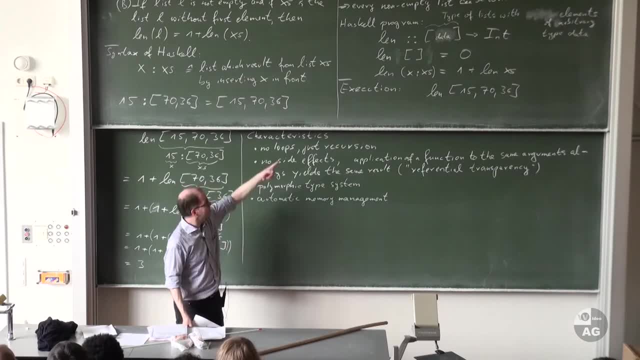 Yeah, So int is a Haskell keyword, But data is not a Haskell. At least not at that point. It's not a Haskell keyword. So what else is important? Well, Functions are first class citizens. So in other words, Functions are. 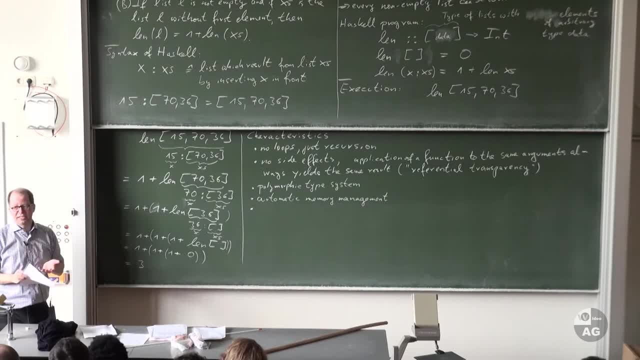 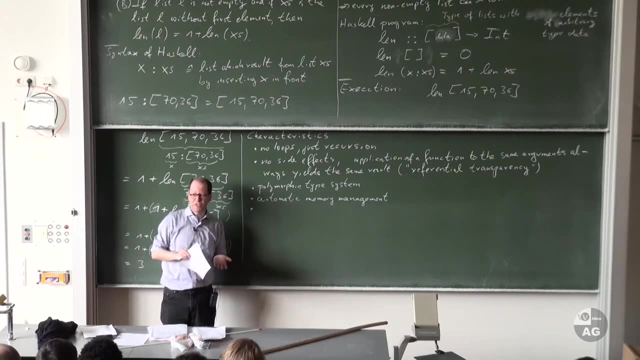 Functions are data objects like any other data object, And that means You cannot only write functions that take an integer And give you back an integer, But you can also take functions That take functions as arguments Or that produce functions as results. 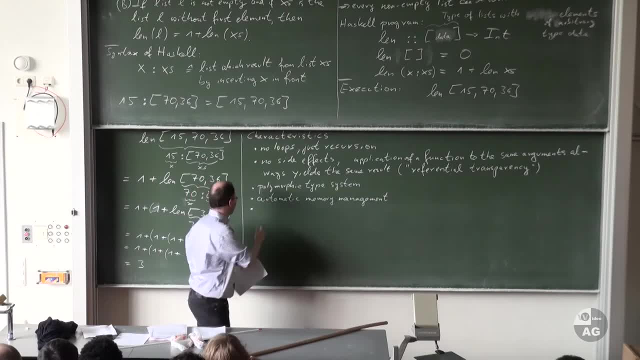 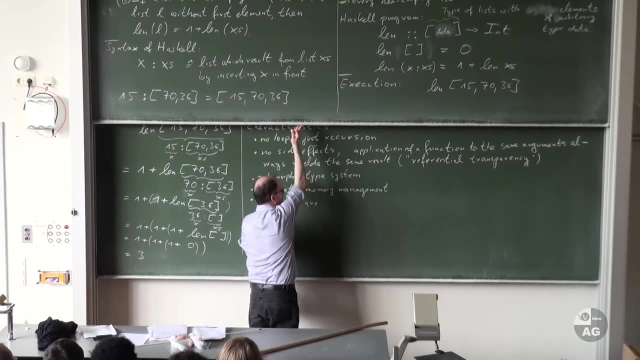 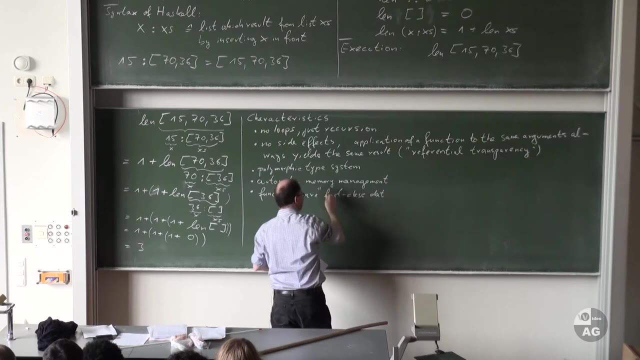 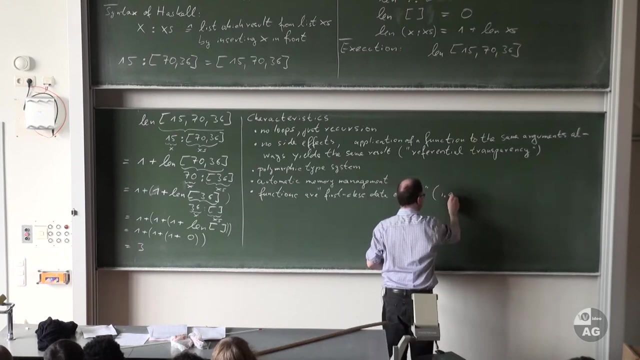 So functions are just data objects Like any other data objects. So Functions are Well, let's say, First class data objects, So First class data objects, And what that means is: So what does this mean? This means Functions can. 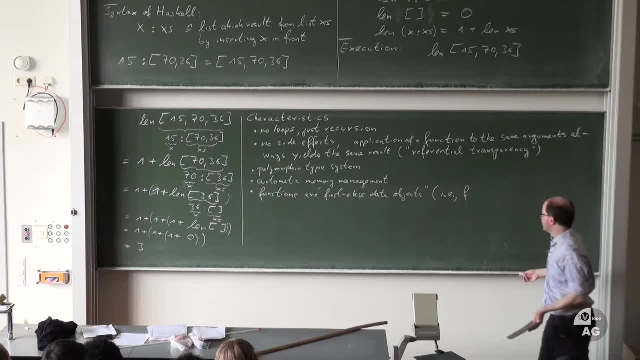 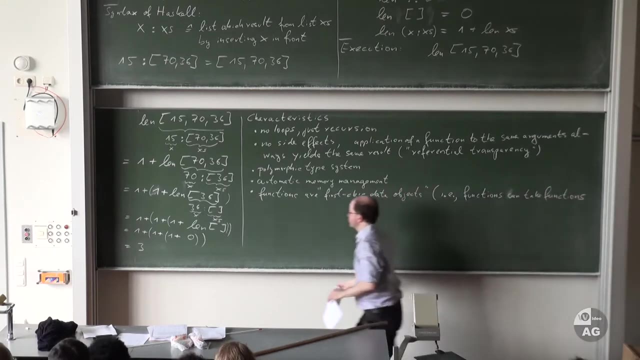 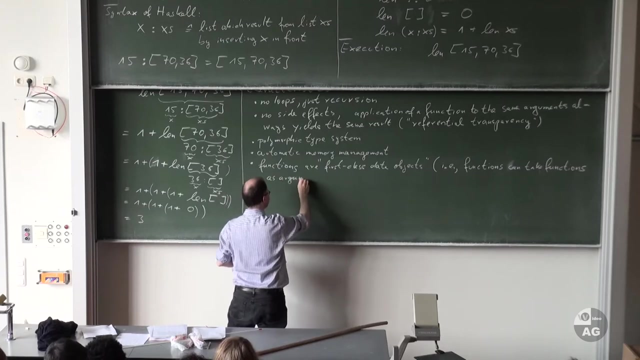 Again take functions as arguments Or they can produce functions as results. We haven't seen examples for this yet, But we will See examples later. So functions Can again take functions as arguments Or as results. Functions can take functions As arguments. 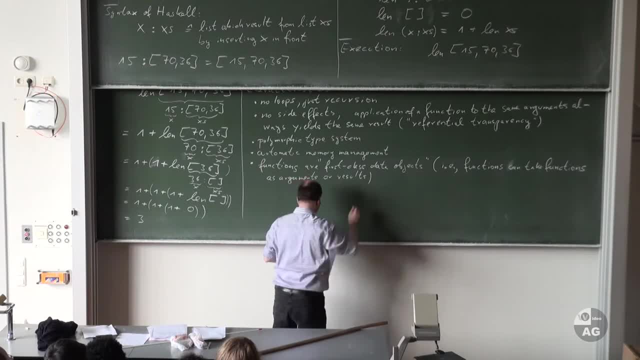 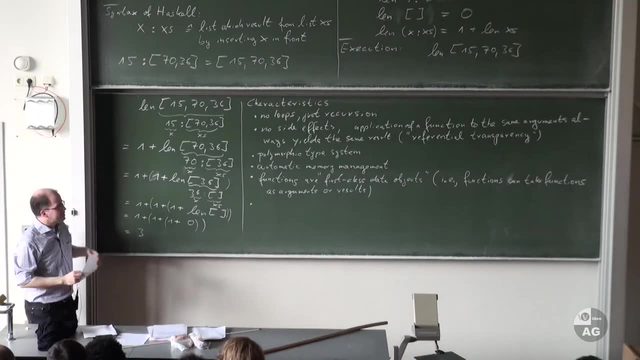 Or results. And then The last important characteristic, At least of Haskell, Is the evaluation strategy, And that's A particular characteristic of Haskell. That's not true for every functional language, But Haskell has A so called lazy evaluation strategy. 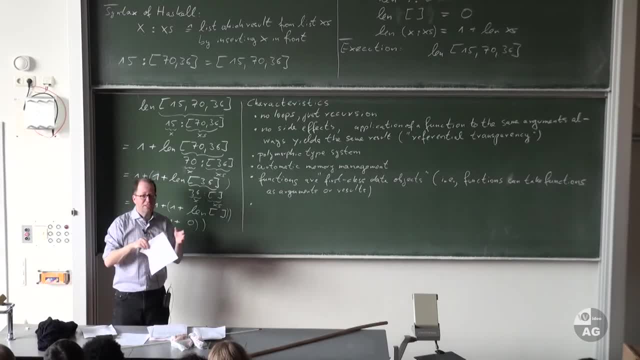 And the idea is That evaluation does not start At the innermost point of an expression, But as the At the outermost point of the expression. So you Only evaluate those parts of an expression That you really need for the result. 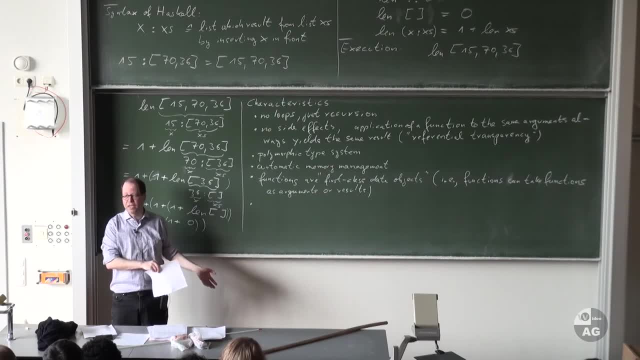 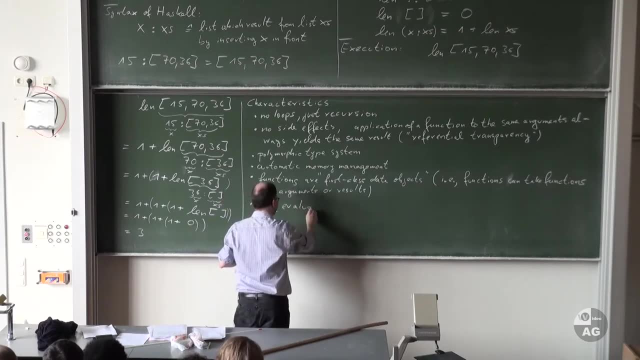 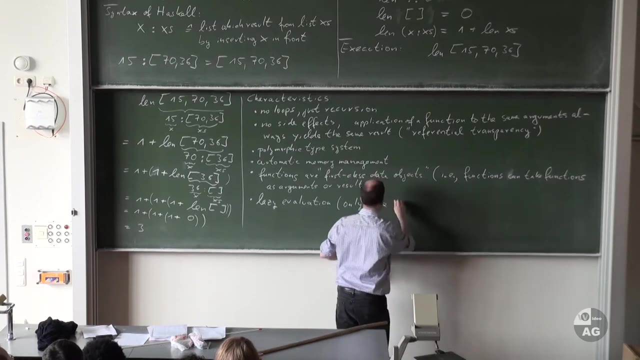 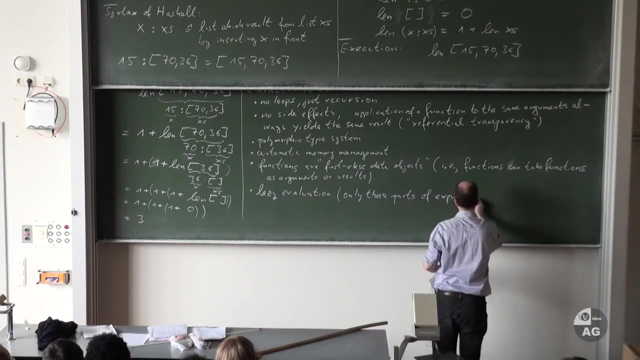 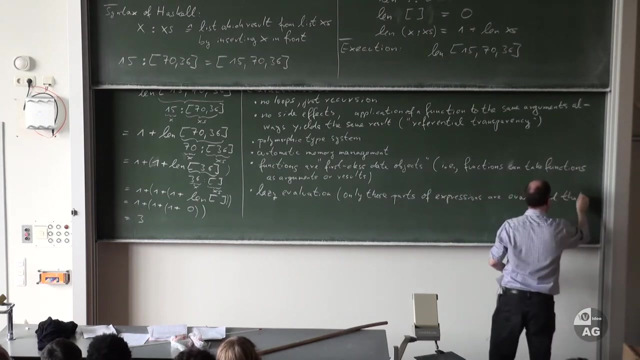 And those parts that are irrelevant for the result Are not evaluated at all. So Lazy evaluation, And that means Only those parts of an expression are evaluated, Only those parts of expressions are evaluated That are really needed for the result Are evaluated. 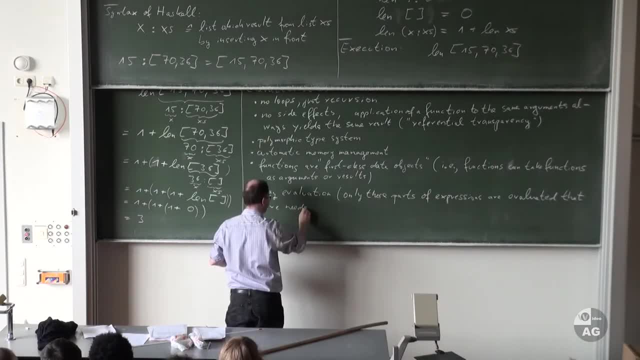 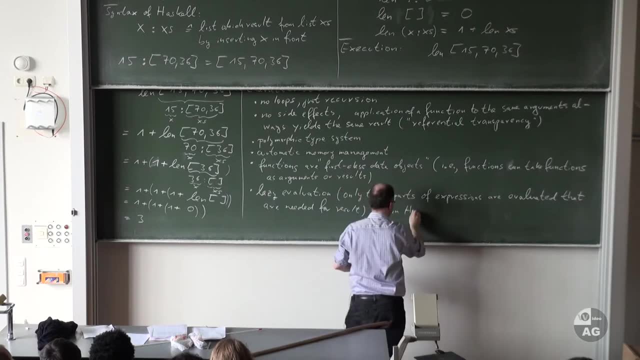 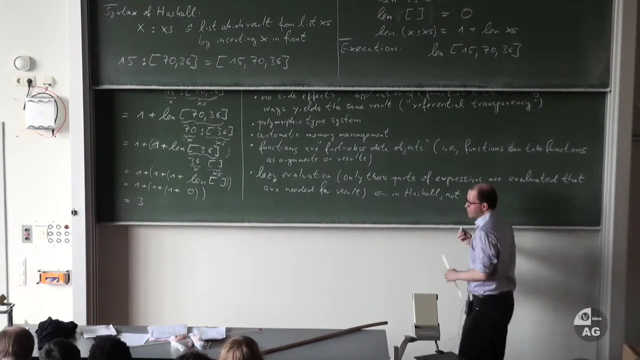 That Are really needed For the result- And that's a Feature of Haskell, But Not In every functional language. So, For example, Popular other functional languages Are ML Or Lisp Or Scheme, And in these 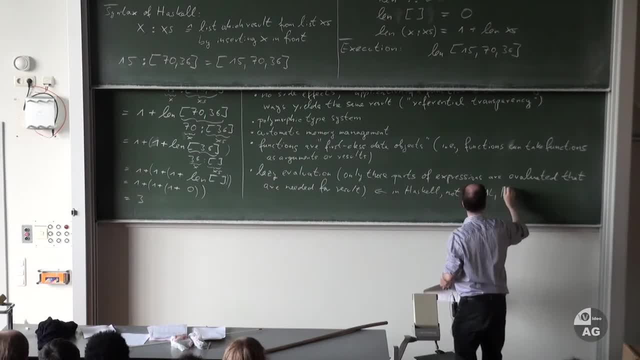 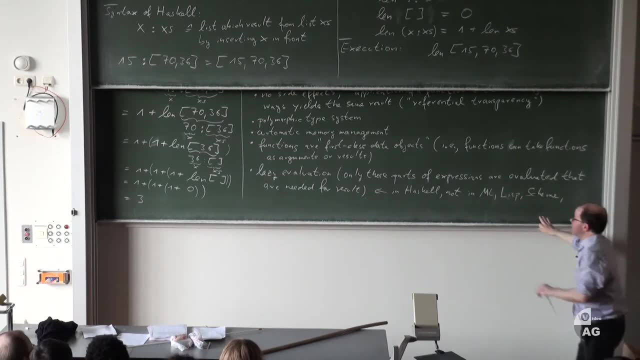 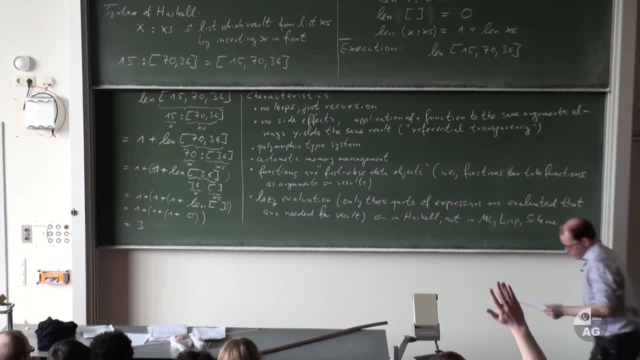 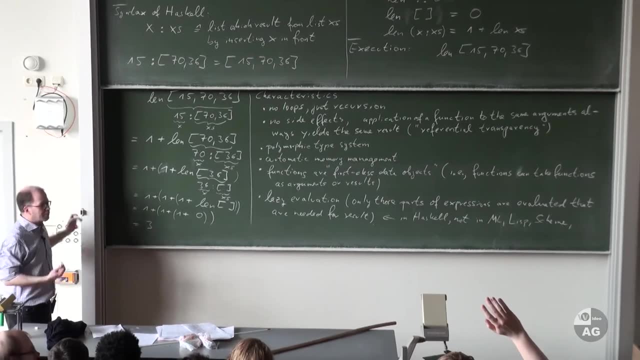 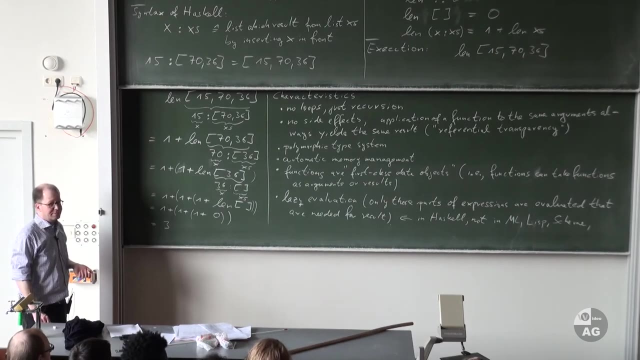 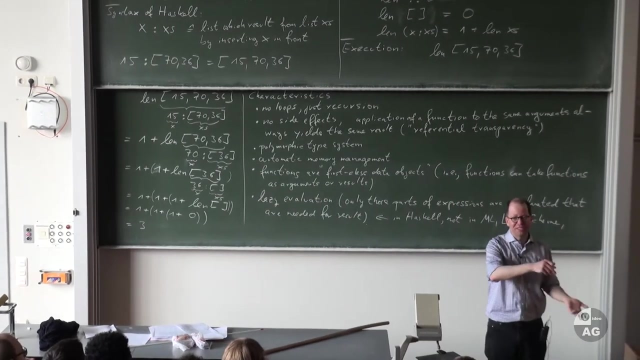 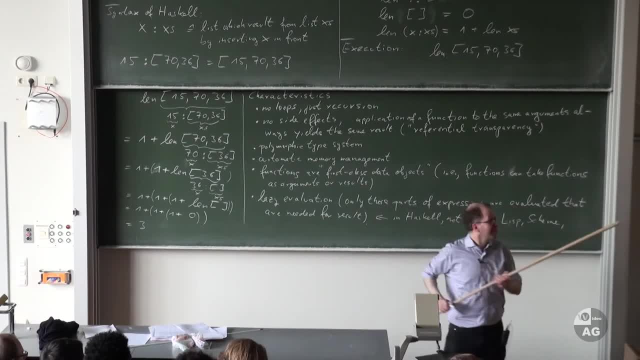 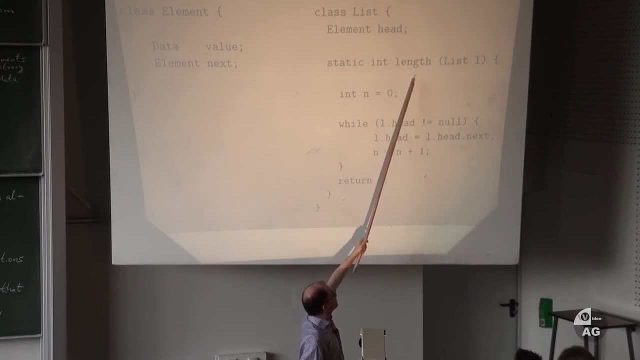 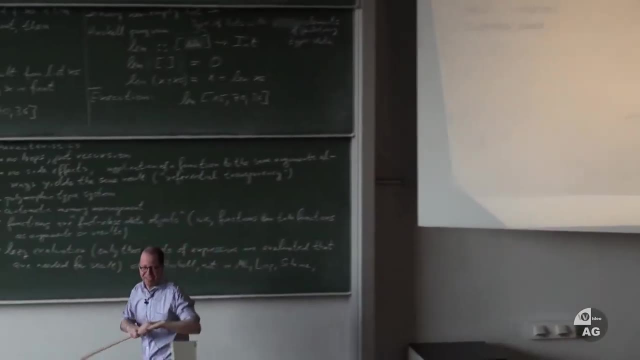 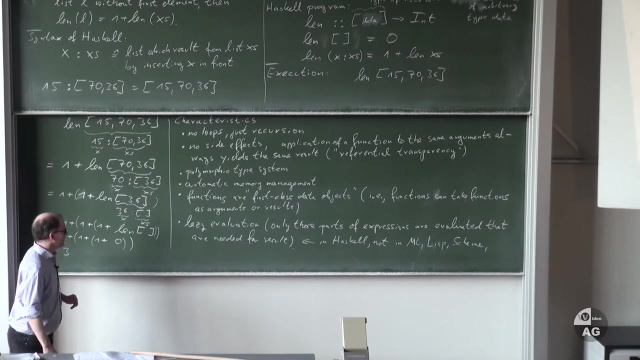 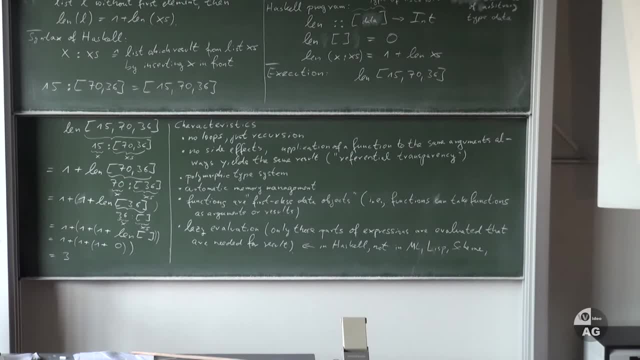 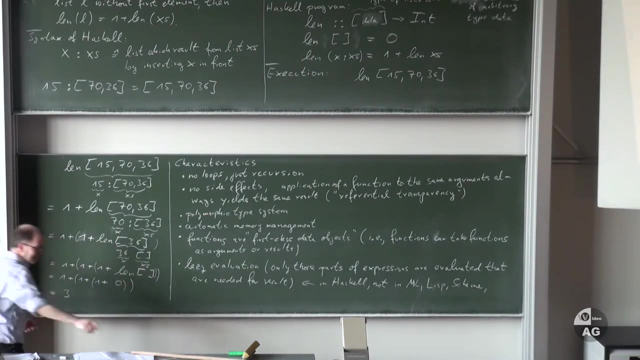 So, So, So, So, So, So, So. Well, data is a result evil, OK, then It's a keyword for a different purpose, Then let's rename it to something else. Let's rename it to A, and then it will compile for sure. 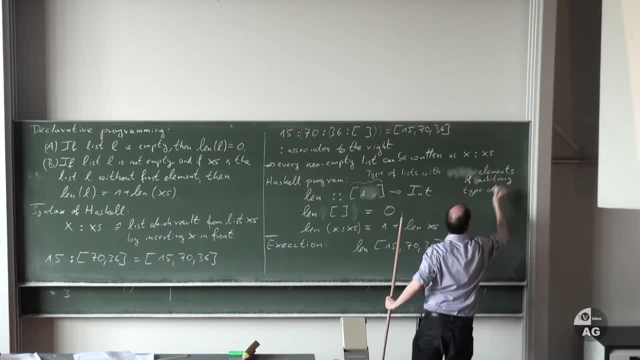 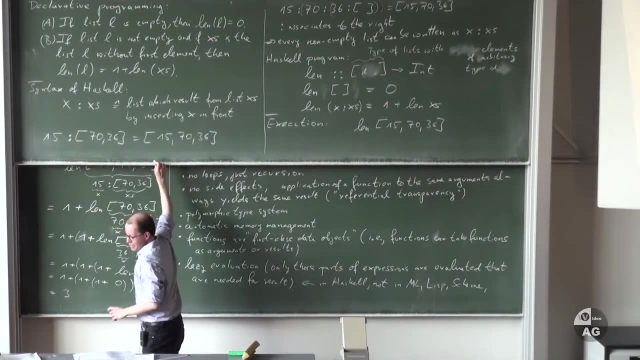 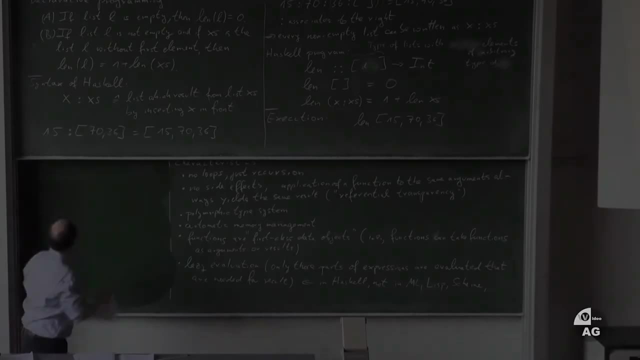 Let's call it D, So the data. OK, now I called it D, and now I'm sure it compiles, You're right. So what's the plan for the lecture? What will we do in this lecture? So what's our plan? 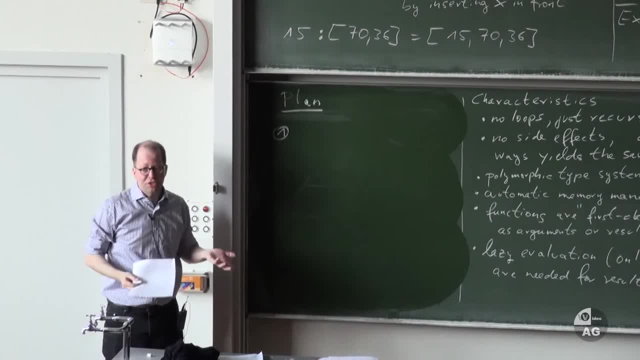 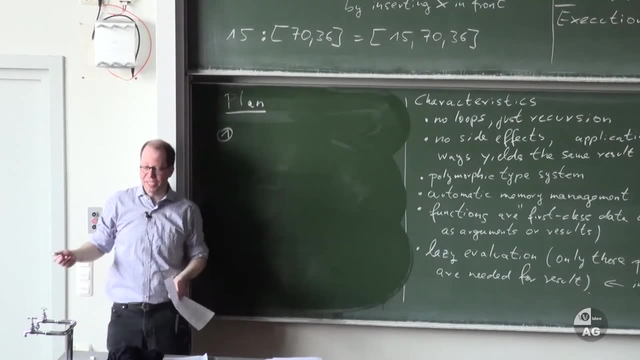 Well, we will start with an introduction to an actual functional language, namely to Haskell. So I mean we want to do this concretely. It's not just an abstract lecture, but we really work with a concrete functional language, and we take Haskell. 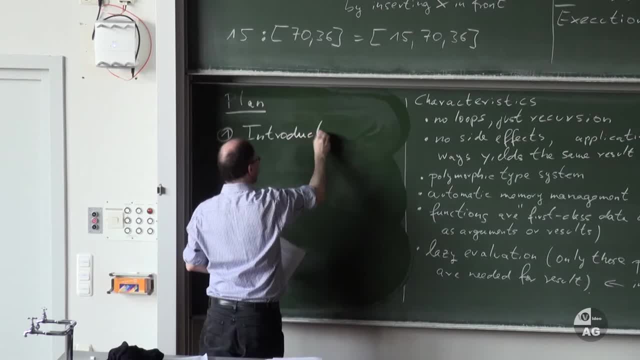 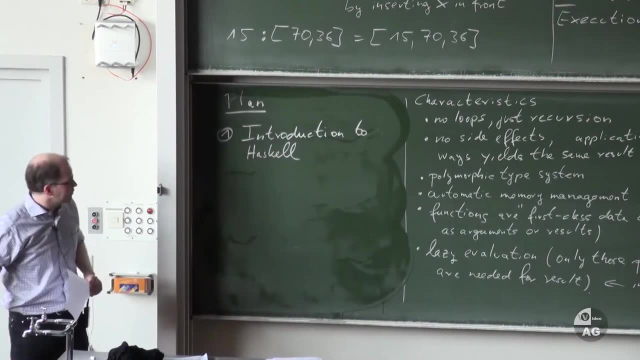 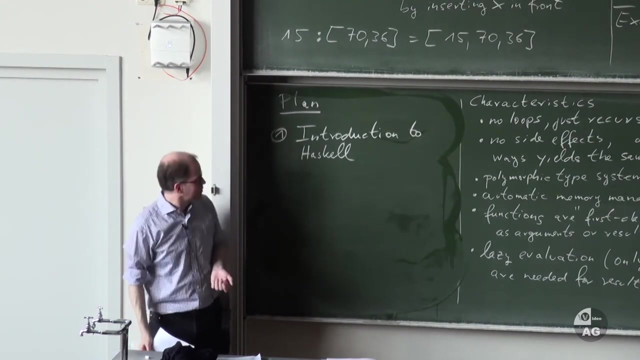 So we start with an introduction to Haskell, And so, in particular, we introduce the syntax of Haskell here, And for those of you who studied in Aachen, you will know Haskell already a little bit, because we did this in the first year course. 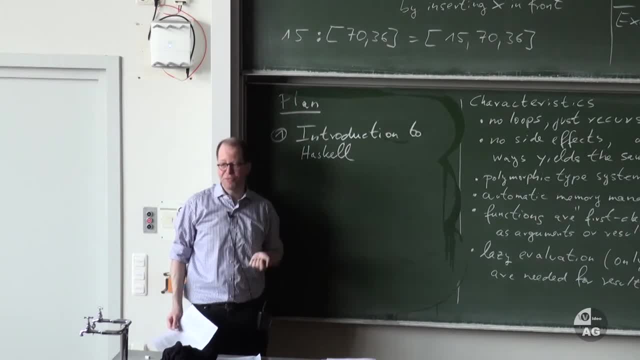 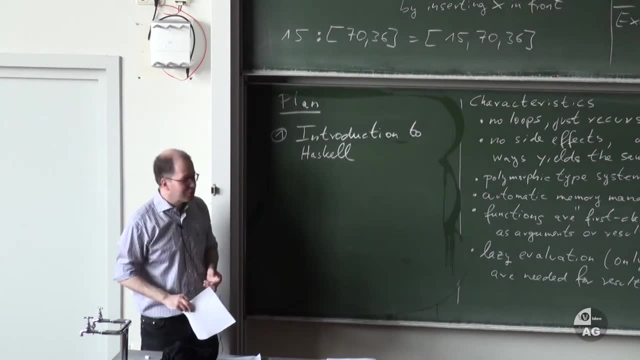 So this is a strict superset of what has been done in the first year course. So there will be some boring parts, but hopefully many non-boring parts, And for those of you who don't know Haskell, this will all be very interesting and not boring. 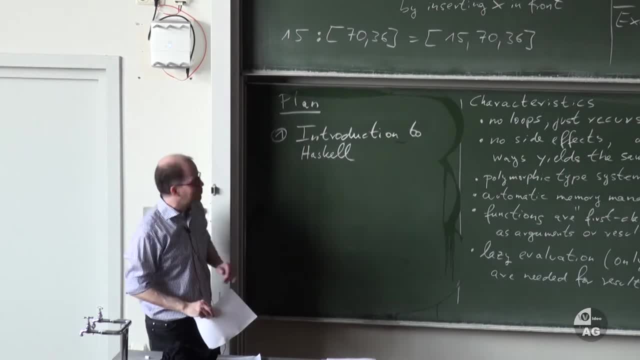 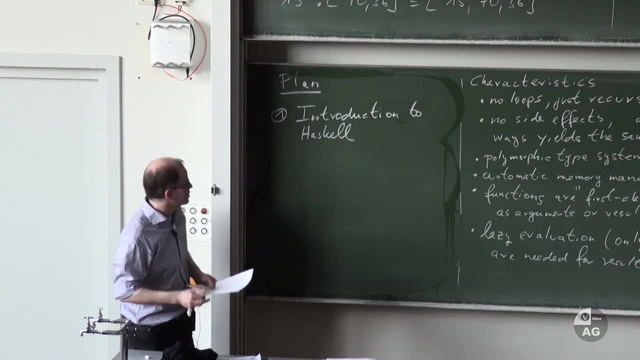 So don't worry if you don't know Haskell, that's fine, And don't worry if you do know Haskell, that's also fine. So, well then, you will know some of these things, but there will also be many things that you don't know. 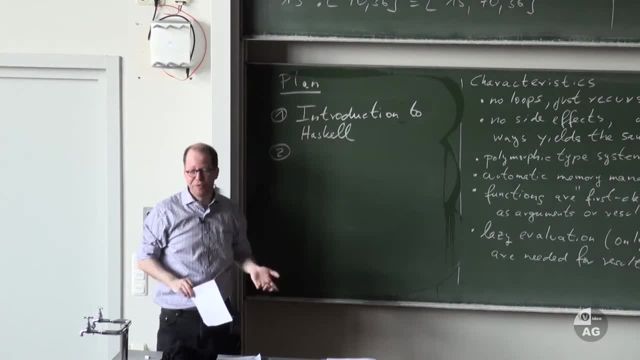 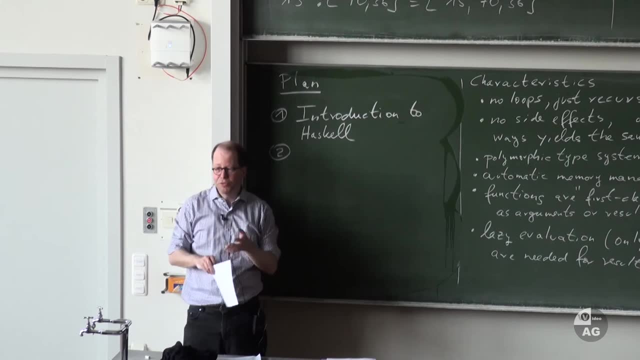 So in that sense, this is the practical part of the lecture, because we really have a concrete functional programming language, And then the remainder of the lecture is the more theoretical part, And we do this with a concrete language. So we do this all with Haskell. 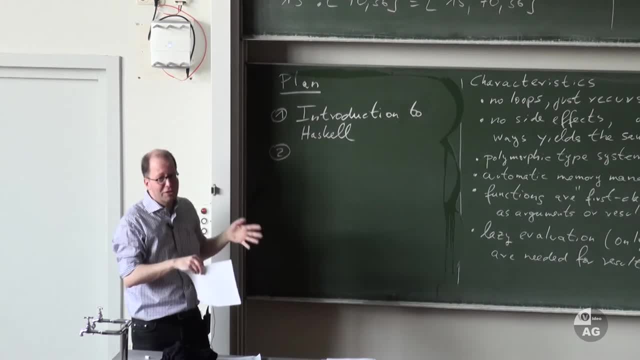 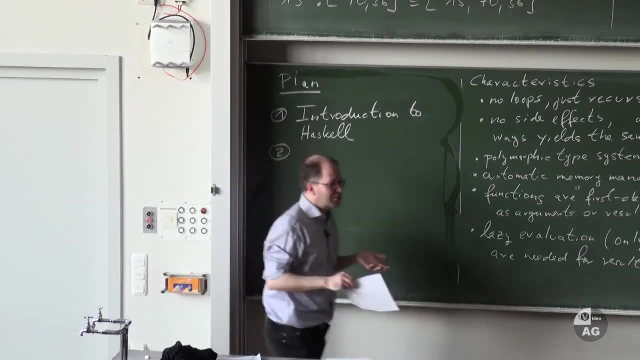 And well, here we introduce the syntax of the language. So what are the constructs that you can write down? What is a legal syntactic program? But a programming language has not just a syntax, but it also has a semantics. So you also have to say: what does this mean? 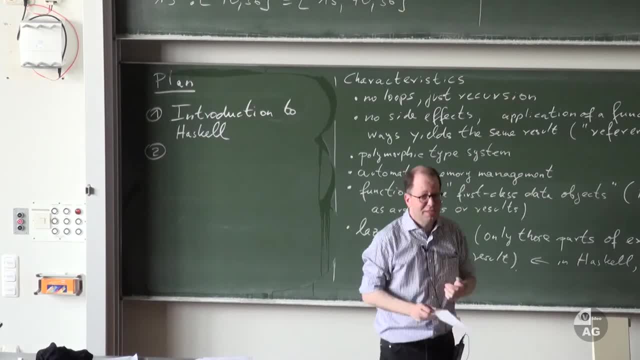 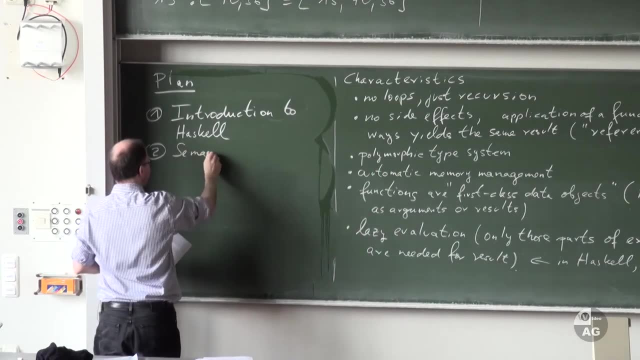 So if you, for example, write down a program like this, what does that mean? How does this execute? And to define this formally, one has to define the semantics. So you have to define the semantics of your language In particular. this has to be fixed. 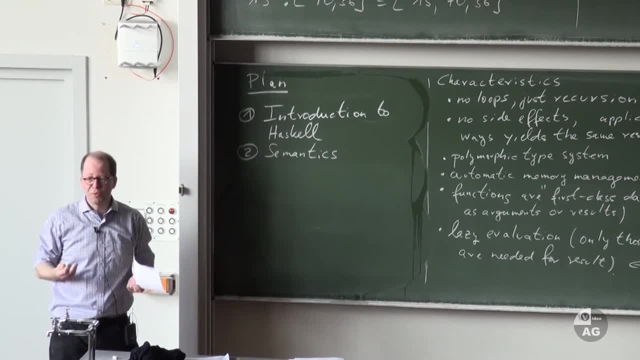 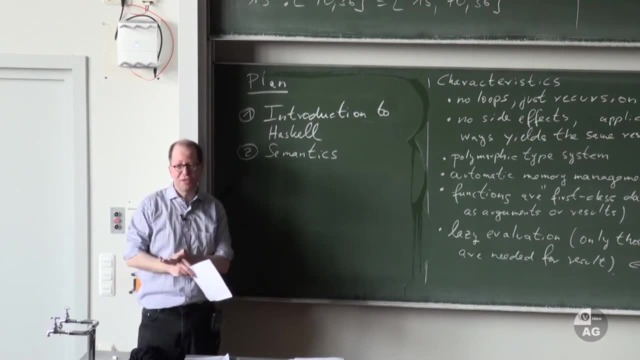 if you want to write a compiler, I mean the compiler- not every compiler- should do what it wants, but they should all do the same thing. I mean the meaning of the program should be well defined and it should do the same thing, no matter which compiler you 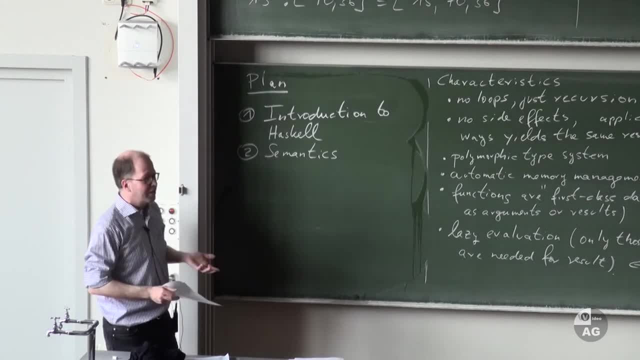 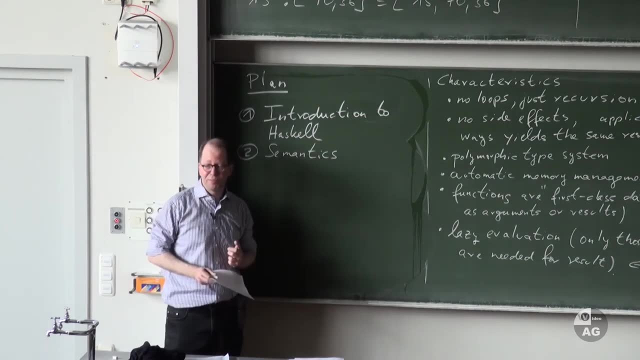 use, or no matter which computer you run it on. And so the question is: how can one define the semantics of programming languages in a precise way? And well, for functional languages this is rather nicely possible. This is much easier than for imperative languages. 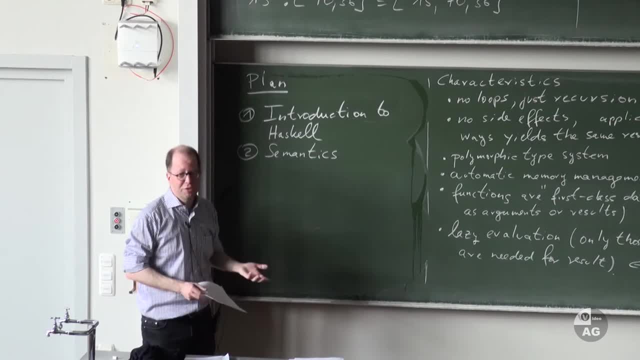 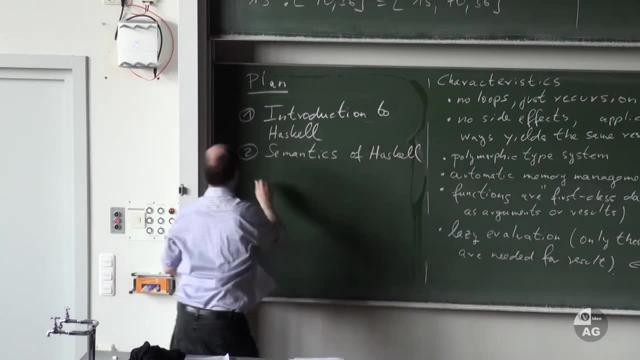 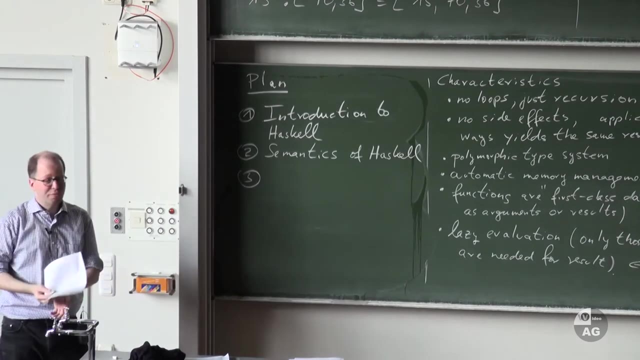 And so we will define the semantics of functional programming languages. and we do this for Haskell, So we will define the semantics of Haskell. And then- the third part- we will think about how to implement functional languages. So, if you really want to write an interpreter or a compiler, 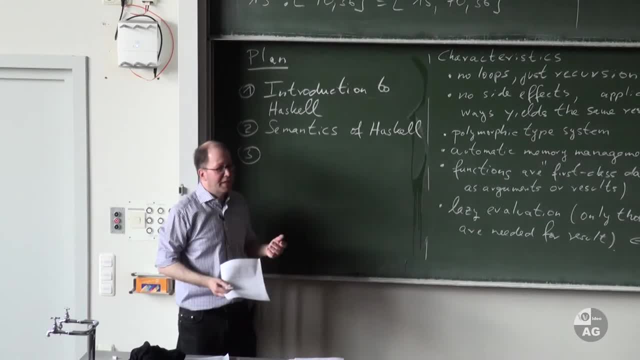 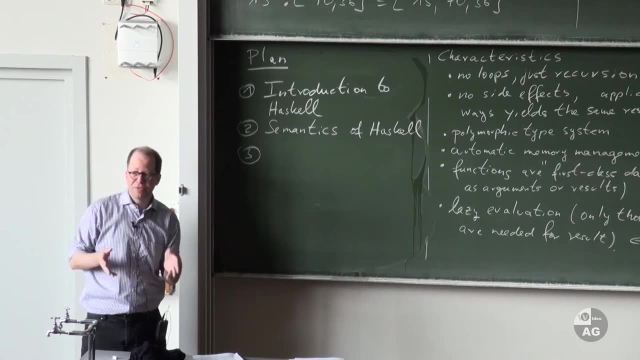 for a functional language. how would you do this? And well, there are several ways to do this, And what we will do is we will reduce Haskell to a subset of Haskell, to a very small subset, very easy subset, which is called the lambda calculus. 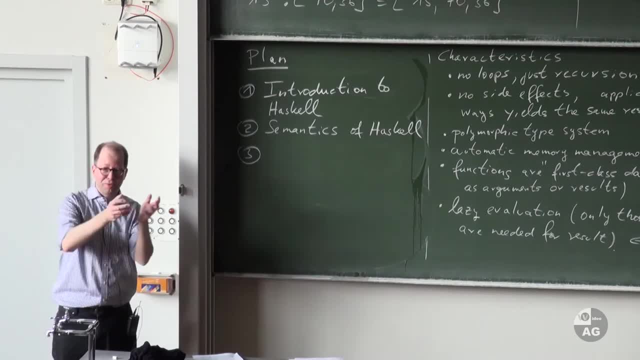 And to implement this is trivial, And so our implementation works in the following way: First Haskell programs are automatically compiled to this kind of machine language, to the lambda calculus, And then this machine program, this lambda calculus program, can be executed. 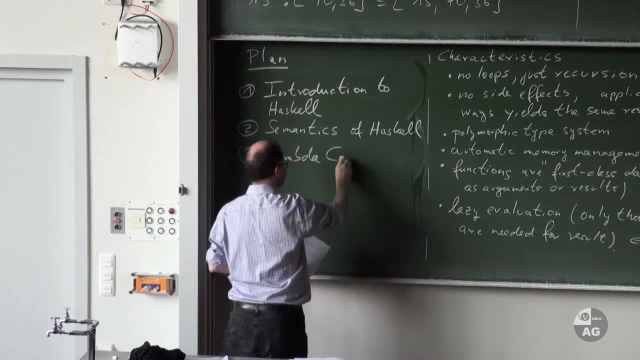 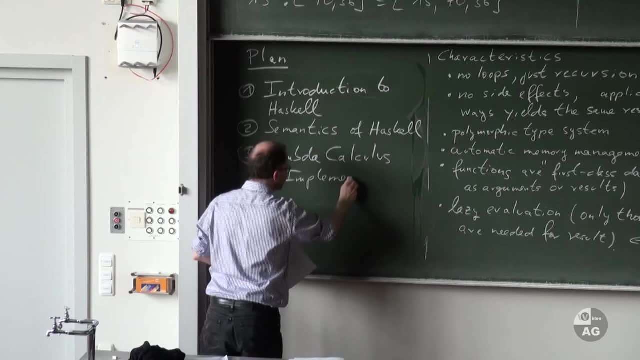 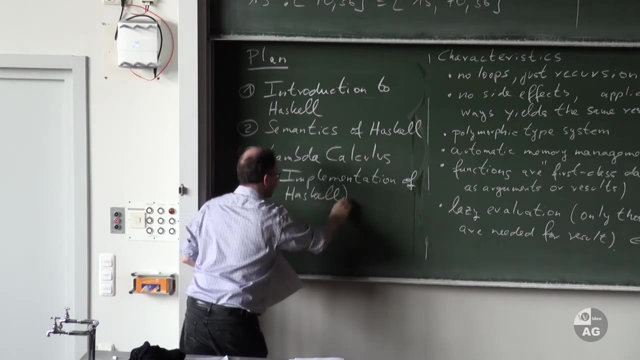 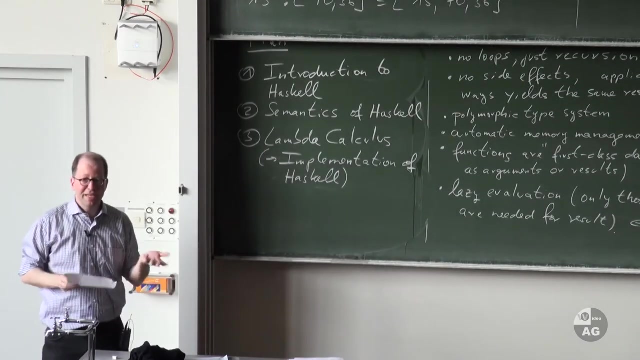 So we will look at the lambda calculus. One purpose of this is a possible implementation of Haskell, But this only executes the program. It does not type check the program And of course, as you know from all typed languages, whenever you want to compile your program. 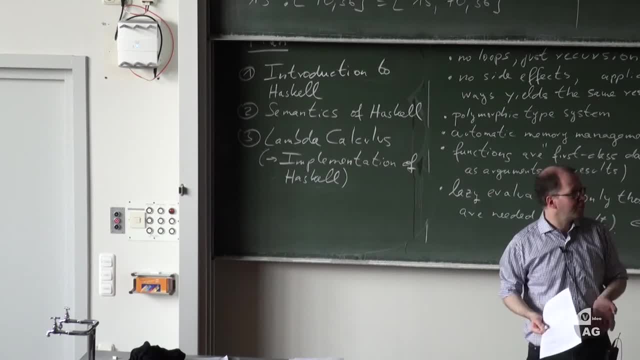 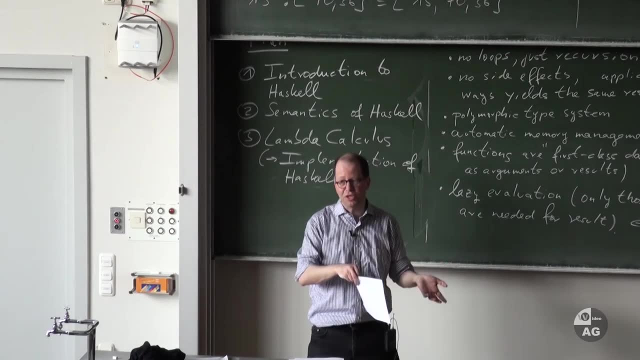 the first thing that happens is the program is type checked. And well, this happens in Java and this happens in Haskell as well. So first one checks: Is this program well typed? Are functions always applied to arguments of the correct type? 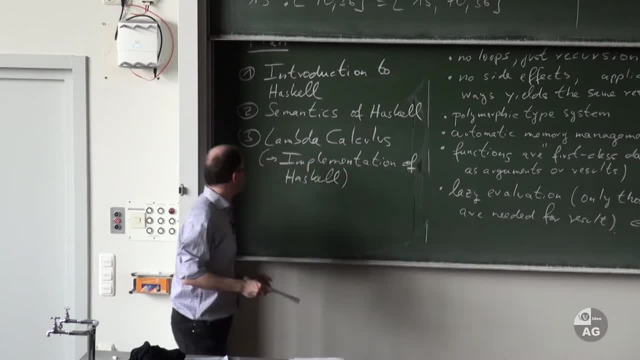 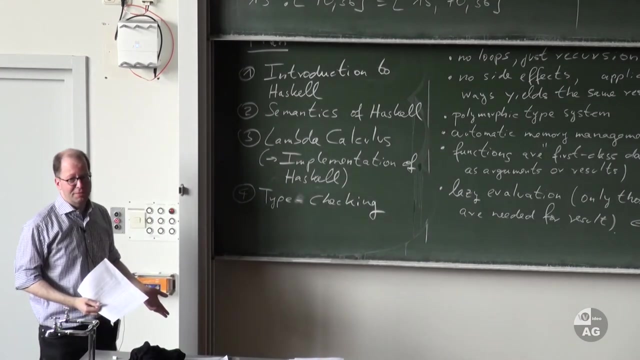 And of course, this can be done automatically. And how this can be done automatically, that's the topic of the fourth and last chapter. So this is how to do type checking automatically, And this is not entirely trivial because we have the polymorphic type system. 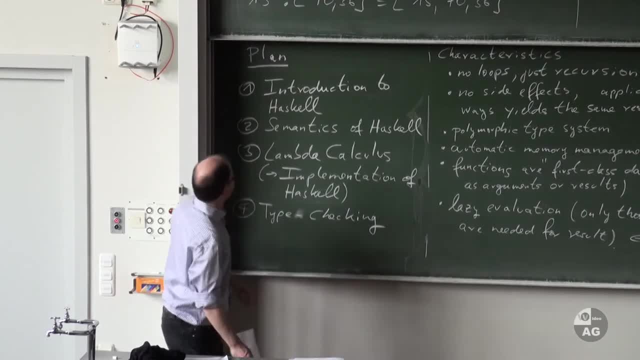 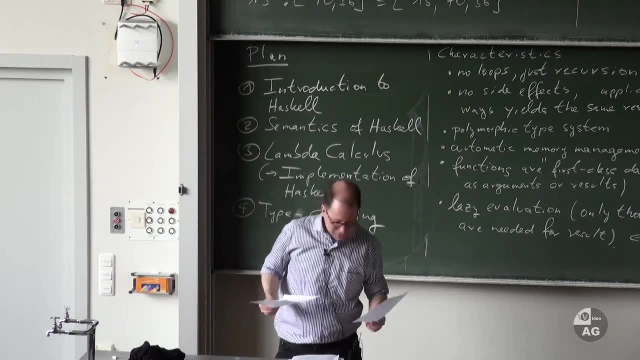 And so how to do this automatically we will learn there. So that's the plan for the lecture, And now I have to go. I hope I made you interested in the whole thing, And I will now say something about the organizational details. 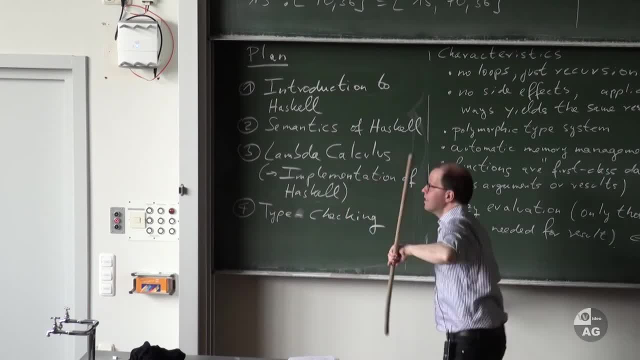 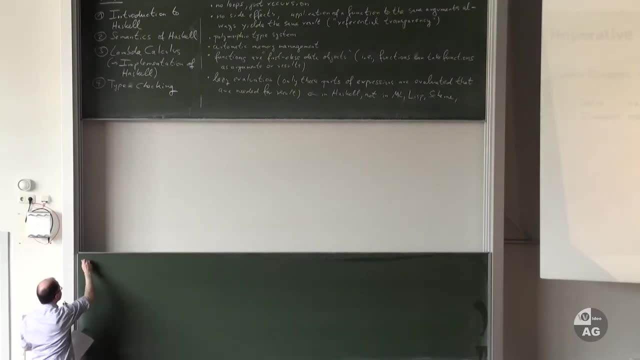 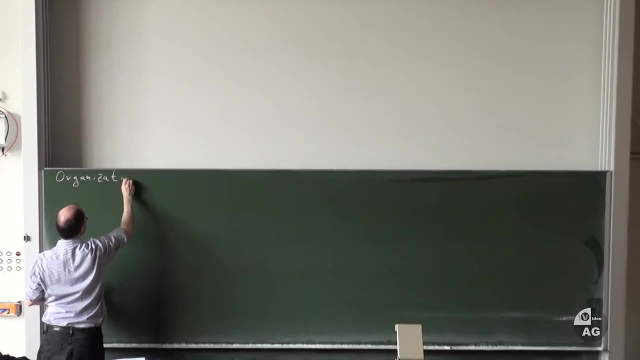 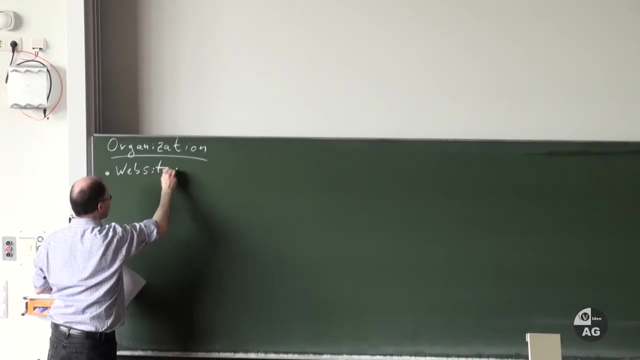 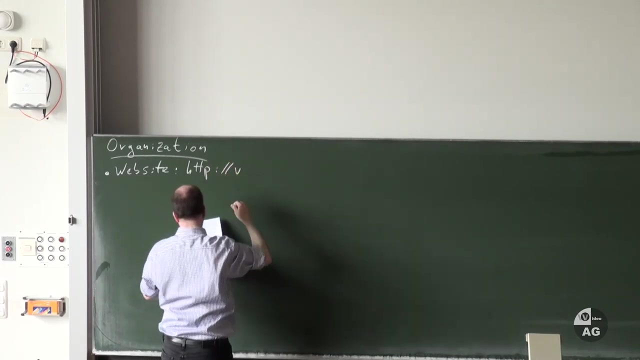 But before I do that, I will wipe the board And then I'll tell you about the organizational stuff. OK, so something about the organization. Organization. So there's a website for the lecture, And the website is the following: http//verifyrwthachende. 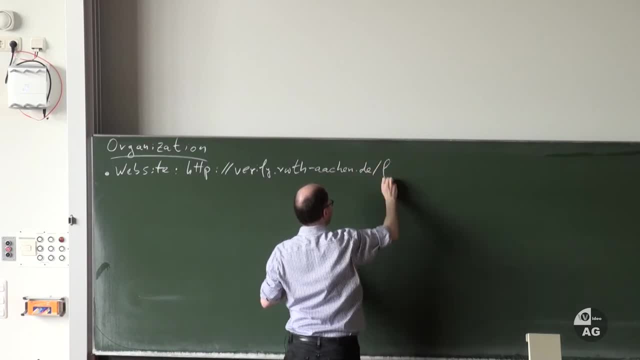 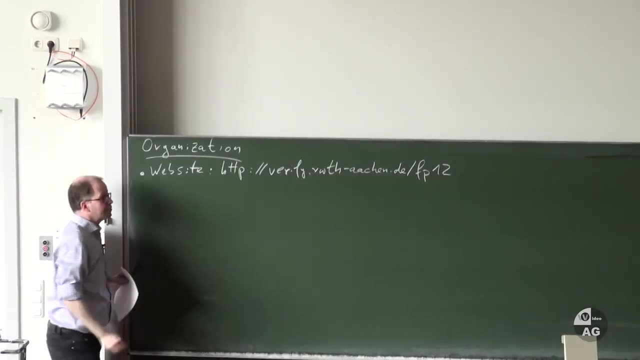 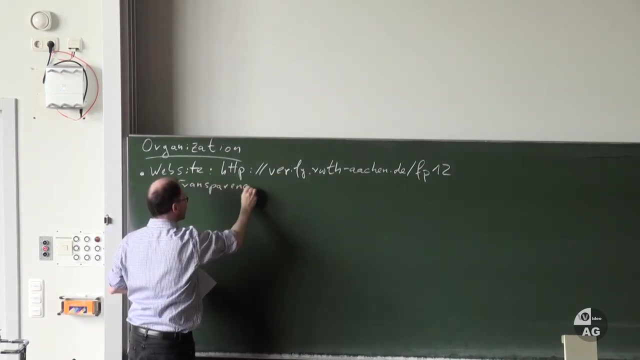 FP 12 for functional programming 2012.. And on this website, what can you see there? All the transparencies that I put up in the lecture can be found there, So there's no need to copy these transparencies. 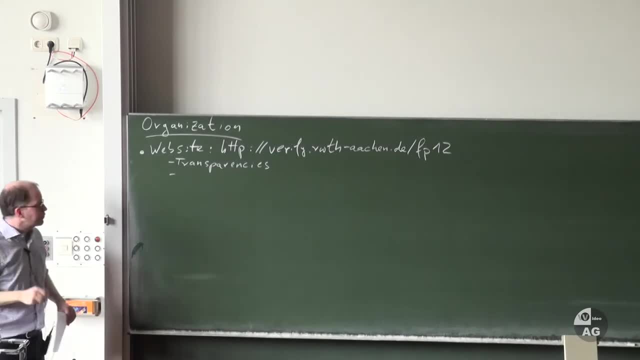 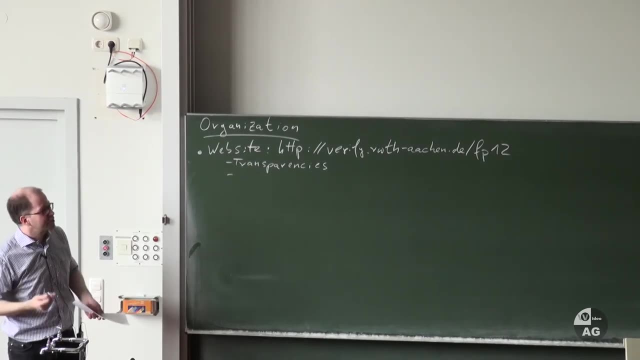 You can download them from the website And I will try to put them there in time before the lecture. So the transparencies that I put up in the lecture should be there at least the day before So you can download them and print them if you want before. 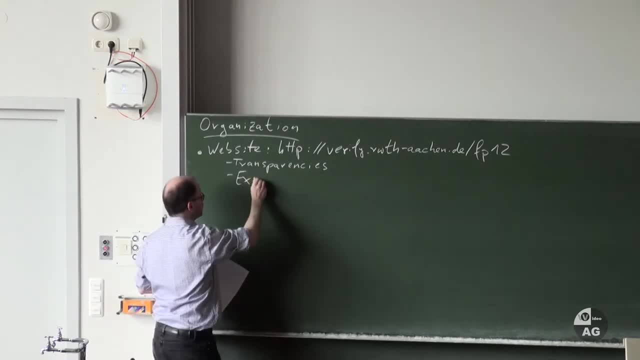 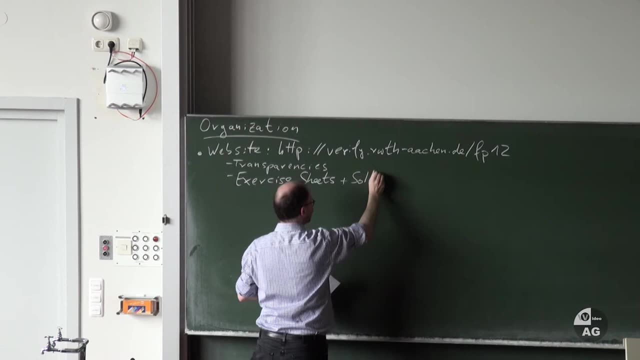 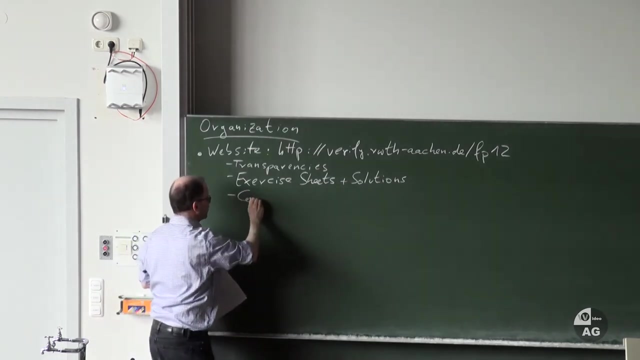 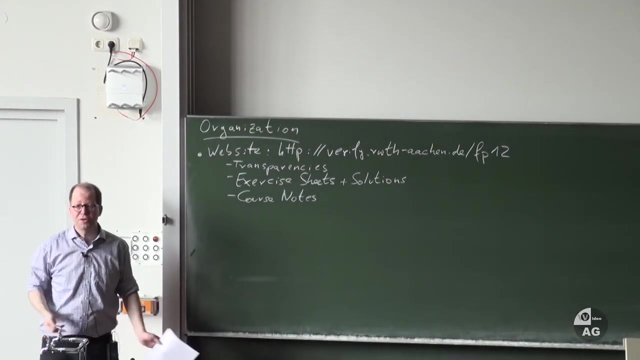 Then the exercise sheets. The exercise sheets will be there And later on also the solutions for the exercise sheets, Then the course notes. So there are course notes for this course And also the course is in English, But the course notes are in German. 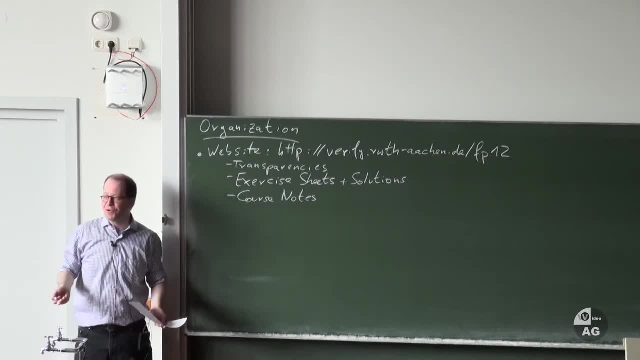 So there's something for everyone. So, for those of you who are English speaking and not German speaking, you can benefit from the course, But you can polish your German by reading the course notes, And vice versa For those of you who are German. 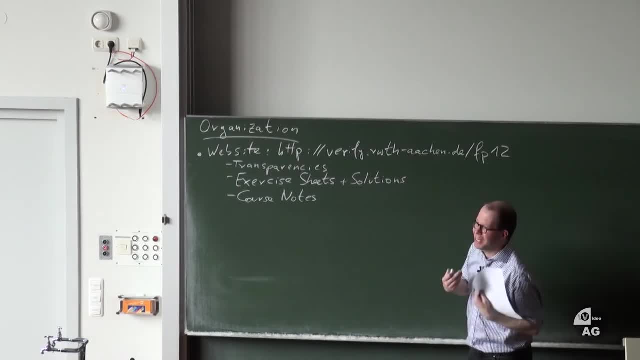 you can polish your English. Well, OK, polish. You can listen to my English, which is not, And you can read the German course notes. So, anyway, the course notes are in German, But of course the programs look just the same. 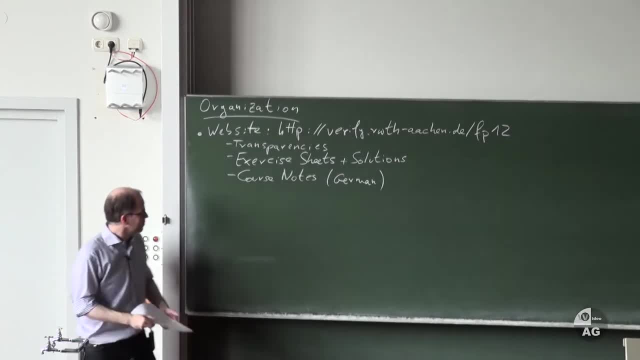 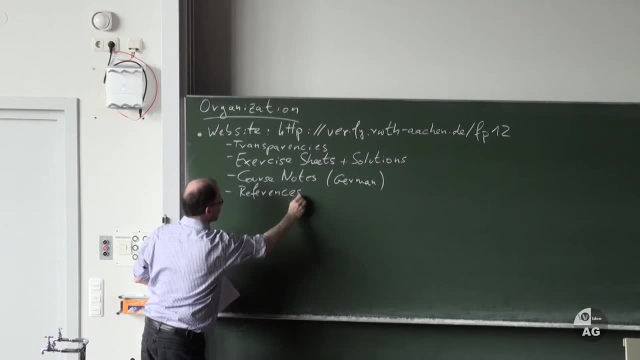 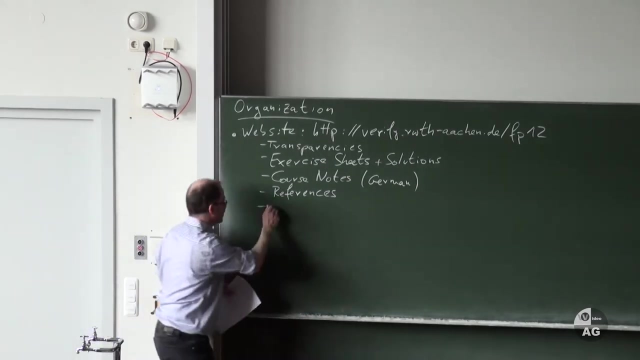 So programs, formulas, stuff like this are pretty international, And references and all these things can be found there, Details about software and so on, And also announcements. So announcements, that's maybe the most important thing. So dot dot dot. 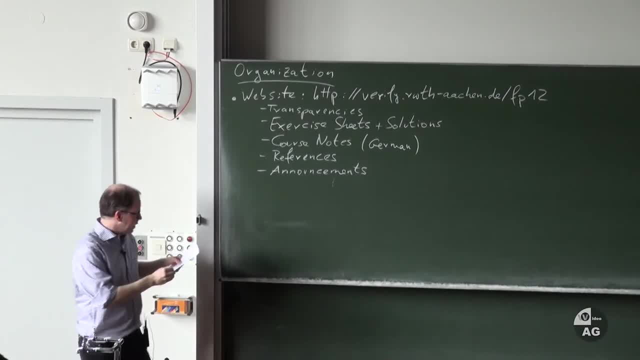 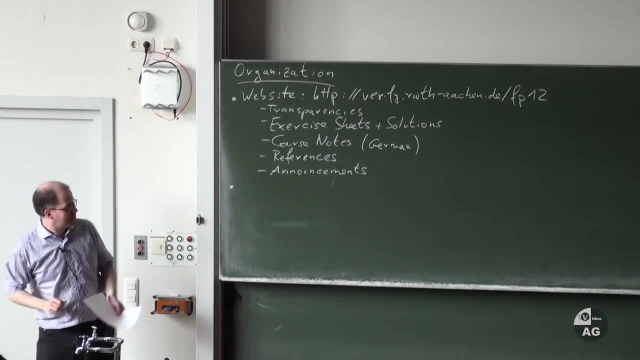 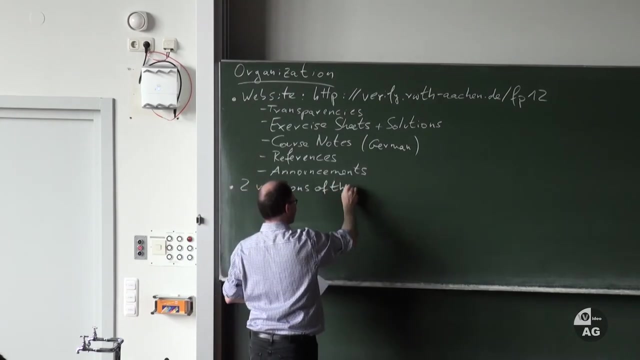 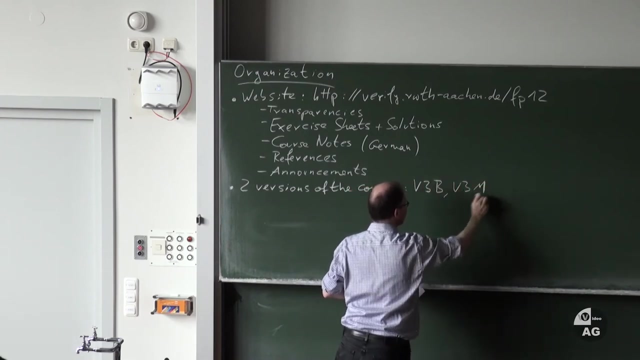 So this is the website for the course. Now, the course is a course which comes in two versions: A bachelor version and a master version. So there are two versions of the course, And I call them V3B and V3M. V3, V means Vorlesung lecture. 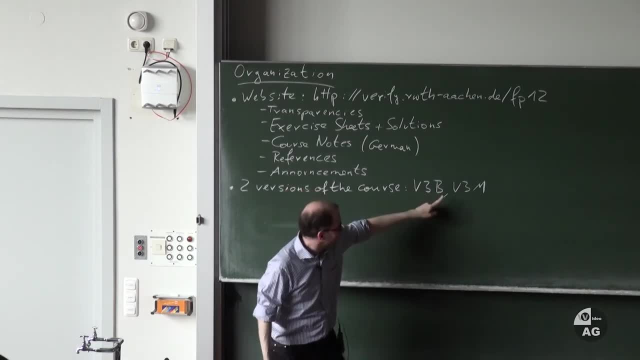 Three means three And B means bachelor And this means master. So this is the bachelor version of the course, This is the master version of the course. Both of them have, on average, three lecture hours per week And they are not disjoint. 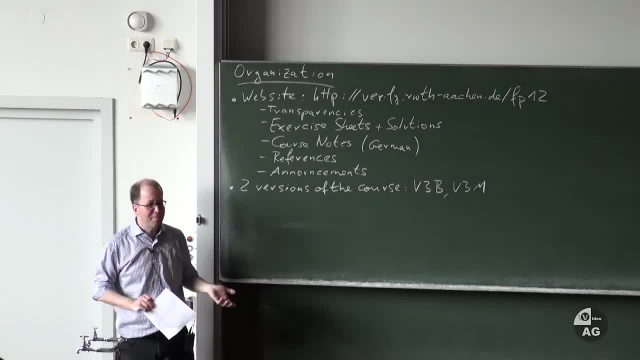 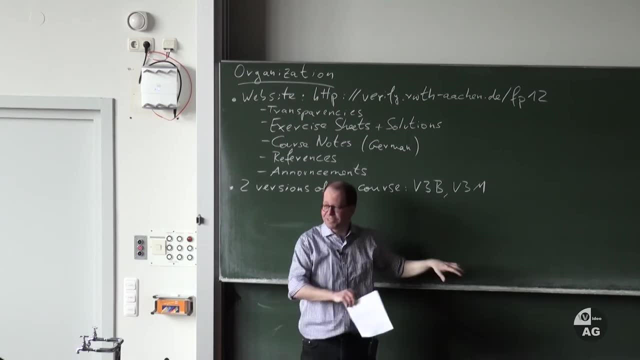 Not at all, But they are not completely identical. So there are some parts of the lecture which are only for bachelor students And some parts which are only for master students, Only in the sense that they are not secret. So I mean, the other students are welcome to attend. 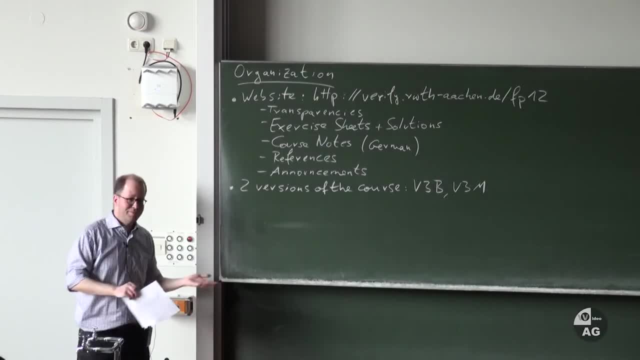 But they will not be part of the bachelor exam And well, the other parts will not be part of the master exam. So the union of this thing is a V4 lecture. That's why we have two. we have two times two hours per week. 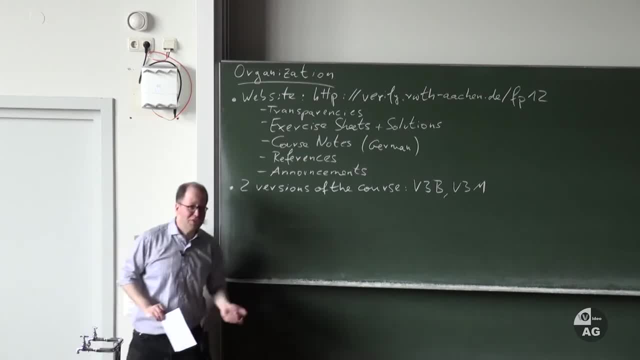 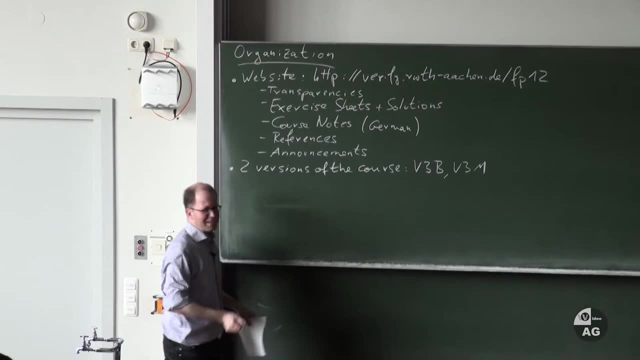 But that means that some lectures are not mandatory for the bachelor students And some lectures are not mandatory for the master students. Okay, so I don't write this down, So I hope you understood. And who attends which course. So V3B is for bachelor informatic. 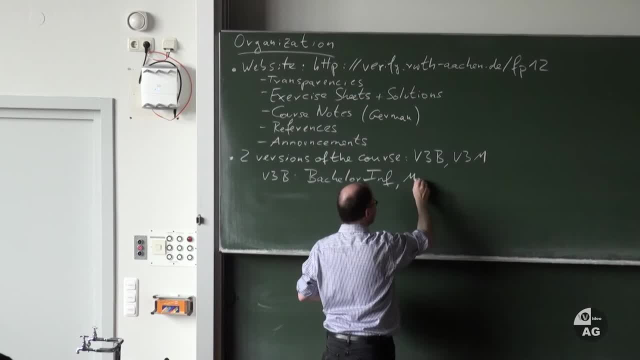 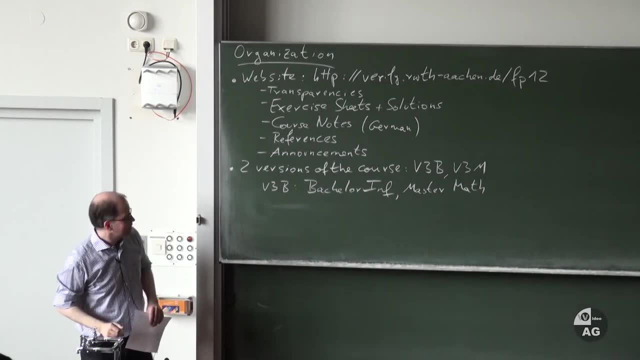 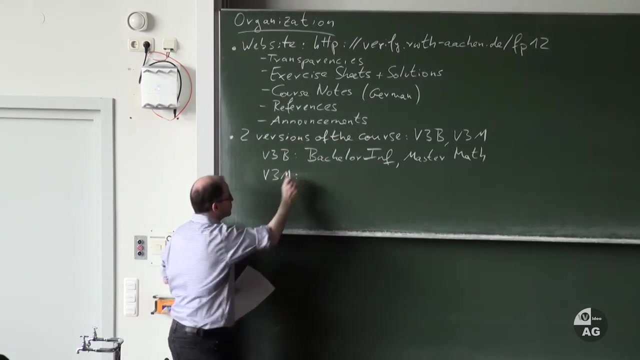 As you would have expected, And for master mathematics. So for some unclear reason, the master students in mathematics are. they attend the bachelor courses. I don't know why, but this is written in the regulations And the V3M course is for. 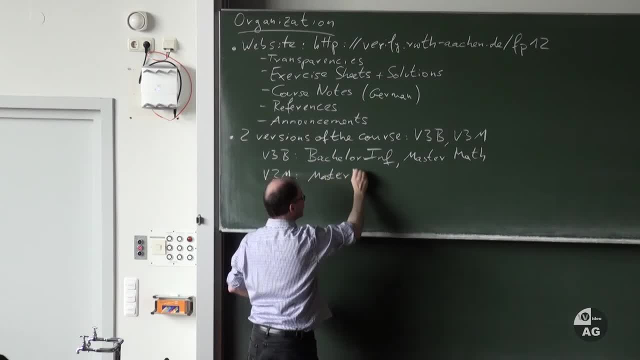 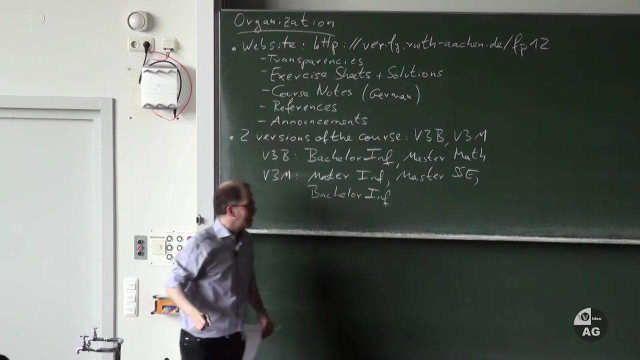 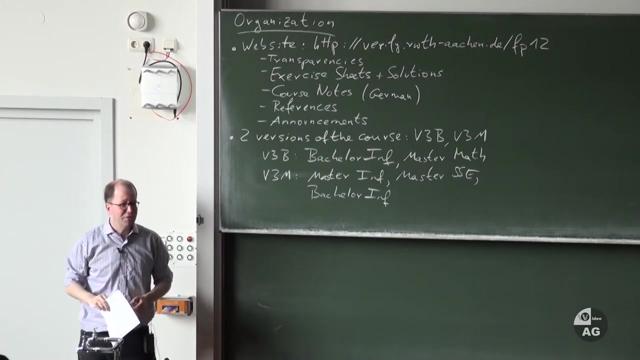 master informatic, Master informatic master, software systems engineering And also for bachelor informatic. in case you want to take this course, as if you study bachelor computer science and you are in the last semesters of your bachelor, you can already do master exams. 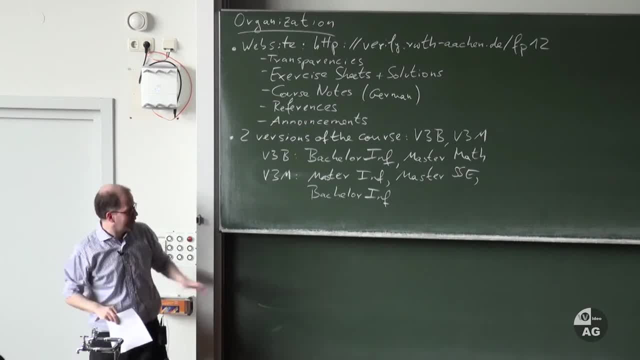 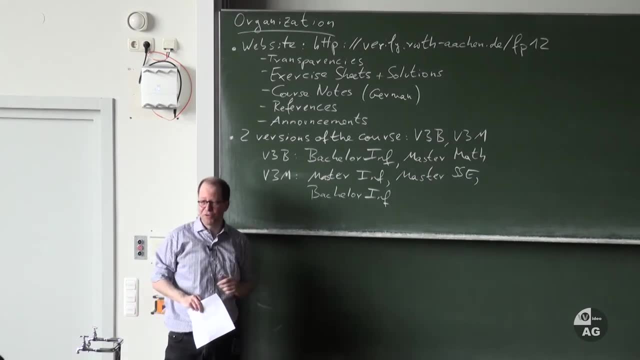 And so you can also decide: well, I don't want to take this course for my bachelor, I want to take this course for my master, That's fine. So this will then count for your master, but then, of course, you have to attend the V3M version. 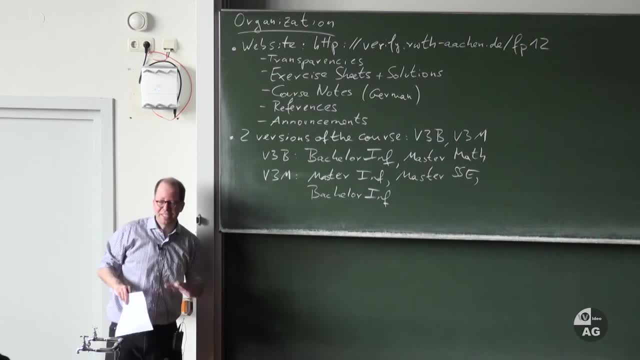 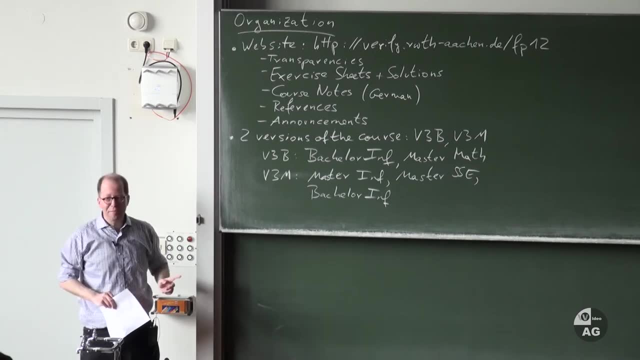 instead of the V3B version. So these two versions are not that different. but well, there are some details which are in here and not in there, and vice versa. Is there anybody studying in a program not listed here? Okay, Yeah, okay, so you can probably come to me later and we can discuss. 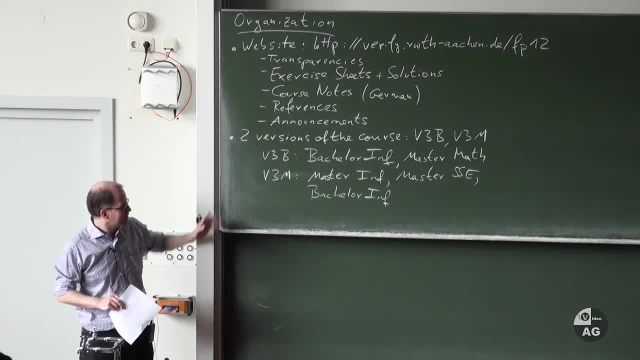 which version is appropriate for you. Anyway, so this is. the differences are minor, but so there will be some exercises on the exercise sheets where we will say this is only for V3B students or only for V3M students, And I will also. 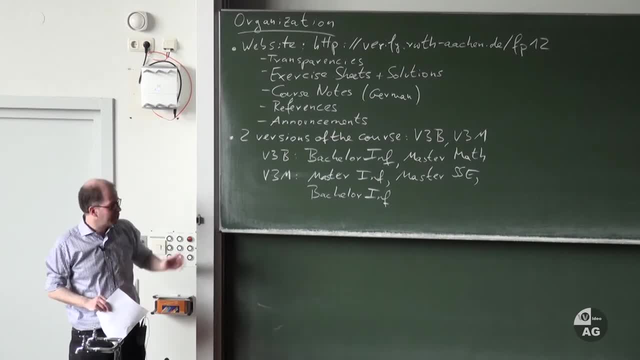 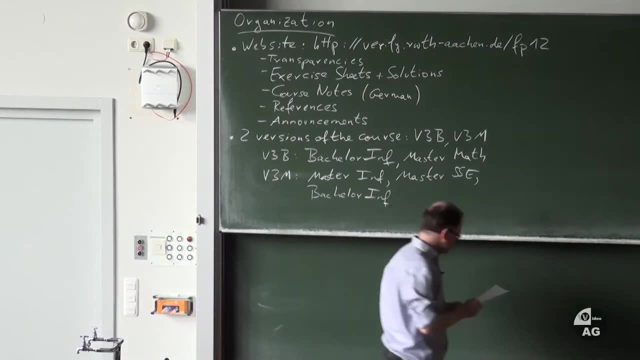 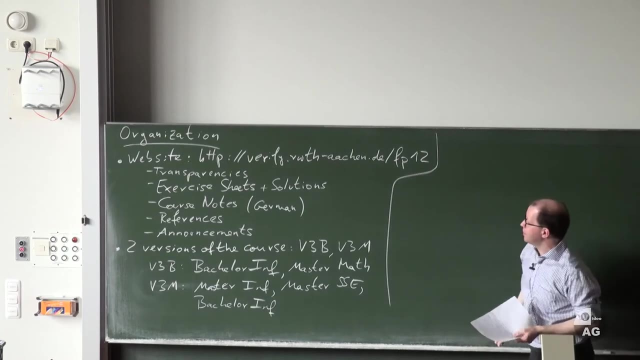 announce in the lecture which parts are just for one of these courses, And we will also write this on the website, of course. Okay, so Now what about the exercises? So, on average, there will be an exercise course every week on Wednesdays. 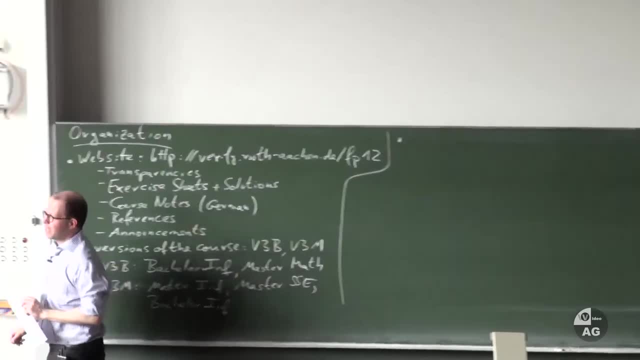 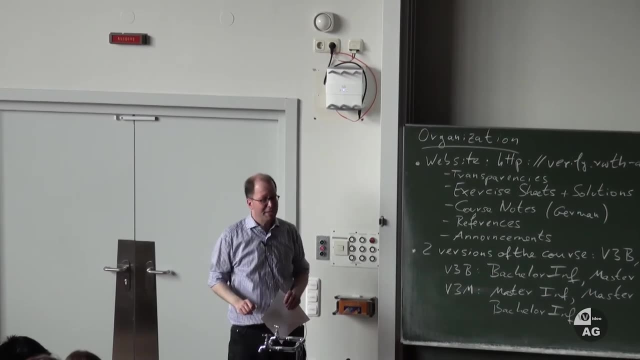 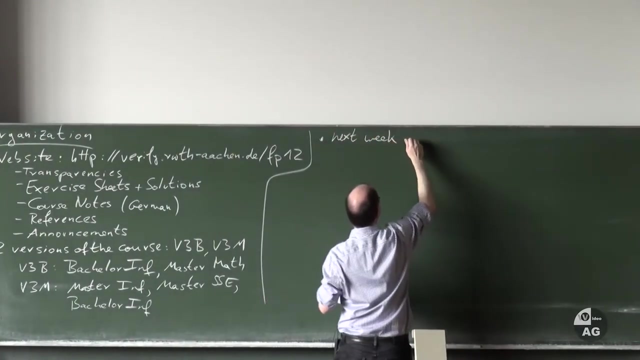 but since we had to- I mean, there were no lectures in the last week and only this lecture in this week due to all the holidays- And so next week instead of the exercise course I will do a lecture. So next week we will have three lectures. 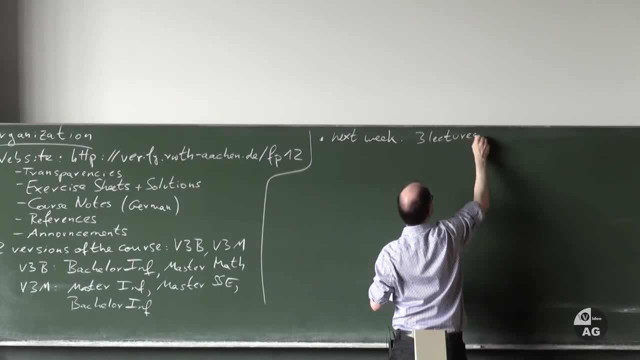 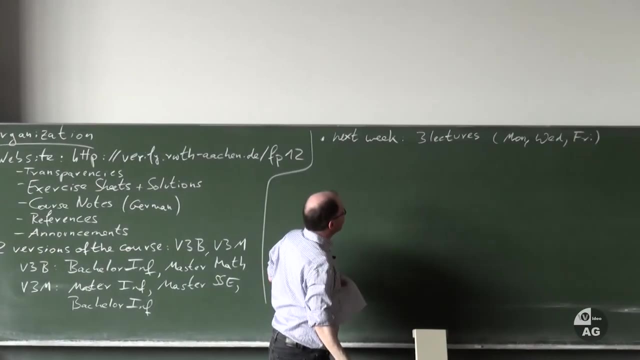 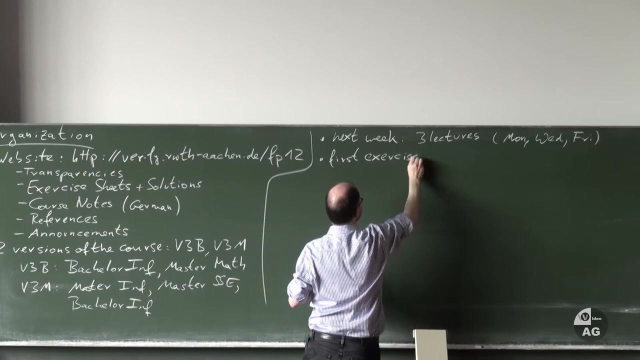 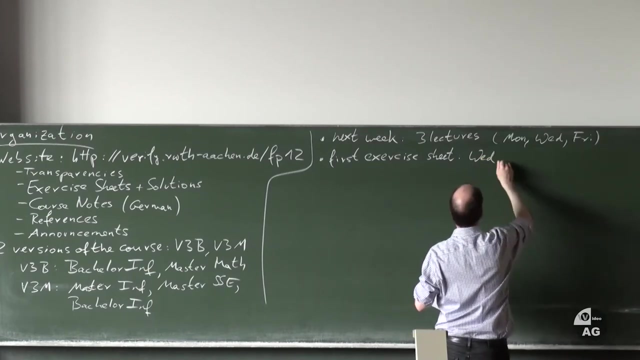 on Monday, Wednesday and Friday. So Monday, Wednesday and Friday. So instead of exercise course I will do lecture next week Because there is not yet too much to exercise And the first exercise sheet will be distributed next Wednesday. So this will be on Wednesday. 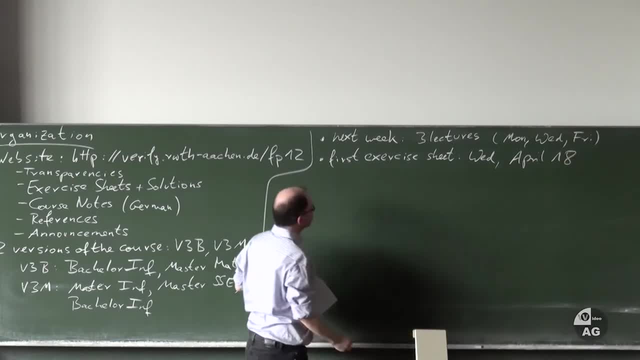 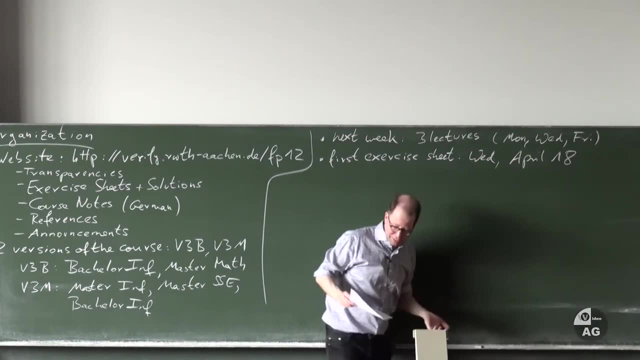 April 18.. And this will be so. there will be an exception next week: We will do lecture instead of exercise, And in the week after there will also be an exception because we switch between exercise and lecture, because I am not here on Monday, but I am here on 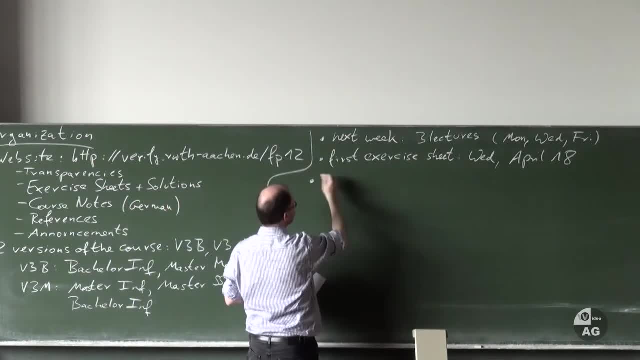 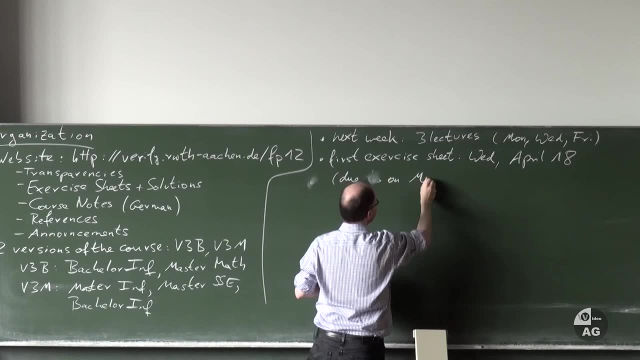 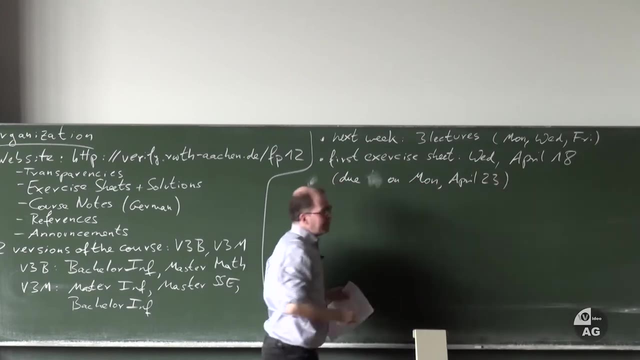 Wednesday. So this thing will be. this will be a small exercise sheet and it will be due on on Monday, April. what is this? April 23, I think, But normally the exercise sheets will be distributed on Monday and you will have time until Wednesday the week after. 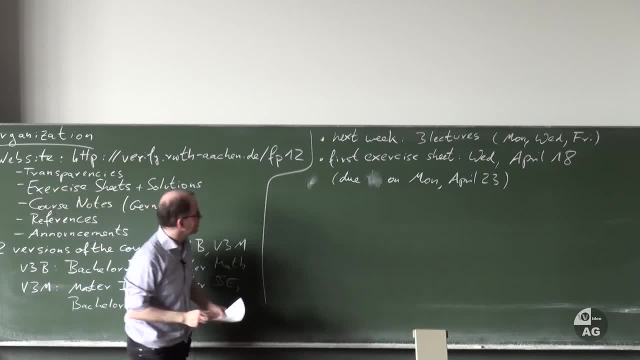 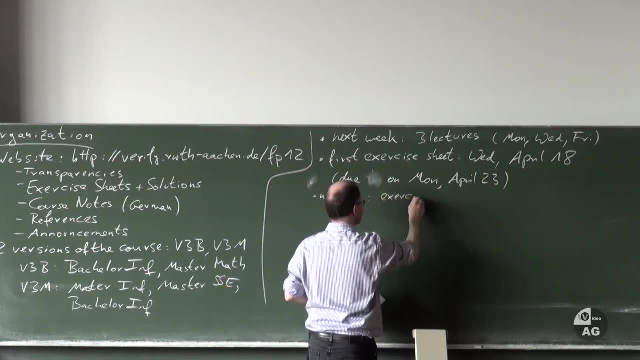 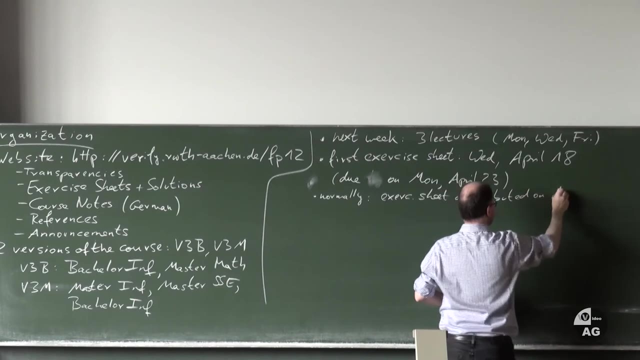 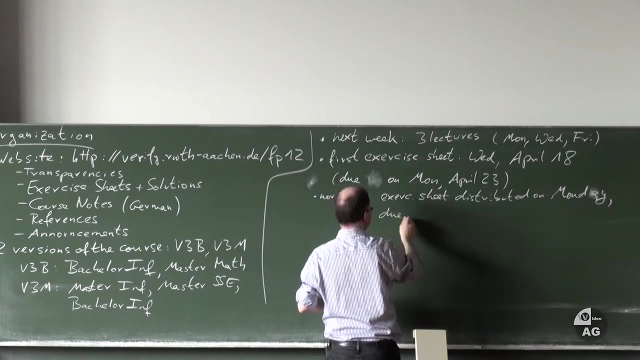 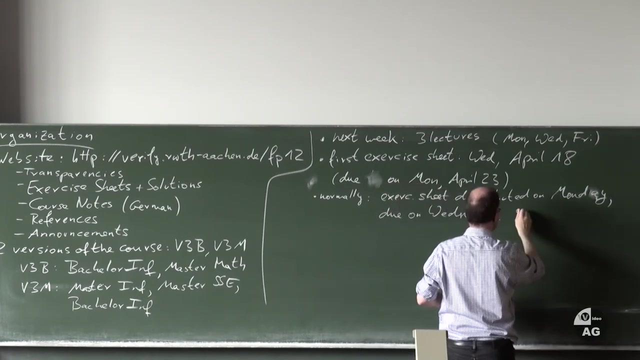 to work on it. So you will have a little bit more than one week for the exercise sheets. So normally, normally means after that exercise sheet will be distributed on Monday and Monday and it will be due in the exercise course on Wednesday, Wednesday, nine days after. 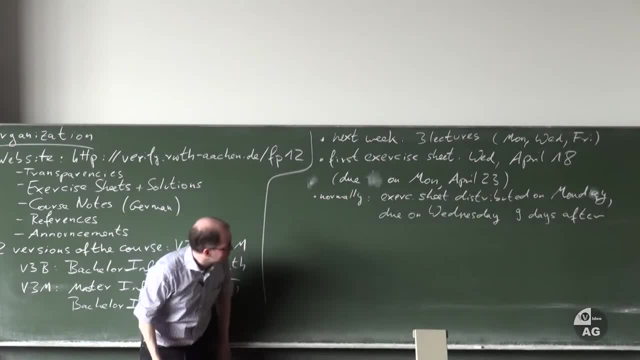 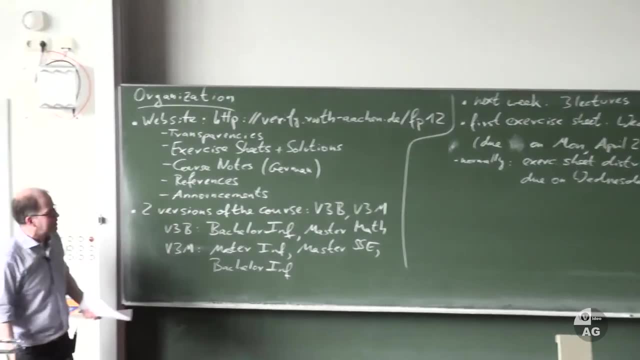 So in the beginning we start a bit irregular, but then later on, this should be the idea. And these exercise sheets: well, on these exercise sheets, there will be some exercises accompanying the lecture and you should work on them and hand them in and they will be graded. 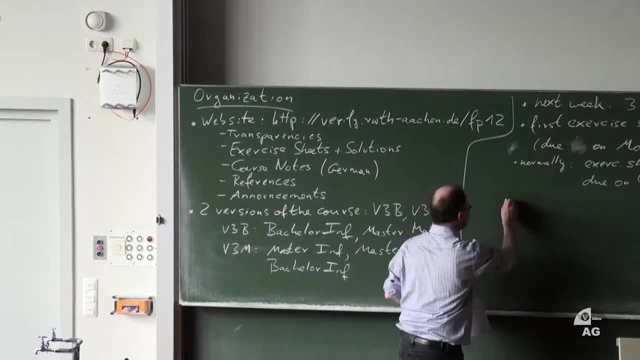 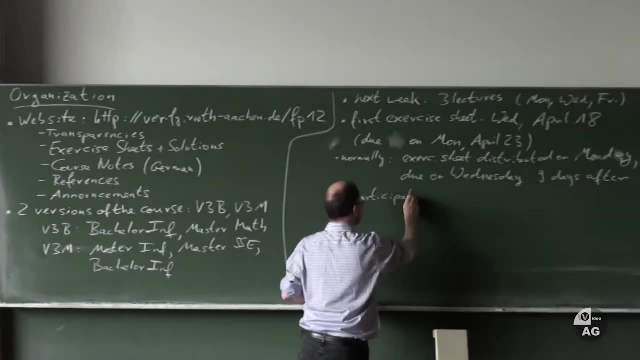 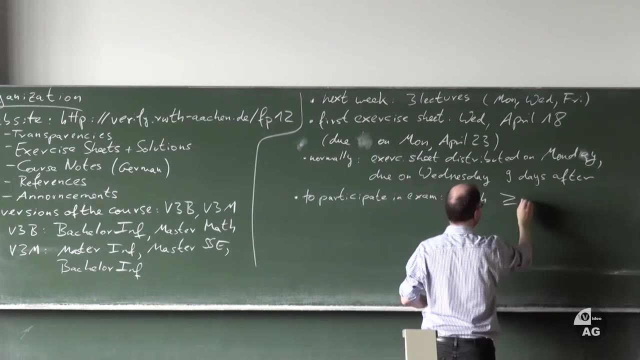 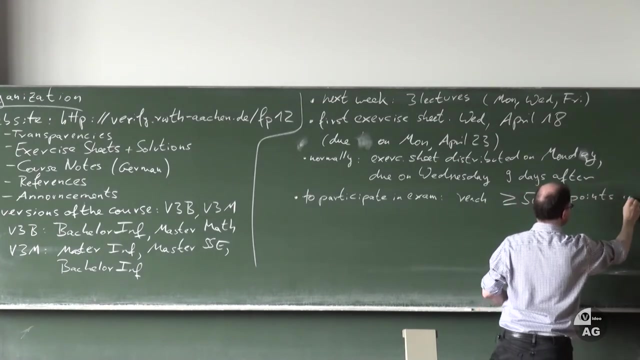 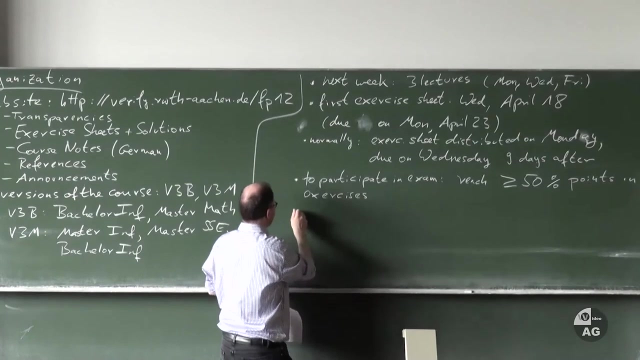 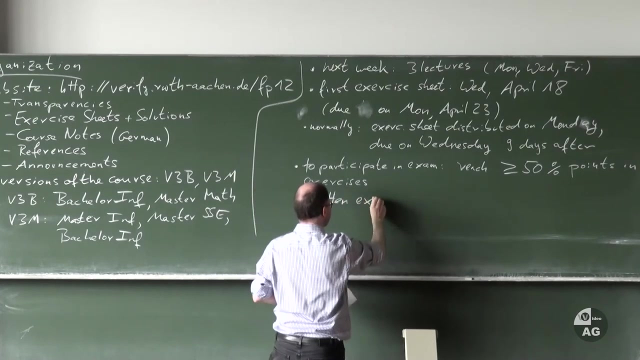 and you should reach as many points as possible. but to participate in the exam in the end, to participate in the exam, you should reach at least fifty percent of the points in the exercises in the exercises and the final exam will be a written exam. so there will be a written exam. 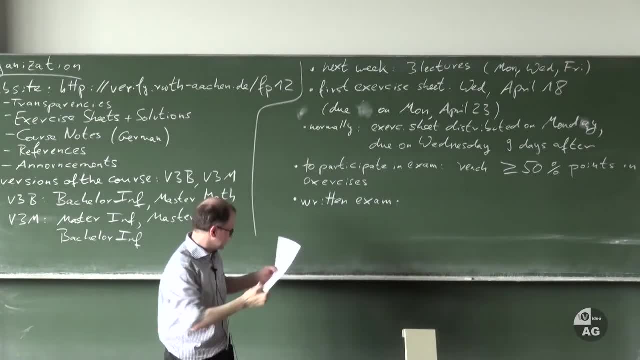 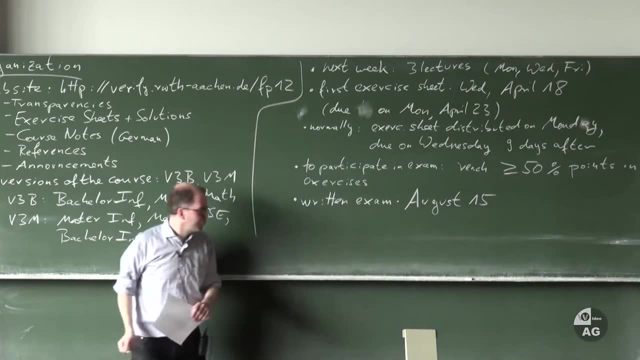 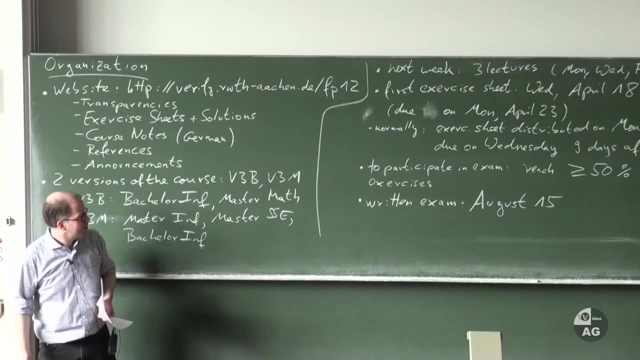 and the exam will be on August, August fifteen. on August fifteen, and for those of you who failed the exam, there will be another exam in September, but I didn't look up the date. if you look into campus you can find out, but I don't have it here. 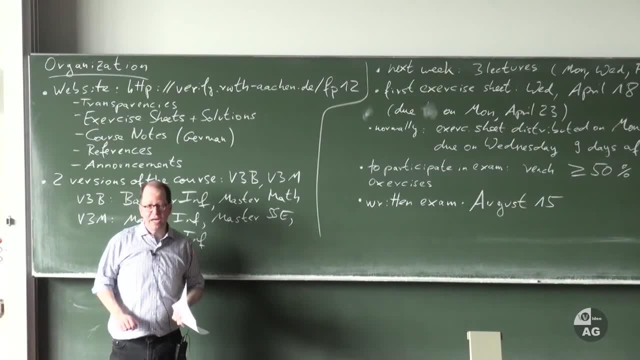 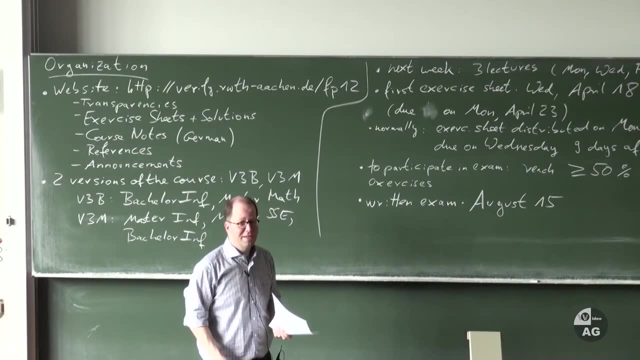 okay now. several people already asked me: where do I have to register? Yes, this is the cycle. are there maybe two weeks exercise, or are there from Monday to next Wednesday where you have time to do both? so the exercises are every week. so it's like this. so 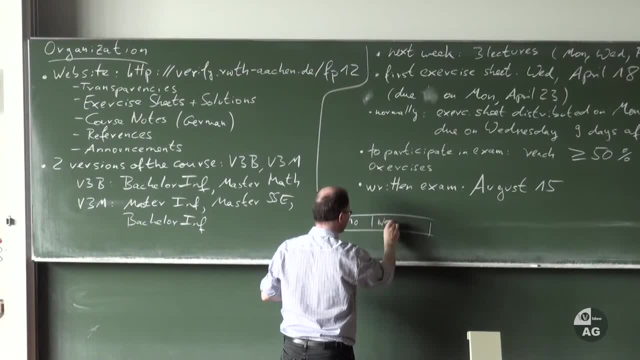 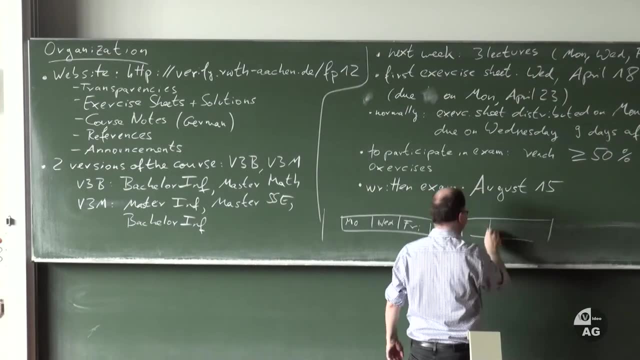 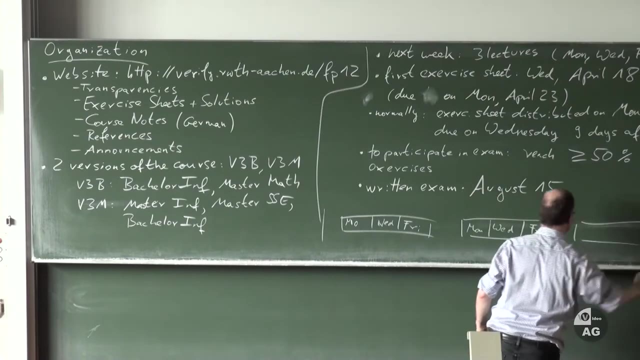 let's say this is the week here. we have Monday, then we have Wednesday, then we have Friday. these are the important days of the week, because these are the days where you have functional programming, and so the idea is: and it continues like this. so here you get the exercise. 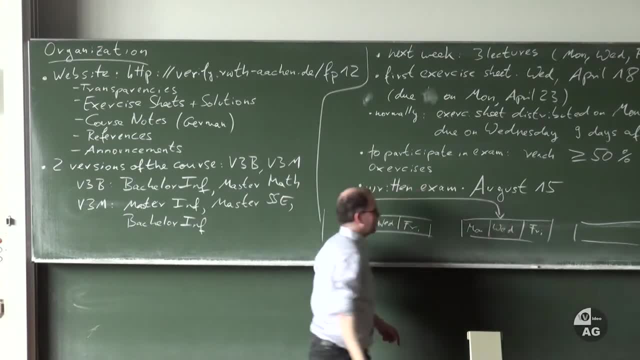 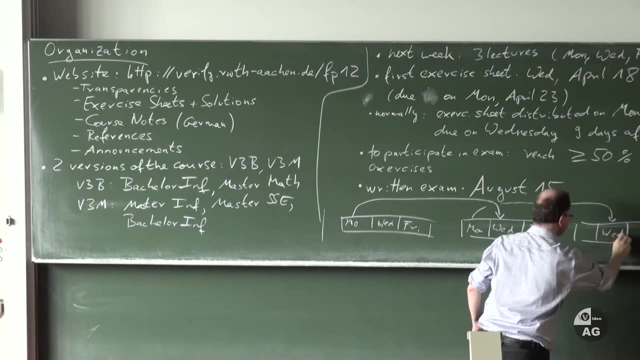 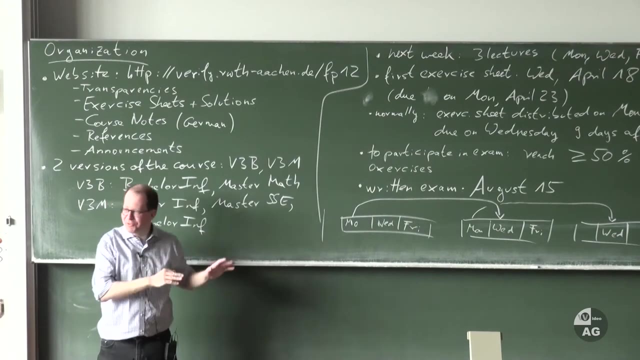 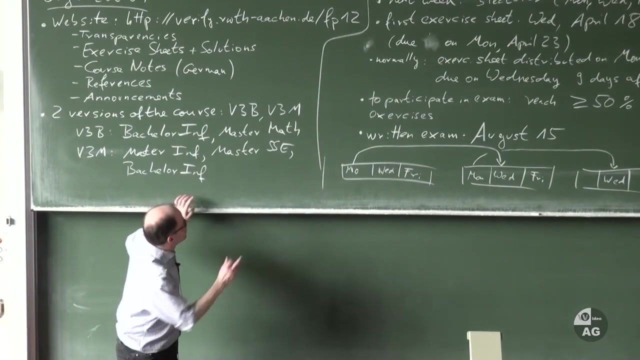 sheet and then you work on it and return it here, and here you get the next exercise sheet and you work on it and you return it here. so that's the idea, okay, yeah, okay, so maybe we should write a program in Haskell to compute this, okay, okay. one more thing, because many people 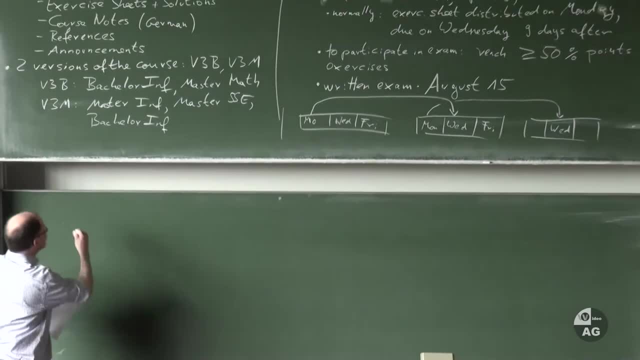 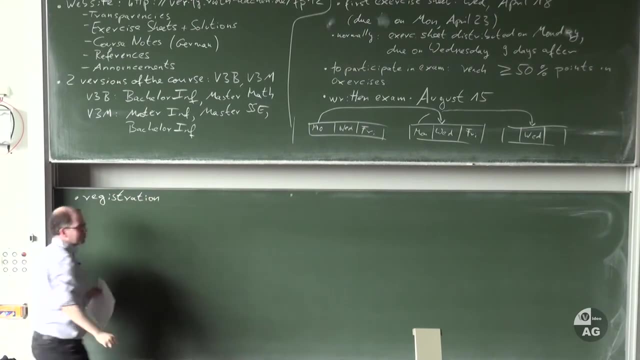 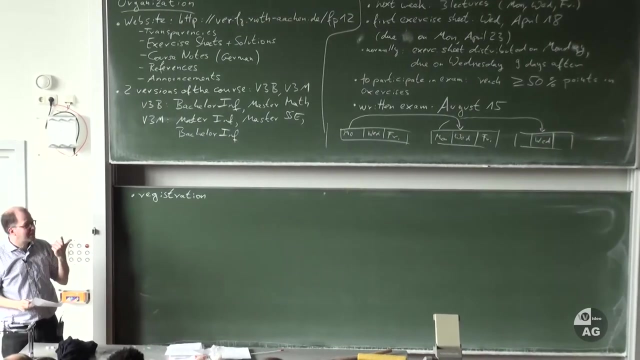 ask me: where do I have to register? and okay, you have to register, so registration. so there are two forms of registration needed. so I mean there are three things that we do. we do have lecture, we have exercise, we have exam. so for the lecture you don't have to. 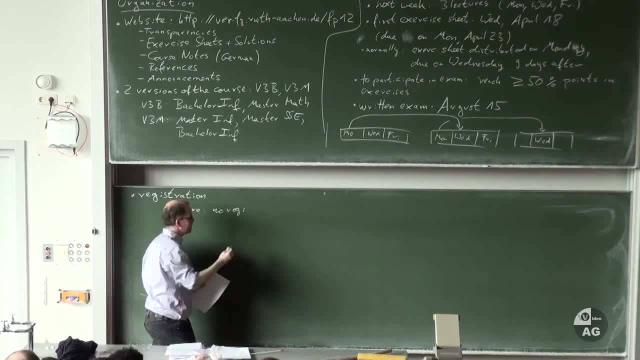 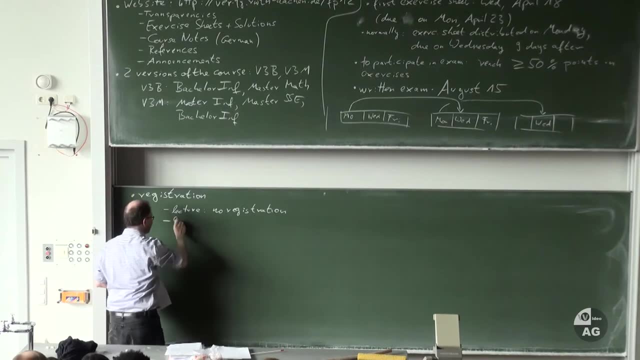 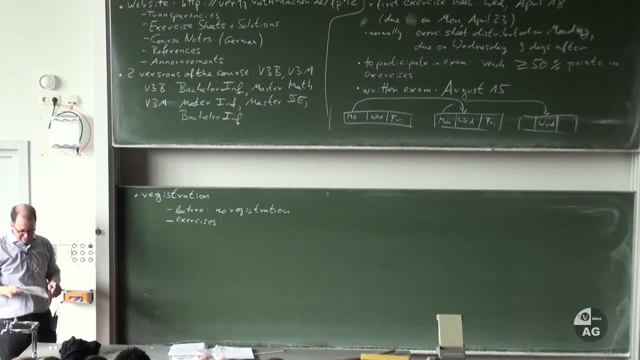 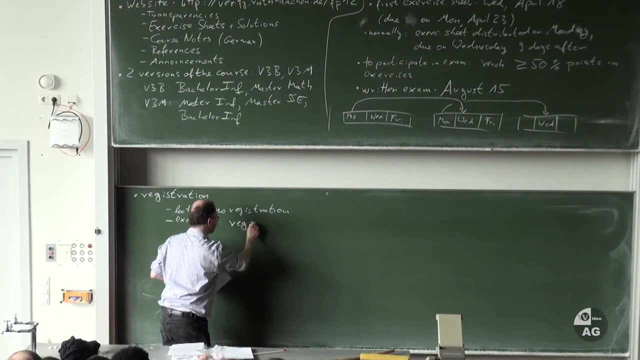 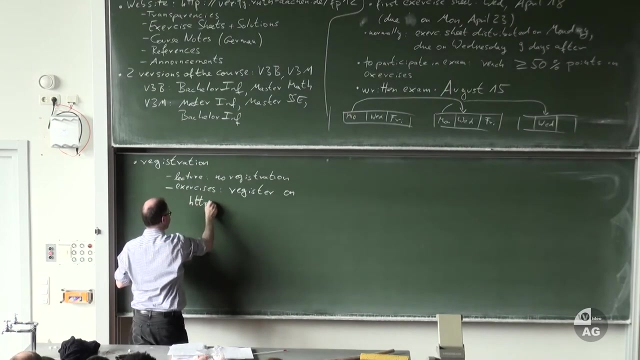 register, no registration, just sit here and enjoy. so no registration for the lecture. to participate in the exercises, you have to register, because we have to put your name into our database and to do this, you can register on the following website. the following website: https. so this is even secure. 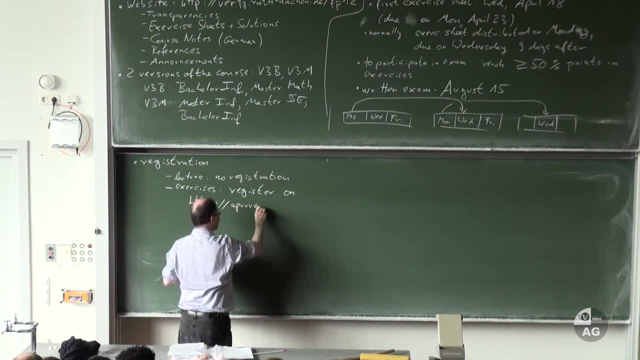 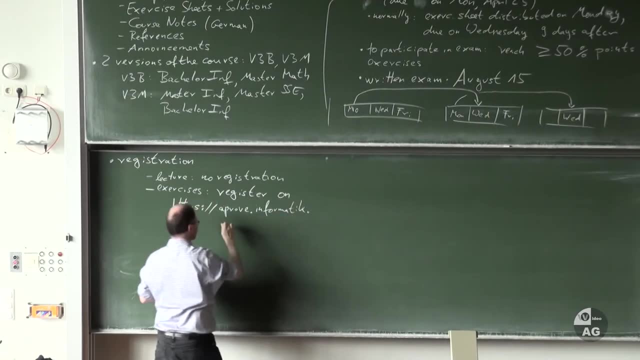 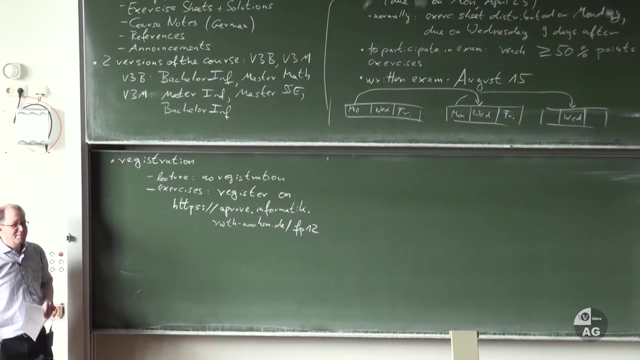 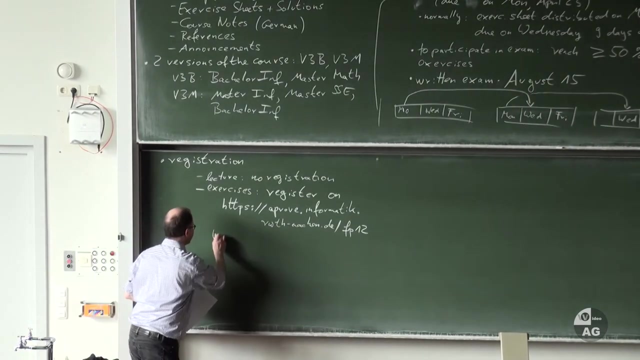 ah, a proof with one P only: informatic RWTH Aachen. RWTH Aachen DE FP 12. so if you go to this website you will be able to register for the exams, for the exercises, and please do that until next Wednesday, so that we know. 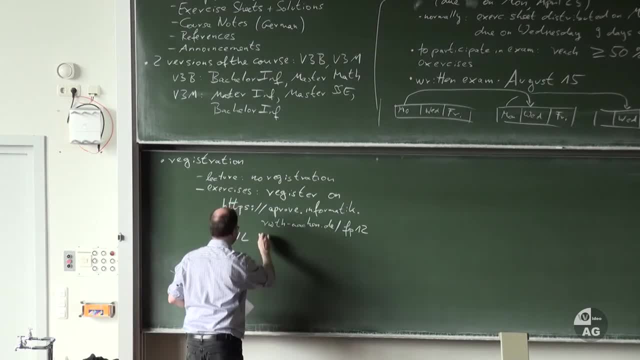 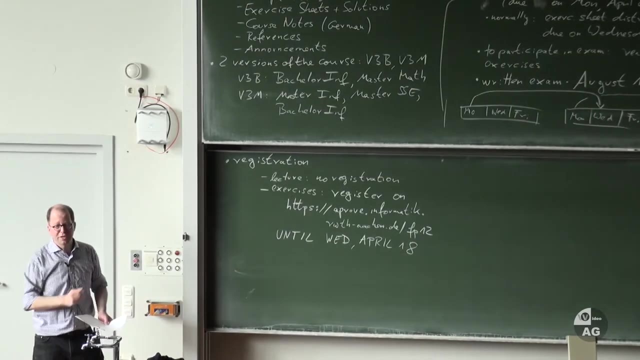 how many students participate here. so until Wednesday, April 18. so this just means that we have your name in our database and then we will collect the points you reached in the exercises, and you can also look into the database again and see how many points you've reached. 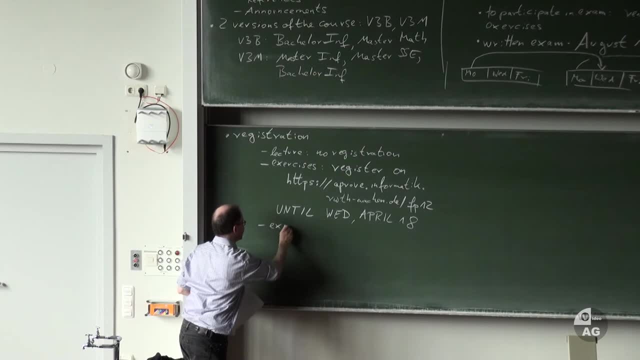 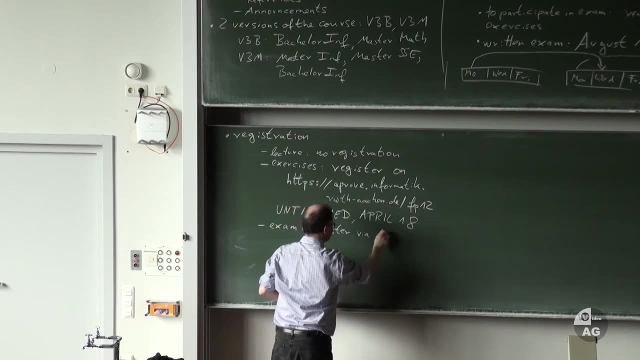 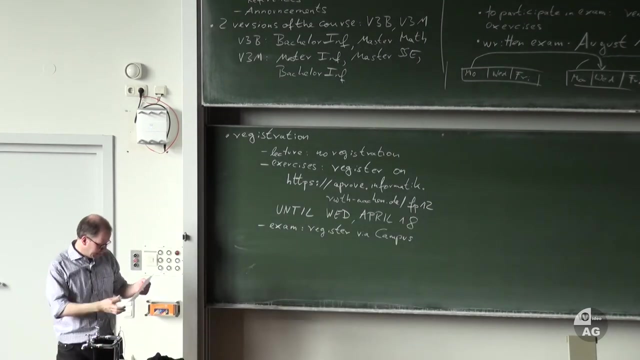 and now for the exam. you have to register as well, and this registration works via via campus. so this is the normal registration, as you do it for other exams as well, and the deadline for registering is May 18, so that's the same deadline for all exams. 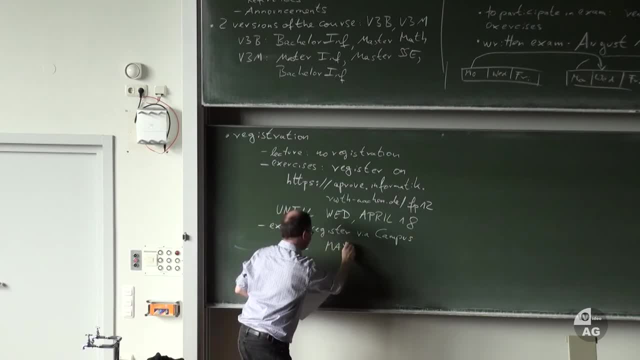 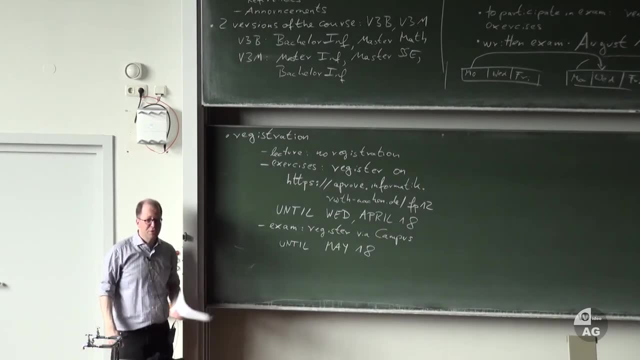 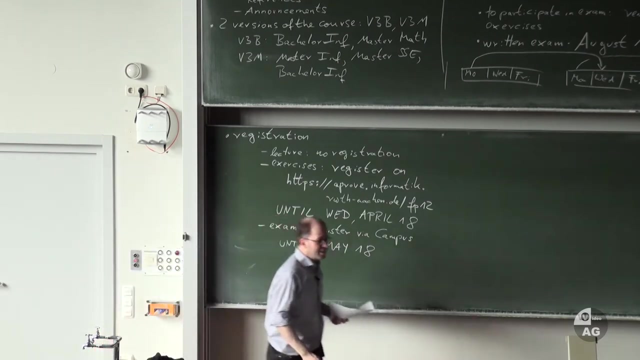 so this is nothing special, and I looked at it yesterday and I saw that 43 persons have already registered. so well, you have time until May 18 to do that, and that's that's all that's needed for registration. yes, that's a good question, and this: 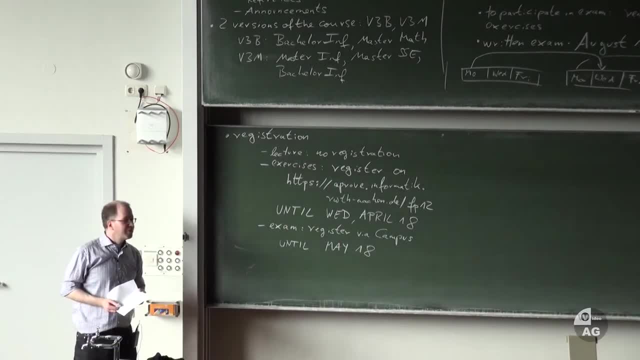 in former times you didn't have to register, but there was the promise of the ZPA that this should be possible now as well. so maybe one of you should explore, so one of. did you, do you have a common theory? that's not possible yet for some of you. 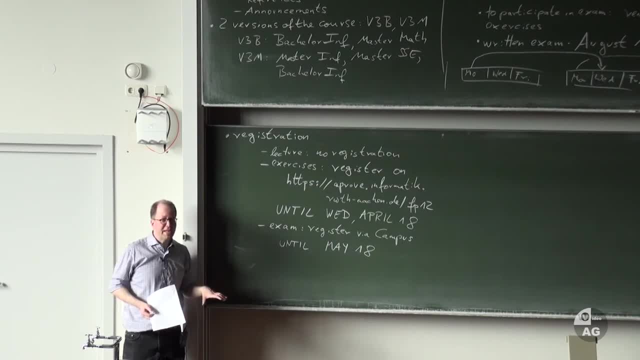 who have extended. ok, so you are sure that this is still like this in this semester. that's how it was previously, but they promised to change it, ok, so ok, then, this is so. then this doesn't hold for the bachelor students who take this as a master course and then. 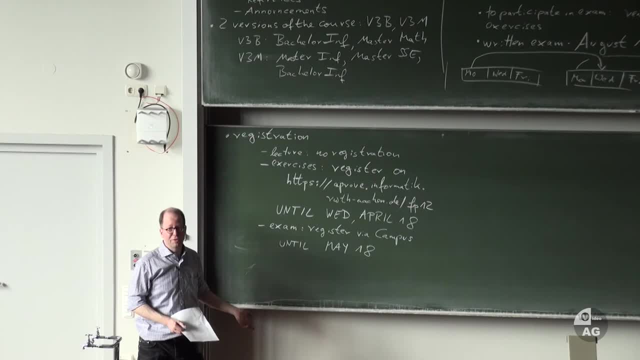 the bachelor students who take this as a master course. they have to register with us. only so informally. but I will check this again. so I will let me write this down and I'll check it and get back to you next time. so I'll tell you next week how this works. 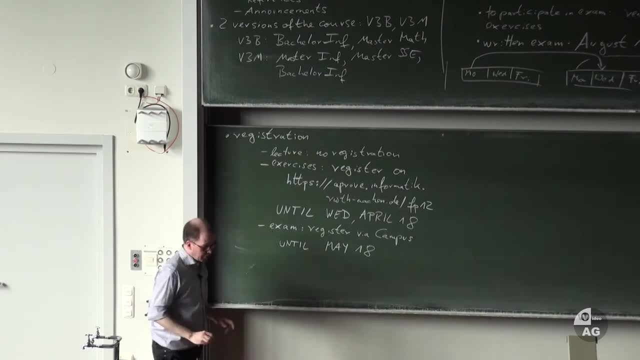 ok, ok, so any. are there any further questions concerning organization? yes, ok, handing in the exercises. you can do this in the exercises course, so just at the beginning of the exercise course you could do this, and there will also be a box, a wooden box, on our floor. so 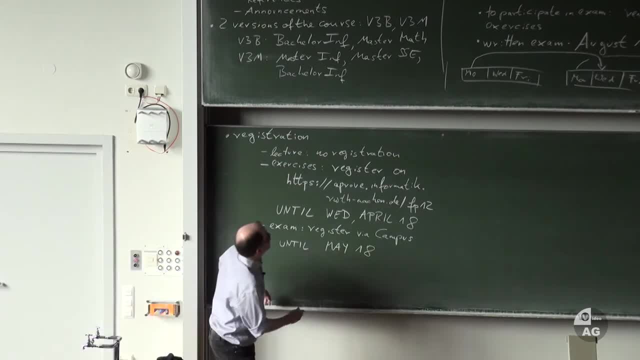 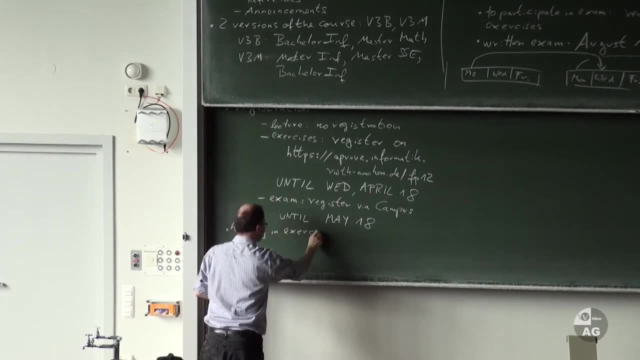 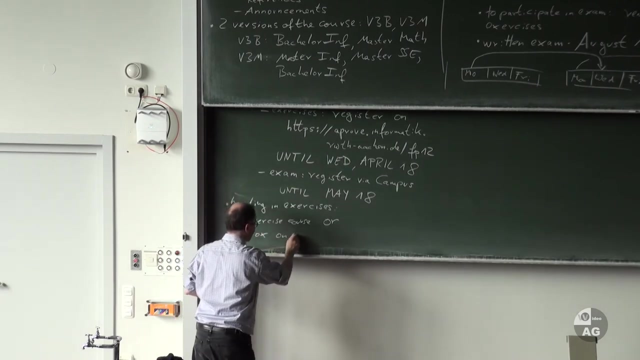 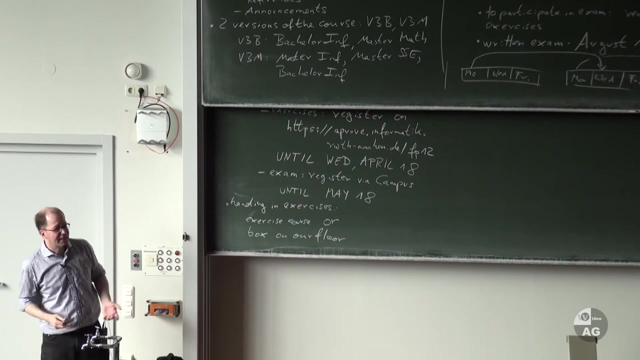 most likely beside my office, and so, with ok, we are handing in the exercises. so handing in exercises either at the beginning of the exercise course or box on our floor, and the deadline will be the beginning of the exercise course, because the exercises are presented in the exercise course, so afterwards you. 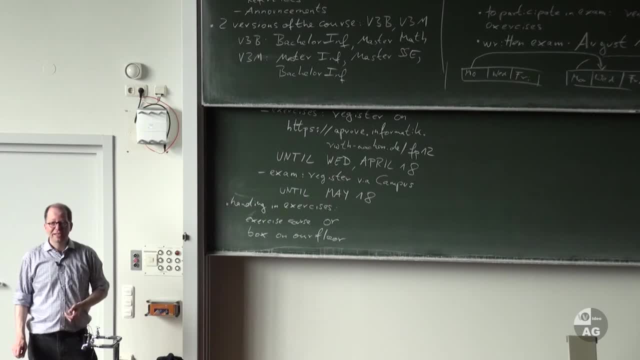 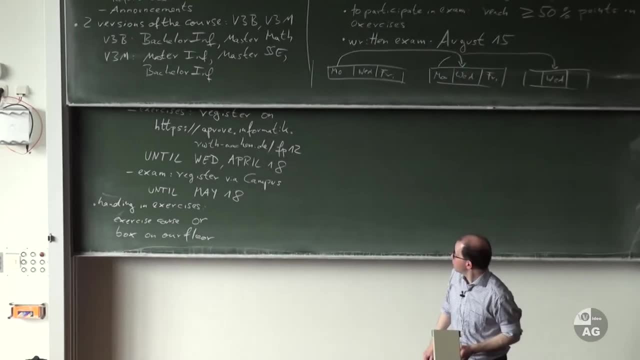 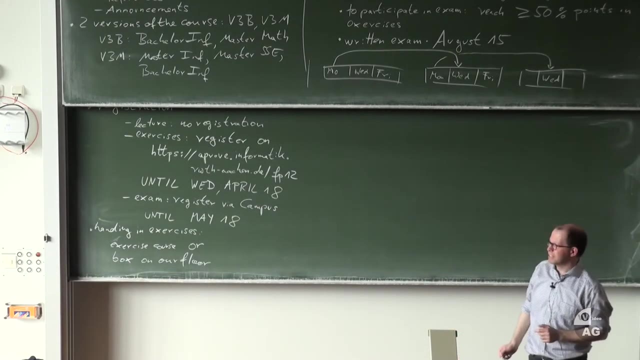 know the solutions then makes no point anymore and in fact, since there are so many people in this lecture, we are still looking for someone who helps us with grading the exercises. so, even if you are attending the course, that is still possible that you grade the exercises simultaneously. 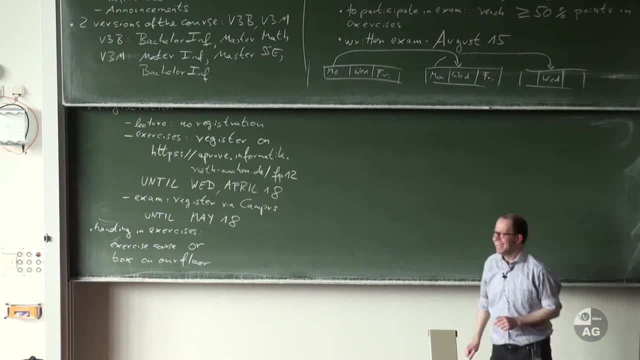 we have ways of organizing this, yeah. yeah, that doesn't mean that you don't have to do this yourself, but we have some experience in doing this. we did that before. so if you are interested in earning some money and getting some money for solving these exercises and grading exercises, 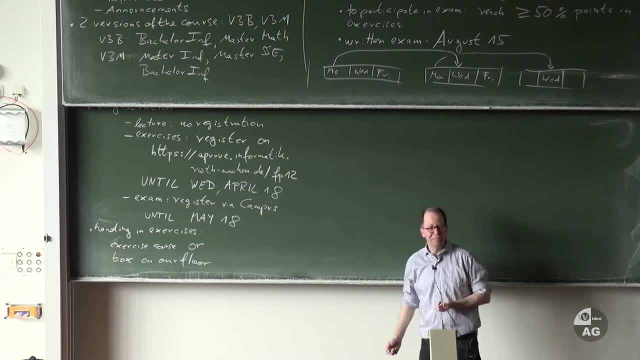 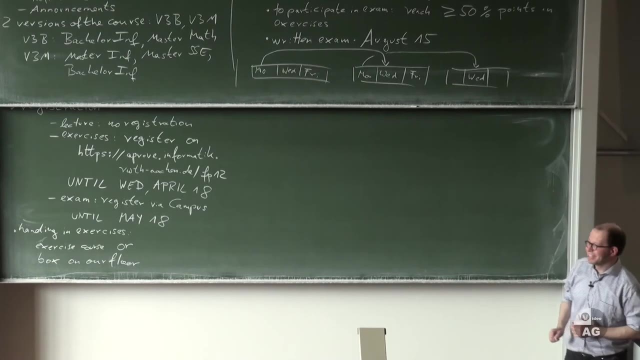 then please let us know, because there are so many people here, it would be good to have some more students grading. yes, you have to do the exercise in groups, and how large these groups are depends on how many people we have for grading. so definitely doing this alone there is no way. 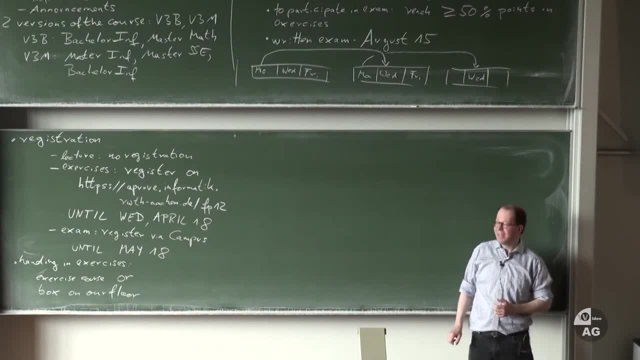 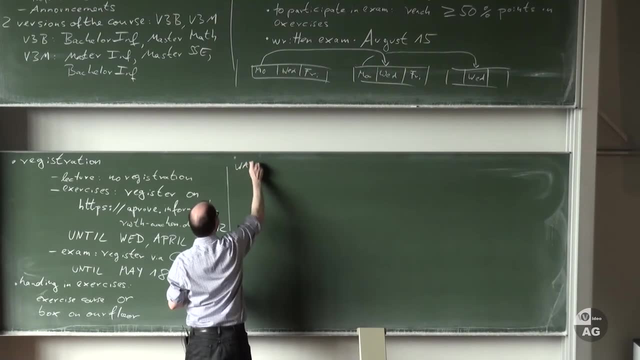 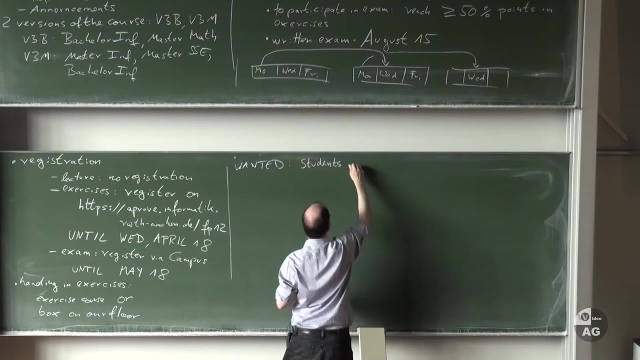 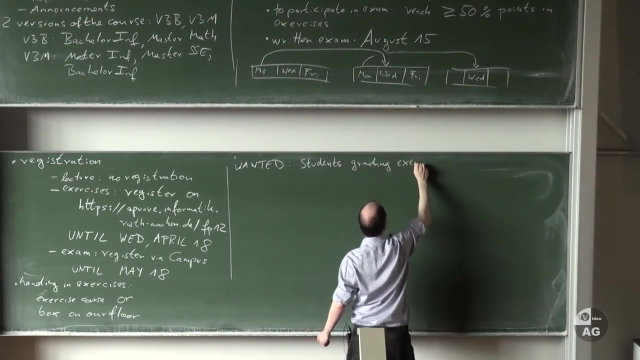 that we can grade all these exercises because we don't have enough students to do this. so wanted students, students, students, students, students, grading exercises, grading exercises- and this has something to do with money, right? so so you don't have to do this for free. ok, so think about it and let us 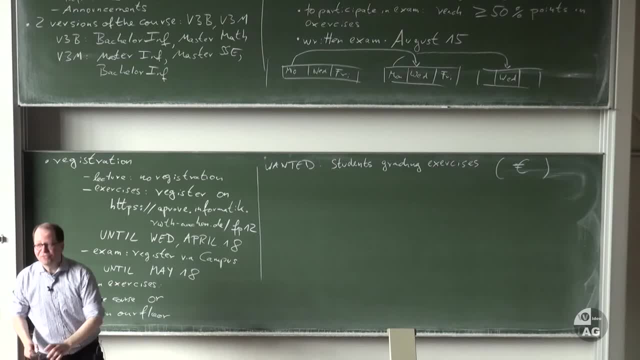 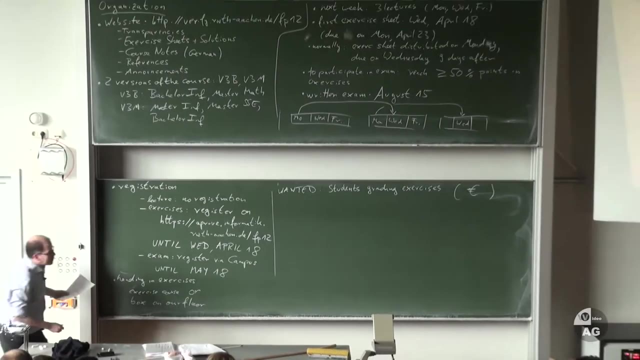 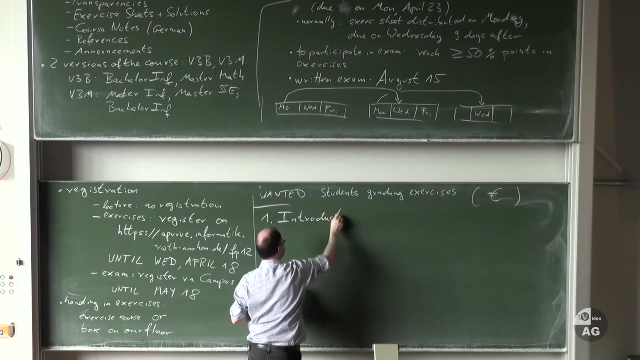 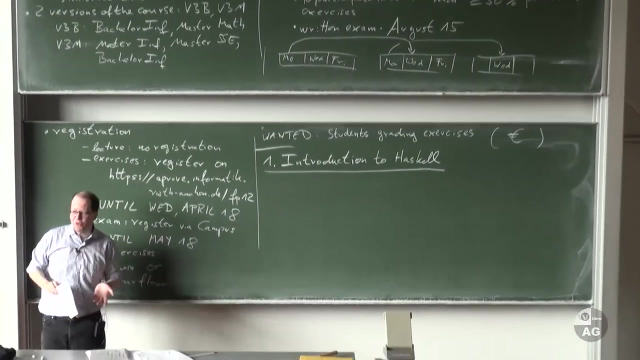 know if you are interested. ok, further questions. ok, no further questions, so we can start with the real content of the lecture. so then, let us start with chapter one, and chapter one is the introduction to Haskell. ok, so since we really write programs in Haskell, you should really run them. 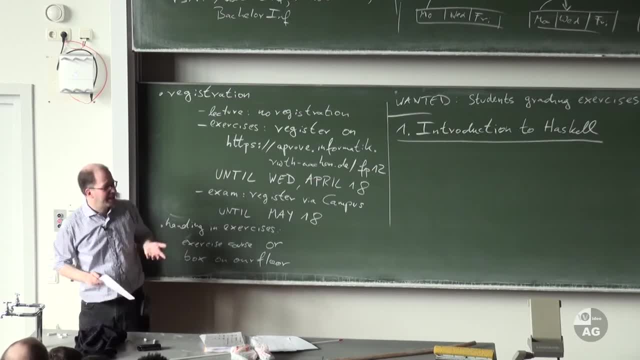 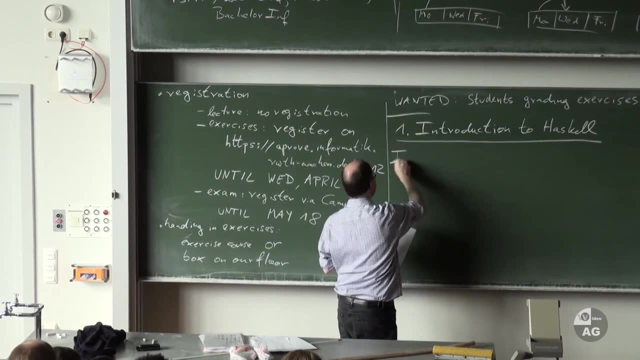 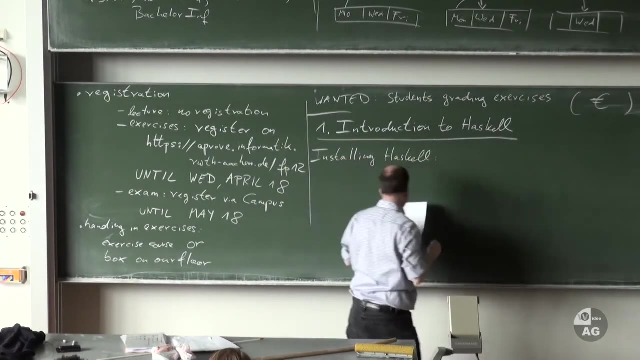 so this is not pure theory. so you should really test your programs, run your programs. so you should install Haskell on your favorite computer. and to install Haskell, the best thing is to visit the Haskell home page, and the Haskell home page is wwwhaskellorg- wwwhaskellorg. 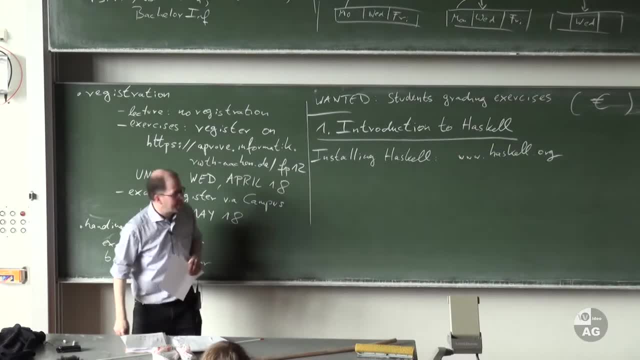 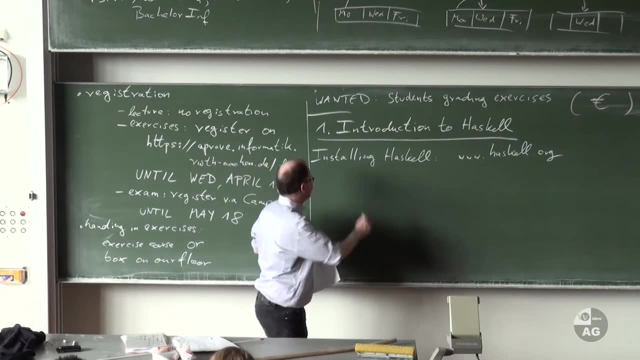 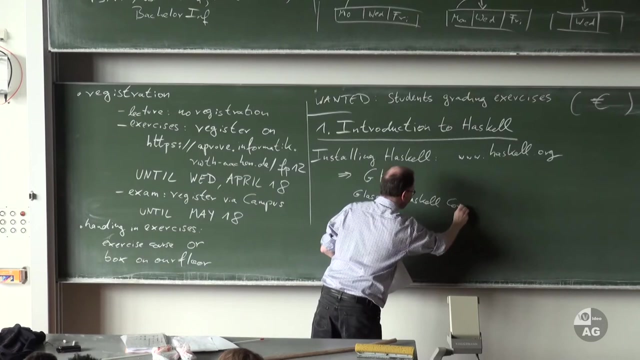 wwwhaskellorg, and on this website, you will find lots of information about Haskell. in particular, you will find implementations of Haskell, and we recommend to download the GHC, which stands for the Glasgow Haskell compiler, because this was developed in Glasgow and so you can download this from this website. 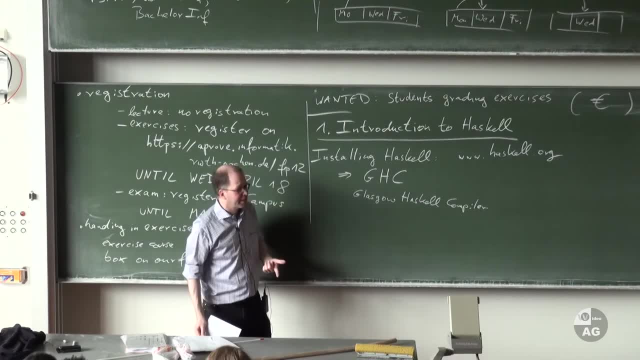 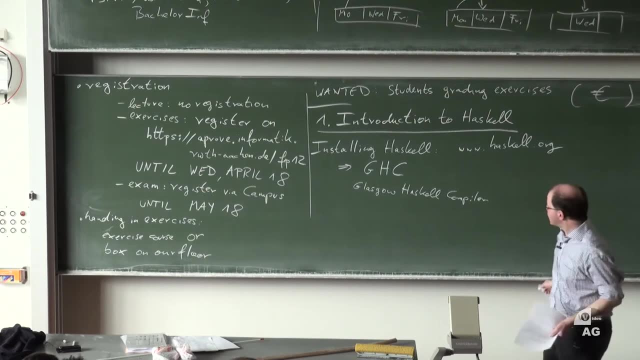 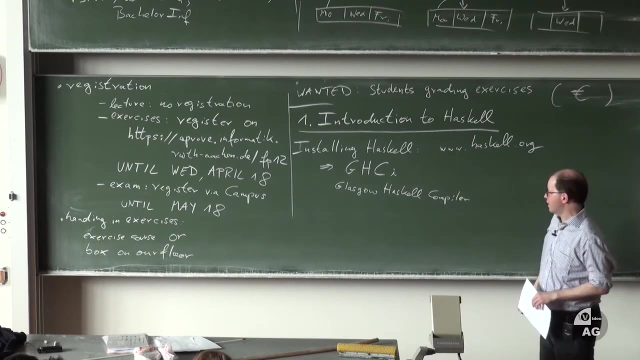 and you can find this for Windows, Mac and Linux, so for all major operating systems, and for the lecture, so for didactical purposes, we use GHCI, and this small i means this is the interactive mode of the Glasgow Haskell compiler and in particular, you can use this also as an interpreter. 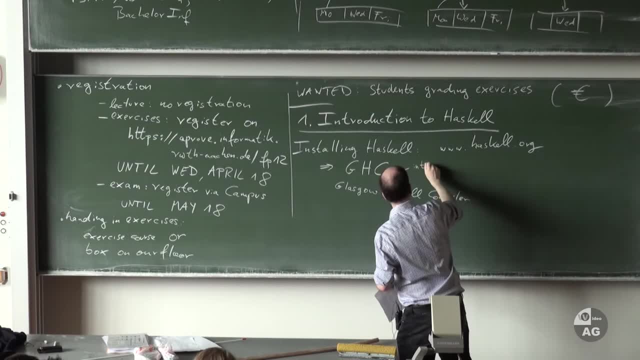 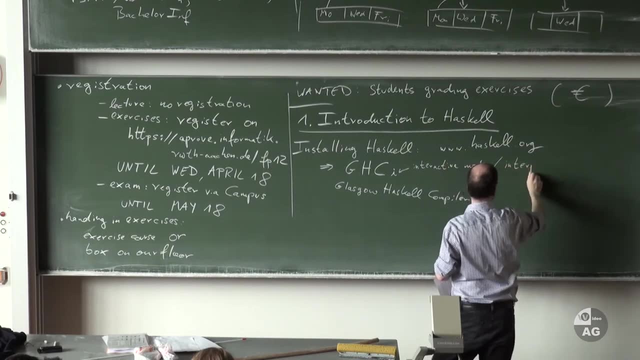 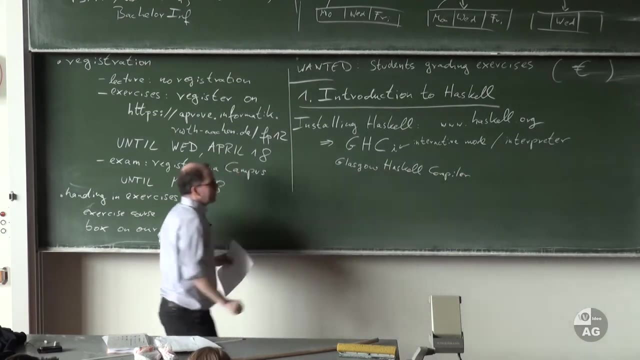 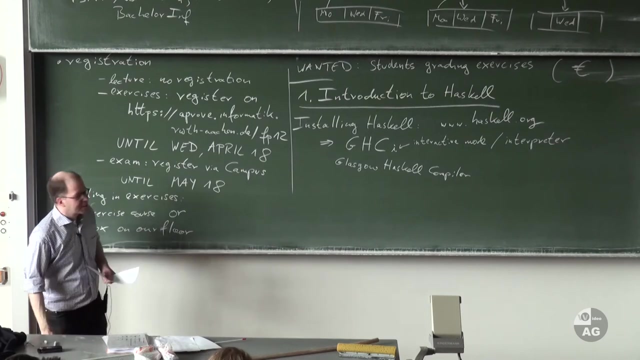 so this i means it's the so called interactive mode, and you can use this as an interpreter for Haskell. so that's the implementation of Haskell that we recommend, but you can use any implementation of Haskell, but that's the most standard one nowadays. so what's the plan for this chapter? 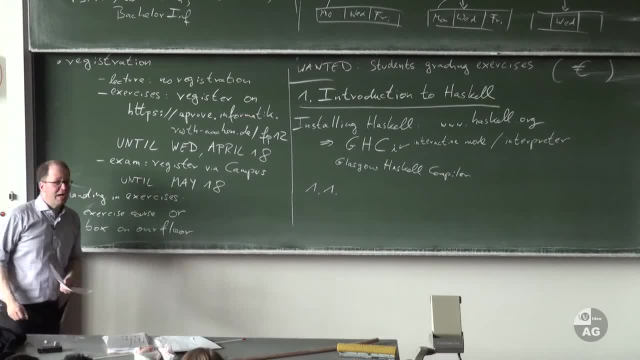 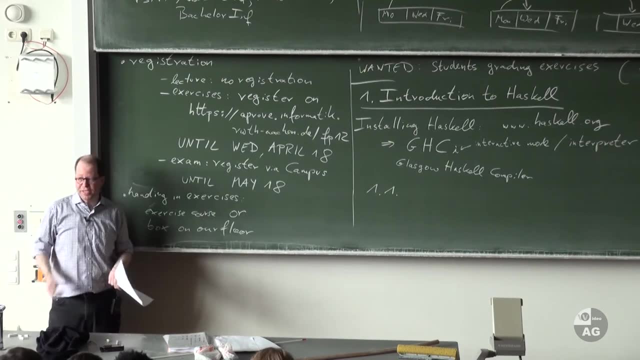 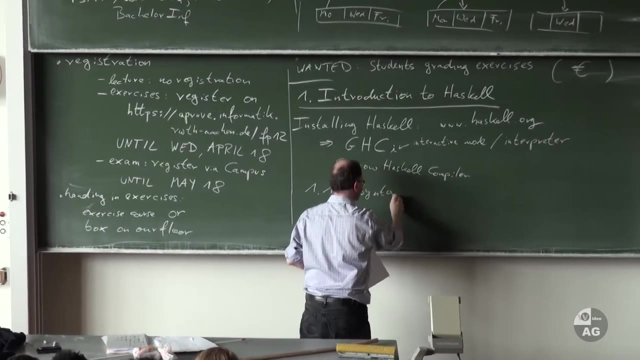 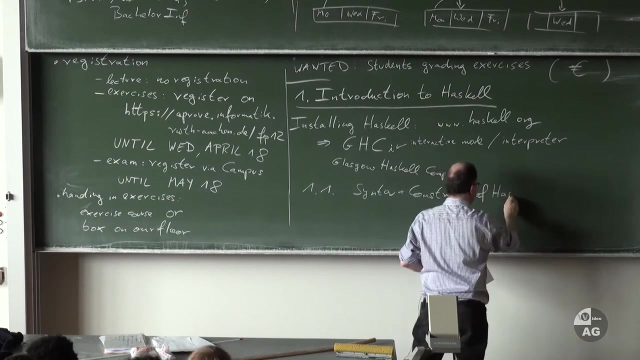 well, in section 1.1 I will introduce the syntax of Haskell, so the constructs of Haskell. we will not introduce everything but, well, 80% of Haskell. so this is: we introduce the syntax and constructs of Haskell and then, once we know what Haskell is, in the remaining subsections, 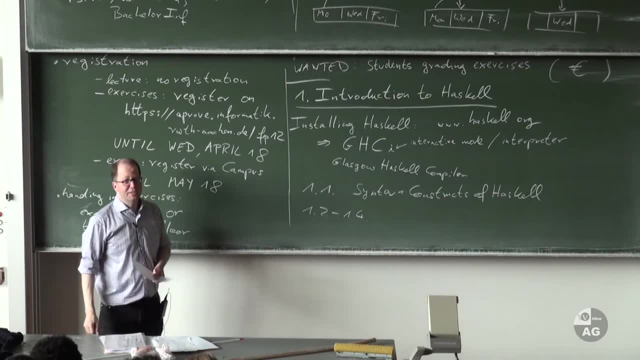 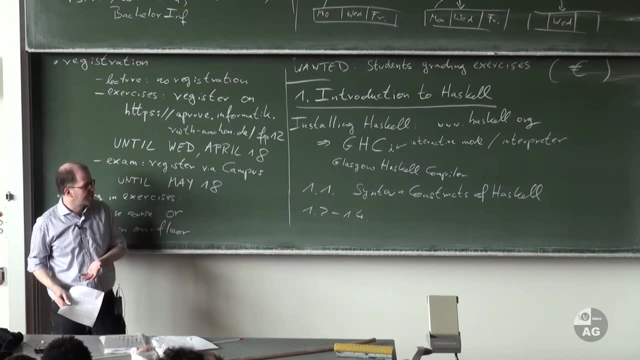 1.2 to 1.4 we will discuss typical programming techniques in functional languages. so I mean many programming techniques that you know from imperative programming you can also use for functional programming. but there are some specific things, so here we will focus on those things. 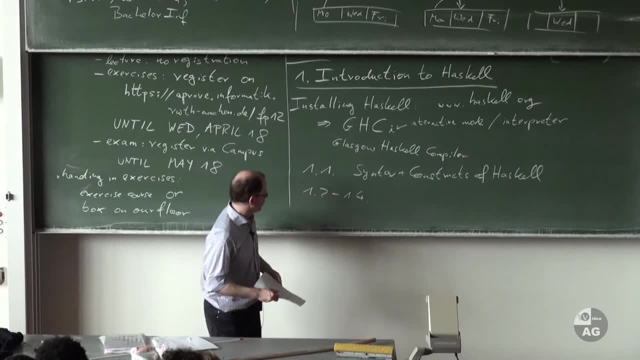 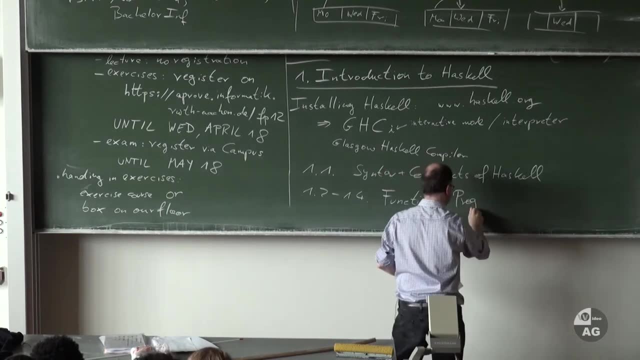 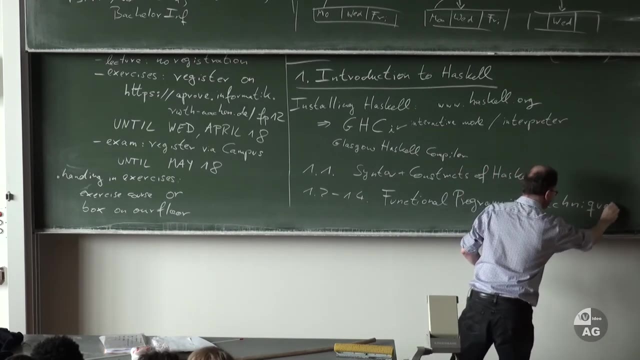 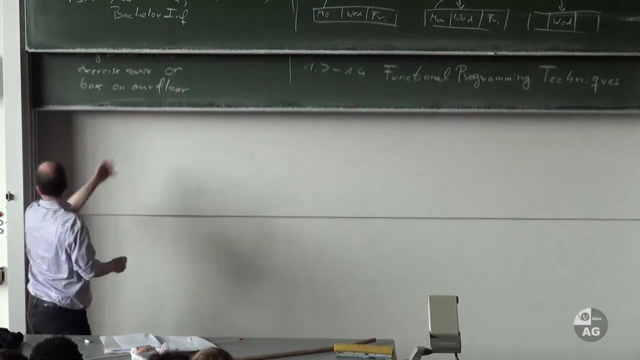 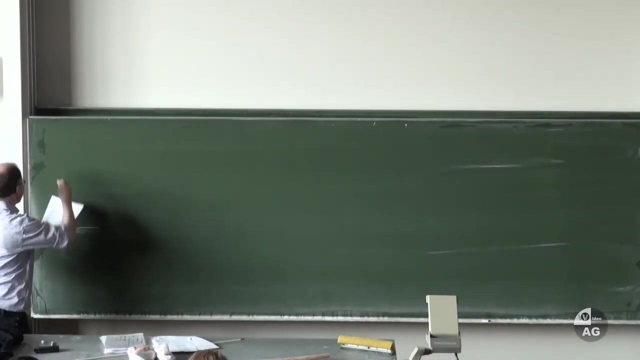 that you can do in functional languages and you cannot easily do in imperative languages. so functional programming techniques, ok. so this is the plan. ok, and before we start I again have to wipe boards a bit. ok, so let's look at the syntax and the constructs of Haskell. 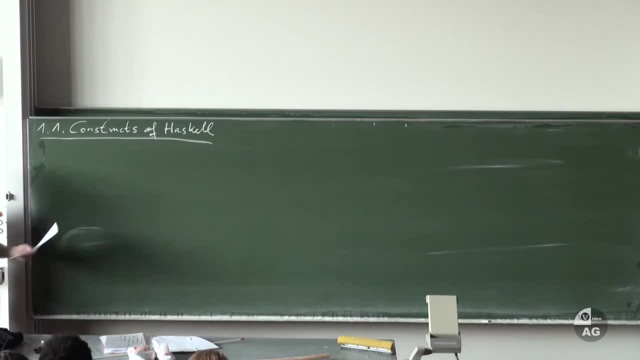 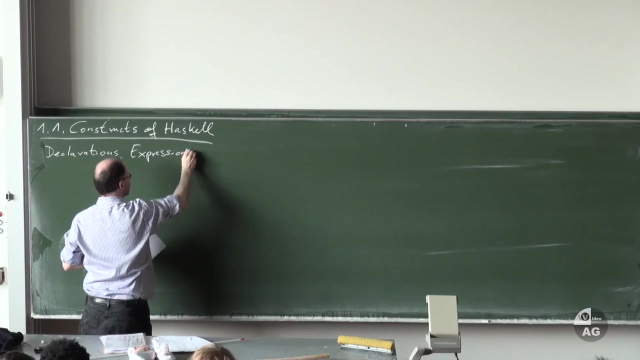 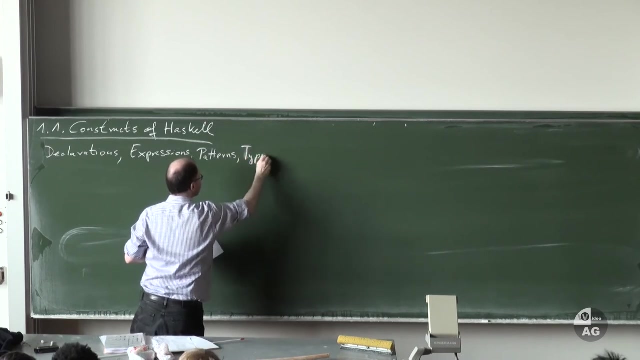 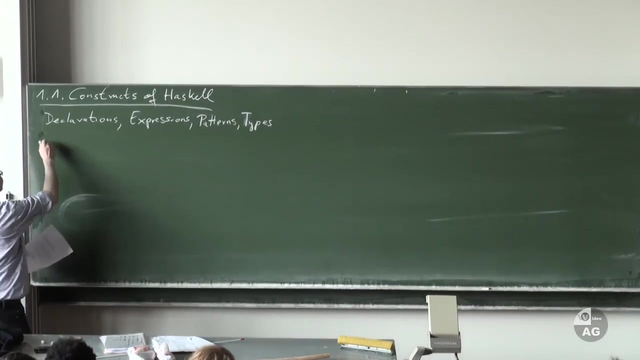 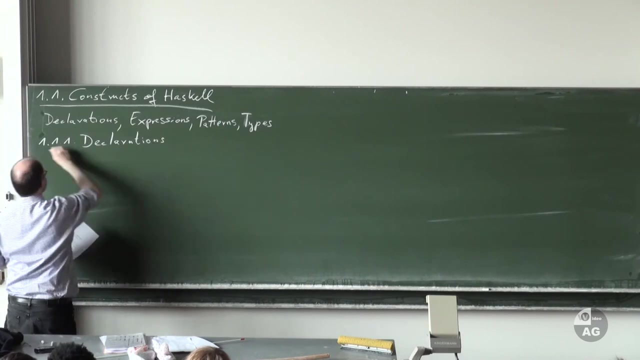 and essentially there are four main constructs in Haskell, namely declarations, declarations, expressions, expressions, patterns, patterns and types, patterns and types, patterns and types. so these are the four main constructs in Haskell and we will introduce them one after another. so let's start with declarations: declarations, declarations, declarations, declarations. 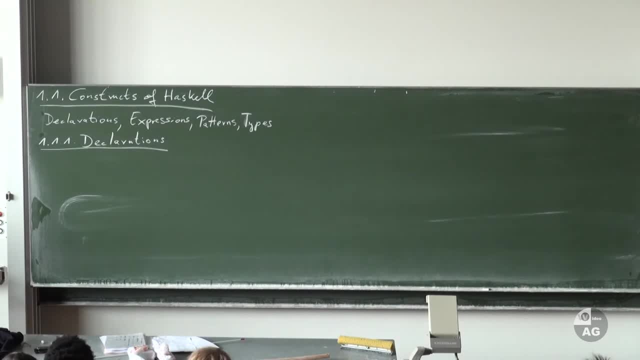 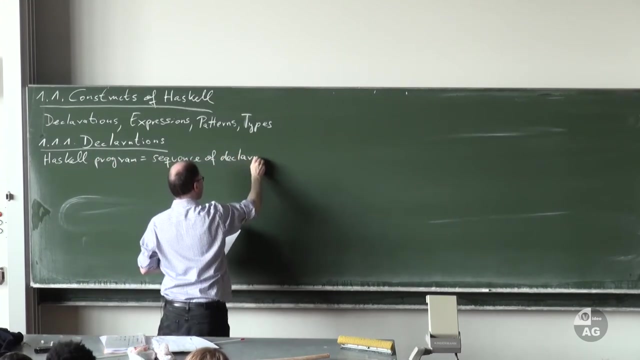 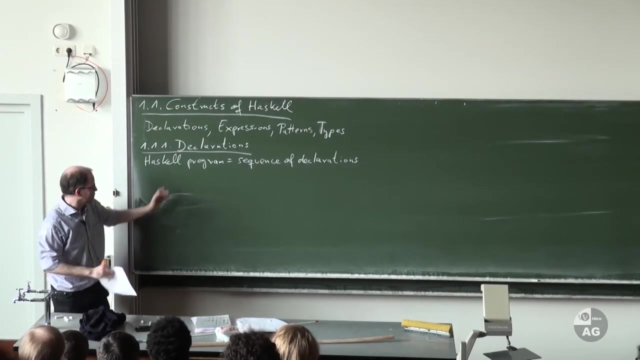 so, essentially, a Haskell program is just a sequence of declarations. so a Haskell program is a sequence of declarations and, for a certain reason, these declarations all I mean. you write these declarations in rows and these rows have to start at the same position, so it looks like this: this is the first row and the 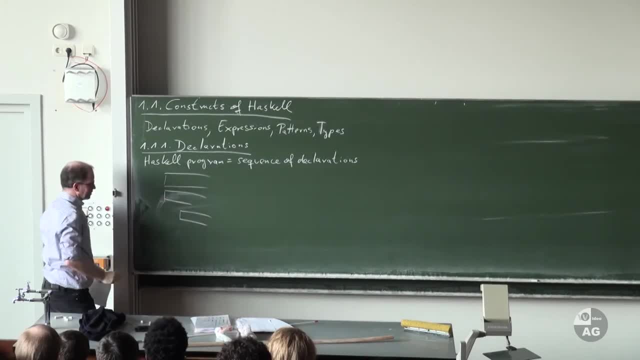 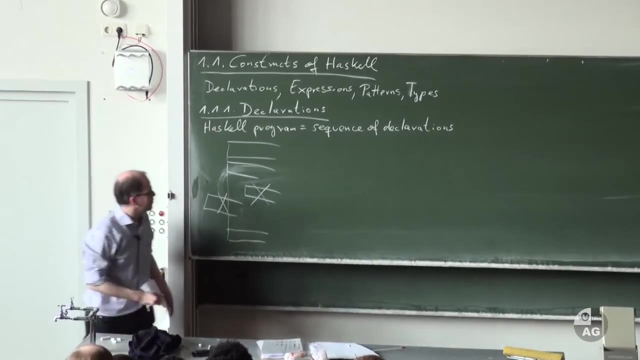 second row looks like this and the next row does not look like this and it does not like it look like this, but it starts at exactly the same point, so they really have to be have to start at the same position. that looks awkward and there's a certain reason for that that we will learn after another, afterwards, so so. 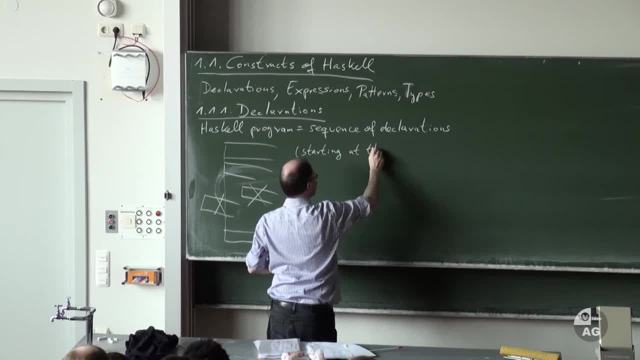 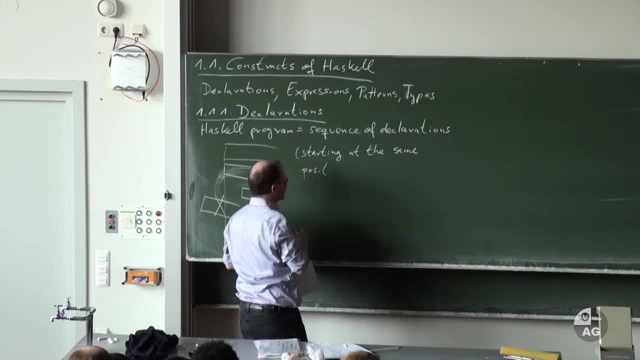 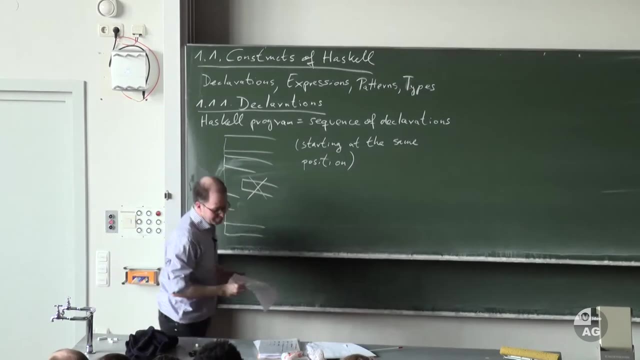 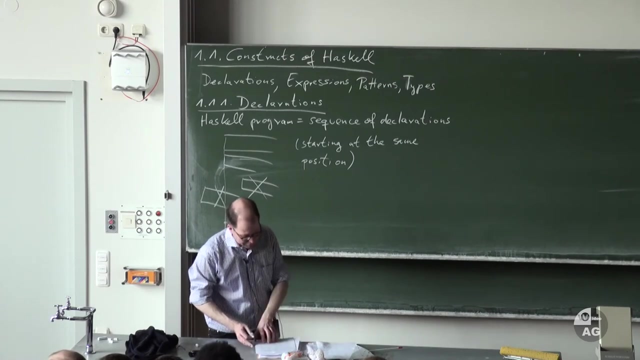 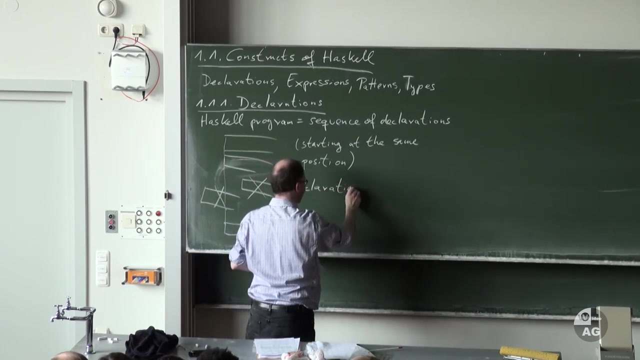 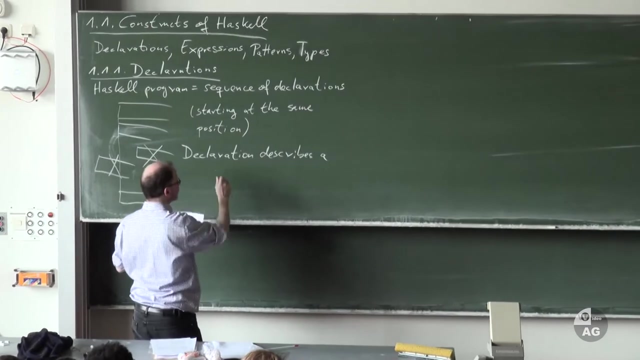 starting at the same position. so the layout of the program plays a role in Haskell. so that's, that's awkward, but that turns out to be quite handy afterwards. and what? what does the declaration do? a declaration describes a function. so the idea is that a declaration describes a function, and there are two kinds of declarations, namely type. 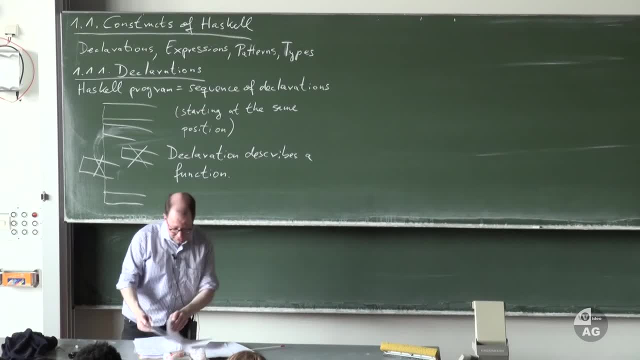 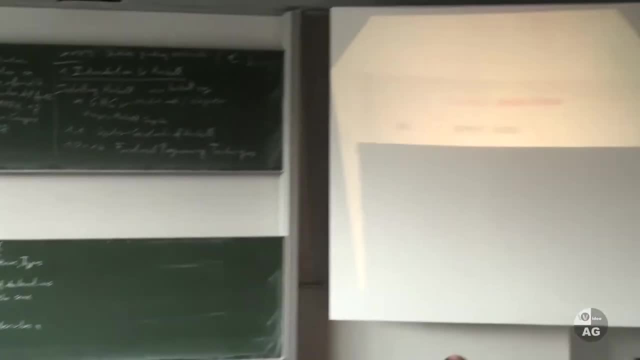 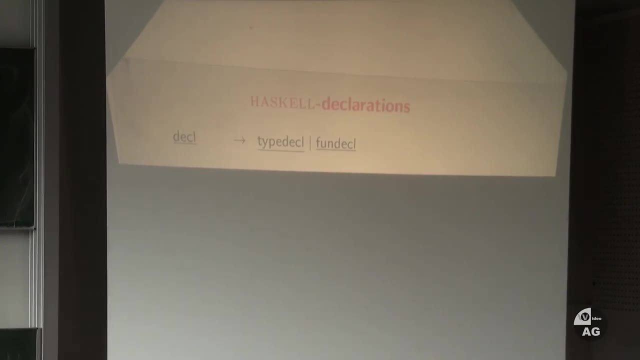 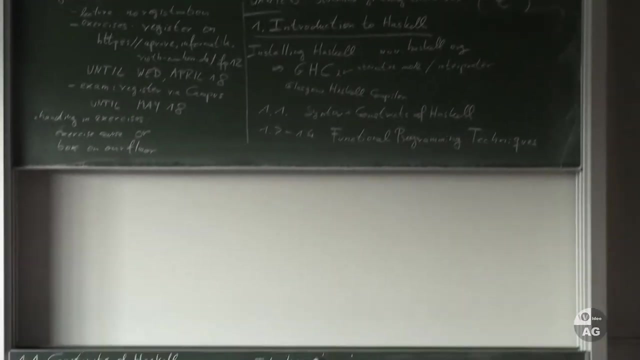 declarations and function declarations and to introduce the syntax of Haskell formally. I will do this via a context-free grammar, and I will extend this more and more. so the first grammar rule is this: you, so we, introduce the syntax of Haskell by appropriate context-free grammars. the 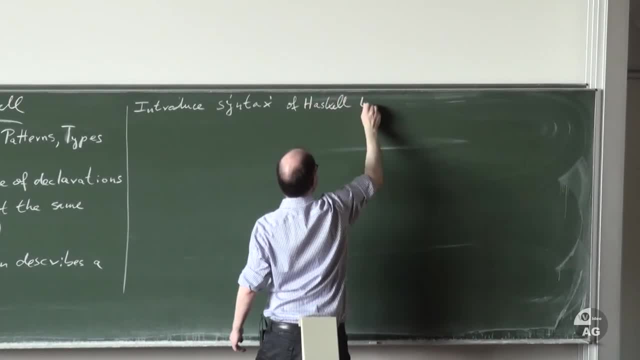 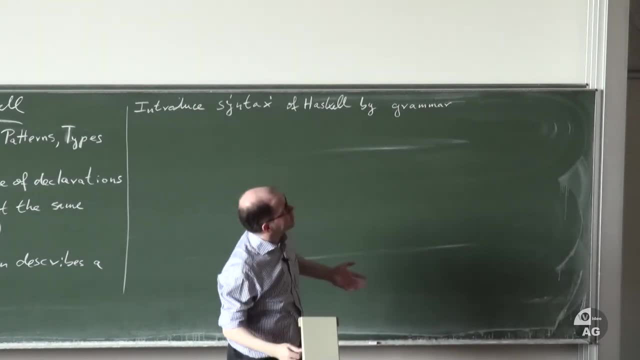 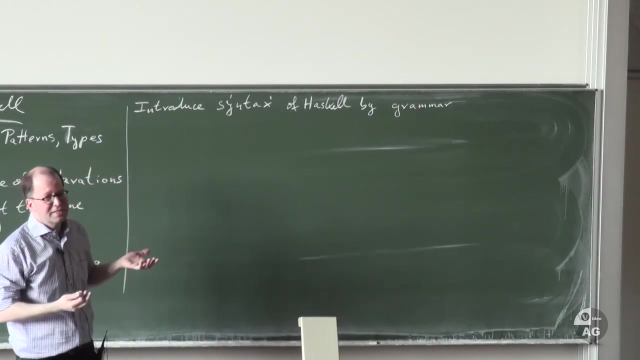 syntax of Haskell by a grammar, and the non-terminals in this grammar are underlined. so in this way you can distinguish non-terminals from terminals. so if you know nothing about grammar, you don't worry. the underlying things, these are things that i just auxiliary symbols. they don't occur in the program, so you don't write tackle in your. 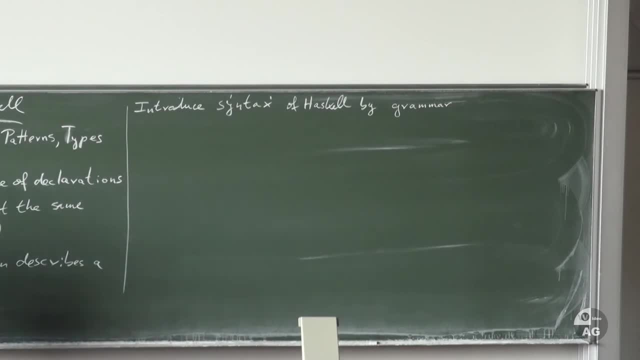 program or type daqui. this is just something to to construct the programs. but later on there will be some keywords that you really write into your programs. for example this cold and colon. you're writing a program or in, so these things really occur in your program. but tack, dec are type t email account to uniliation. 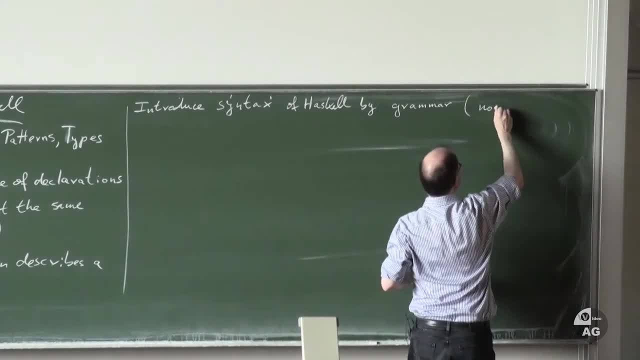 write by a grammar, by the non-terminals underline things that are just auxiliary symbols. they don't occur in the program, so you supports are�� are underlined here. so if you want to have a declaration then it's either a type declaration or a function declaration. 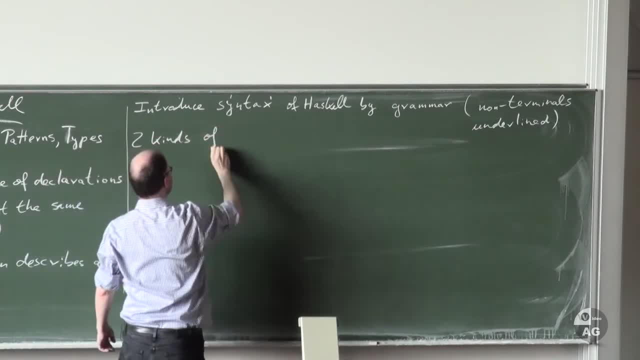 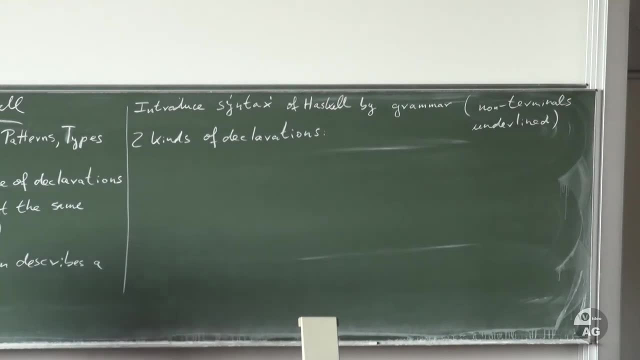 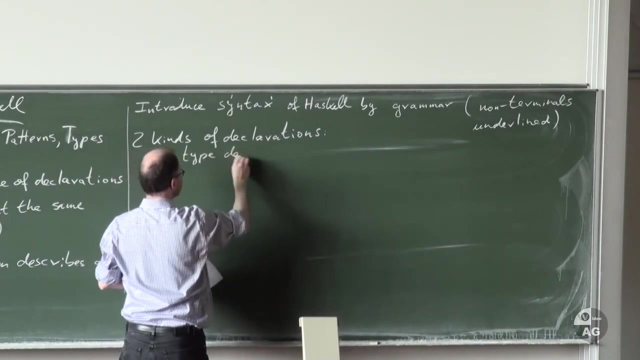 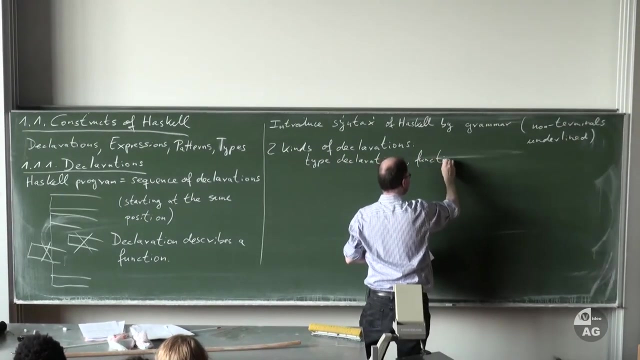 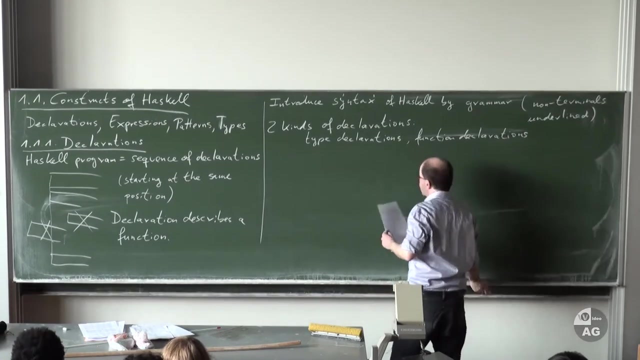 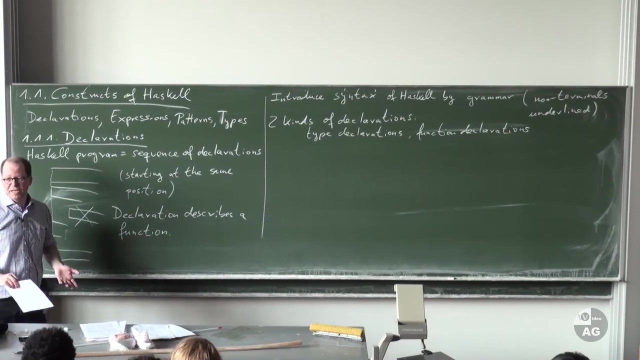 so there are two kinds of declarations. so let's first look at type declarations, type declarations and function declarations and, before I forget, comments. so apart from declarations ASK, the program can have comments like in any other programming language, and comments are important as in any other programming language. 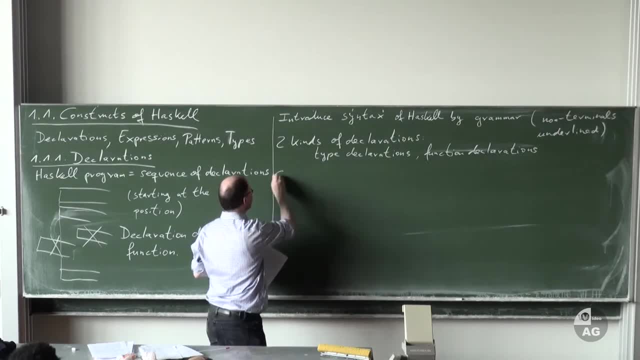 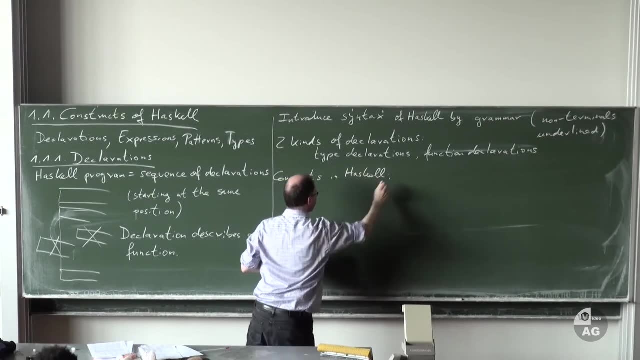 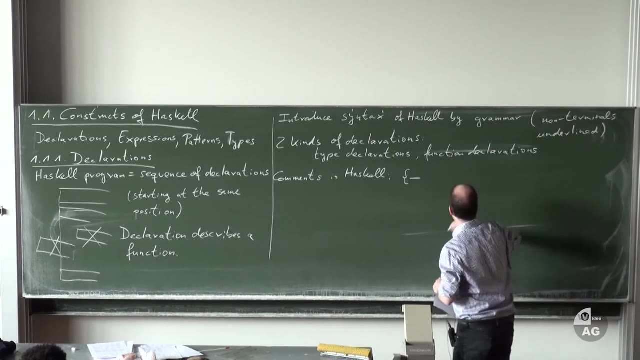 but the syntax for comments differs from language to language, so before I forget that, I will mention this. so comments in Haskell you can either write curly bracket, dash, and then everything which comes after that is a comment, until you reach dash curly bracket. so if you want to have long comments, 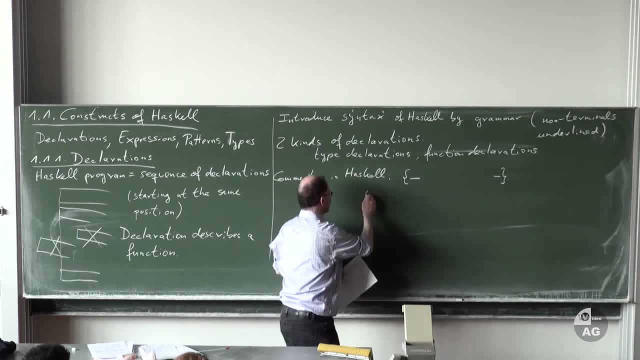 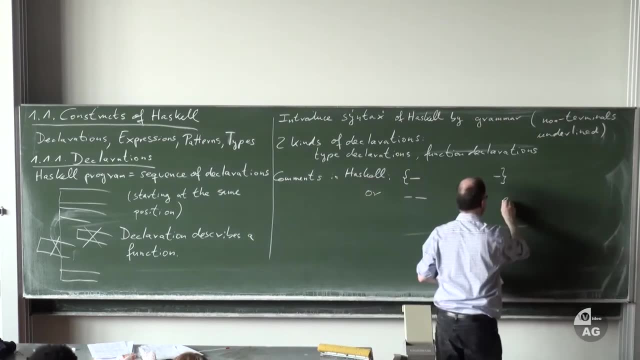 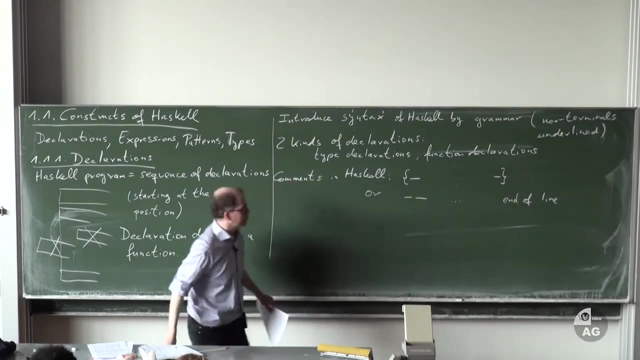 which go over several lines. you can use this, and if you have a short comment which fits in one row, you can write dash, dash and then everything until the end of line. everything in here is a comment. so that's similar to other programming languages, but the syntax 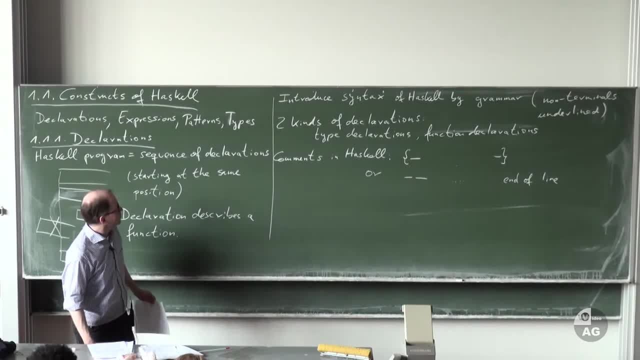 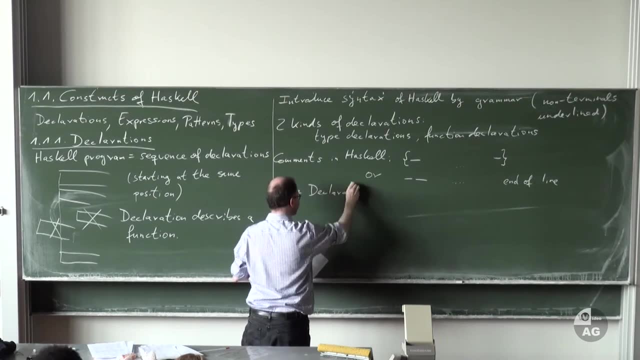 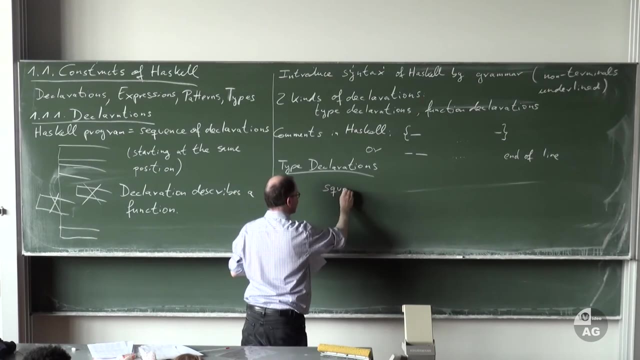 is a little different, but that's it. so let's go back to the declarations. what are type declarations? ok, here's an example for a type declaration. for example, I might want to define a function called square, and the idea is that square should take a number and square it. 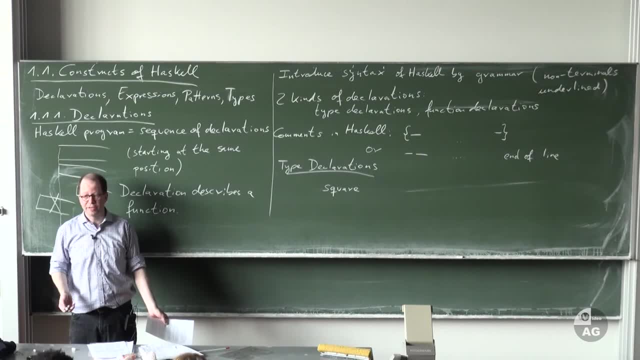 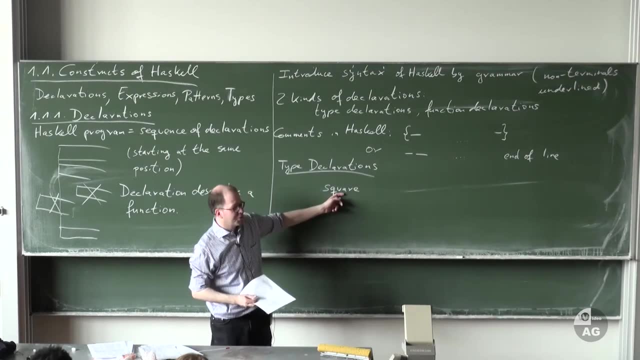 so square applied to 3 should give me the number 9 3 times 3. so the type declaration tells me what is the type of this function and they look like this: they start with the name of the function, then we have this double colon and then we have the type of the function. 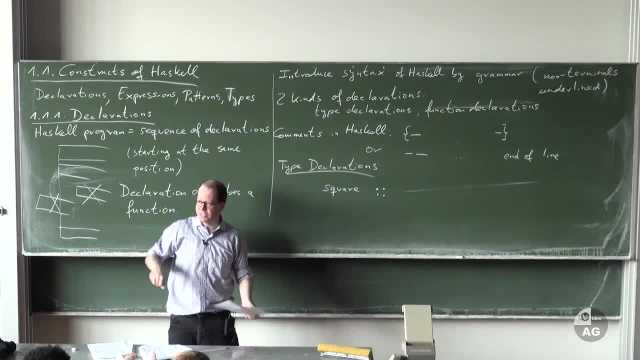 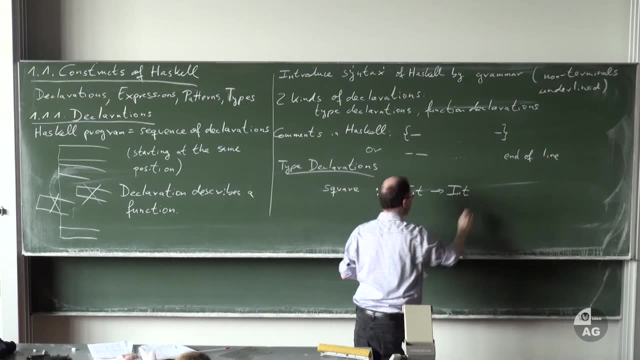 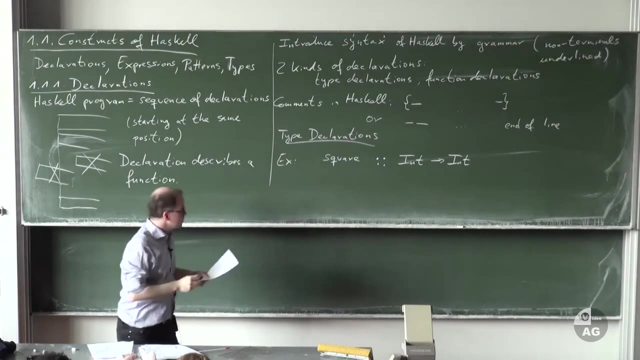 so in this case this would be a function from int to int. takes an integer number and returns an integer number. so it's a function from int to int. so this would be an example for a type declaration. so, in general, what's the syntax for type declarations? 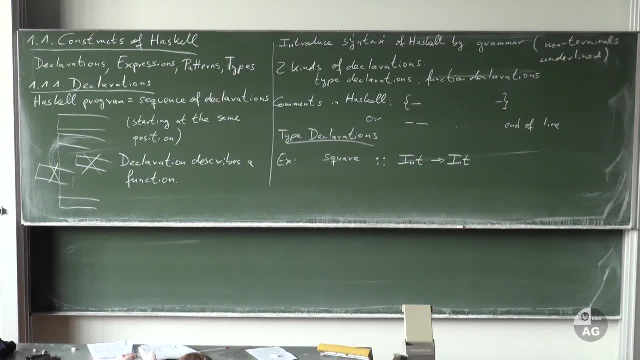 the syntax for type declarations looks like this. so a type declaration. type declaration has the following form: you start with the name of a function, and for names of functions we use the name of a function, the same syntax as for variables. so a function name is simply a variable. 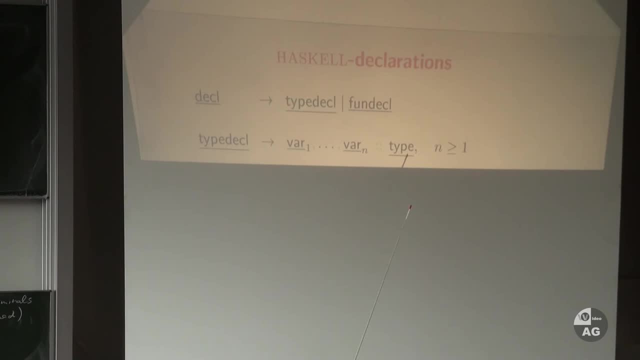 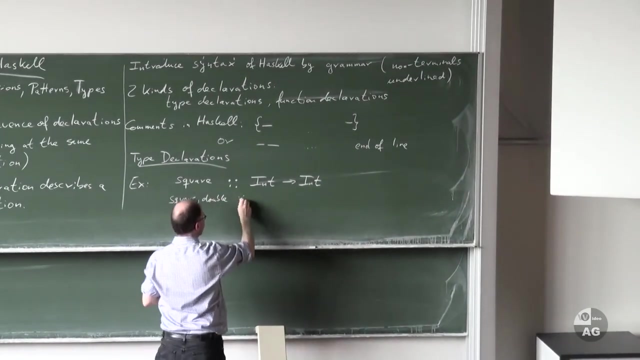 and then comes this double colon and then comes a type and you can, in one single type declaration you can declare several functions of the same type. so you could also say: well, square, I want to declare square and double simultaneously. both square and double are functions of type int to int. 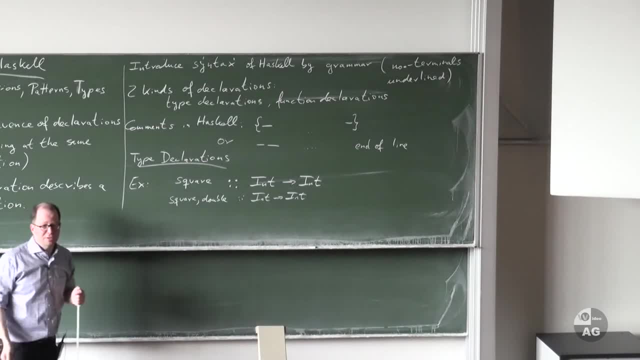 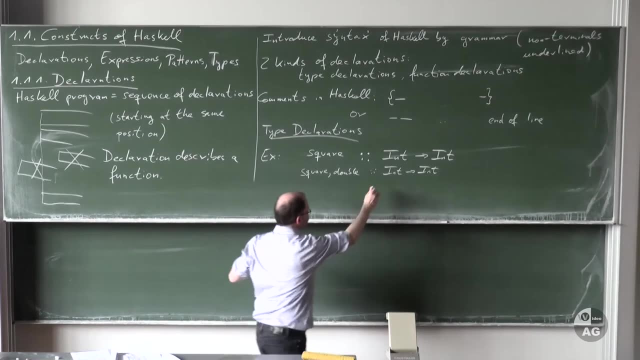 so something like this would also be possible. so if the functions have the same type, you can do it in one way or another. so you can do it in one way or another. one single type declaration. and so what's the meaning? well, this means this is the domain of the function. 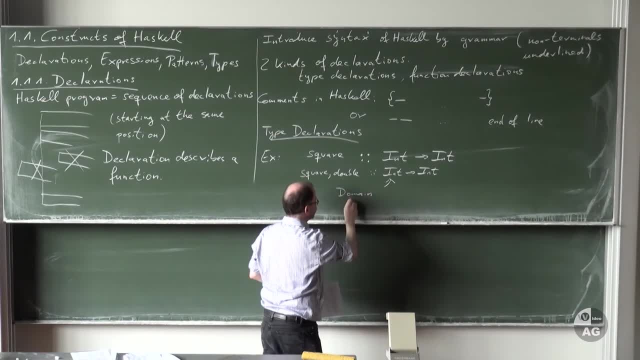 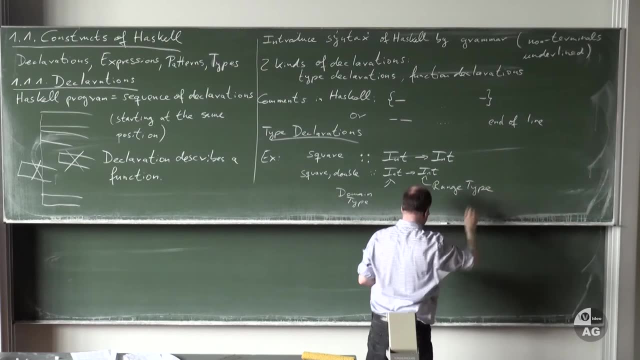 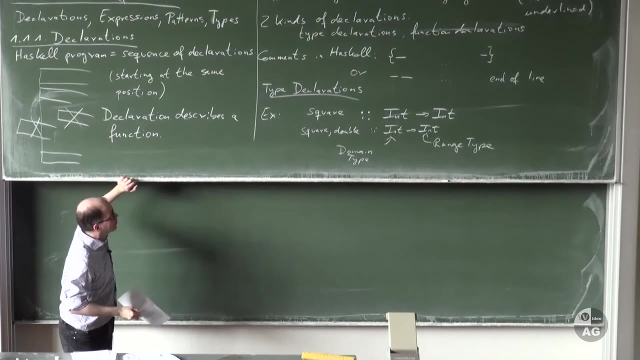 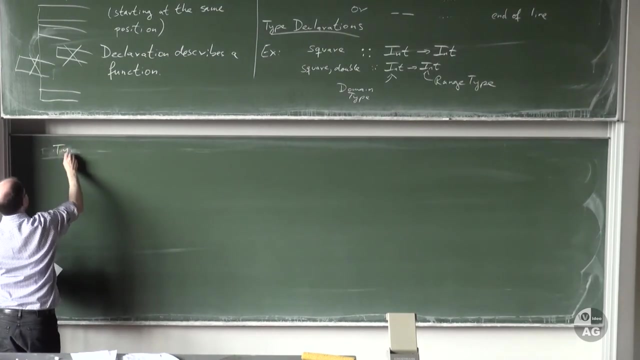 so this is the domain type of the function and this is the range type. and how types are constructed we will define formally later on, but you can already see how this works. so what types do we have? well, we have types like int for the type of integer numbers. 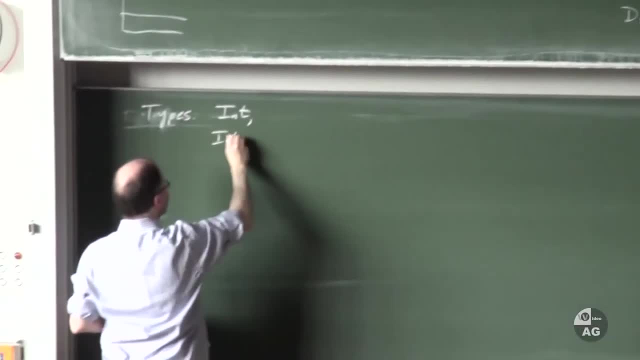 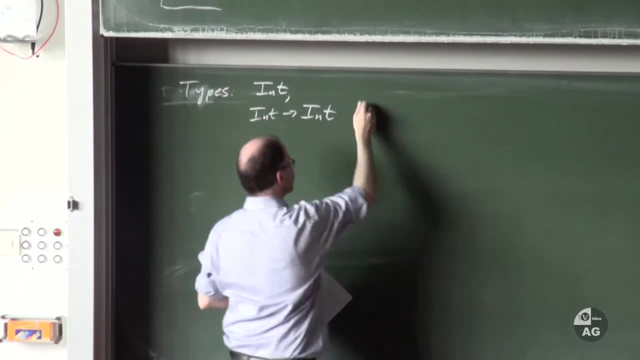 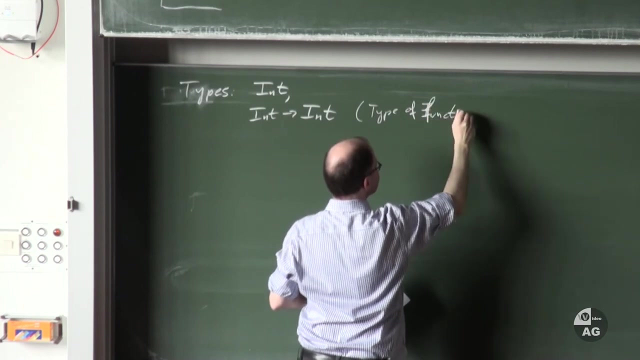 we have also types like this: int- arrow, int. this is also a type on its own, because this is the type of functions from int to int, type of functions from int to int, and so you can already see that if you have a type, you can construct new types. 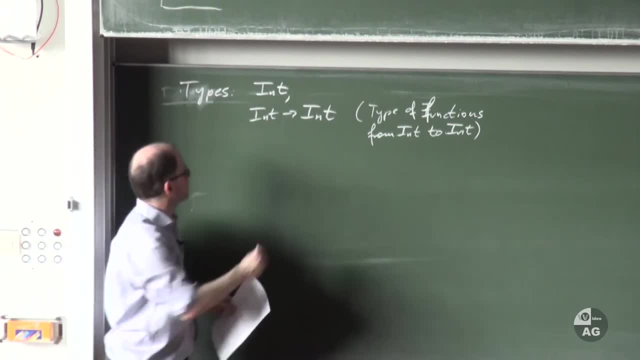 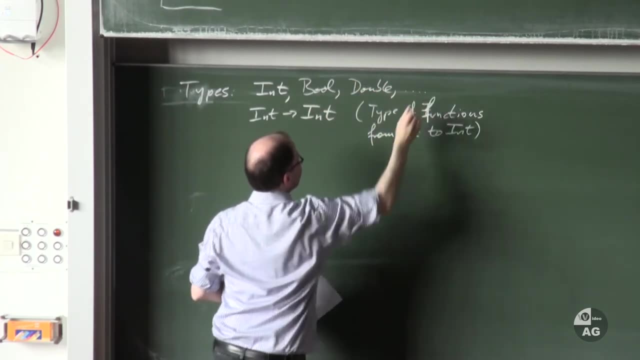 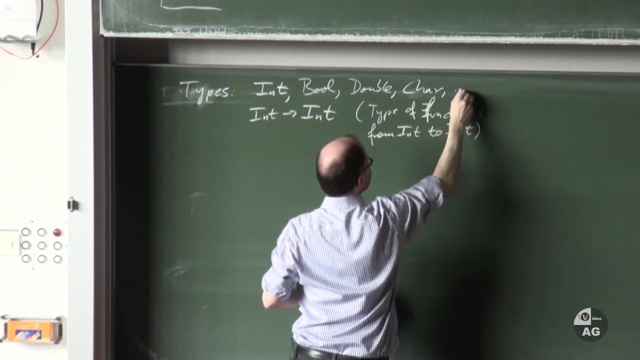 by writing an arrow between two already existing types. there are also some more of these base types, so there's also something like bool or double or well- all the standard basic types that you have in other languages. you have here as well- character, so all the stuff you have also here. 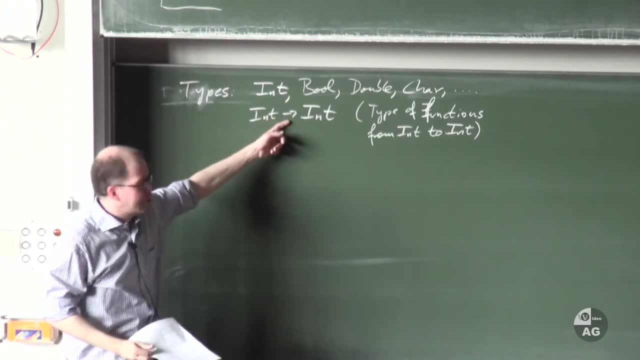 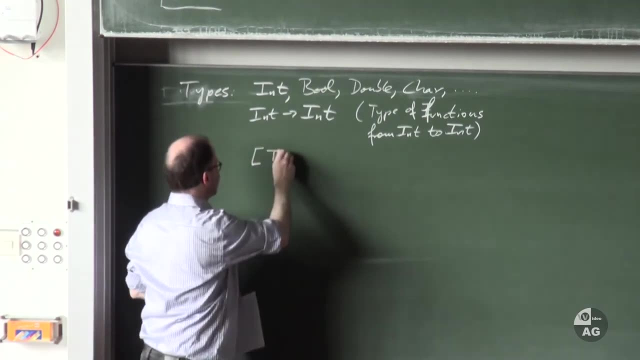 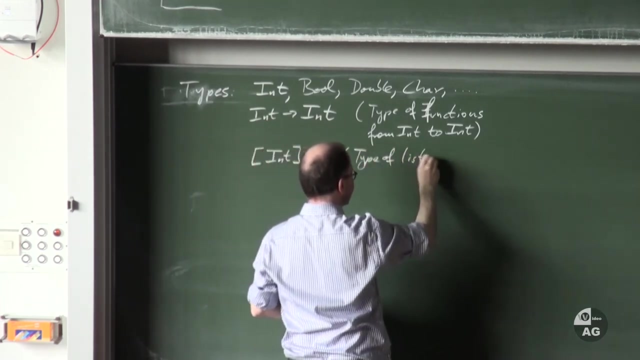 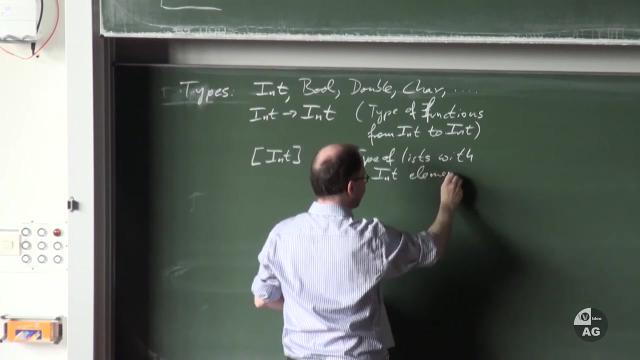 and you can construct new types of types by writing an arrow between two already existing types, and you can construct new types by writing square brackets around the types. so this would be the type of lists with integer elements with integer elements, and well many other types are possible. 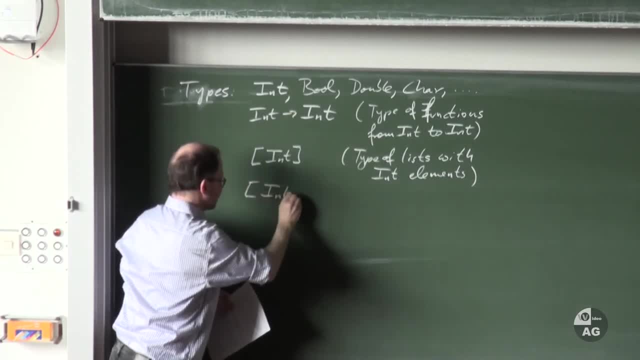 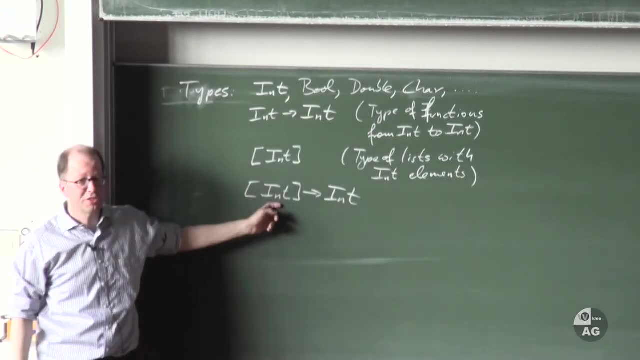 for example, you could write a type like this: now what would this be? this would be the type of functions that take a list with integers as input and return an integer. so, for example, a maximum function might have this type: it takes a list of integers and gives you back. 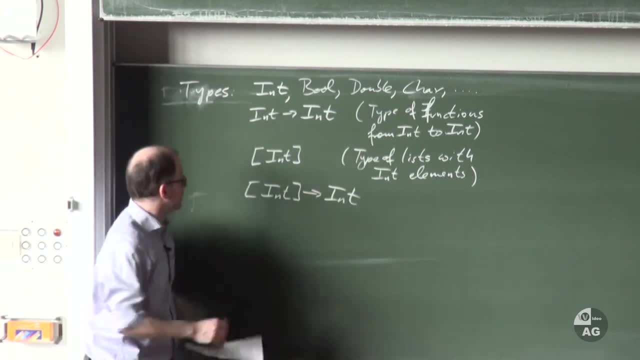 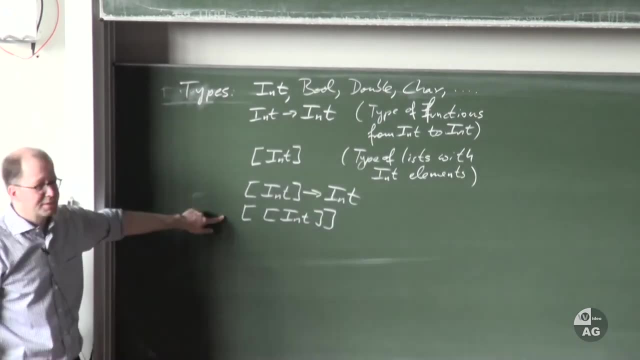 the maximum element of the list. or you can write: you can also write something like this: what type is this? it's a list of list of integers. right, you can also write something like this. you can also write something like this. you can also write awkward things like this. 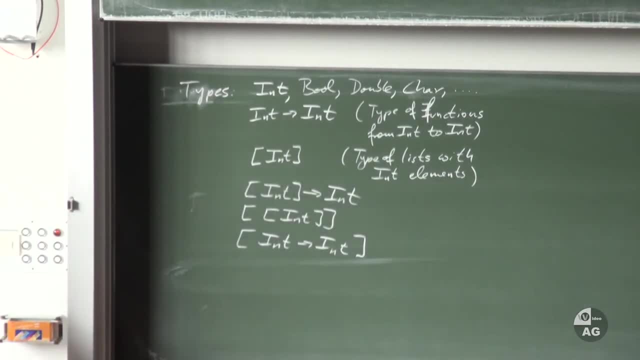 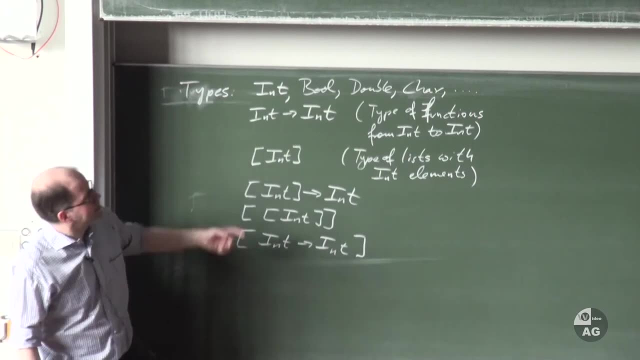 what's this? it's a list of functions, and all the functions go from int to int. so, for example, this could be the list containing square and double. i mean, square goes from int to int, double goes from int to int. so this list containing square and double. 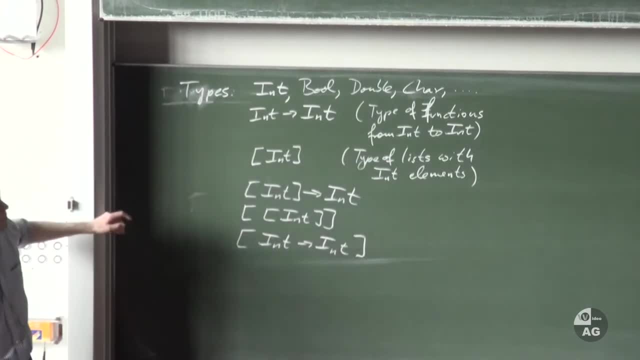 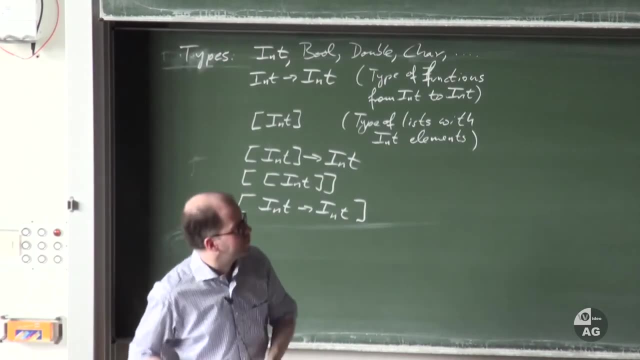 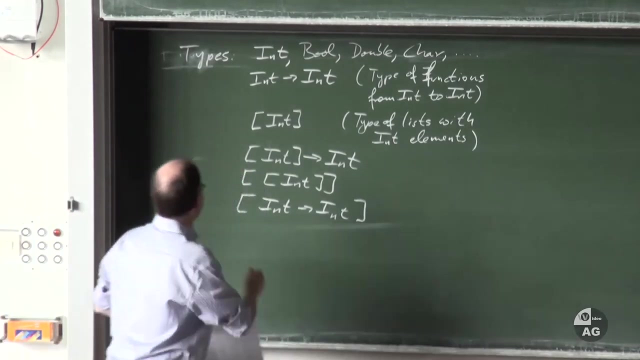 would have this type. so this gives you some ideas of types. there are other possibilities, but just to to show you how types can look like. and type declaration says: we have a function or a variable which has a certain type. this is, uh, what is declared here. 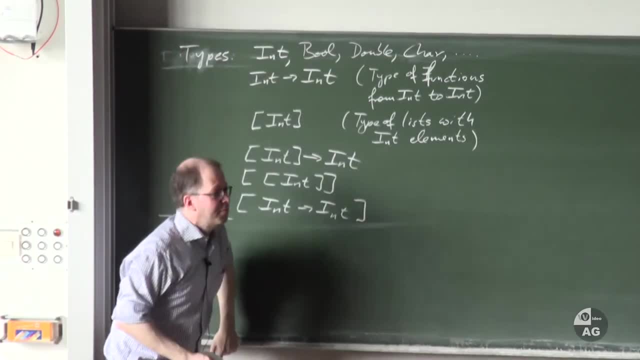 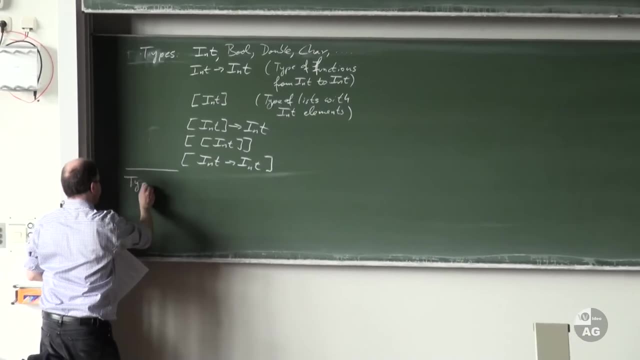 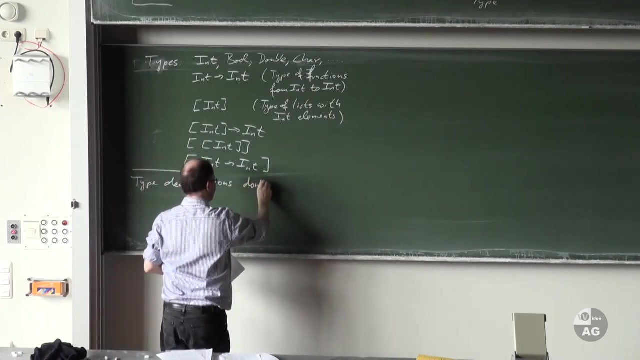 now these type declarations. they don't have to be written by the programmer. if the programmer doesn't write them, then Haskell infers them automatically. so type declarations. so type declarations don't have to be written by the programmer, by the programmer. and if the programmer doesn't write them, then 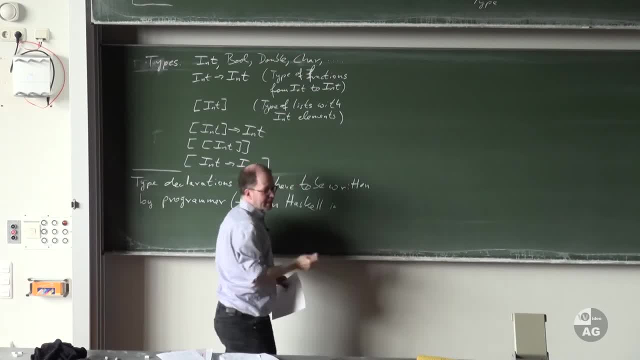 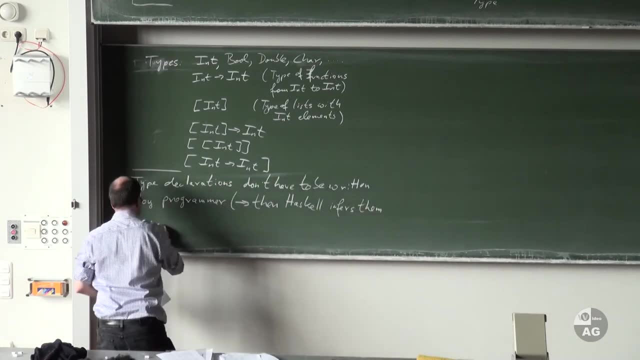 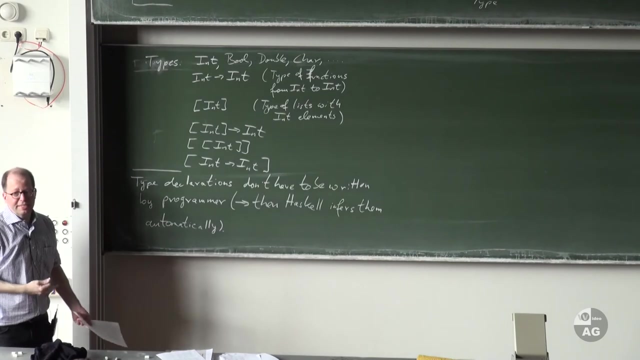 then Haskell infers them automatically. how Haskell does that we will learn later on in chapter four. then Haskell infers them automatically. but if the programmer writes them, then Haskell checks whether the function really has this type. so if your type declaration does not correspond to the definition of the function, 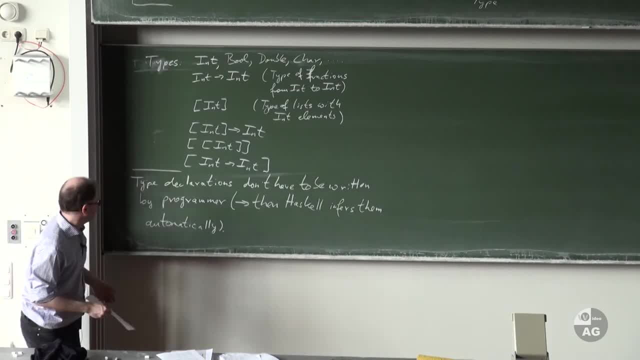 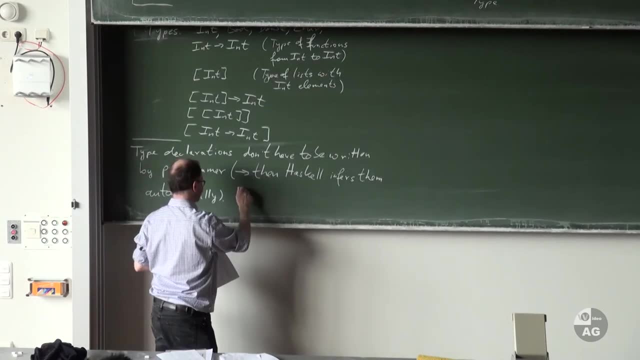 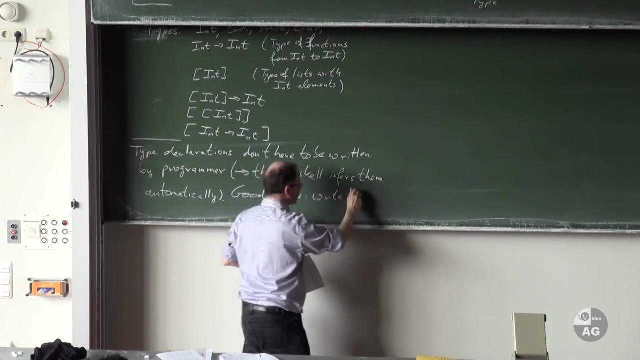 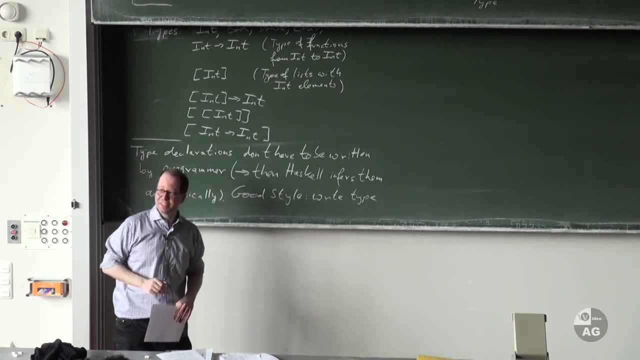 then, well then, the Haskell compiler will notice and it will complain so, but it's good programming style to write type declarations. but, uh, so good programming style is write the type declarations yourself, because then, uh, you can express what you think the type of this function is, and 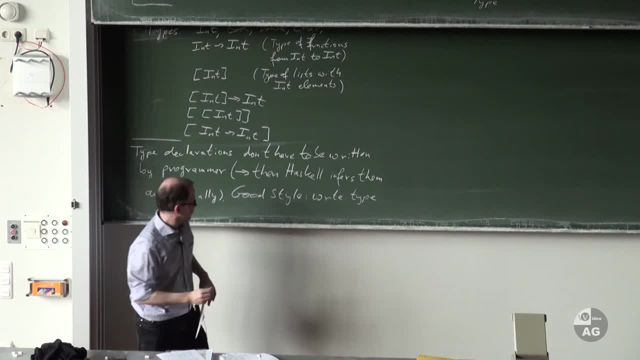 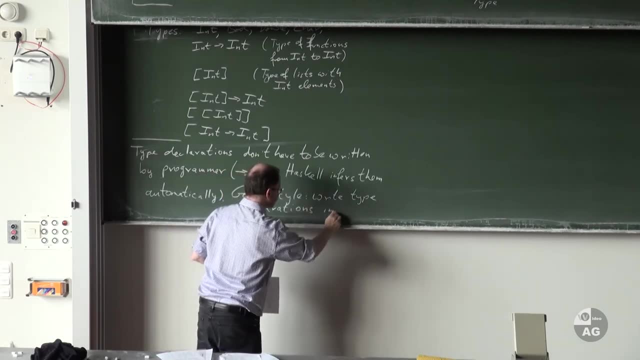 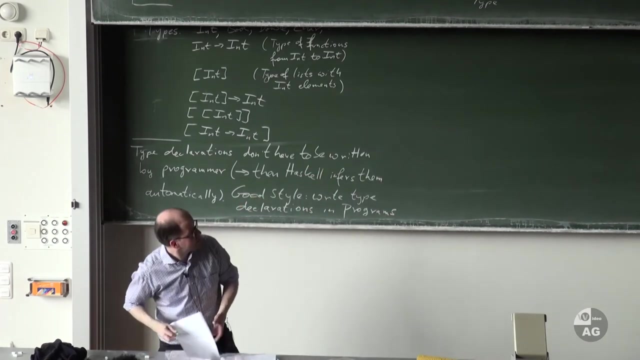 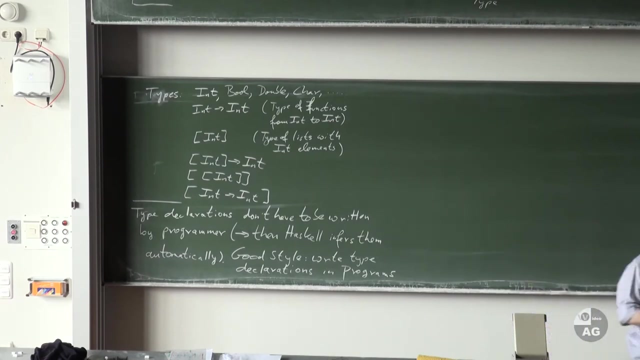 if this does not work, then Haskell will already know when compiling. so write type declarations in your program. and- uh, I need to make the syntax clear here- these variable names, so this var1 and var2, these variable names, so this var1 and var2, these are the names of functions or of variables and in Haskell you can use. 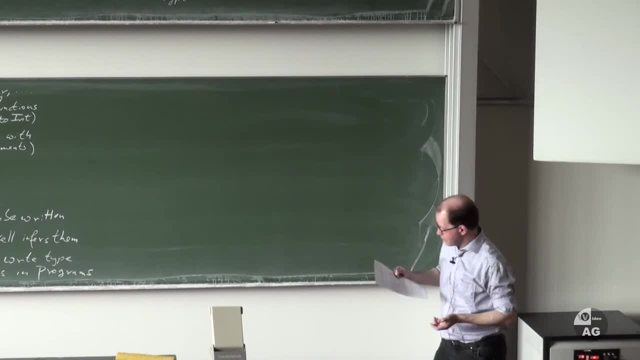 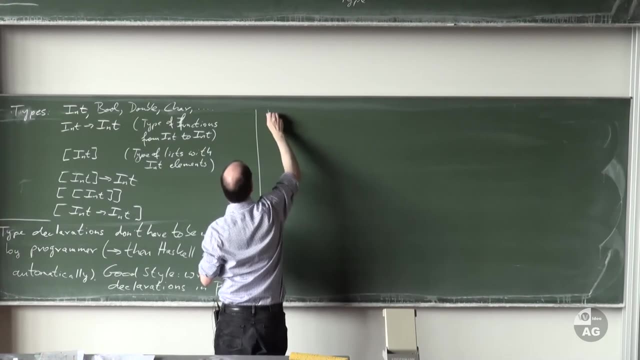 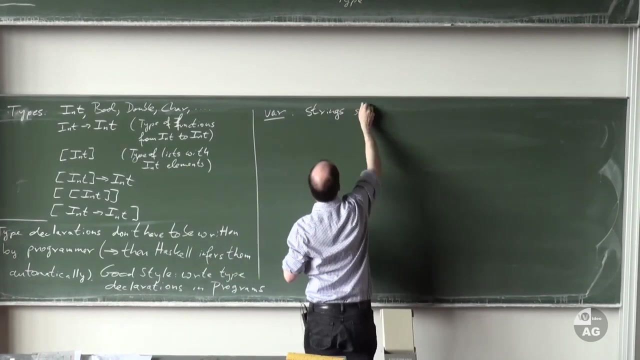 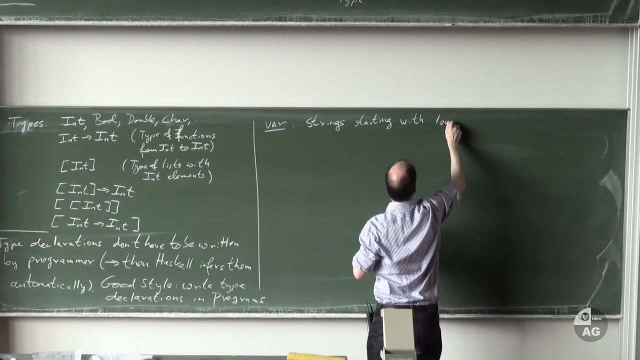 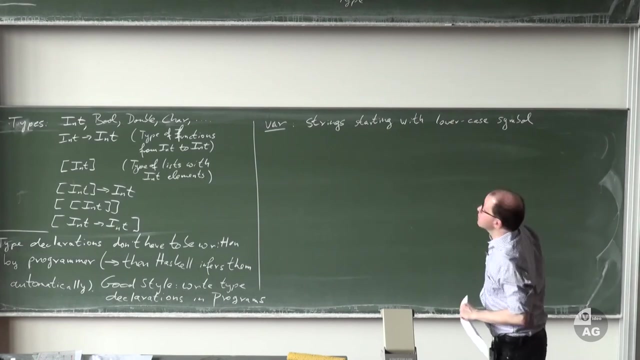 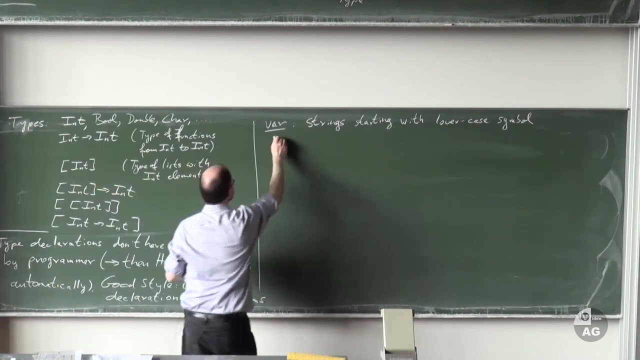 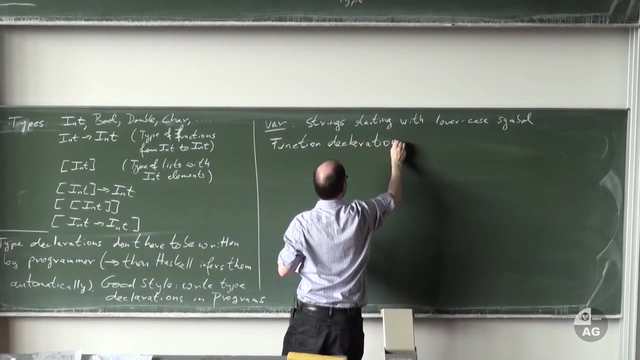 as names for variables or functions. you can use strings, but the strings have to start with a lower case symbol. so so variable names are strings starting with a lower case symbol. so so it's a very complex function. so, as you notice, square and double here start with lowercase letters. 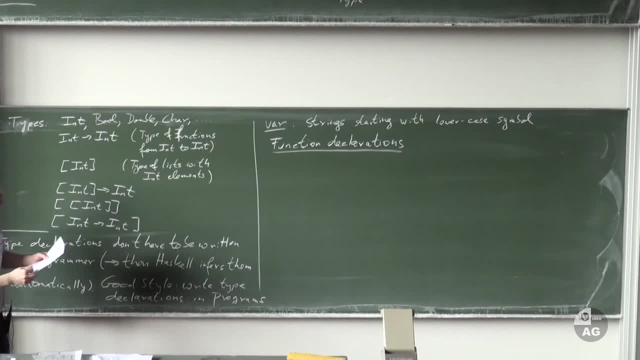 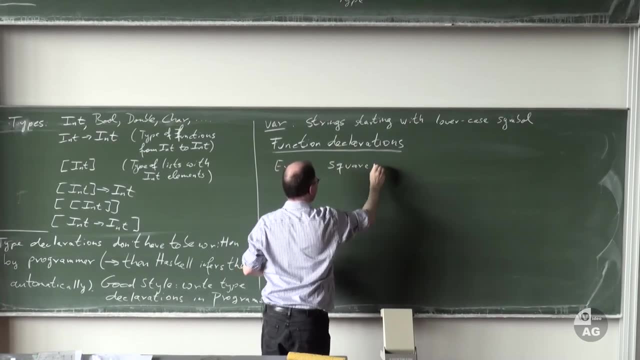 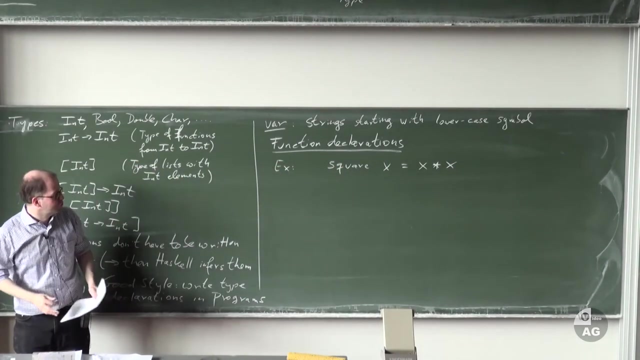 okay, so these are function. these are type declarations. what our function declarations? well, the function declarations now really describe what the function does. let's do it again with square. an example would be something like this: square of x equals x times x, so this describes what square should do. this is the definition of square. 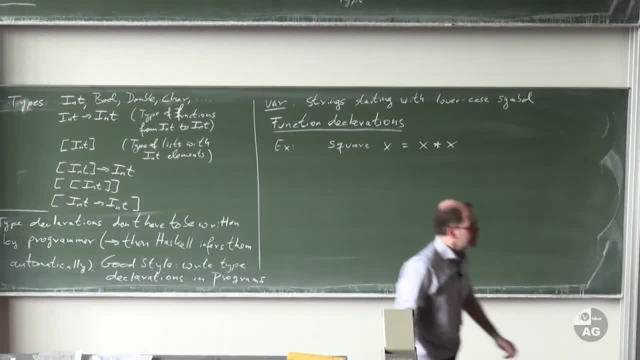 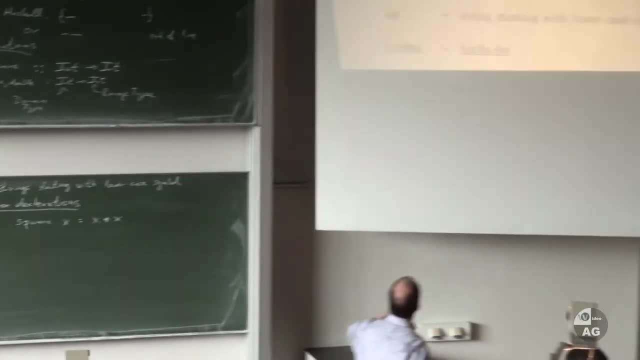 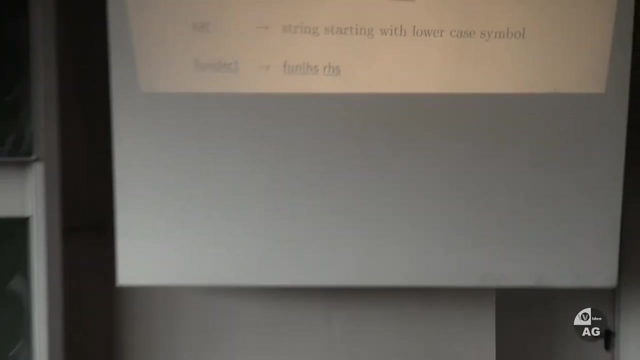 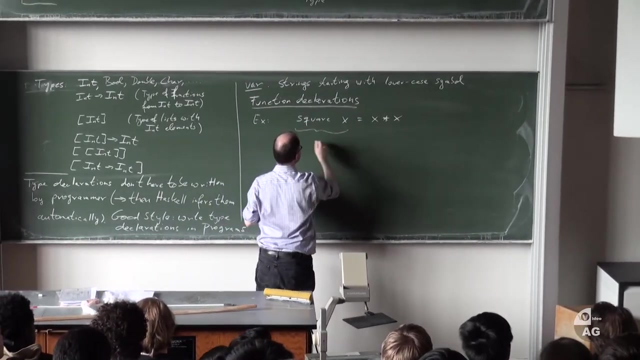 so what is the grammar rule for function declarations? here I also wrote it down: variables are strings starting with lowercase symbols, and a function declaration consists of a function left hand side- LHS- and a function right hand side, and in our example the function left hand side is this: 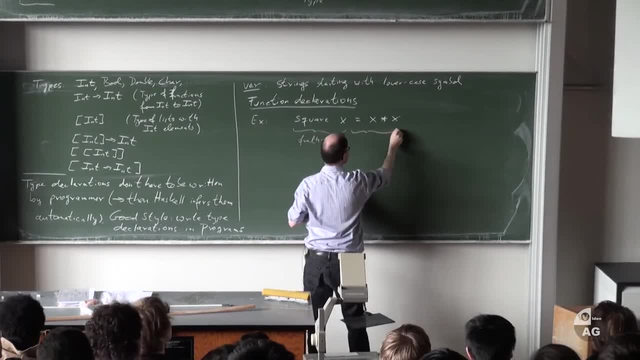 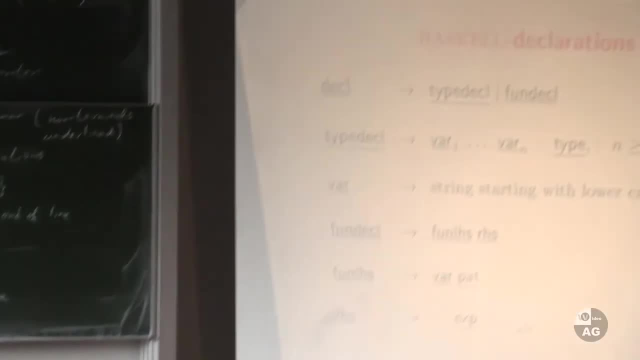 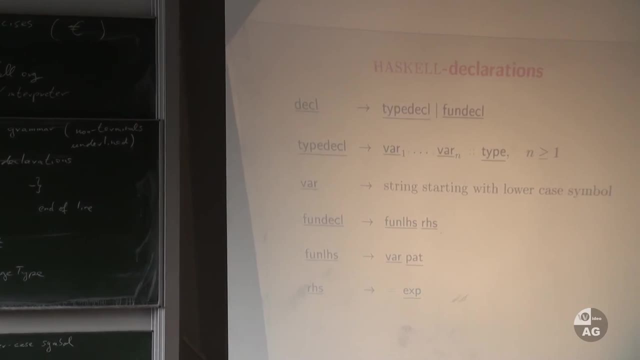 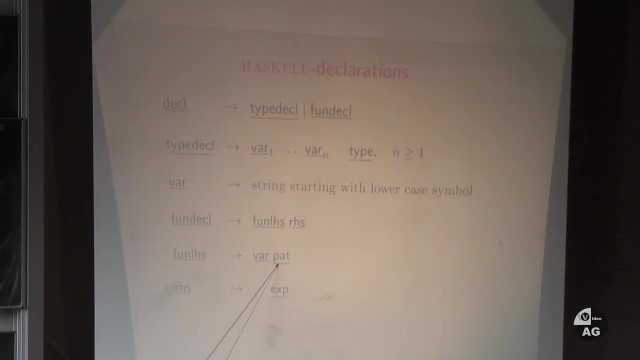 and the function right hand side is this. so what's the grammar rule for left hand sides and right hand sides? well, the grammar rule is the following: the left hand side consists of a variable- that's the name of the function- and a pattern, and this pattern 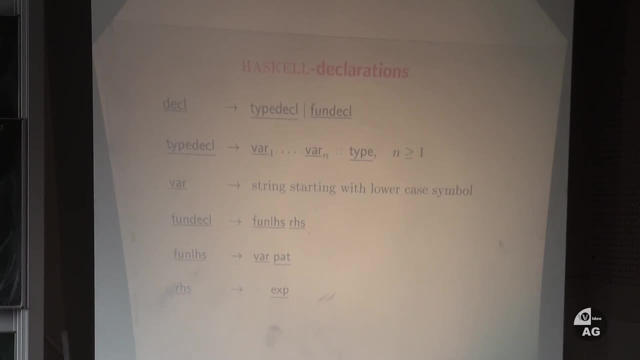 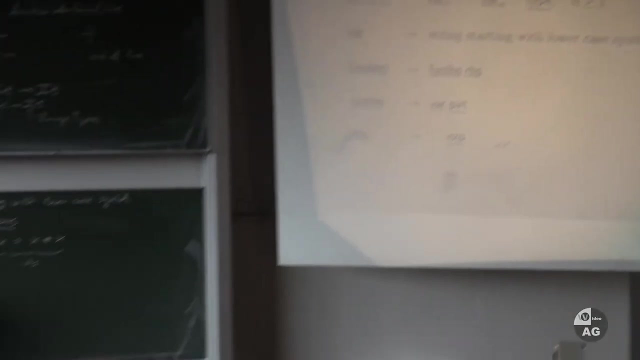 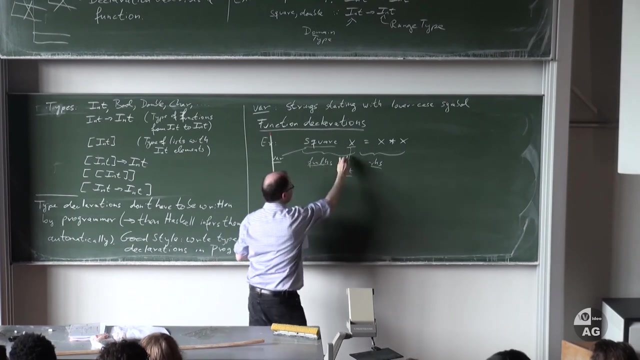 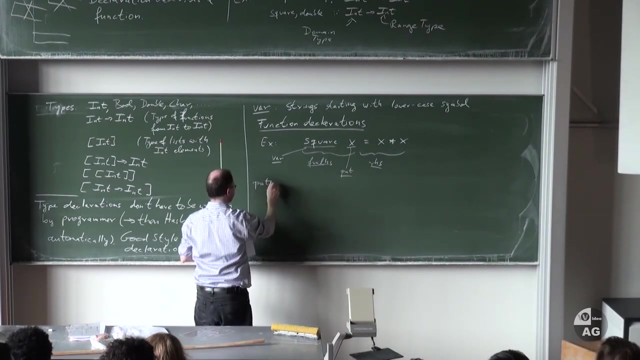 describes the form of the expected argument. so in our example this thing is the variable, so this is the name of the function and this thing describes the expected argument. so this describes that here we expect an arbitrary argument, an arbitrary argument x. so a pattern is a special expression. 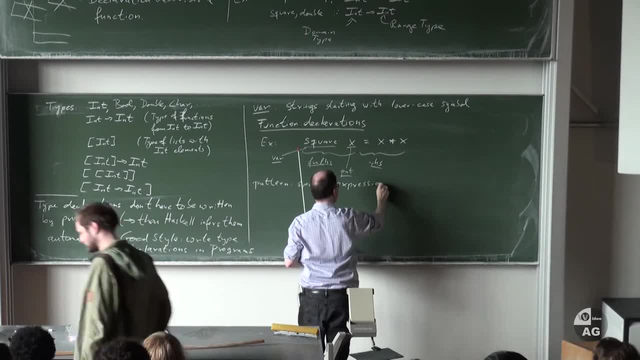 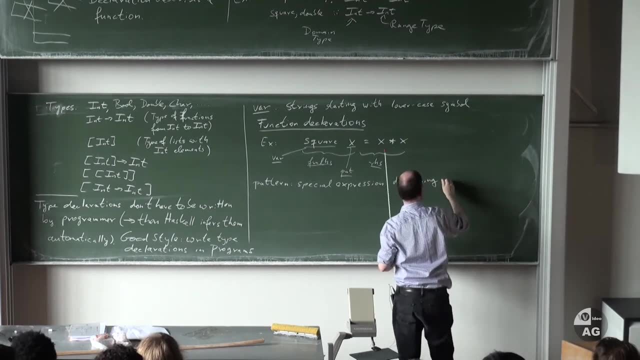 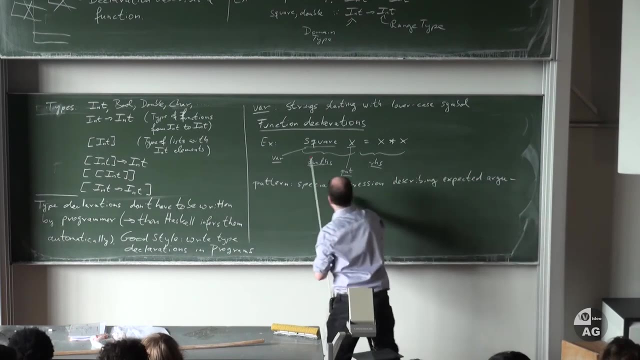 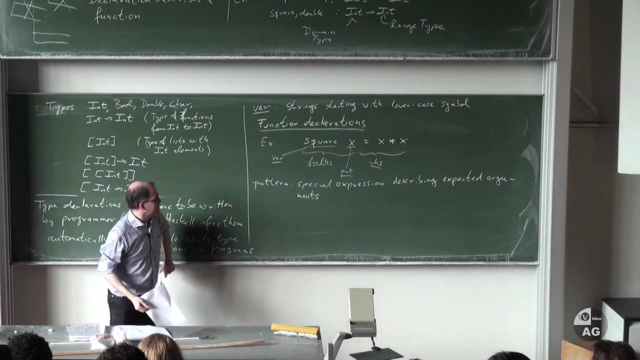 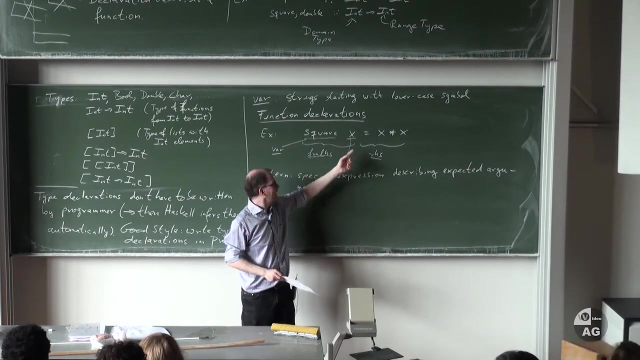 describing the forms of expected arguments. describing expected arguments again, the formal definition of patterns will come afterwards, but at the moment you can, you can think of patterns as something like variables. So a variable describes that any argument is allowed here, So square can be applied to any argument. 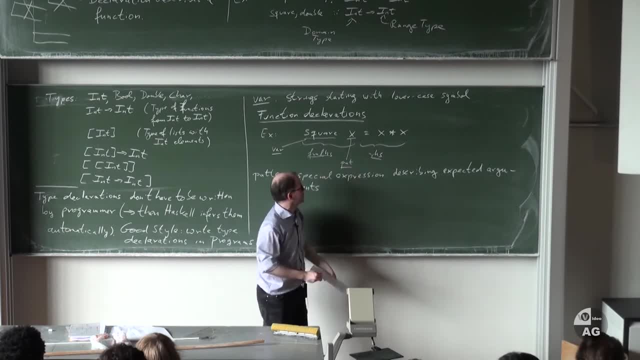 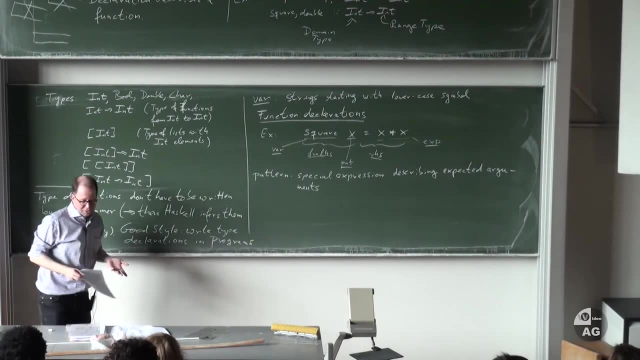 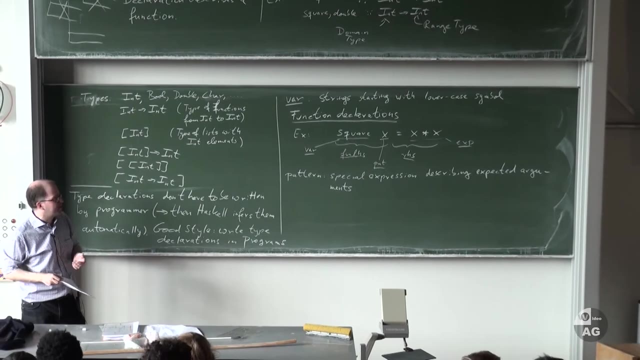 And then the right-hand side starts with an equality sign and then an expression. So this thing here is an arbitrary expression. And well, how expressions look like, we will see very soon, And one possibility is something like this: So you take two variables and you apply a function to them. 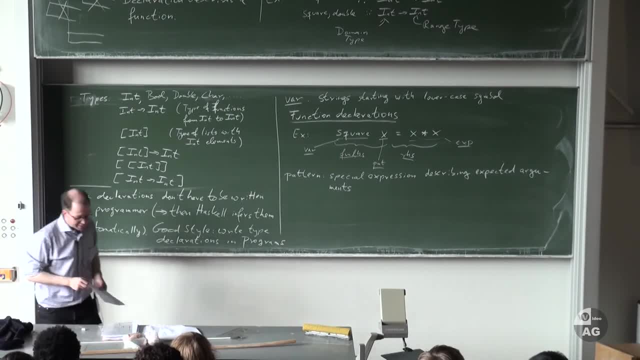 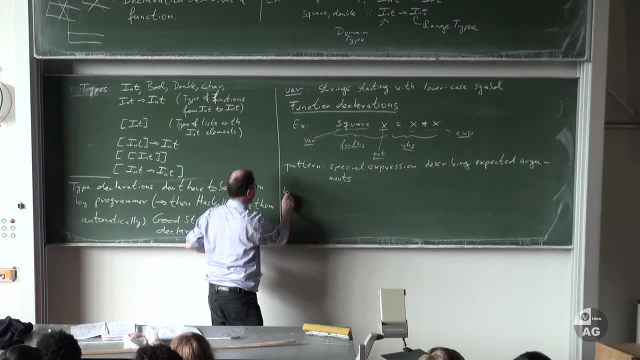 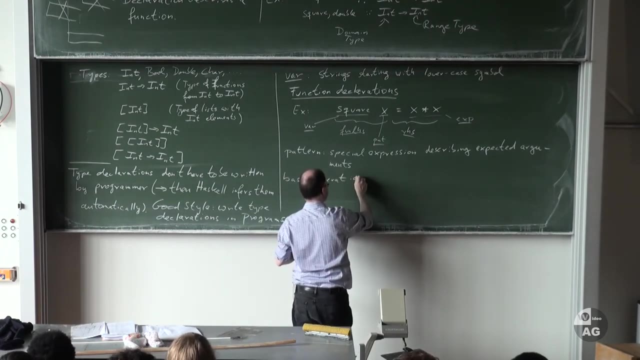 And this star is a function that is predefined and it computes multiplication, as you would have expected. So basic operations in Haskell are predefined in Haskell. So what are basic operations that are predefined? Well, arithmetic, basic operations like plus, minus, multiplication, And well, division is also predefined. 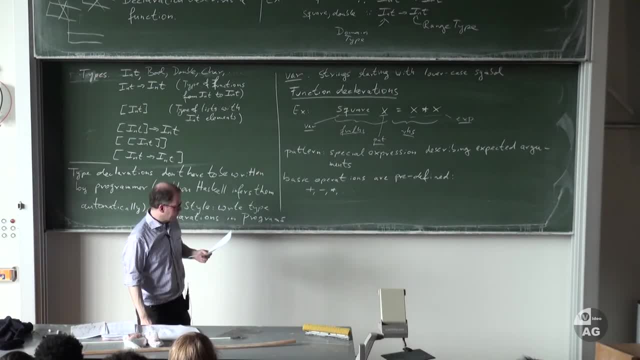 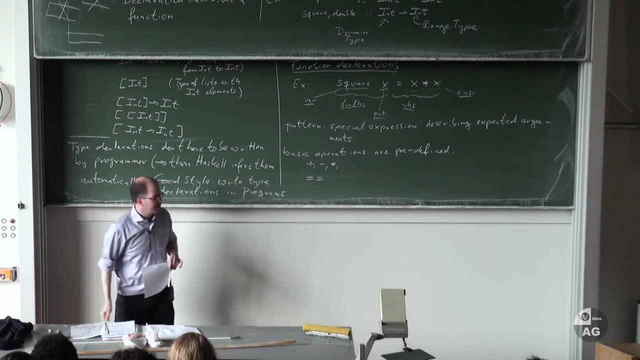 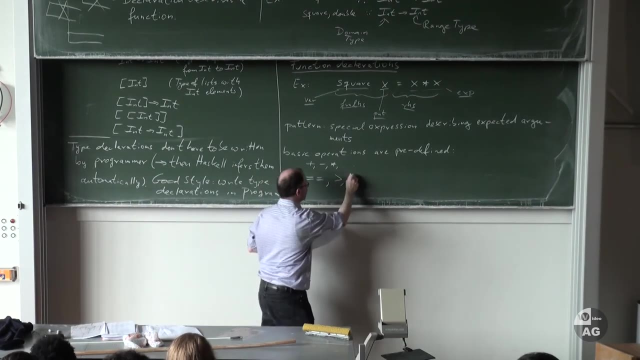 And modulo is defined and so on. So these are basic arithmetic operations. Then comparison operators are also predefined, So for example something like this: This checks whether two values are equal And something like greater or greater equal. So these things are predefined as well. 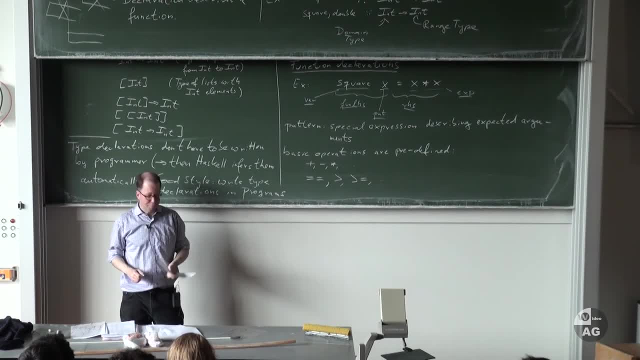 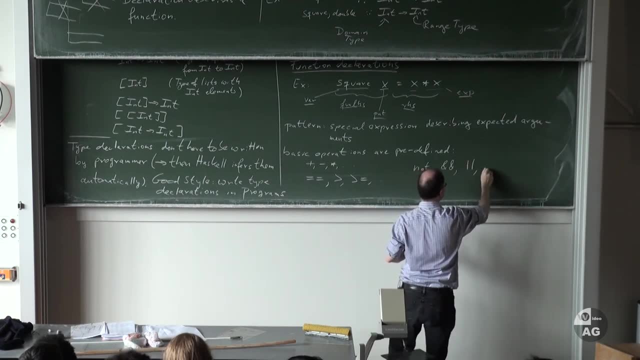 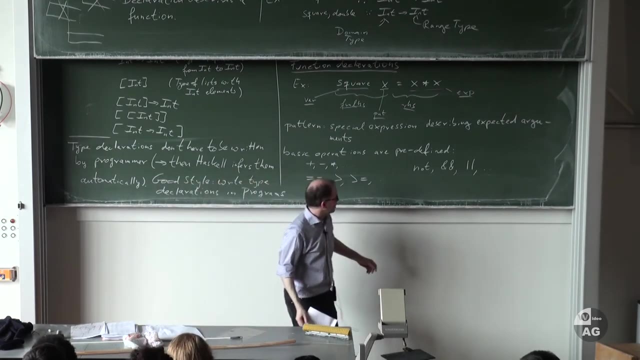 So comparison operators are predefined, And Boolean operators are also predefined, So something like not, or and or or, So these things are predefined as well. So this syntax is like in C or Java, except that not is not exclamation mark, but not. 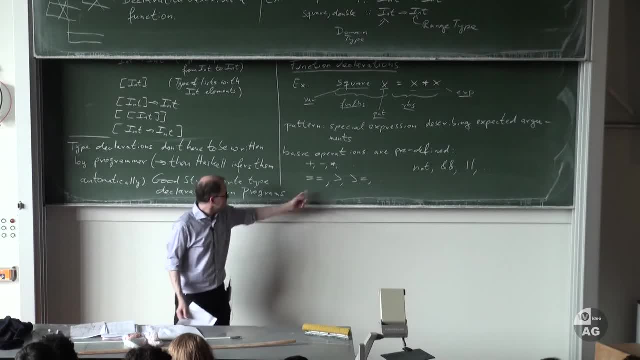 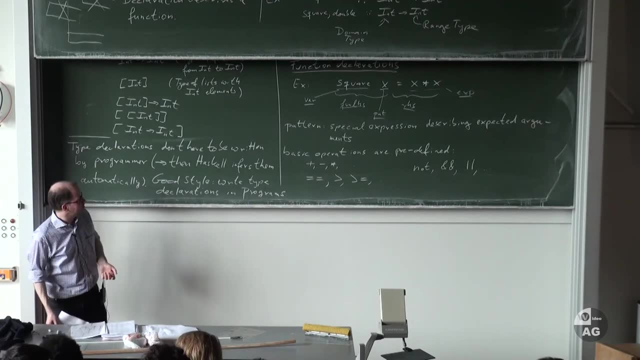 But the syntax for and and or is the same, And the syntax here is the same, The syntax here is the same as well. So nothing new. I mean this is predefined, like in imperative languages. Nothing special, We have basic operations. 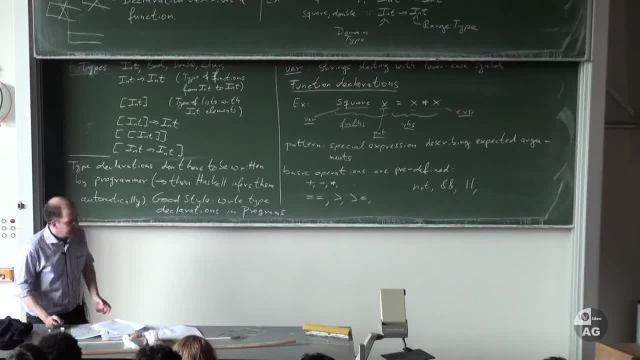 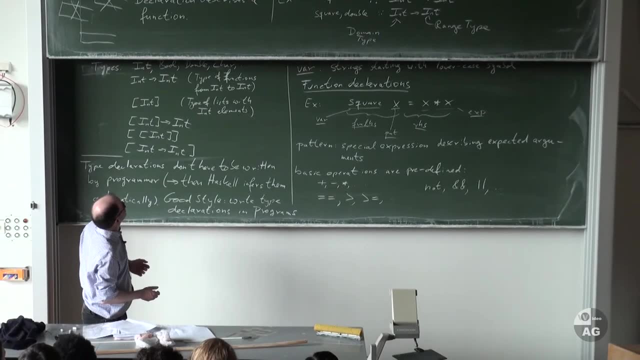 OK, so this is the syntax of function declarations. And now, if I have a program like this, so this square program with the type declaration up there and the function declaration down here, how can I execute it? Well, we have this already. 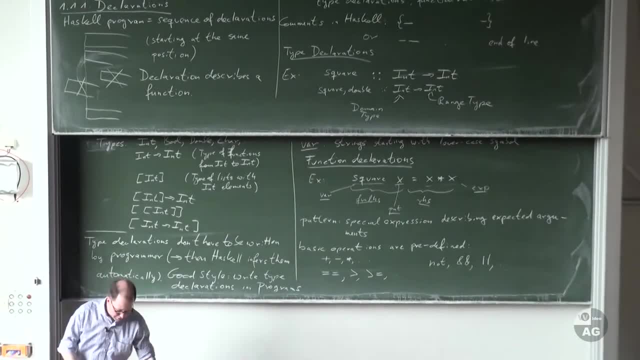 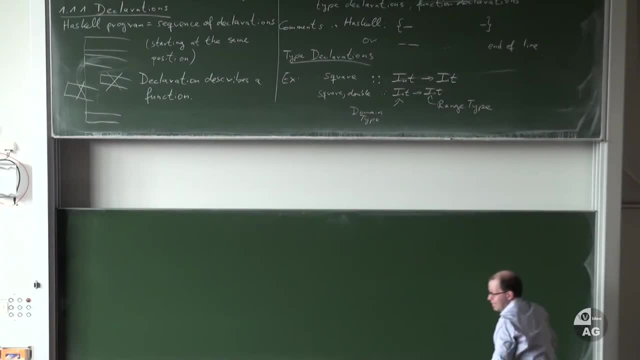 We write down an expression And then this expression is evaluated. So let's discuss this a bit more. OK, so the execution of a functional program. What's the general idea? So let's execute our square program that I just wiped away. 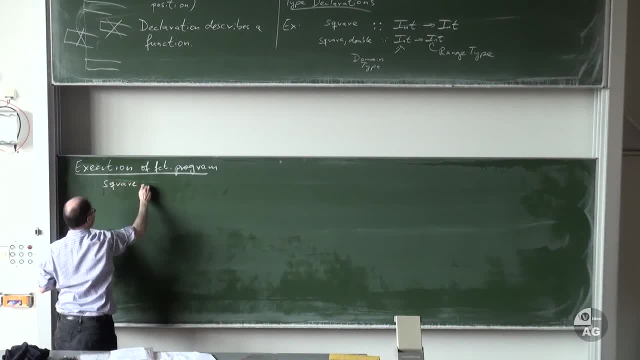 So I'll write it down again so that we can see it. So we had this square program And square is a function from int to int. This was square, It was the type declaration And the function declaration was the following: Square of x equals x times x. 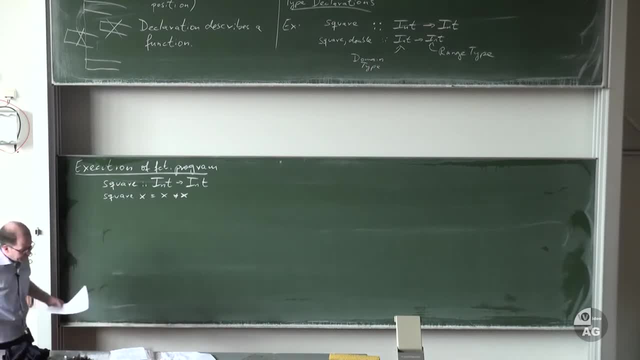 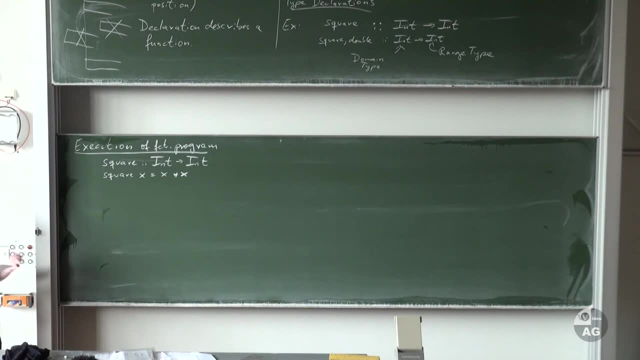 And now, how does evaluation work? Well, the idea is that in the Haskell interpreter, you type in expressions, You press Return And then Haskell tries to evaluate this expression. And the idea for evaluating this is: well, I'm going to do this. 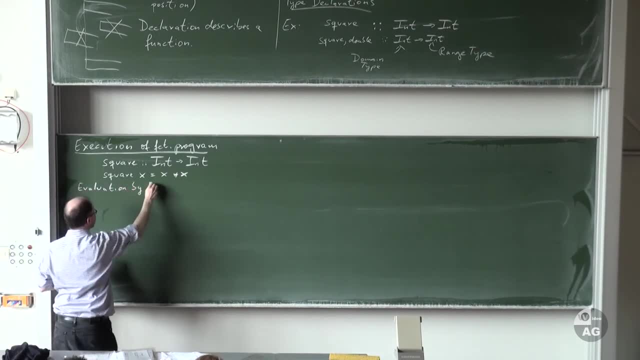 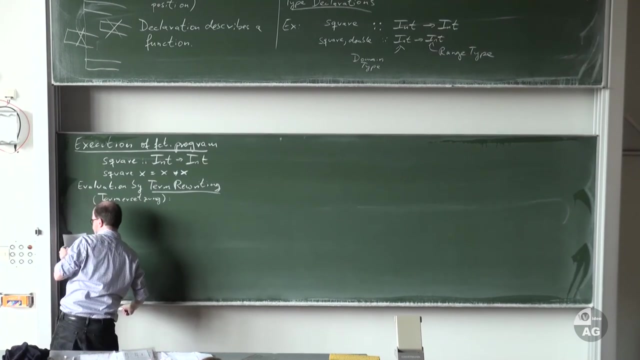 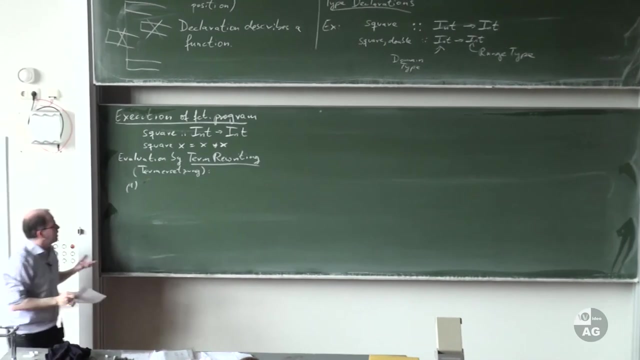 Term Rewriting- Evaluation by Term Rewriting in German. so this is the evaluation mechanism that is used, And it works as follows: In the first step, well, you have an expression that you want to evaluate, And in the first step, Haskell tries to find some sub-part. 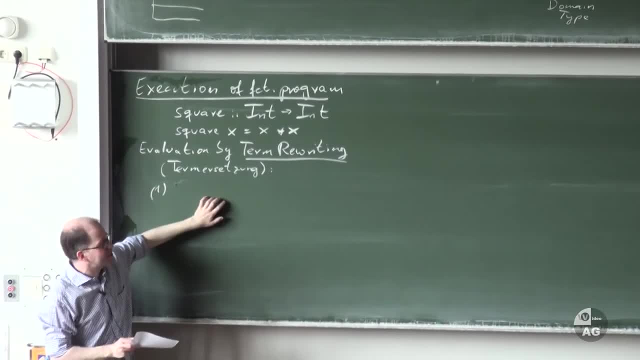 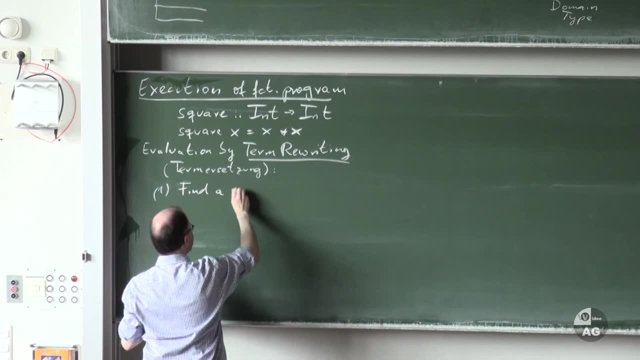 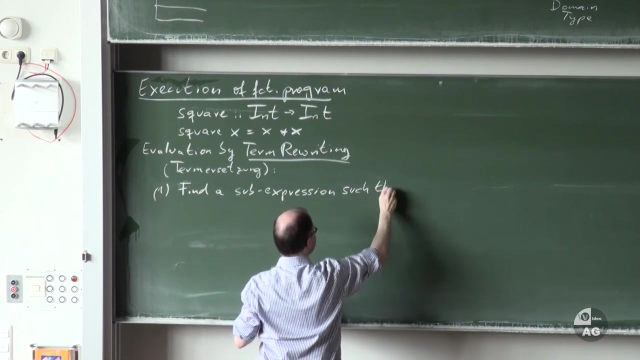 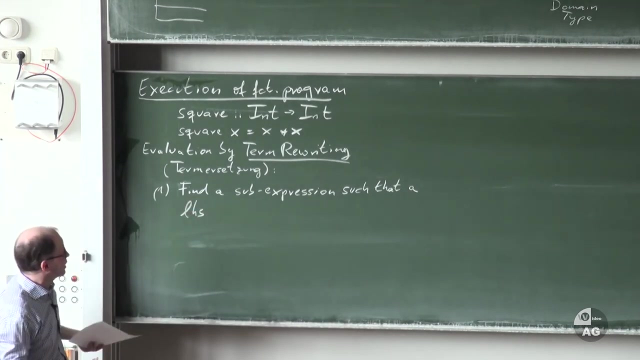 of this expression Such that the left-hand side of an equation matches this sub-expression. So the first part is find a sub-expression of the expression that we want to evaluate such that a left-hand side LHS a left-hand side of a defining equation. 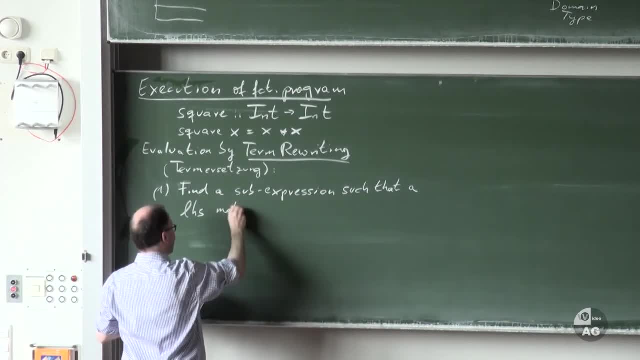 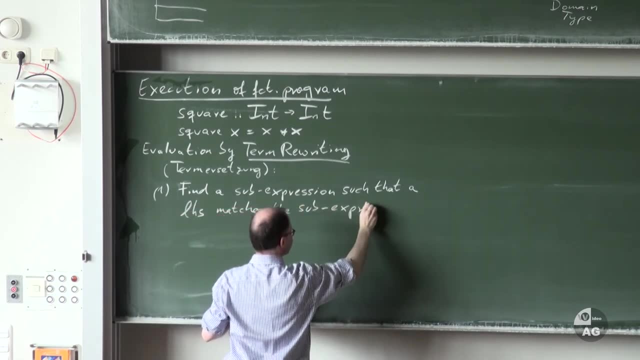 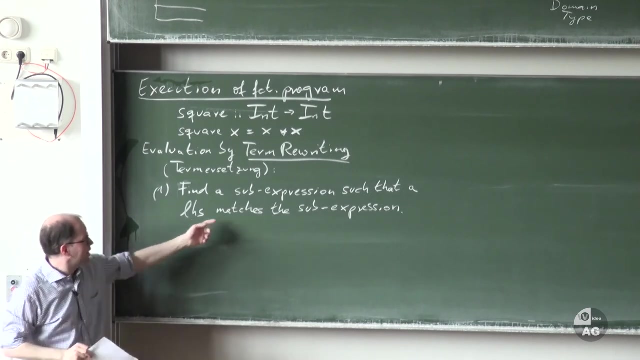 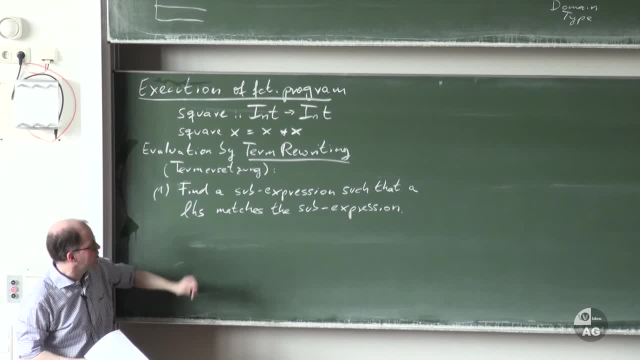 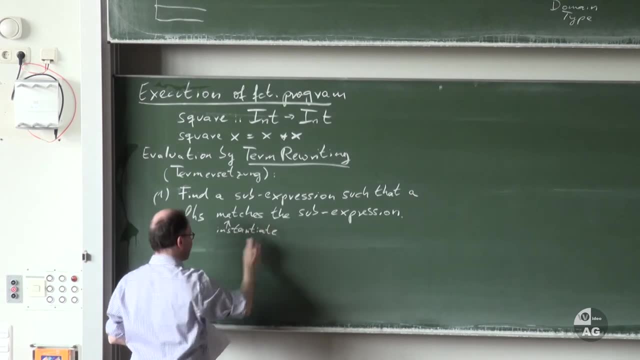 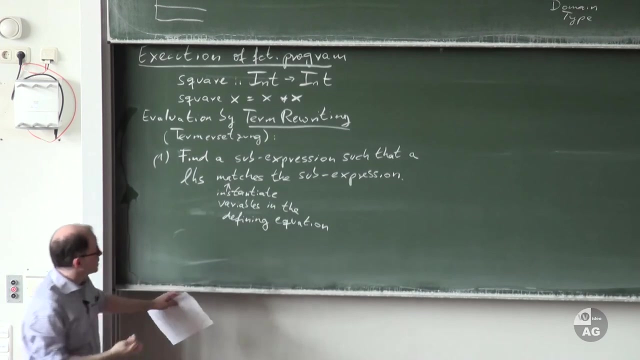 that this instantiated left-hand side becomes equal to the sub-expression. So instantiate the variables in the defining equation. And once we have found such a defining equation where the left-hand side matches the sub-expression, the second step is to replace the left-hand side. 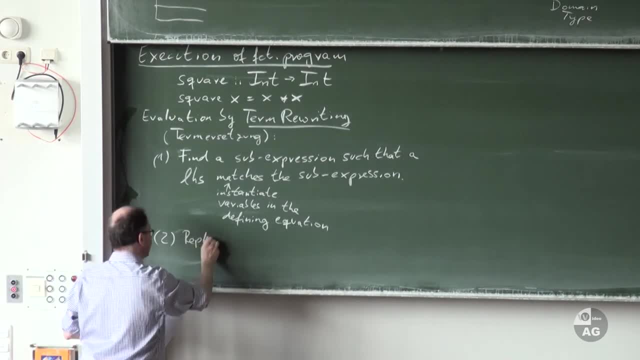 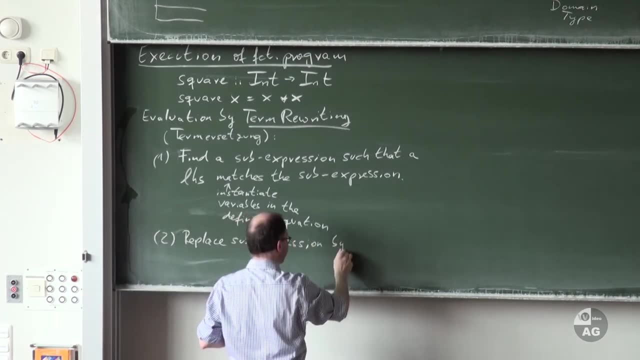 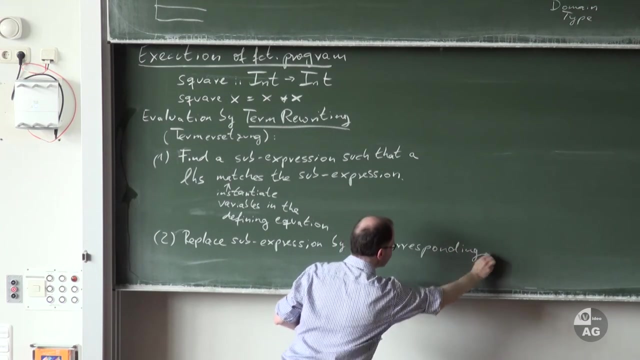 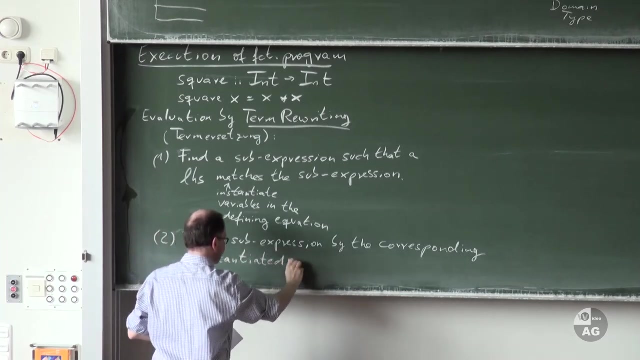 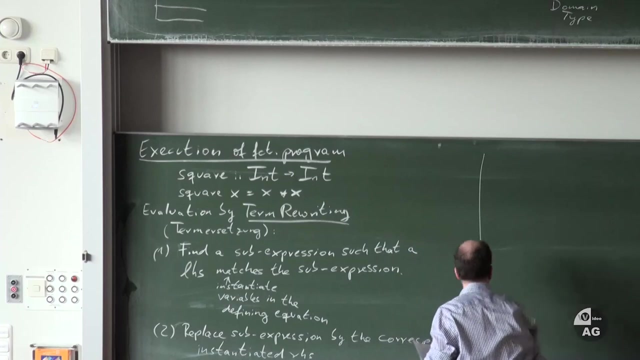 by the right-hand side. Replace the sub-expression by the corresponding instantiated right-hand side. I will do this by an example in a minute. Replace the sub-expression by the corresponding instantiated right-hand side. Okay, so let's look at an expression. 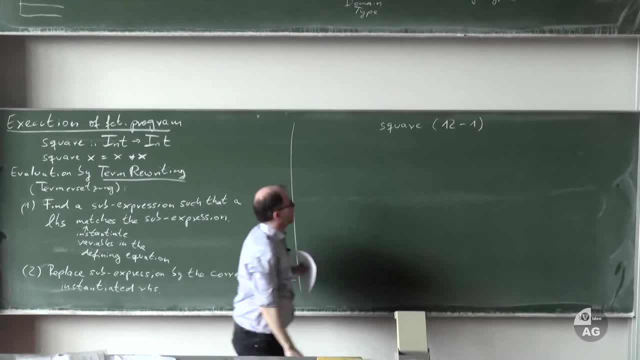 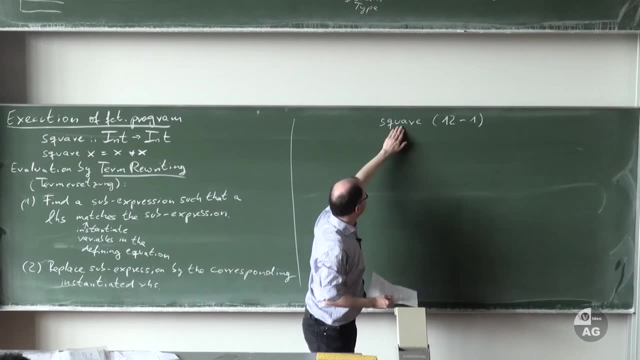 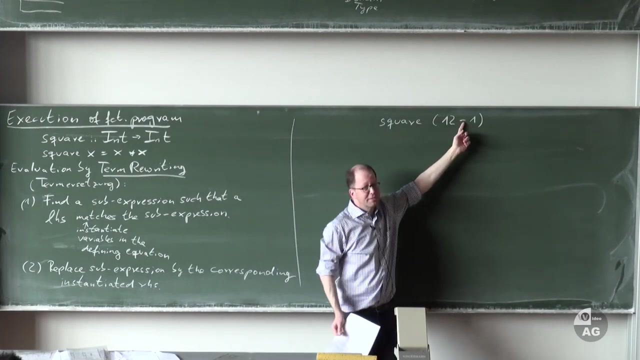 Square of 12 minus 1.. If I want to evaluate this now, there are two principal possibilities I can try. I can try to evaluate the square here, and I have an equation which tells me how a square is defined. I could also try to evaluate this minus. 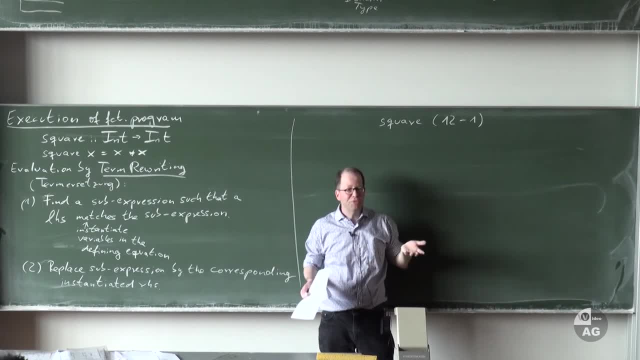 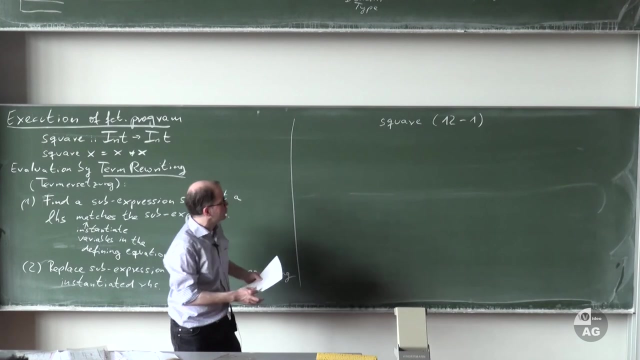 because minus is predefined. So there are equations for minus built into Haskell, and these equations would allow me to compute something like 12 minus 1.. It would find out that the result of this is 11.. So two possibilities. What should we evaluate? 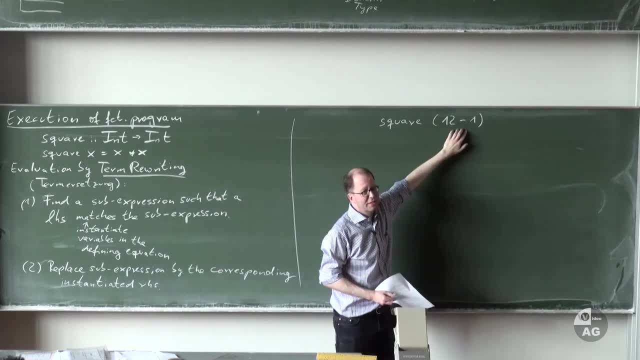 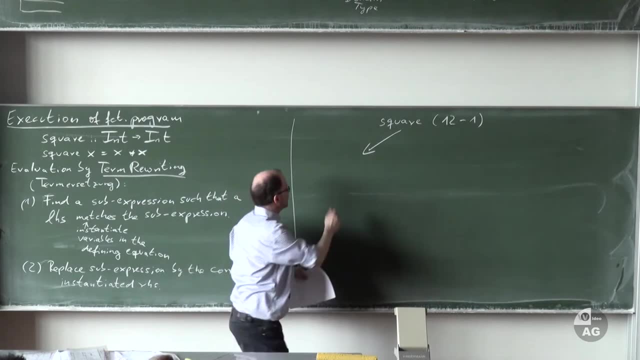 Should we start with evaluating square or should we start with evaluating minus? Let's start with evaluating minus. If I evaluate minus, then I evaluate this sub-expression. So this is the sub-expression which is evaluated and I get square of 11.. 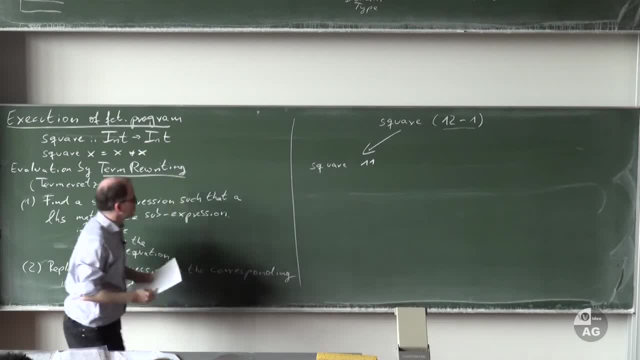 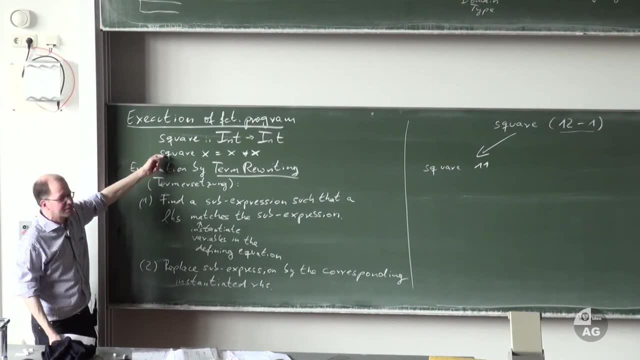 Now I can continue the evaluation and I follow these two steps. So I look for a defining equation such that the left-hand side of this defining equation matches some sub-expression here. So I find this and now the question is: can I instantiate this? 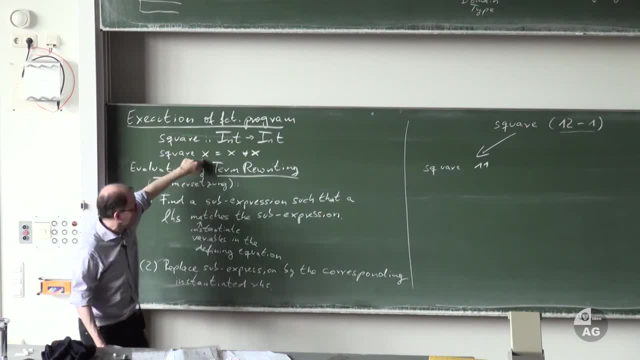 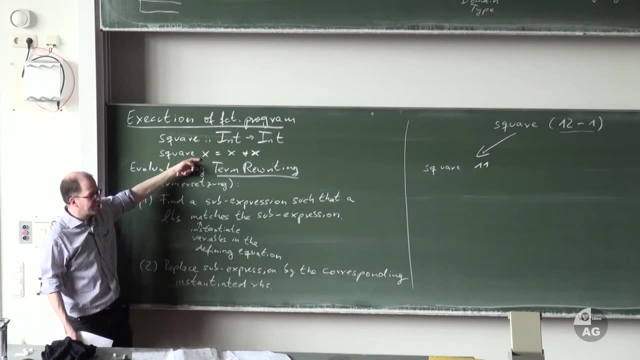 Can I instantiate the variable here in such a way that it becomes equal to this expression here? Yes, of course I can instantiate x by 11. Then I have square 11 here and therefore I can replace this instantiated left-hand side by the corresponding instantiated right-hand side. 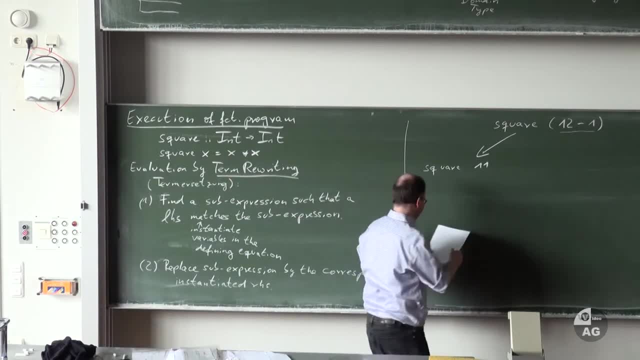 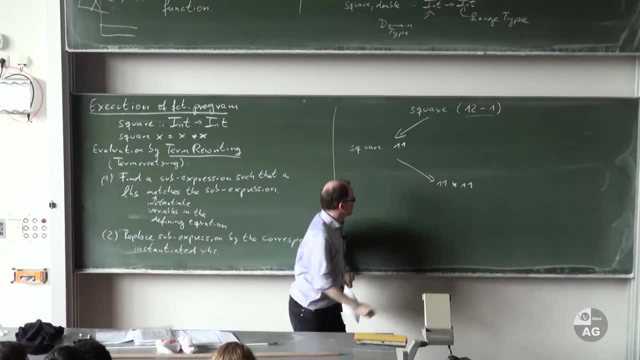 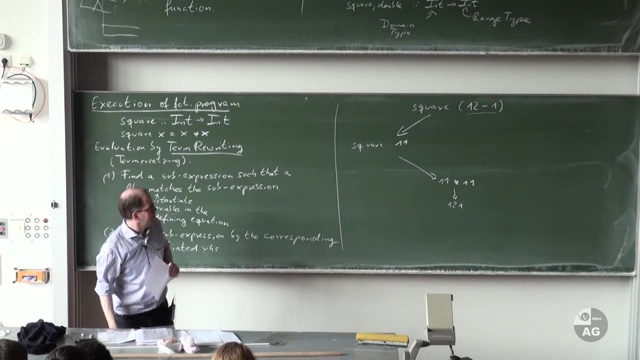 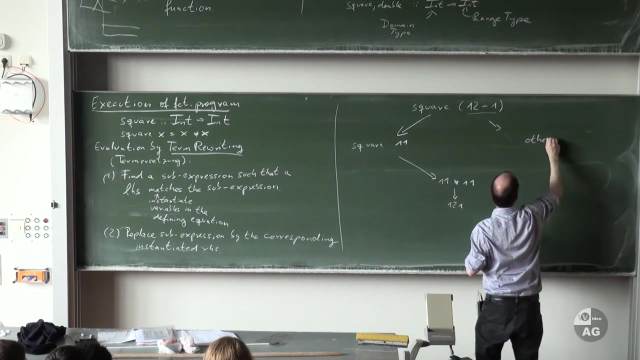 So x is instantiated by 11, and so I get 11 times 11.. And now evaluation can continue and I get 121.. But of course I could have done this differently. I could have started with evaluating square and then I would get other possibilities for evaluation.